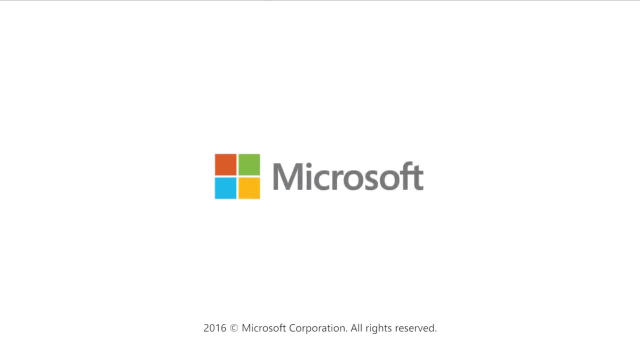 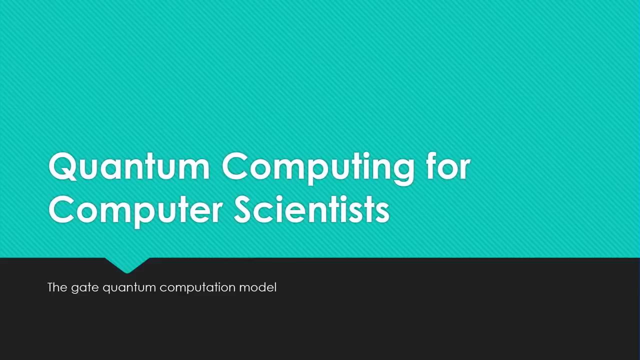 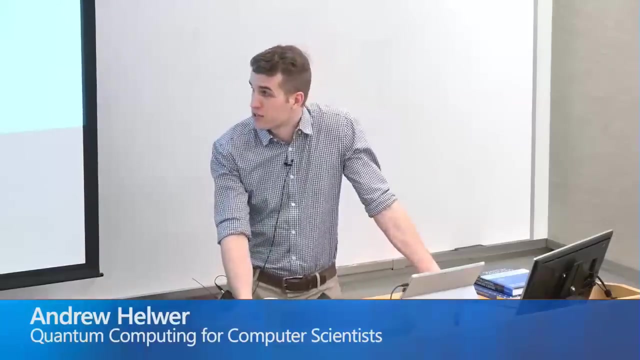 Welcome to Quantum Computing for Computer Scientists. Happy Valentine's Day. We will learn about this most romantic of all subjects: quantum computing. This is a talk aimed at computer scientists. We will not go over very much, if any, physics during this talk. 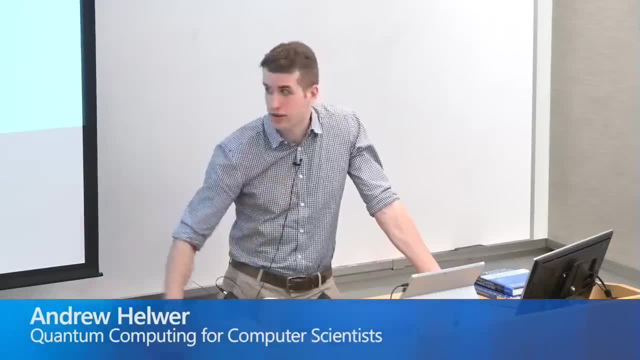 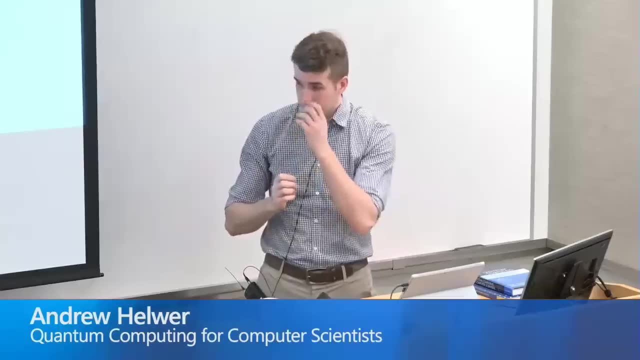 We won't go over like the double-slit experiment or uncertainty principle. We're not learning about any of that. We're going to come up with a computational model which you will all find it fairly intuitive, I think. Use a state machine. 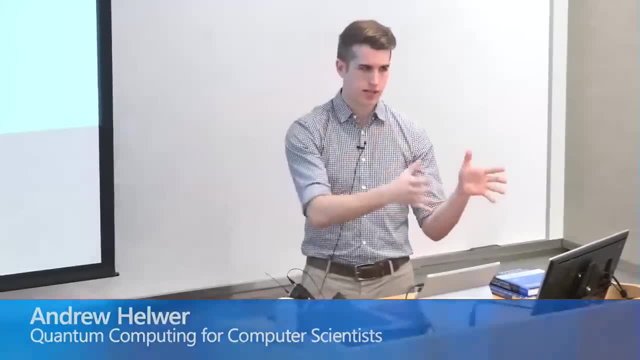 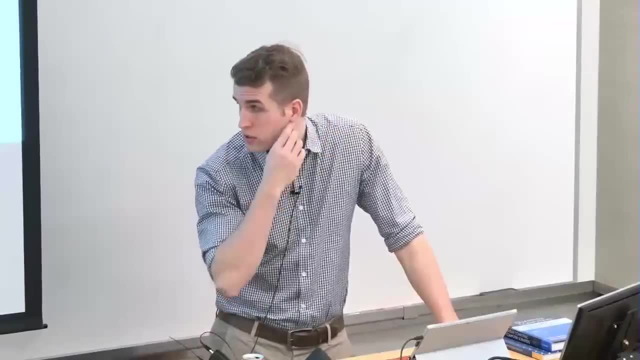 We will run a quantum algorithm on it, show that it outperforms a classical computation model, and then we'll end with some demos, including a running program in Q-sharp, Microsoft's quantum language. This is the gate quantum computation model. 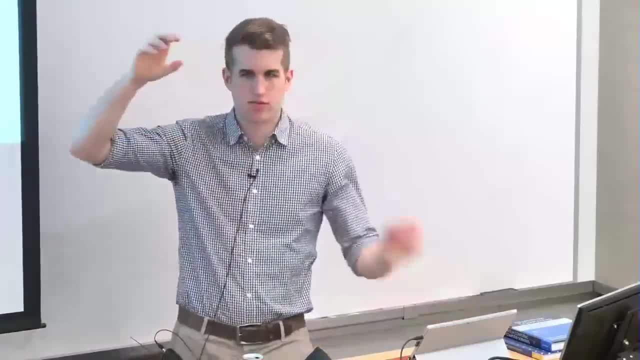 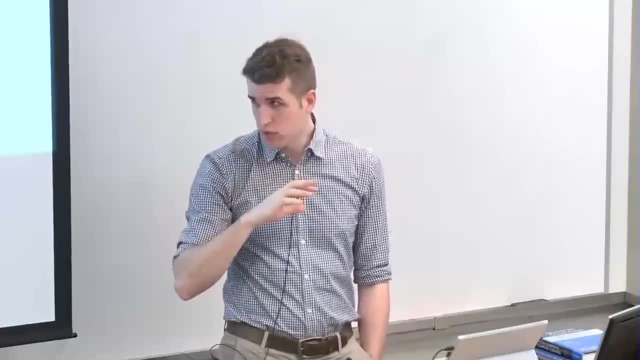 It looks a lot like the classical computation model, where you have bits and you send them through logic gates and transformations are applied to them. There's another computation model called the quantum annealing model, which is used by D-Wave. If you've heard of that, that's something. 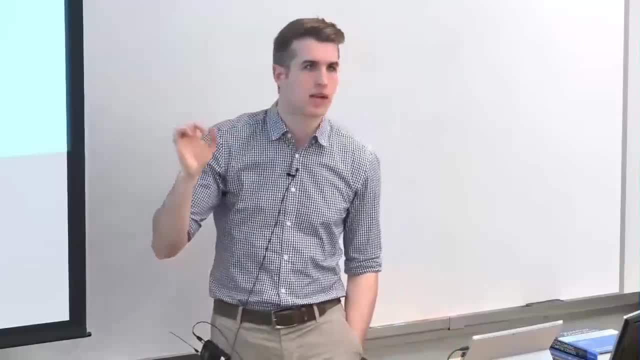 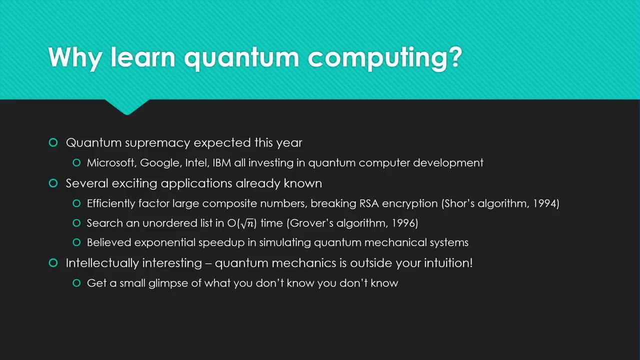 different from what we'll be going over, but people think they might be equivalent. The jury is still out on that. Anyway, I'm sure you'll have a great time, So I'm sure all of you have your reasons for being here. 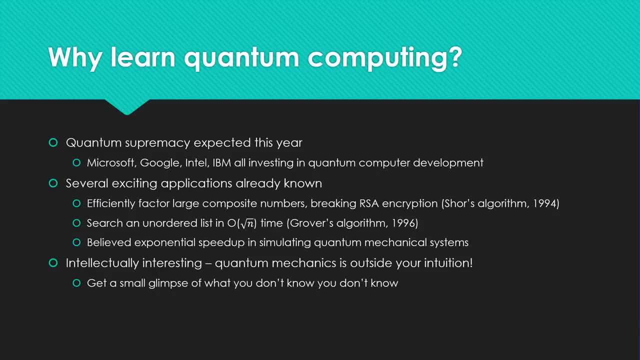 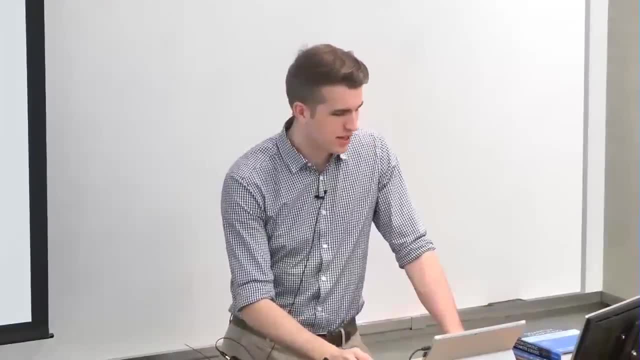 but here are three reasons I've come up with if you need some additional convincing why you should learn quantum computing. The first is that quantum supremacy is expected this year, this very year. Quantum supremacy means we have a real problem running on a real quantum computer. 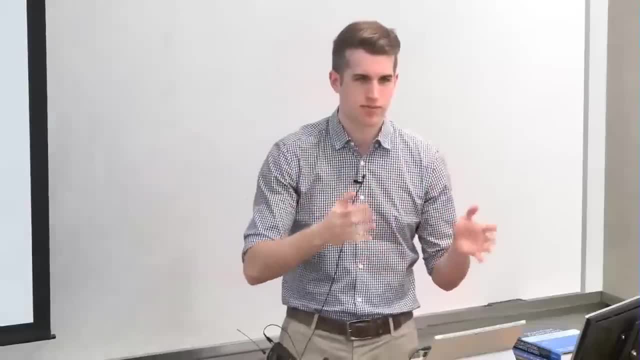 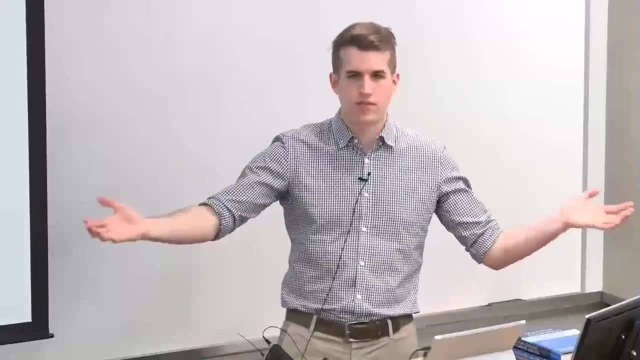 which in real time runs faster than the same problem on a classical computer. So Google has announced they think they'll do it this year. If they do, it's a really big thing. So it might be in your future- Who knows- Five, ten years. 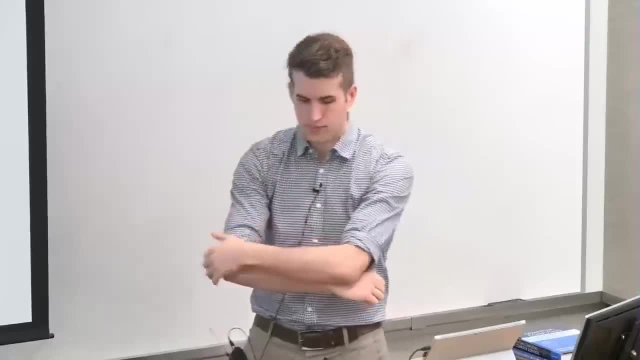 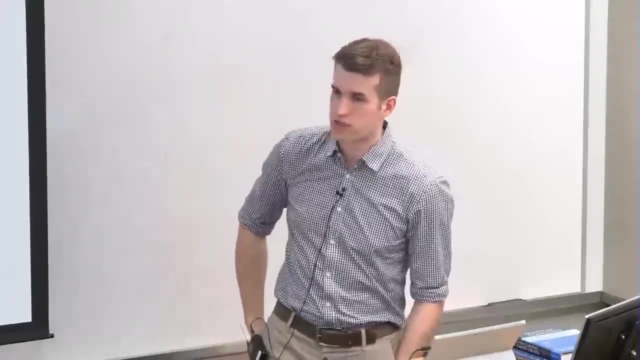 we could all be running some really tricky problems on quantum computers. So we have lots of large companies: Microsoft, Google, Intel, IBM. they're all investing billions of dollars in quantum computer development. There are lots of really exciting applications. This is the one that everyone's heard. 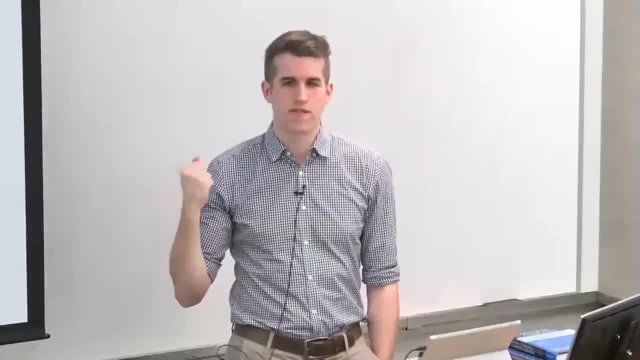 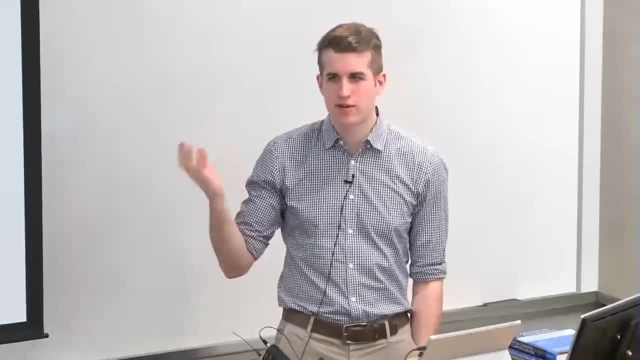 about Shor's algorithm. When this paper came out, it lit the world on fire. People were like, wow, quantum computers could actually have real economic impact. We could factor RSA and undermine our global financial system, which is pretty cool. Here's one that programmers will, I think. 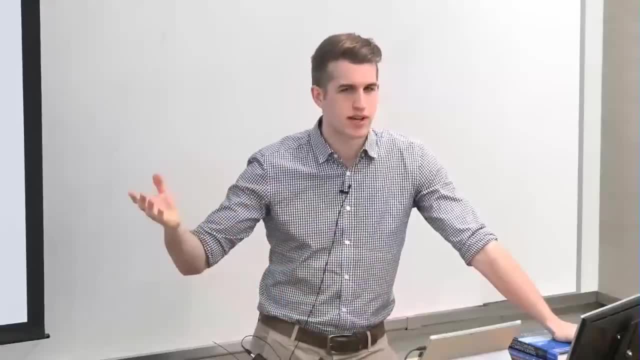 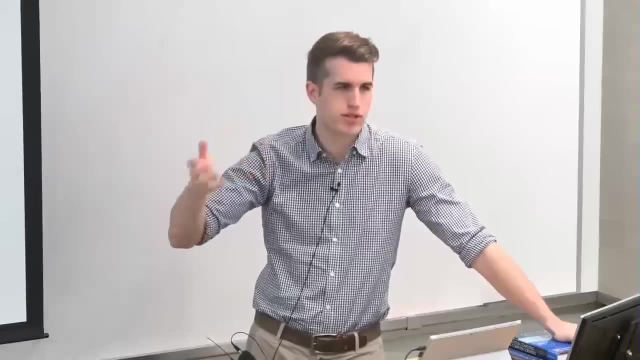 appreciate, which is we can search an unordered list in square root n time. So you think for an unordered list you have to check every element. that's o? n You can just get a nice speed up just square root n queries on a quantum computer. 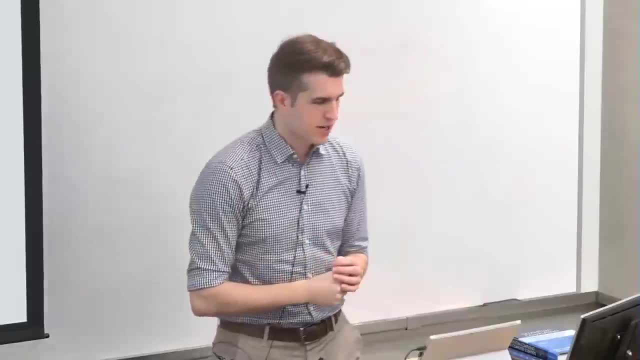 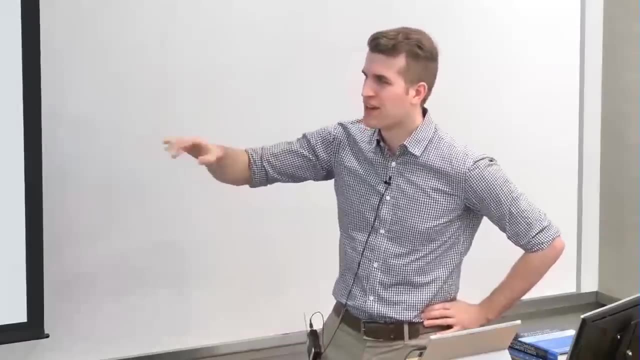 which is pretty nifty, generally useful. Here's the one which I think probably is the best probability of change in the world. Sorry, programmers, square root n search probably won't change the world too much, which is we might be able to have. 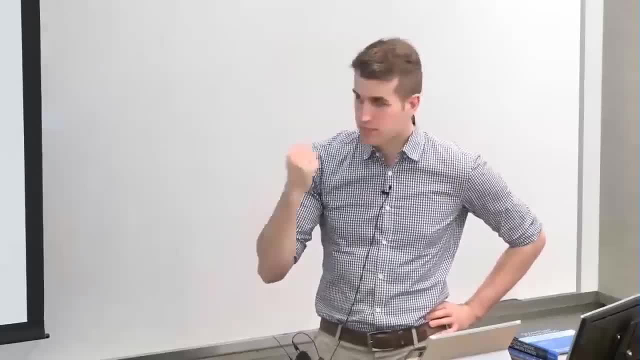 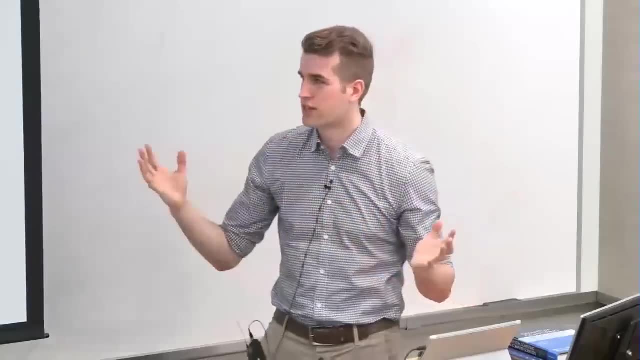 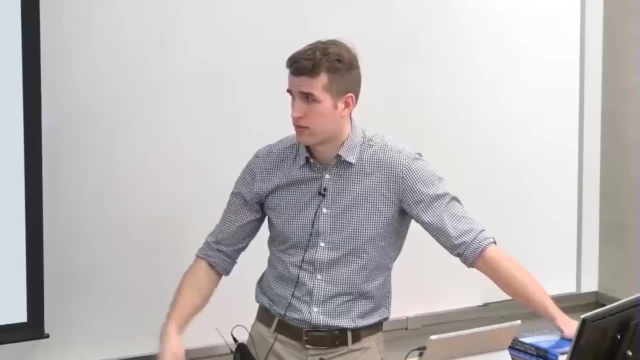 an exponential speed up in simulating quantum mechanical systems. So things like drug design. if you simulate biological molecules interacting, things like that, it could massively speed up a lot of our biological research. Everyone talks about nitrogen fixation for this. That's part of the main Microsoft. 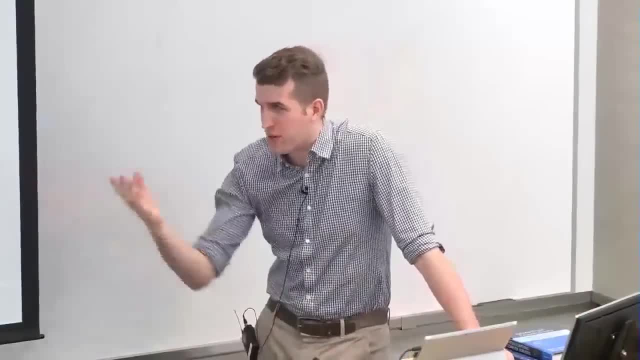 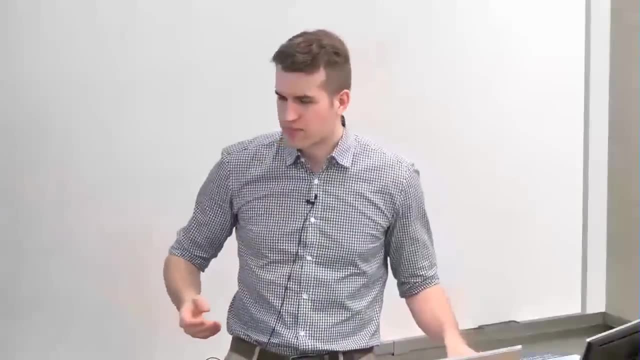 sales pitch, but this is the one that actually motivated me, the bottom one, which I think, from talking to a couple of you before the presentation began, also motivates you. It's intellectually interesting, and it's interesting because it's just kind of outside my intuition. 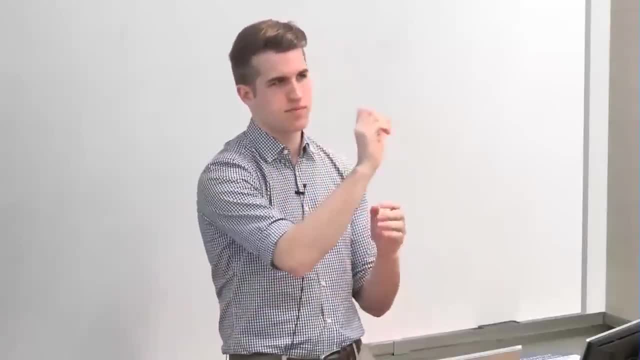 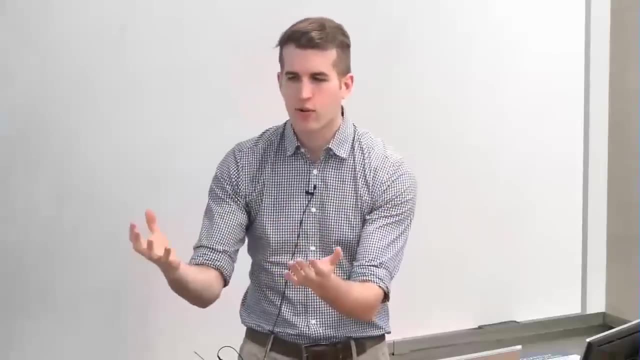 I think all of us at this point in our careers can basically look at any digital or mechanical system and have a ballpark idea of how it works. right. But if you look at a quantum computer, how can a quantum computer outperform classical computation? 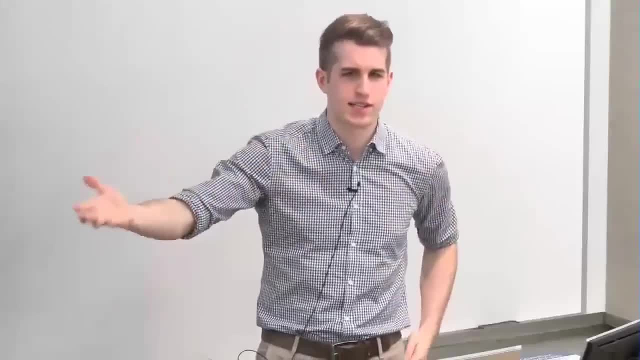 It doesn't make any sense. There's no way I can even start to guess how it would work, and so I really wanted to learn it, And I think there's a reason for this, and this is kind of getting a bit philosophical. 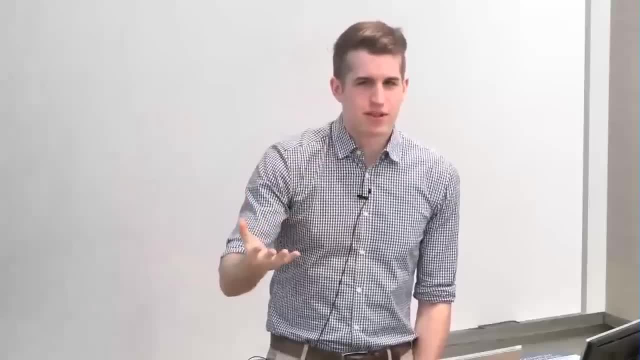 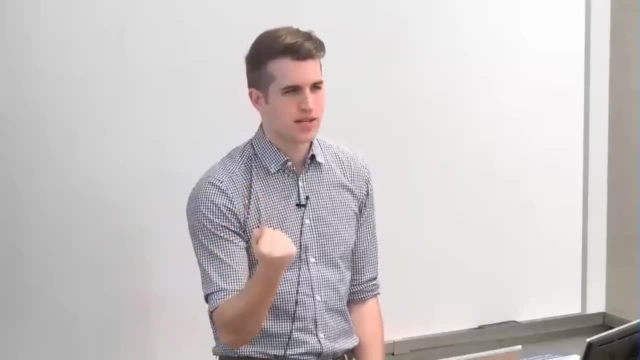 But our language, our informal language that we use, developed in a very classical world. It is simply not equipped to deal with the quantum world and this is why any pop science article you've read on quantum phenomena, it doesn't really ring true. 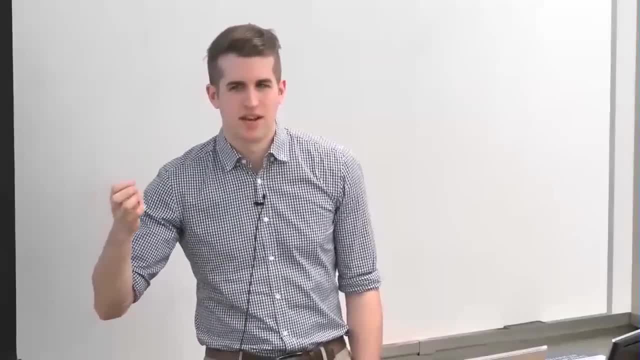 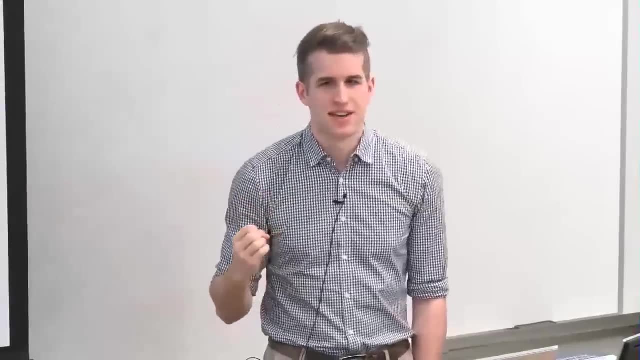 All the metaphors, they don't really make sense because we're trying to express it in this language which developed in a classical world. We need to learn a new language, which is the language of mathematics, And that is the only thing which will actually let us. 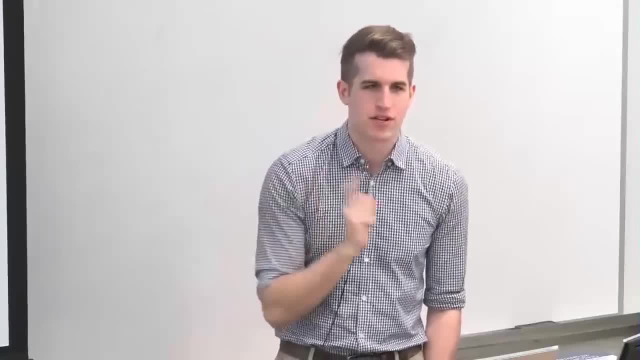 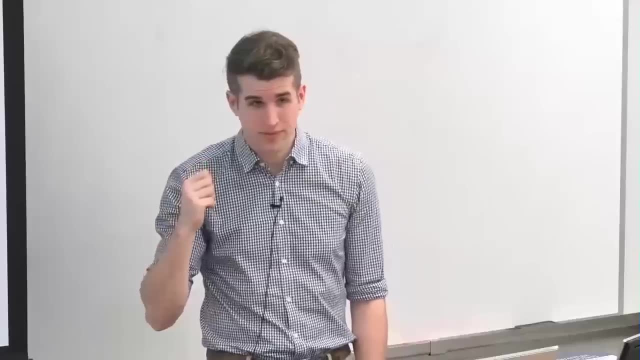 understand quantum mechanics is to learn it mathematically. All metaphors and analogies will lead you astray. There's a famous quote here by a physicist named David Merman, which is: shut up and calculate with regard to quantum mechanics. So some grad students. 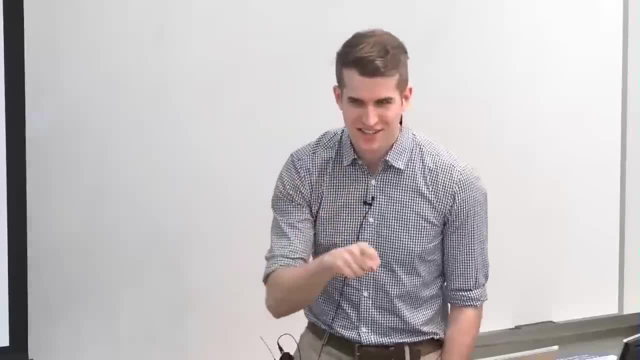 maybe they lean back in their chair and they're like: oh, what does this all mean? Shut up and calculate, Just trust the math. Math is the only thing which will not lead you astray. Okay, Here's how this presentation will break down. 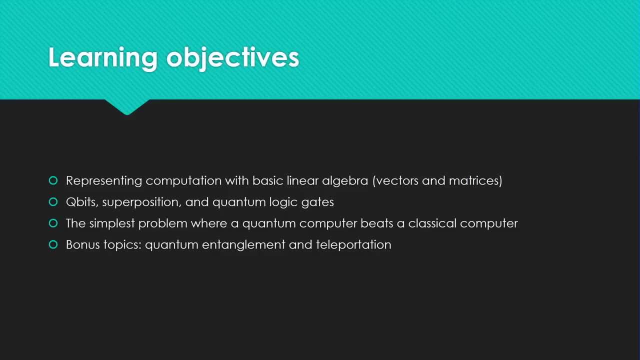 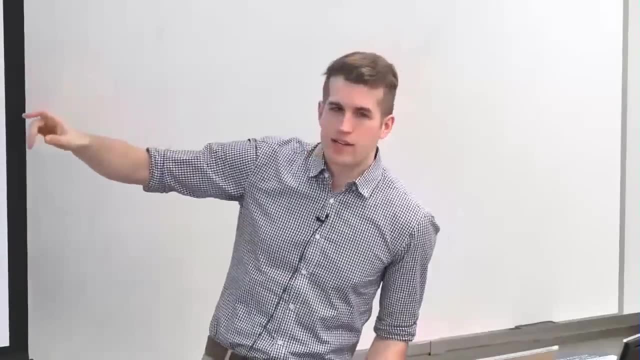 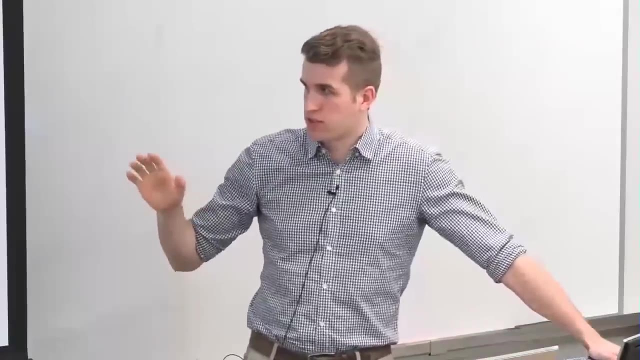 First we're going to learn how to represent computation using super basic linear algebra, matrices, vectors, matrix multiplication. Then we will generalize that to learn about qubits, superposition and quantum logic gates, And finally we will use all those tools we've developed to 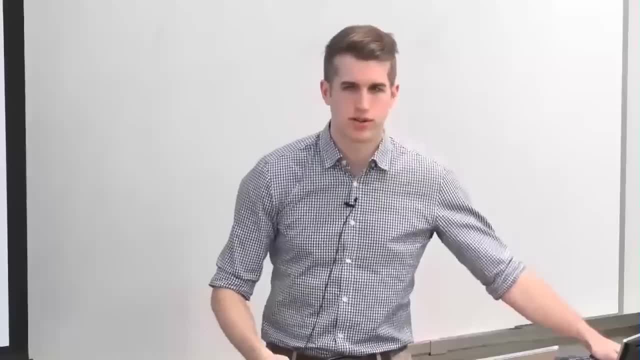 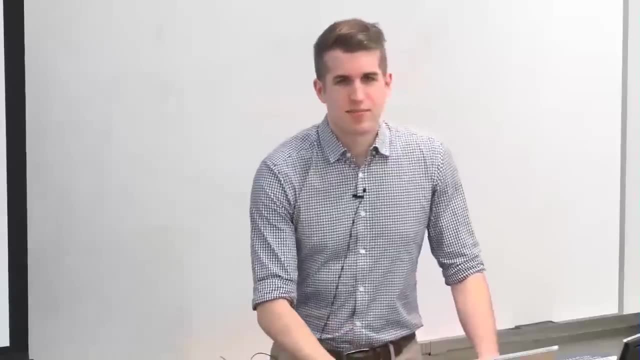 go over the simplest problem where a quantum computer outperforms a classical computer. This is called the Deutsch-Oracle problem. I mean, there are a bunch of problems but this is the simplest. And finally, it'd be almost negligent to let you get out of. 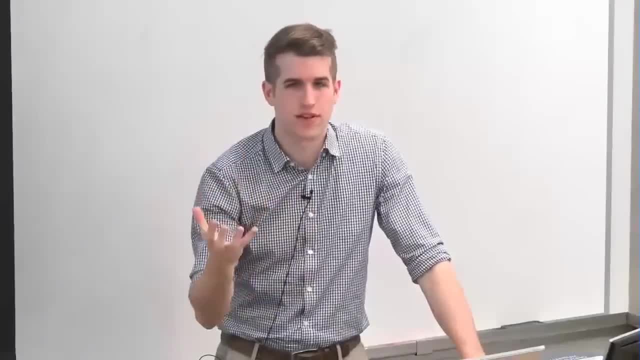 here without learning about quantum entanglement and teleportation, just because with the tools we'll develop, they're like so easy to understand. So we'll have bonus topics and then we'll have some demos. All right, Let's get to it. 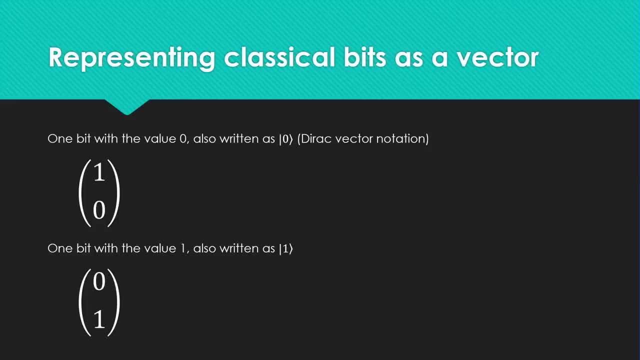 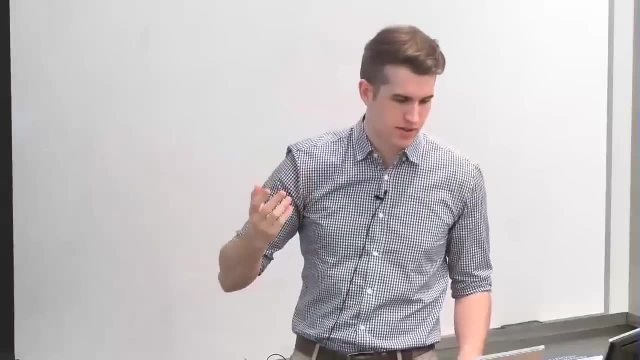 You'll become very, very familiar with these two vectors. This is how we represent a zero and a one, the two values of one bit in classical terms. So the top one is just one over zero and the bottom one is just zero over one. 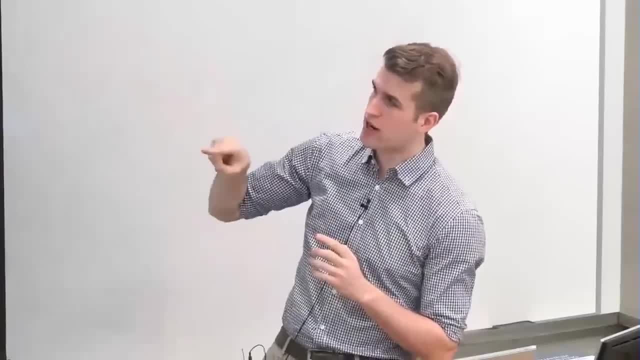 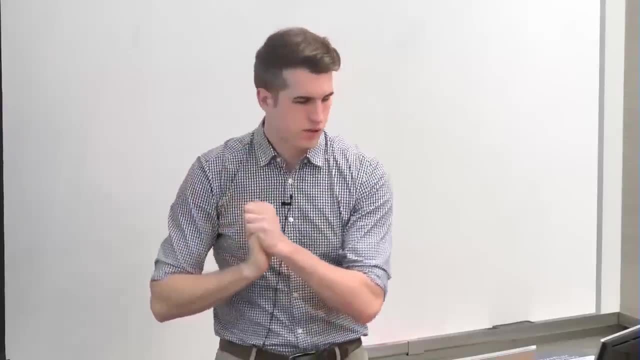 You can also write them in that weird like angle bracket thing that's called Dirac vector notation. So you have a zero in there. that means this is the value of that vector. If you have trouble remembering this, just think of it like an array indexed from zero. 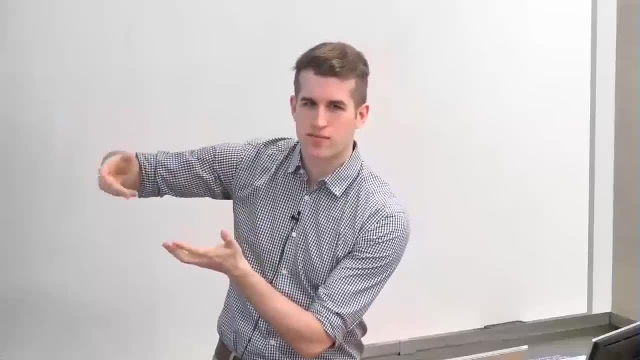 And so there's a one in the zero with index, that means it's a zero. There's a one in the first index, that means it's a one. Okay, Everyone's fine with this. You'll be very familiar with this by. 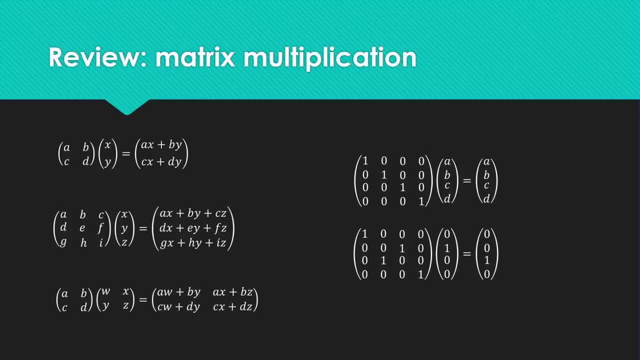 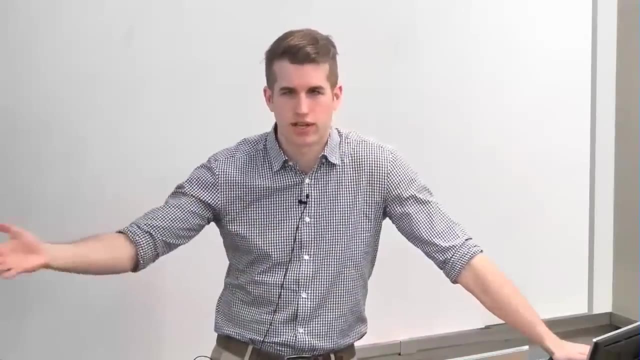 the end of the presentation We're going to go over matrix multiplication really quickly. So, yeah, okay, The way to think about matrix multiplication. just to review it for you. most of you will have gone over this in your linear algebra courses, like the first or second day. 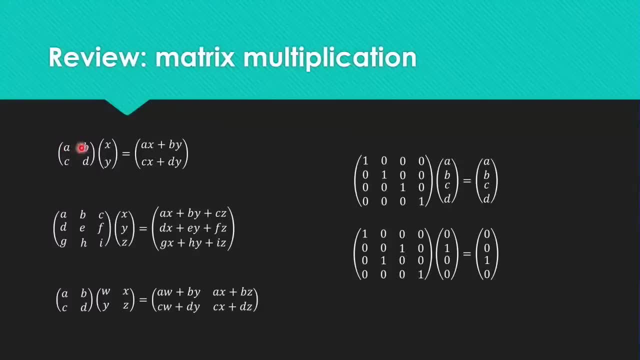 So if we have a matrix multiplied by a vector, you take this horizontal row and then flip it and multiply it point-wise with these vector values, So A times X, B times Y, and that's how you get the top one. 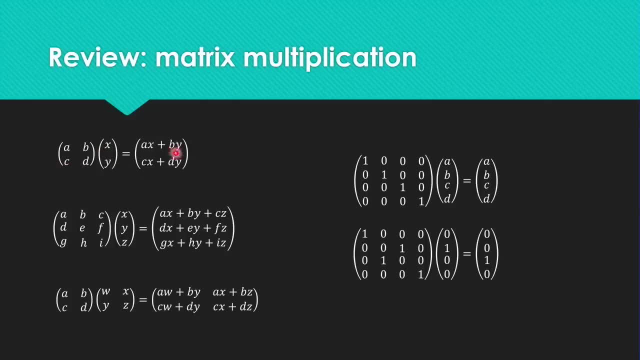 Then you do the same thing in the bottom row- C times X, D times Y- and you get a two vector. The same thing it happens with three by three matrix- A times X, B times Y, C times Z- and you get this vector. 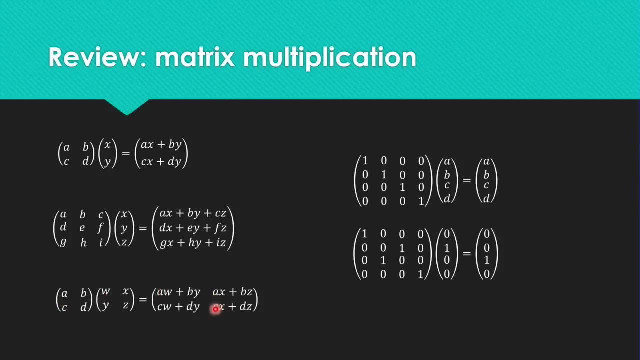 You can also multiply matrices together. We won't really be doing much of that. There's a very special matrix called the identity matrix, which has zeros everywhere except for ones along the main diagonal, and anything multiplied by the identity matrix is itself. It's just like multiplying by one. 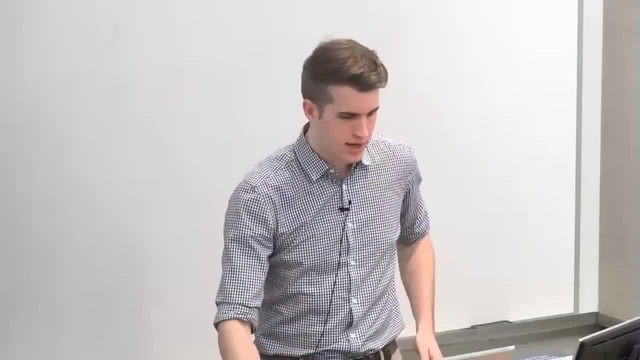 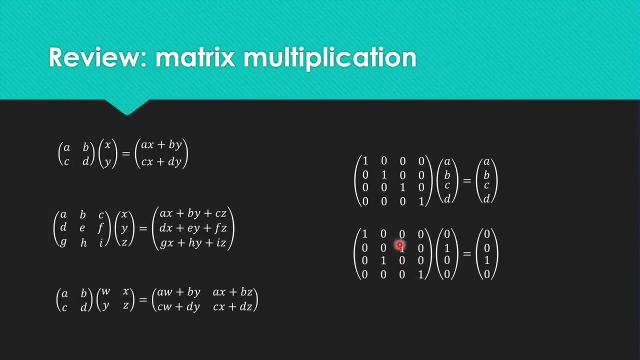 In fact, usually you refer to the identity matrix by the symbol one. Now, thankfully for simplicity, a lot of the matrices we'll be using look a lot like this. They're mostly zeros, with just some ones You can notice is a nice rule of thumb. 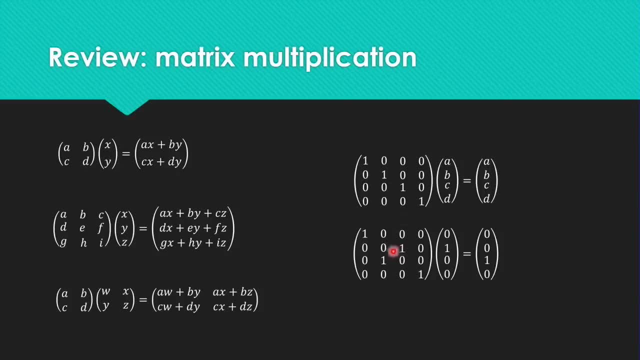 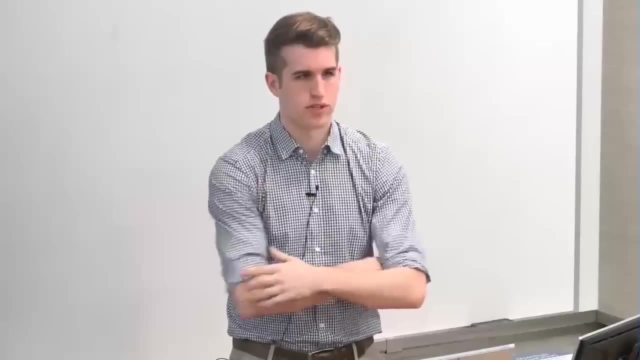 that relative to the identity matrix, this matrix has the middle two rows flipped. That's actually the action it has on anything it multiplies, So it flips the middle two rows. It's a nice rule of thumb to remember how matrix multiplication works. 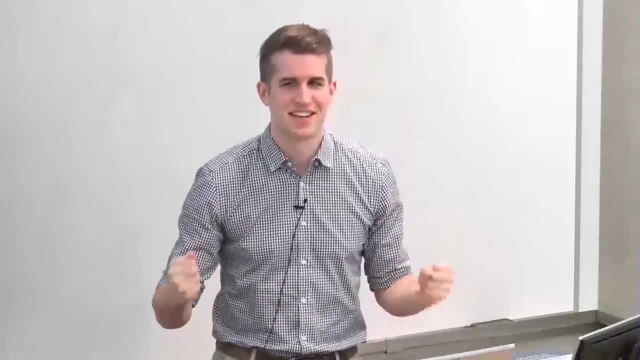 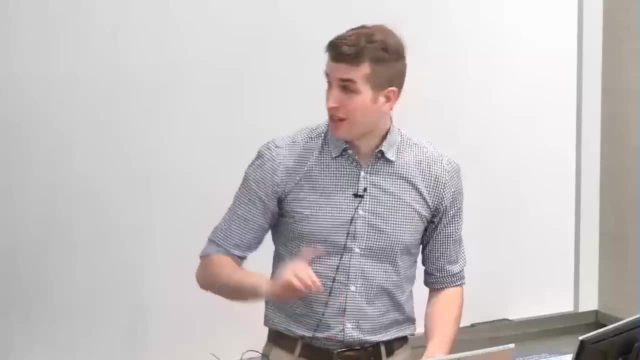 Does anyone have any trouble with this? Because you really need to know this in order to go ahead. You got to know it. Okay, Great Operations. actually, I'd like to make this a quiz. Can anyone tell me what are the four operations on one bit? 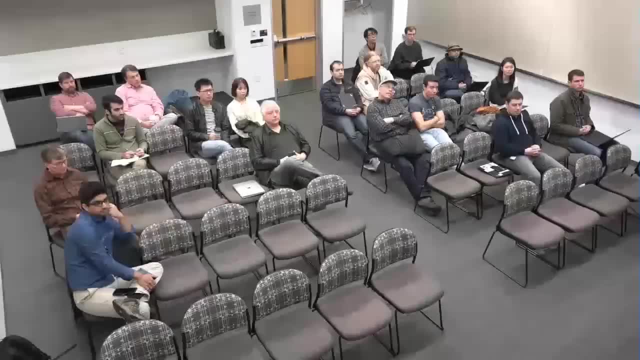 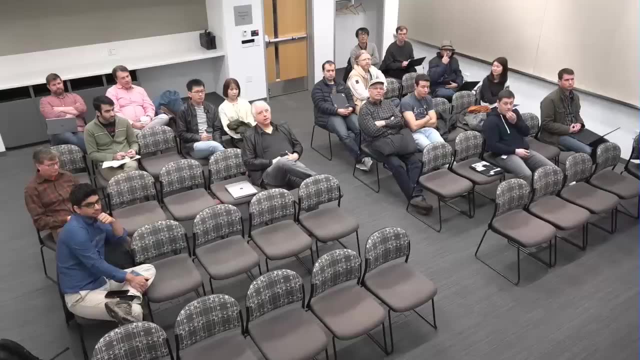 There's four of them: One bit, One bit, And or Those are on two bits. Oh, not Identity. Identity not Set to zero. set to one, Set to zero, set to one. There we go, Good, Yes. 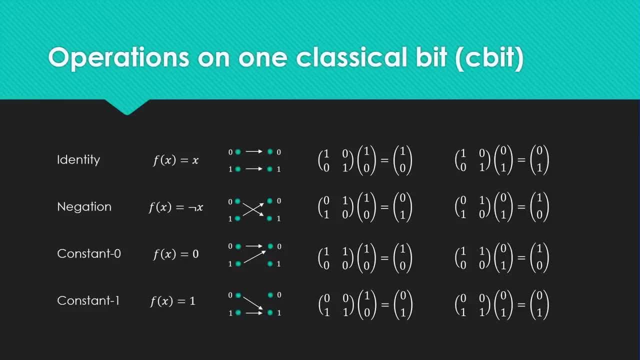 So we have identity. just f of x equals x. Negation f x equals, not x. Constant zero: it's always set to zero. Constant one: it's always set to one. You can see with the diagram how it kind of looks. 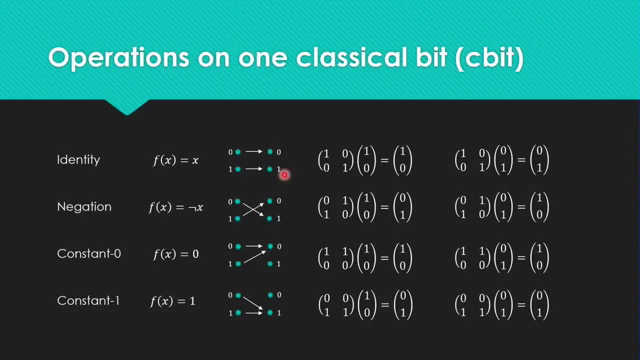 Okay, And we can write these as matrices. So the identity is just the identity matrix. This, remember, is our symbol for zero. Identity multiplied by zero is zero. Identity multiplied by one is one. Here's negation: You flip it from zero to one. 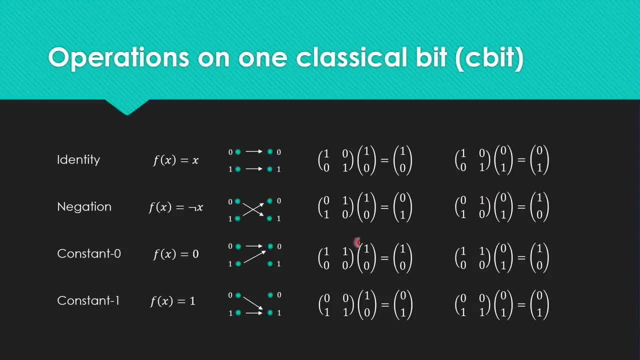 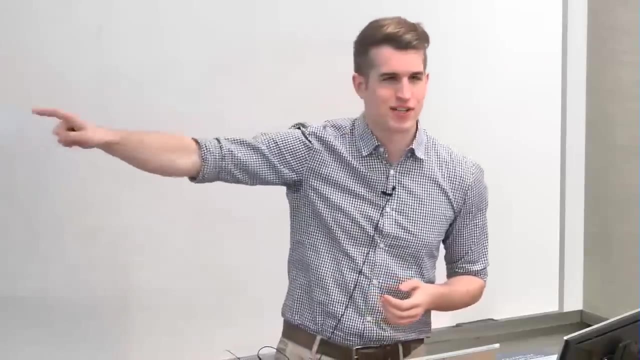 and one to zero. Same thing for constant zero, constant one. So I hope I've convinced you. we can represent very simple functions, at least with matrices multiplied by our zero and one vectors. Okay, And remember these four functions because I will quiz you later on them. 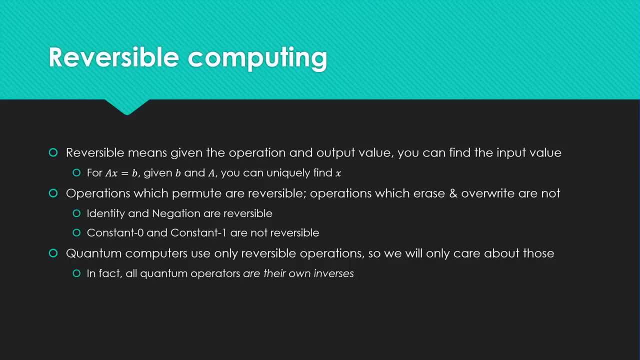 They'll come back up. So let's talk about reversible computing. Reversible computing is a neat sort of buzzword. If you've ever read the popular sci-fi book Accelerando, it talks about reversible computing And basically it means that if I tell you the operation I did, 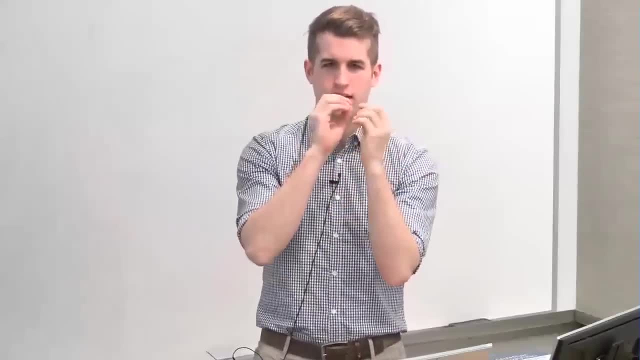 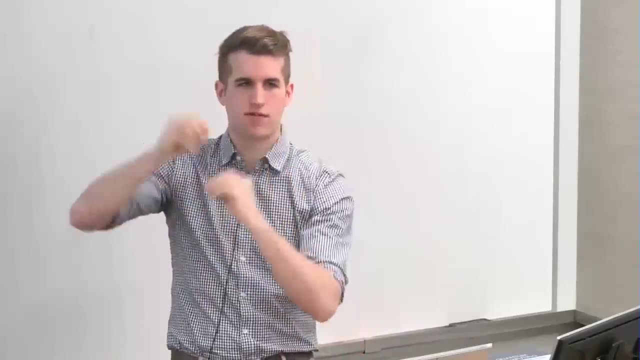 and the output of that operation. you can always tell the input of that operation if the operation is reversible So intuitively. operations that just shuffle bits around, like permute them, they are reversible. But operations that like erase bits and then overwrite them, are not reversible. 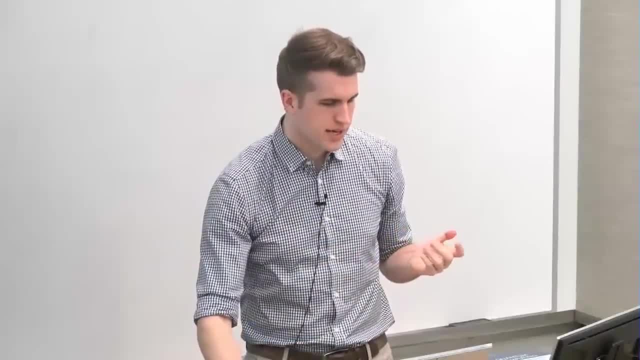 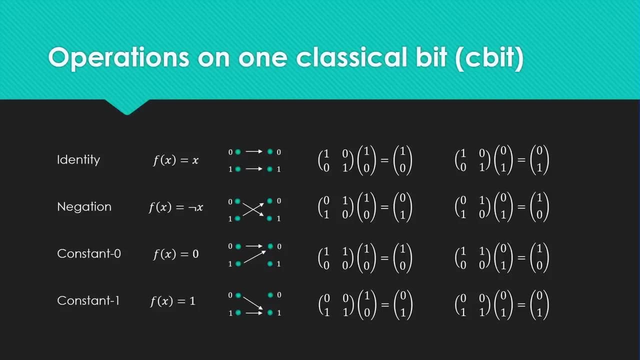 And in our previous slide, identity and negation are both reversible, Because if I say the output is one and I put it through the negation gate, that means the input was zero. You can always tell that. But if I say the output was one, 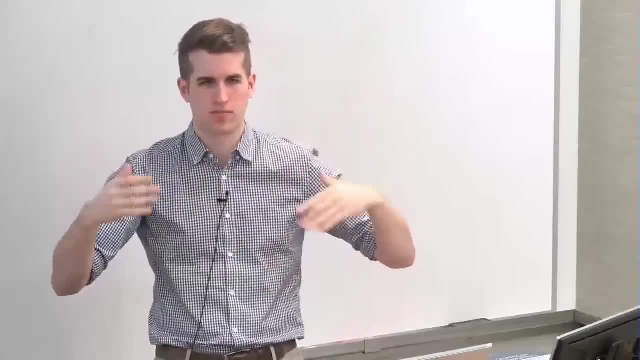 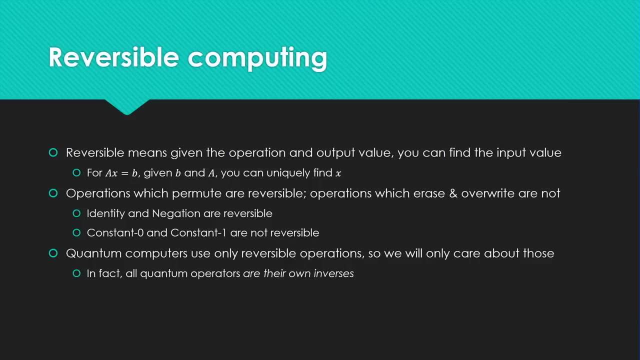 and I put it through the constant one operation, you can't tell what the input was. It's not reversible, It erases information. And the nice thing about quantum computing, which you can remember, is that quantum computers only use reversible operations. 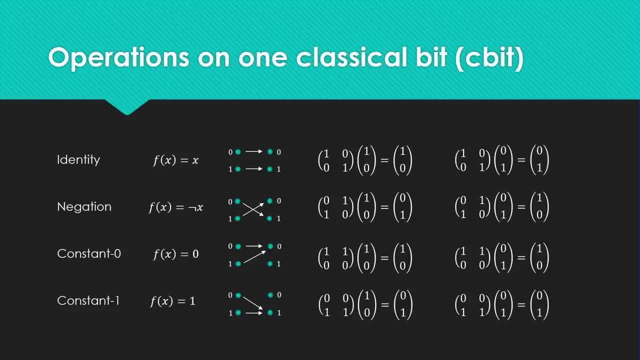 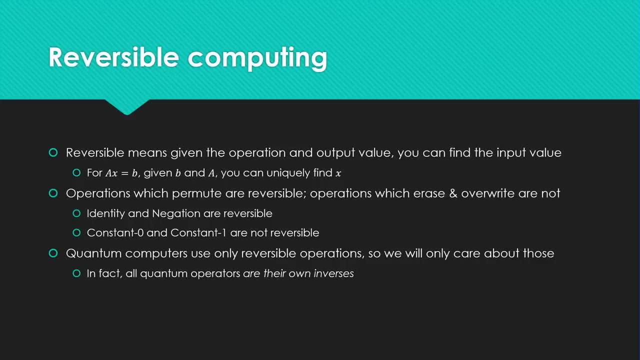 Those are the only ones we care about. So the only operation we actually care about on the slide is really negation, Like also identity, but it's the same as doing nothing. A further fun fact about quantum computers is they actually only use operations which are their own inverses. 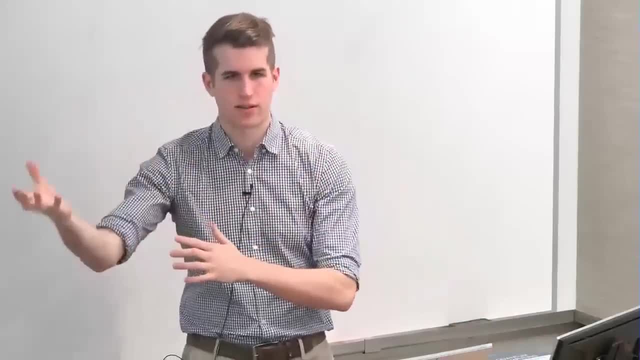 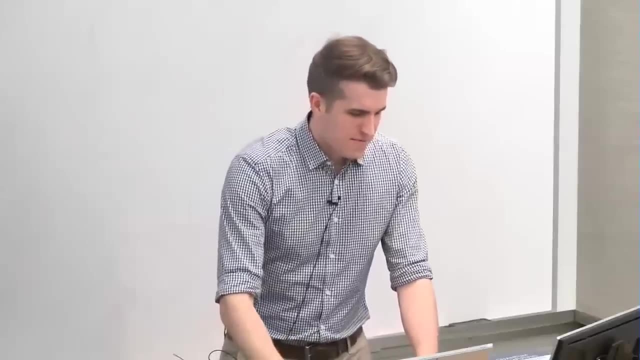 So not only are they reversible, but if you apply them twice you'll just get back the same input value, And we're going to go on a little. this is kind of like getting into pop science, but whatever. There's something called the von Neumann-Landauer limit. 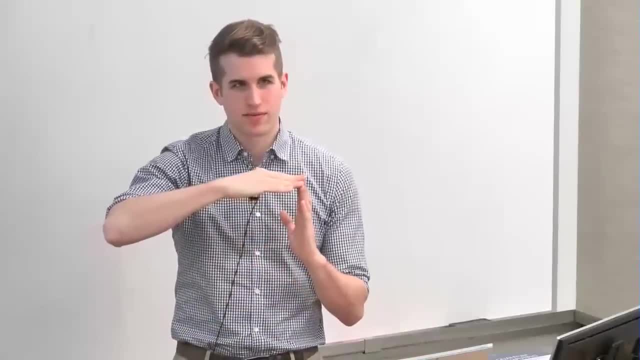 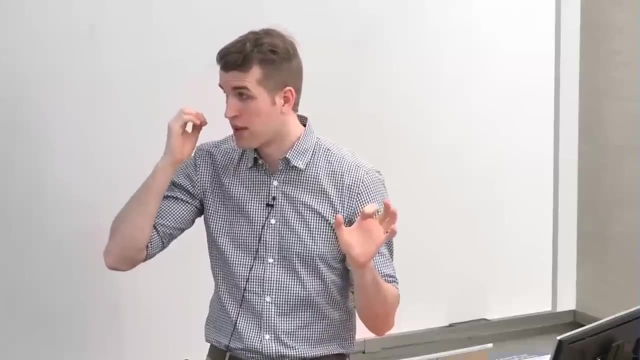 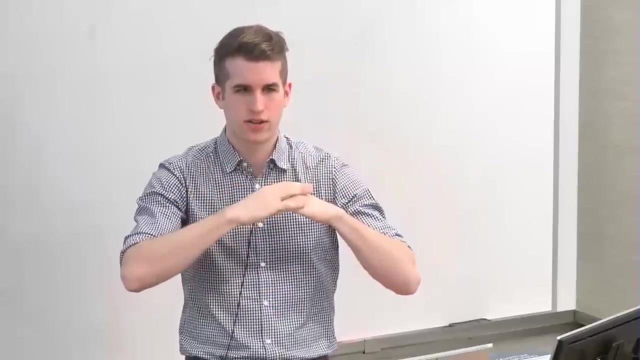 which is the smallest amount of energy physicists have calculated is necessary for the simplest possible calculation, which erases is non-reversible, And reversible computing might eventually let us go beyond that limit, more efficient than that theoretical limit. Now, currently, processors are millions of. 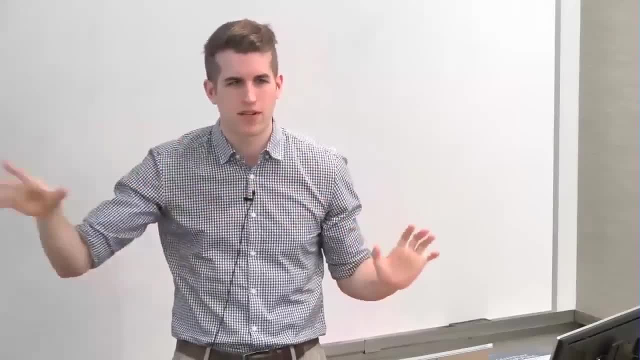 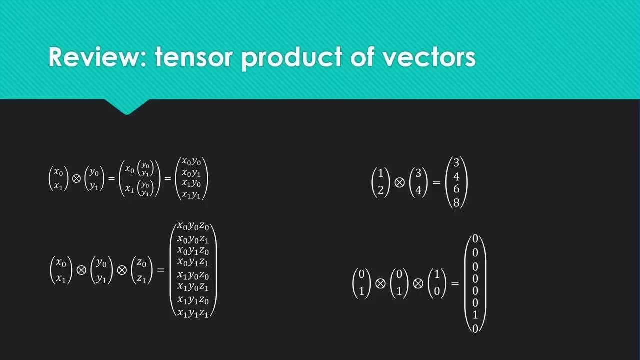 time, use millions of times more energy than the von Neumann-Landauer limit. But 50,, 100 years from now, who knows? pretty nifty, All right. This is something you probably did not go over in linear algebra. 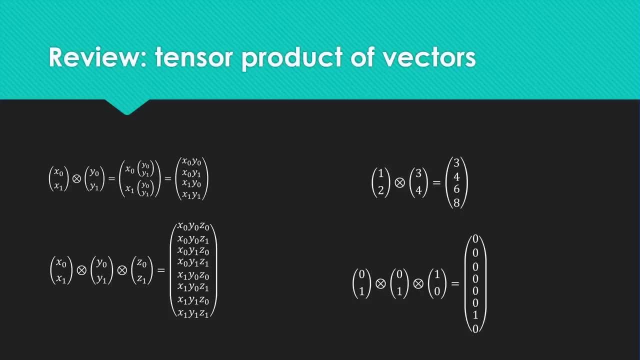 but don't worry, it's still pretty simple. It's called the tensor product. So if you have the tensor product of two vectors, it's kind of like you take the second vector and you tile it for each element in the first vector. 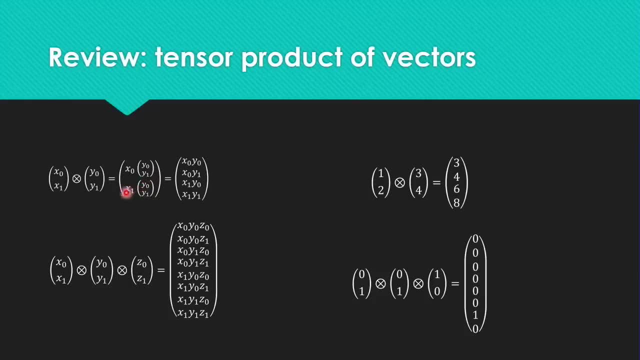 So X0 gets its own copy and X1 gets its own copy, and then you multiply it out so you get eventually X0, Y0, X0, Y1, etc. It might be easier to look at this with real numbers. 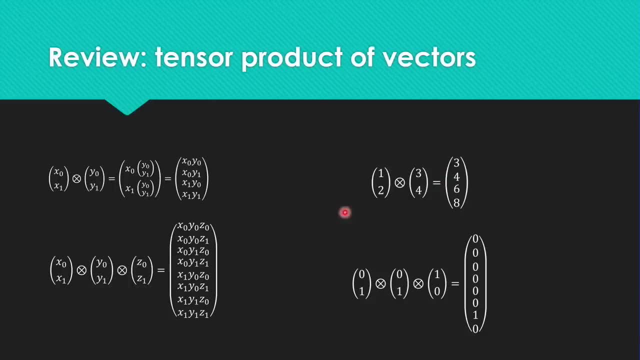 Here we have one times three, one times four, two times three and two times four to get this. Here's how it looks like. with three vectors You get this like giant array, don't worry about it too much. And I'd like to point out that if we use our zero and one values, 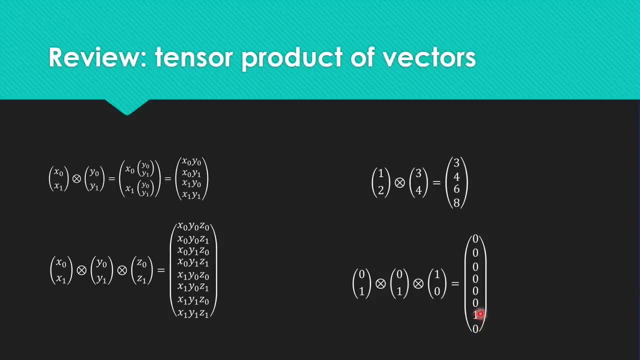 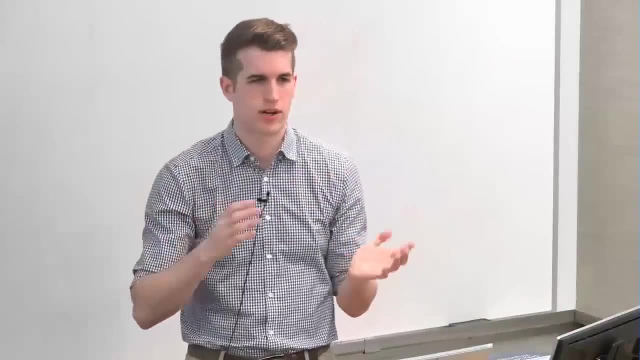 you end up with a vector which has a one and only a single position. Okay, Does anyone have any real trouble with this concept? If I gave you two vectors, you could probably calculate the tensor product. It's not entirely difficult. All right, But the final point I made leads: 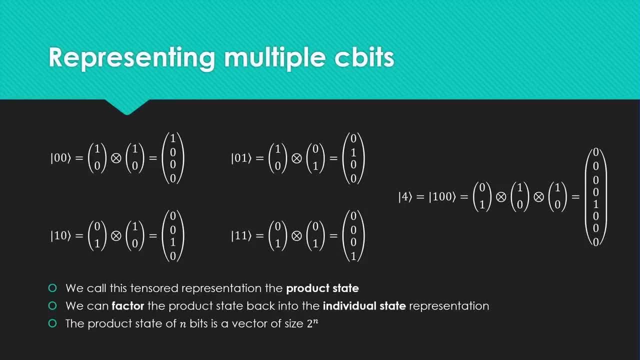 into how do we represent multiple classical bits? and we represent them by their tensor product. So zero, zero, remember we tensor, this is our zero symbol. Zero tensor with zero. is this product state? we call it Zero one is this product state. 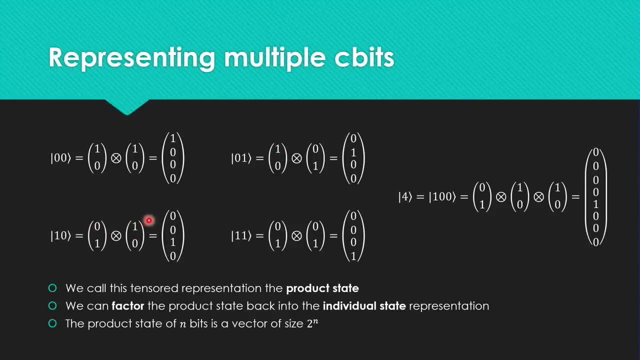 One zero is this product state like: zero times one zero. Zero times zero, zero. One times one one. One times zero, zero. Okay, And one one is this product state And similar to just the single bit. 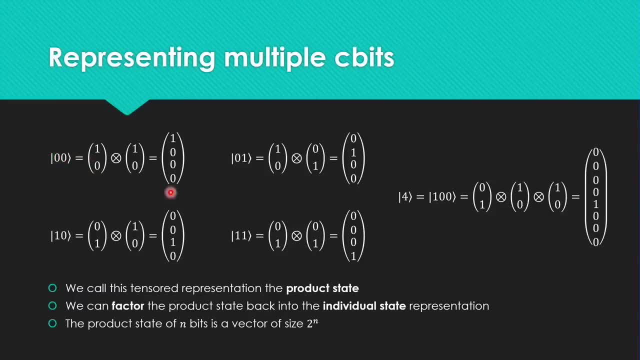 you can think of. this is an index in this vector array. So this is zero. There's a one at the zeroth position, This is one. there's a value at the first position counting from zero And this is two value at the second position. 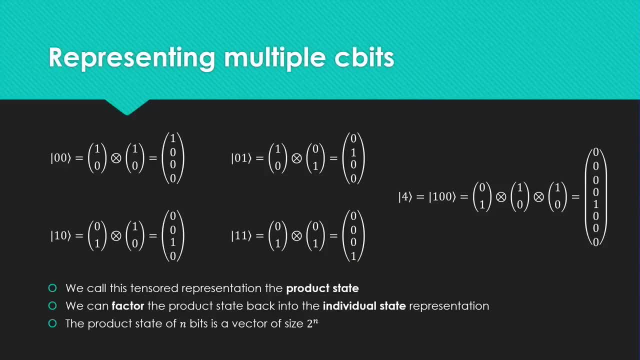 three value at the third position. Okay, This is the only time I will tensor three bits together, thankfully, because, as you notice, they grow exponentially in size, But it works for this. So four is one, zero, zero. You have zero. one, two, three. 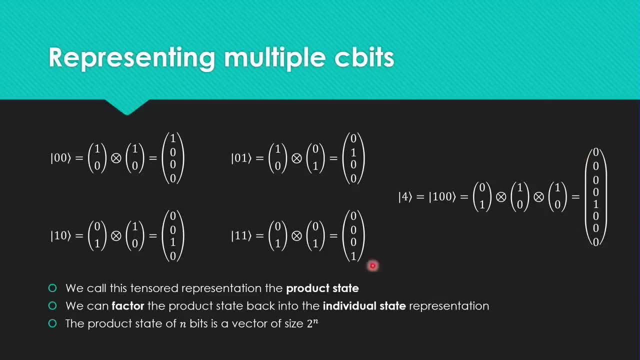 four is where the one bit is Okay, Yeah, So we call this the product state. We can always factor it out into its individual states, And the product state of n bits is a vector of size two to the n. Here we see a sort of whisper of 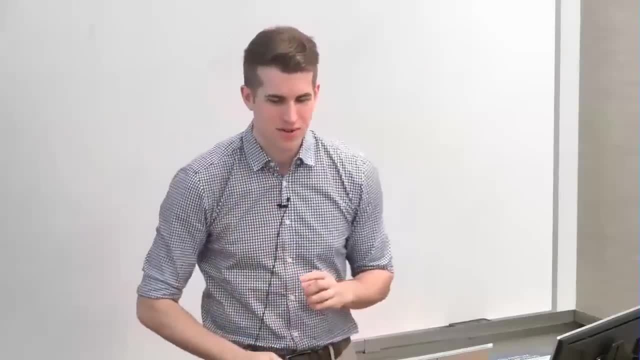 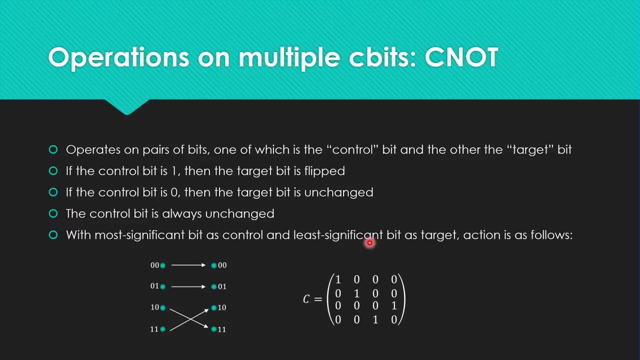 the power of quantum computing, this exponential term. But hold that thought, we'll get back to it. So we're going to learn a very important operation, very fundamental to reversible computing and quantum computing. It's called CNOT or conditional, not. 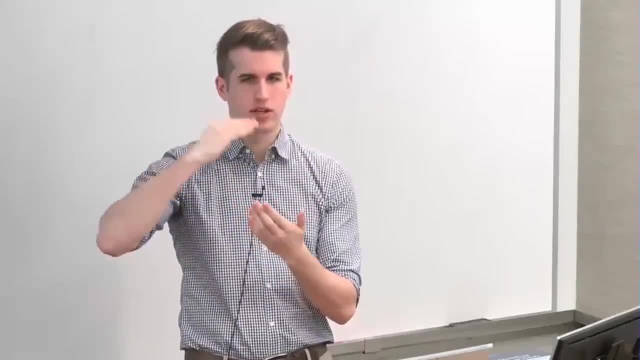 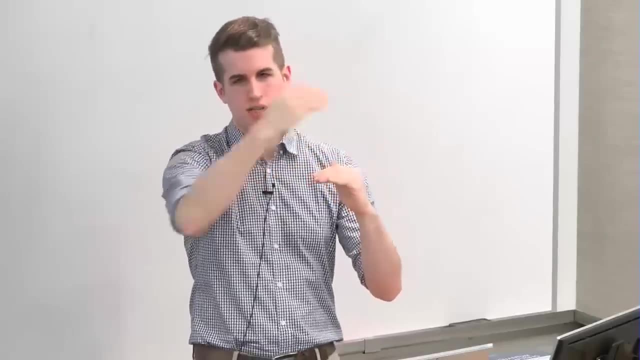 It operates on a pair of bits. You designate one bit, the control bit. The other bit is the target bit. So the control bit, if it's one, it flips the target bit. If it's zero, it leaves the target bit alone. 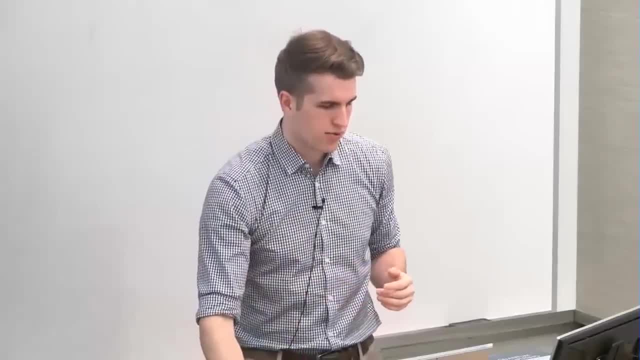 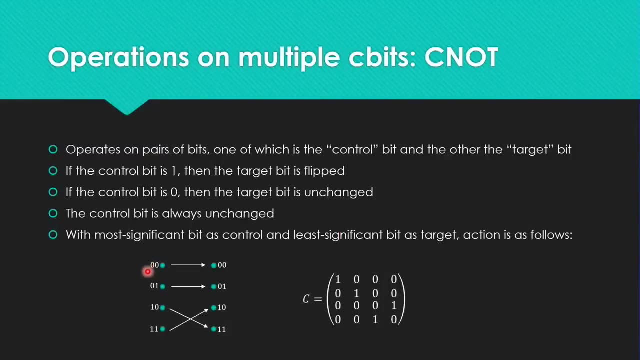 and the control bit is always left alone. So if we have the most significant bit of a two-bit system is control, the least significant bit is target, then zero, zero. since this is the most significant bit, it's the target bit, it just goes to zero, zero. 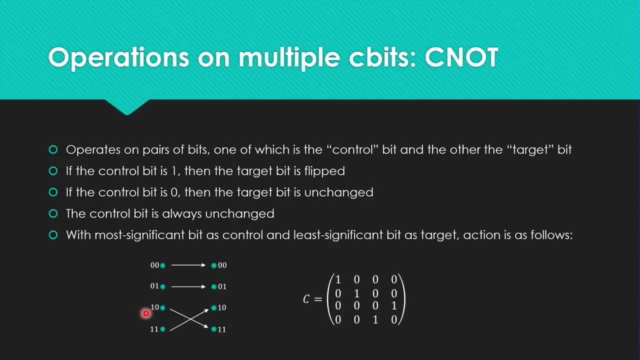 Zero. one goes to zero, one. Now one zero, since the control bit is one, maps to one. one right, Because it flips the other bit, And one one, since it again flips the target bit. it goes to one zero. 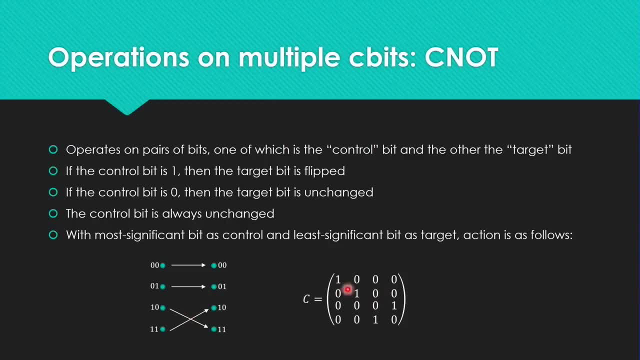 Okay, And this matrix, you can actually kind of write it. You see, there's like a sort of correspondence here. We flip the bottom two rows versus the identity matrix, And this I claim, which I will show in the next couple slides. 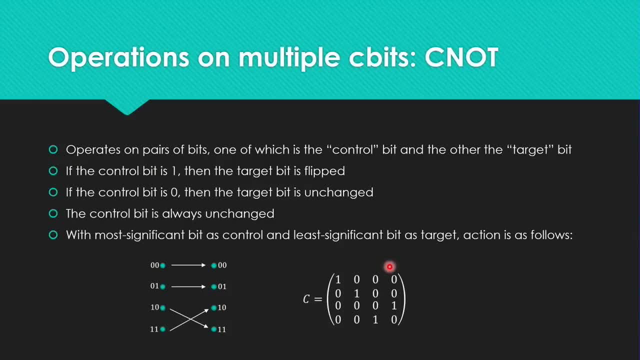 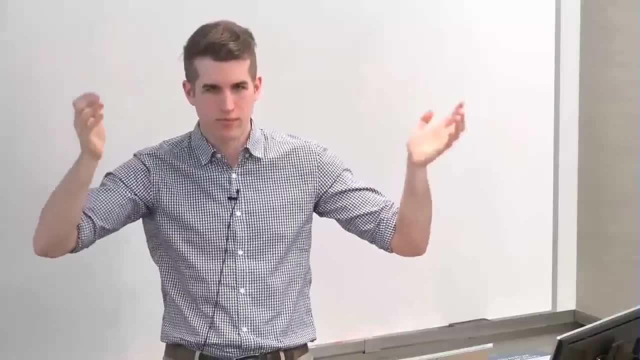 will change our product states according to the semantics of CNOT. So does everyone get the semantics here? We have a control bit and a target bit. Control bit's one, we flip the other bit. Pretty good. Okay, Now, this is a lot of math, but don't panic. 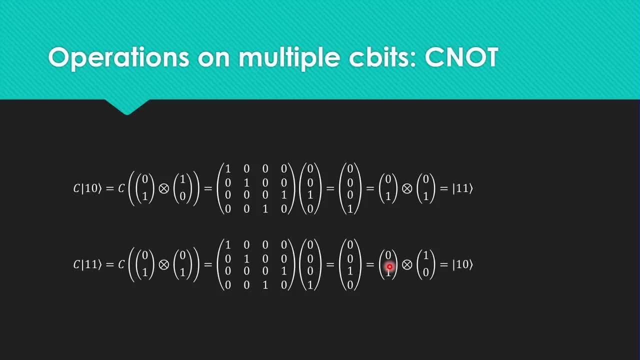 We're going to go over it step by step. If we apply the CNOT gate to one zero, remember that this is the control bit's one. so we're going to flip the other bit, So we expect it to go to one one. 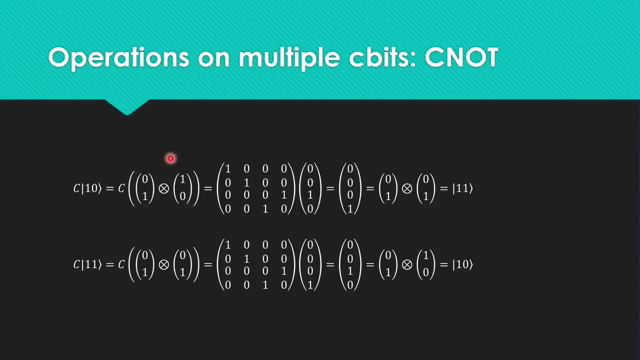 Now let's expand this out step by step. So one zero corresponds to this tensor product. This is the matrix from the previous slide and we're applying it to our product state. Remember, it's just going to flip the bottom two rows. 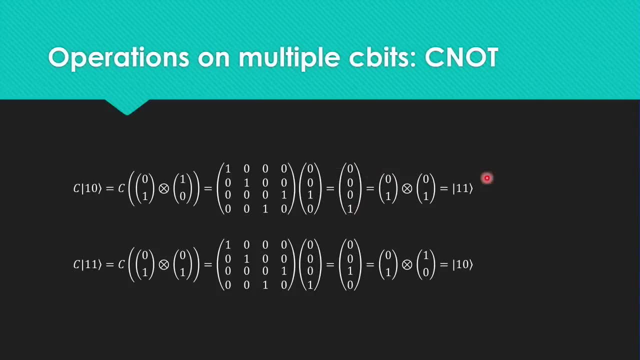 So we get to this product state which, when we factor it out, indeed gets us one one. Okay, Now let's do it with one one Same thing. We have our familiar matrix multiplied by this product state We go to here, which we factor into one zero. 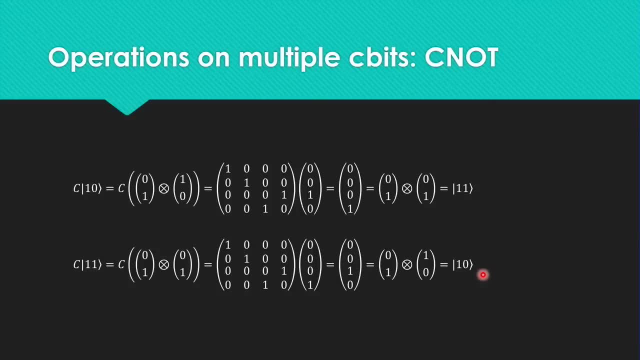 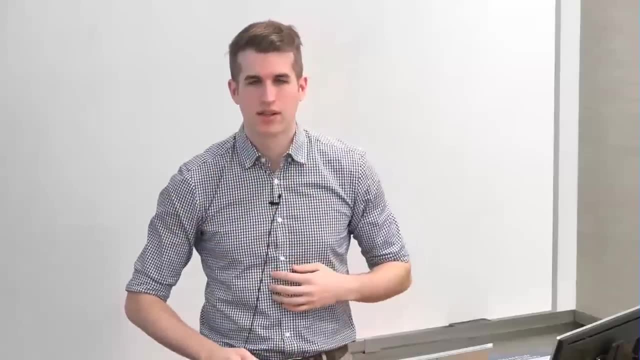 So I hope I've convinced you at this point that we can use matrices to represent kind of more interesting logical operations than just a bit flip. Does anyone have any trouble? Yes, So is that factoring always possible or practical for larger vectors? 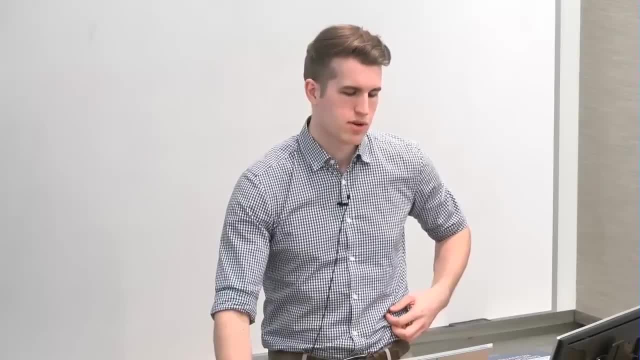 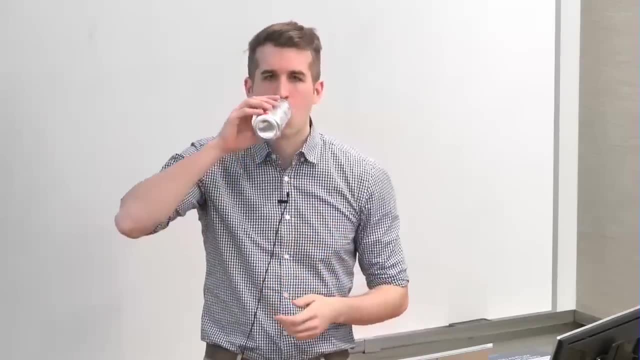 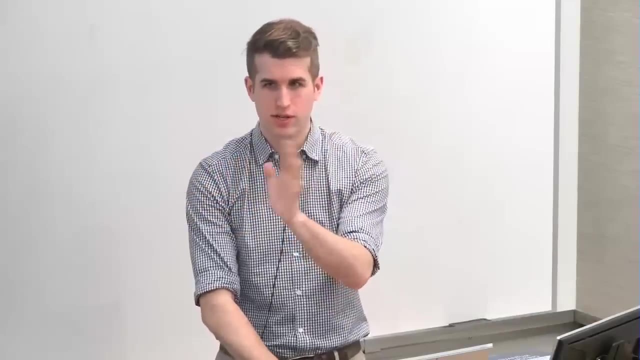 It is practical, yes, Not always possible. which kind of? we'll get into that when we get into quantum entanglement Basically. But good question, Okay, So this is fine for everyone. Nobody's lost in the gigantic equations here. 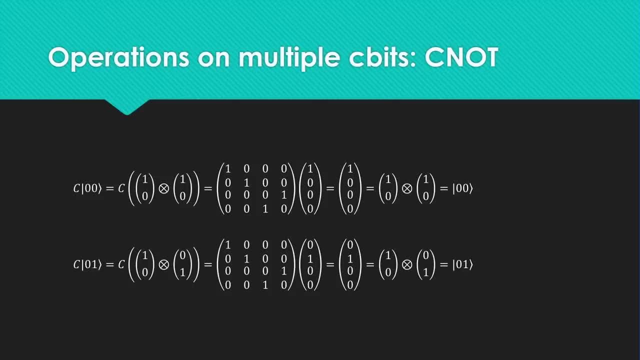 Okay, We're going to go over one zero then. Or sorry, zero, zero, zero. So the control bit is zero. That means we're going to leave the other bit alone. right, And we see that indeed. 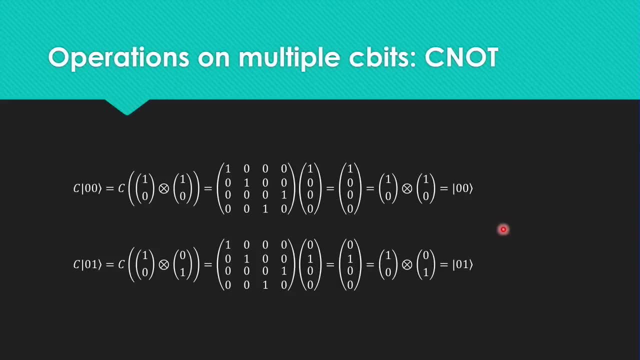 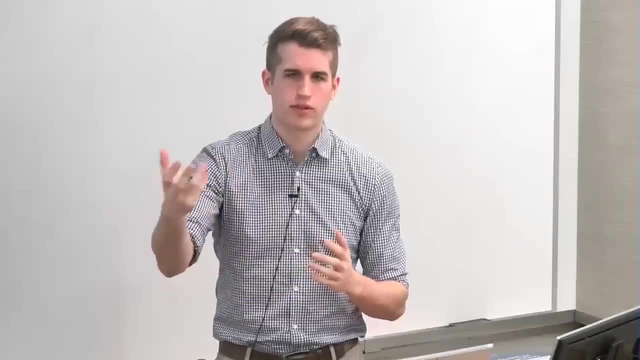 this is what we do, and same with four zero one. Okay, So everyone. well, maybe you're familiar with how classical computers, or like real CPUs, they're all built on the sort of NAND gate, Like everything is fundamentally built on NAND. 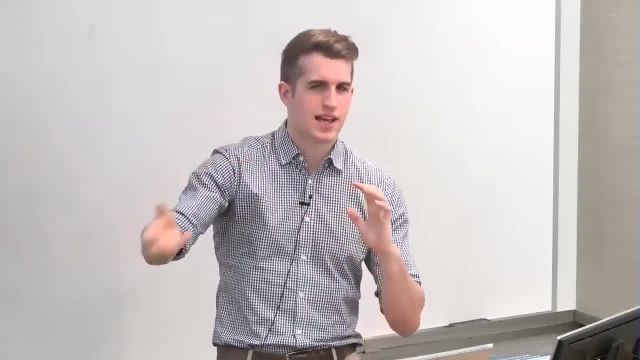 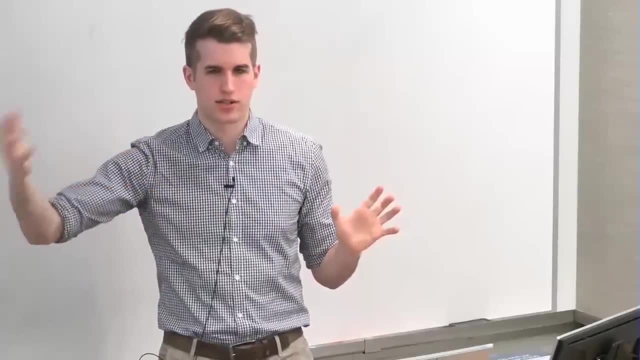 And CNOT is kind of the analogous NAND for reversible computing. It's like a really basic thing that is used to build up larger and more complicated logical statements. So I'm sure if I gave you a task like build some more complicated logical formula with CNOT, you'd probably be able to do it at this point. You just like stick them all together and eventually it comes out. I will note that it's not actually universal. You can't make every logical function with a CNOT gate. You need something called a Toffoli gate. 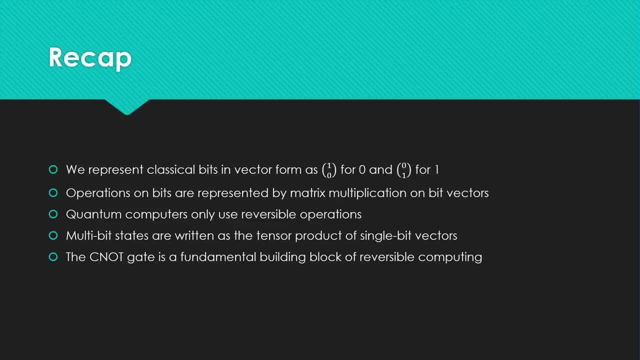 But we won't see that in this presentation. And we've learned everything we need to know about how to use linear algebra. excuse me to represent classical computation. And we can now go on to quantum computing. So to recap, we learned that we can represent. 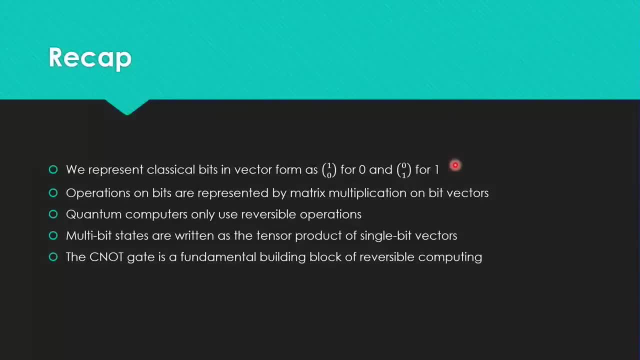 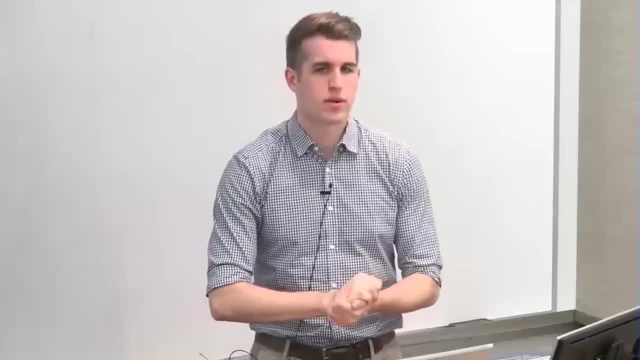 classical bits in vector form is one zero for zero and zero one for one. We can represent operations on bits by multiplications on their bit vectors. We learned that quantum computers only use reversible operations and in fact the operations are their own inverses. 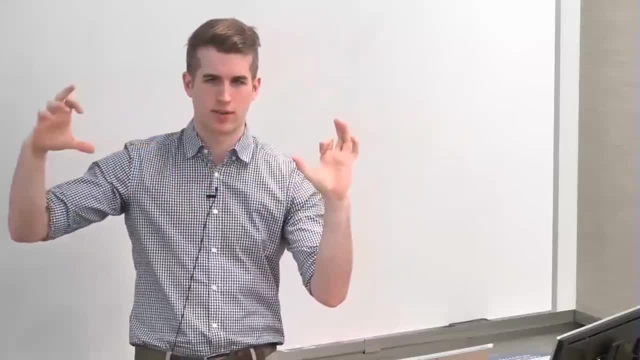 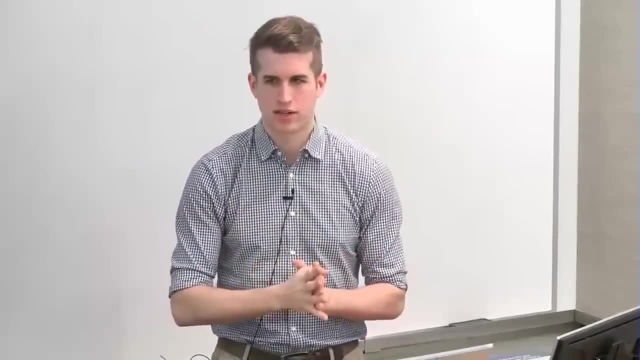 And multi-bit states, we write is the tensor product of our single-bit states. Finally, we learned about CNOT, which is a very fundamental gate in reversible computing and quantum computing. So is it anyone everyone's following along so far? This is pretty simple, right. 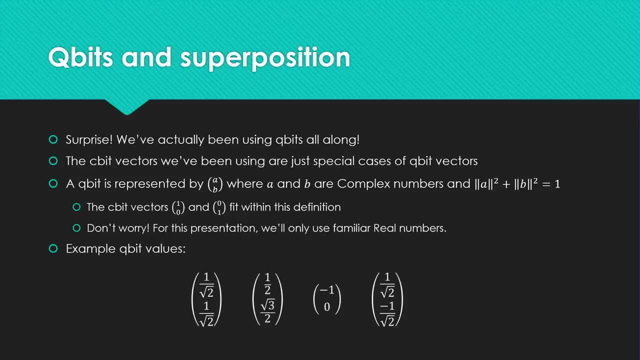 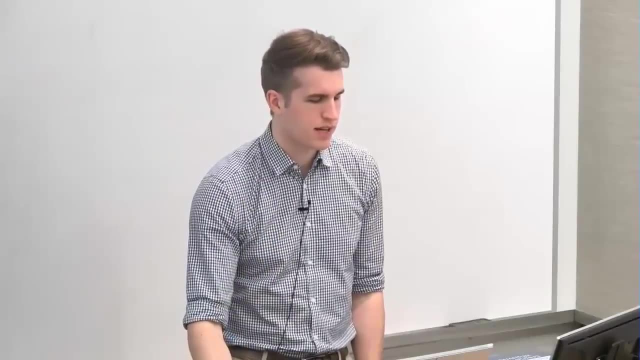 It's not that bad. Okay, Let's make the jump qubits, And I will surprise you. we have been using qubits all along. actually, The cbits are just special cases of qubits And we represent a qubit in general by a vector of two elements. 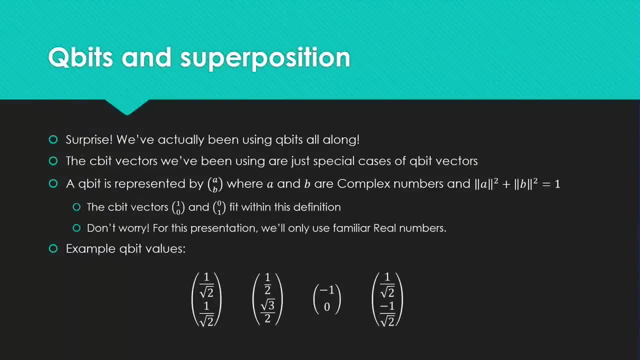 a- b, where a and b are complex numbers. Don't worry, we'll only use real numbers for this presentation. We're keeping it simple, only using real numbers, And we have the constraint that a squared plus b squared is one. 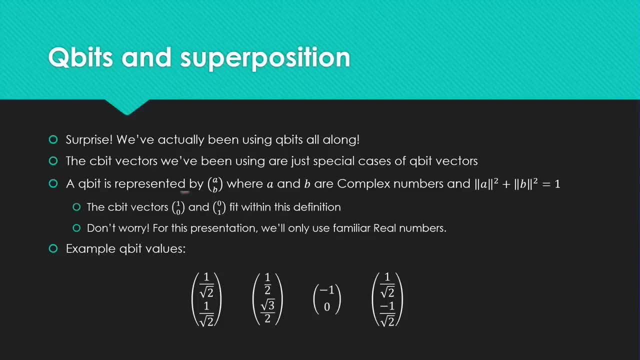 So one, zero and zero. and fifth is definition, because one squared plus zero squared is one and zero squared plus one squared is one. right Now, here are some example: qubit values. This is one with which you'll become very familiar. 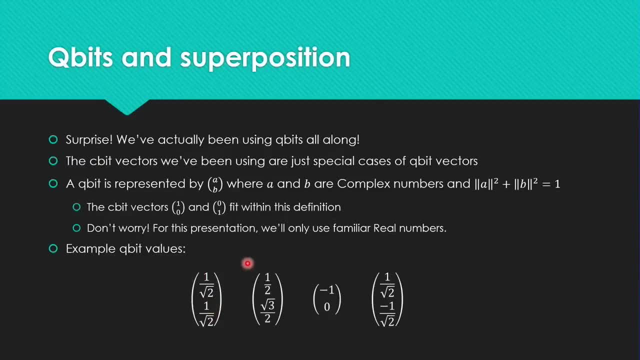 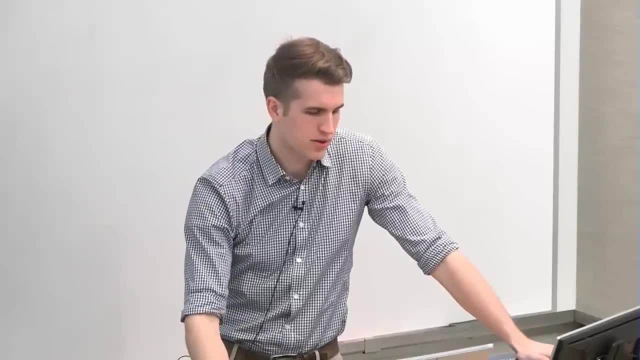 It is one over root two, one over root two. Can anyone tell me what one over two squared is? One half, One half, exactly. One half plus one half is one. So this is a qubit. What about one half and root? three over two? 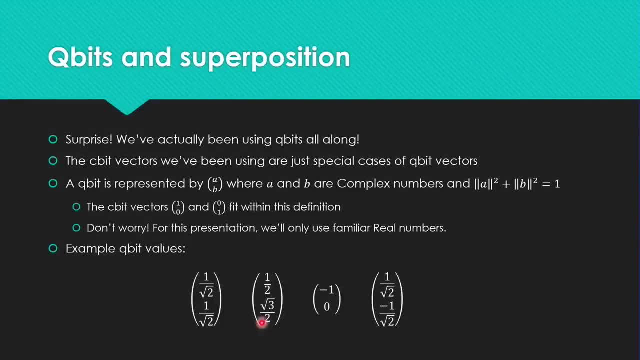 What's one half squared One quarter. So one quarter plus three quarters is one. Here's an interesting thing: we can actually use negative numbers now, Because a negative number squared is a positive number. So negative one squared is one. 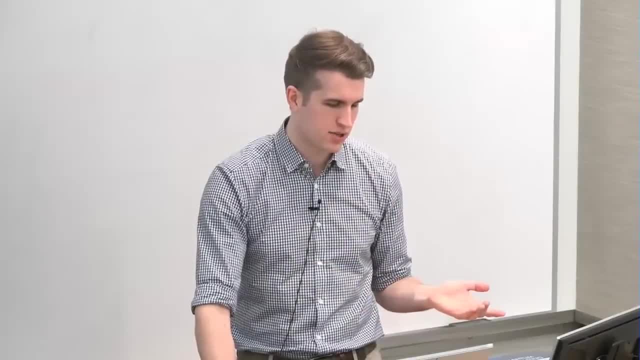 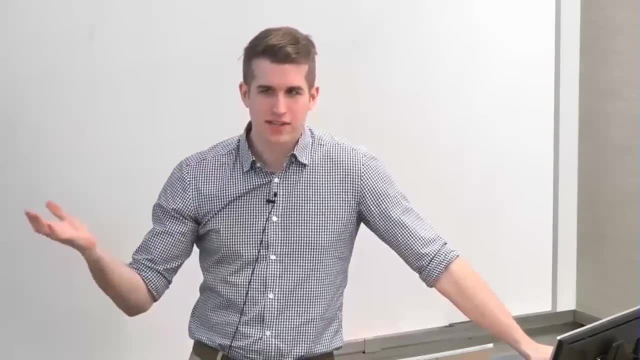 One plus zero is one And the same thing here. it's just the same as this first matrix, but one of the values is negative. Pretty neat, Not bad, so far, right, Okay. but you might say this is kind of like saying that a qubit has a value which is: 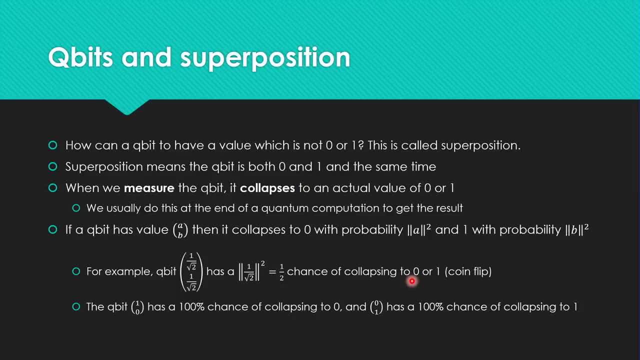 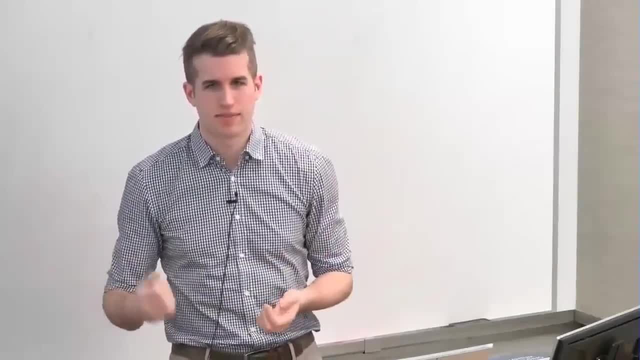 not zero one, but actually both zero and one at the same time. This is called superposition. Everyone's probably heard of the Schrodinger's cat being both alive and dead. that's just like a pop science way of articulating this concept, sort of. 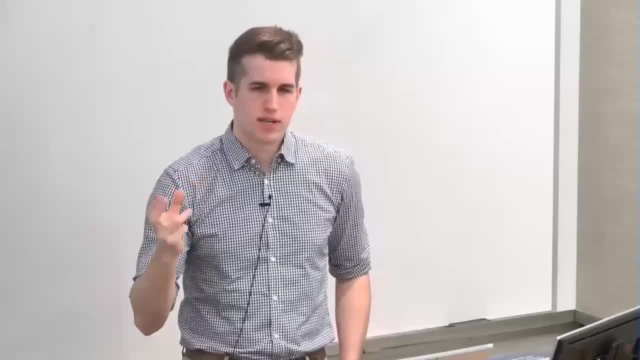 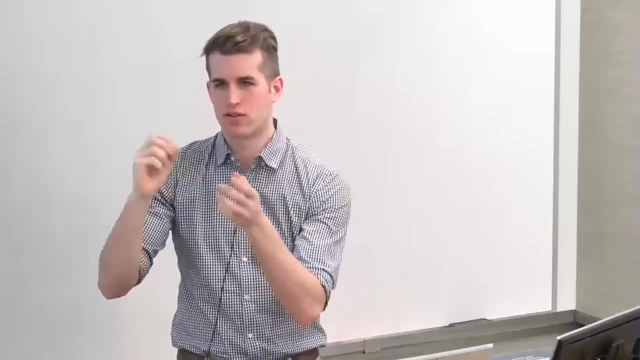 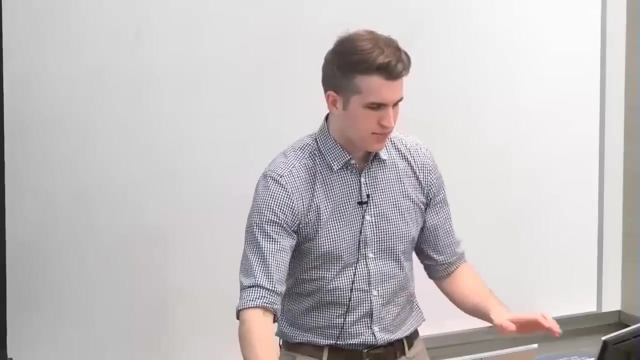 And the interesting thing about a qubit being in superposition: it means we can kind of- I want to really qualify this kind of compute with the values of both zero and one at the same time, Which again is the sort of whisper of some quantum speed up power. okay. 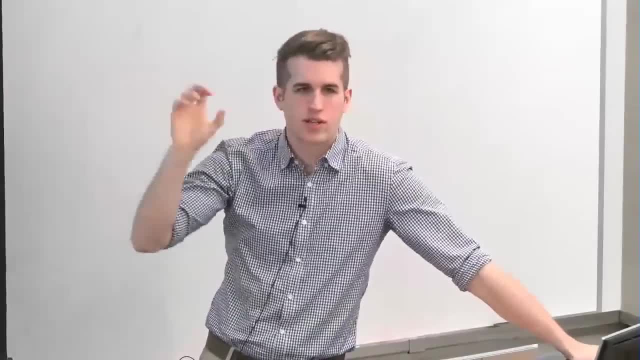 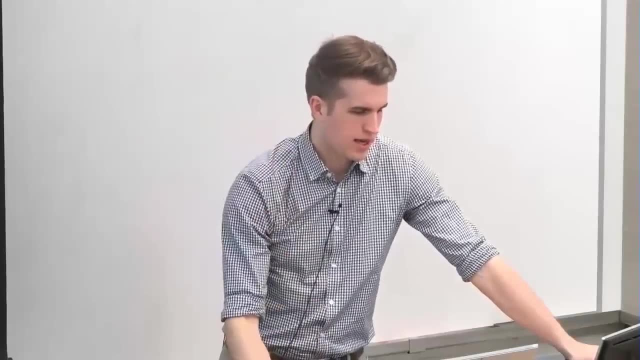 Now how this works is: when we measure this qubit, it collapses to our familiar values of zero and one. with some probability- And this is what we usually do at the end of a quantum computation- to get the final result, We send it through the measurement gate. 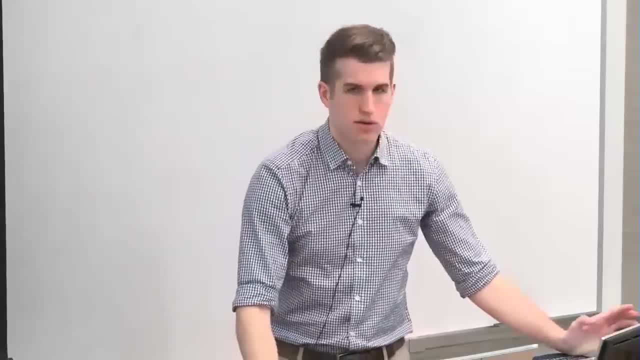 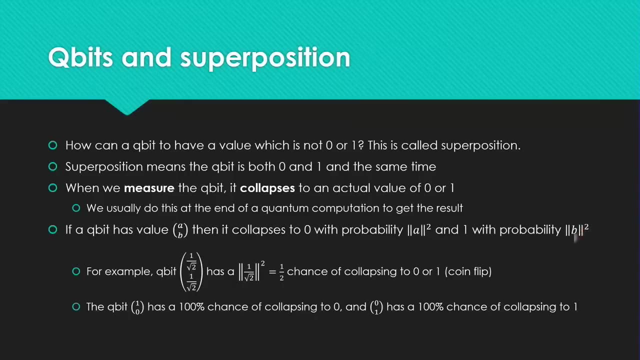 we see what the result is. So how the probability works is: if you have a value a- b, it collapses to zero with probability a squared and one with probability b squared. So if we look at our familiar qubit from previous slide, 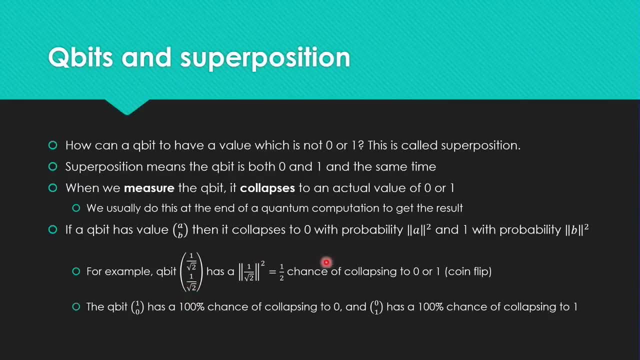 one over two. one over two, it has a one-half chance of collapsing to zero and a one-half chance of collapsing to one. It's like a coin flip Now if we just measure our classical qubit or classical c-bits. 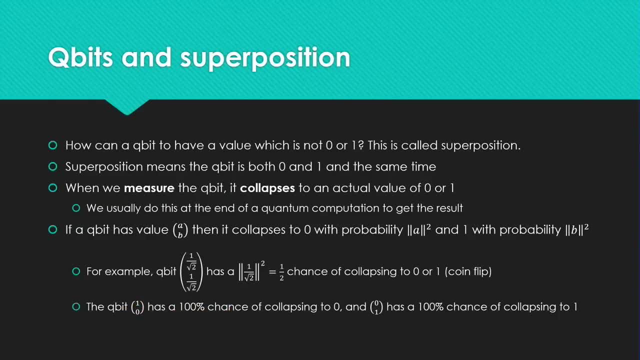 the one, zero- has a 100 percent chance of collapsing to zero and zero one has a 100 percent chance of collapsing to one. So it's sort of item point in that way, And I found it useful here to give people a sort of physical intuition about what we're doing. 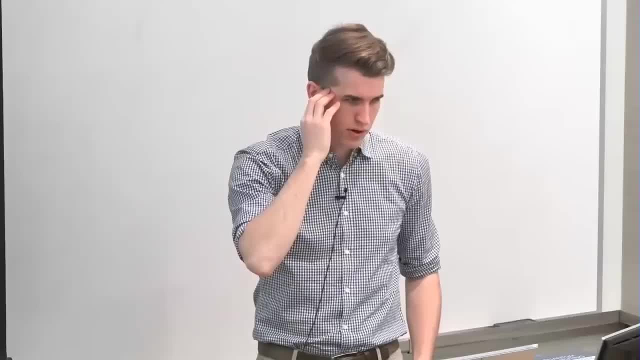 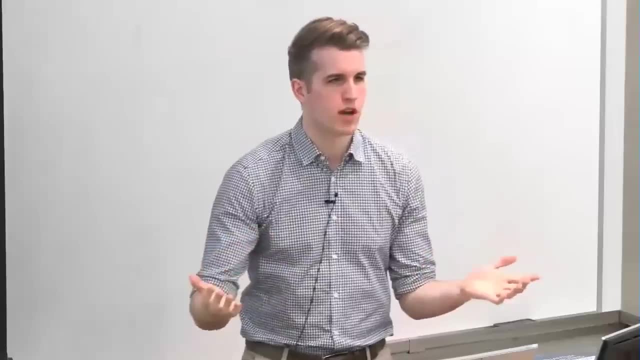 what a c-bit is or a qubit is. If you've heard of polarization, you've probably bought like fancy sunglasses. it says that they're polarized. So polarization is actually sort of a quantum phenomenon. You can be polarized like this way or this way. 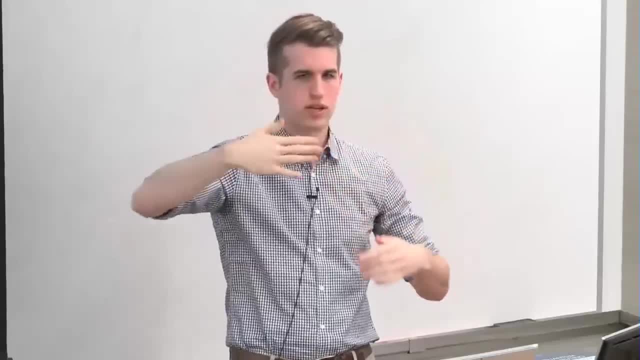 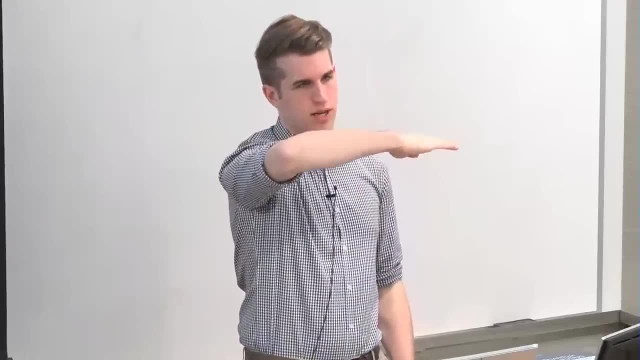 and your glasses will only be polarized a certain way, so it'll only let light polarized in this way through. basically, It turns out that qubits you can think of like this: yeah, photon being polarized this way is a zero. 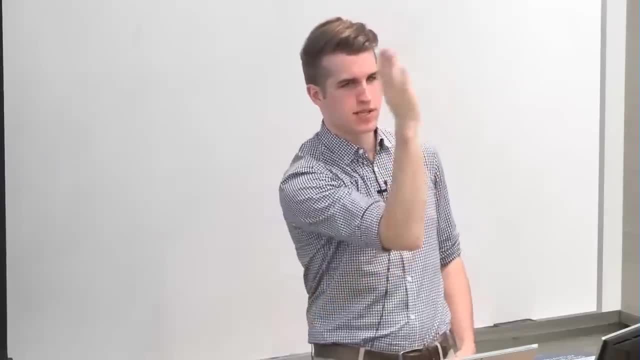 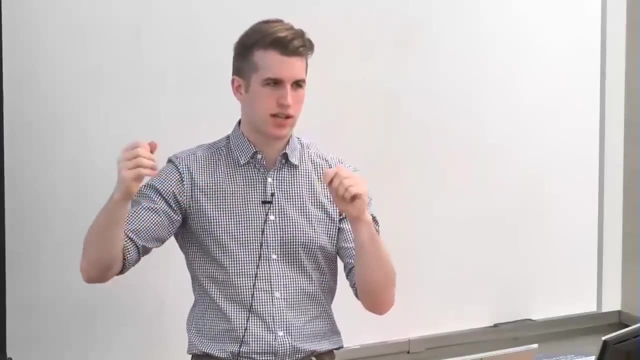 and photon being polarized this way is a one Superposition means it's actually like both right, So it could actually go through both gradients. And then if you measure it- and a way to measure it is just to like, fire it through a grading. 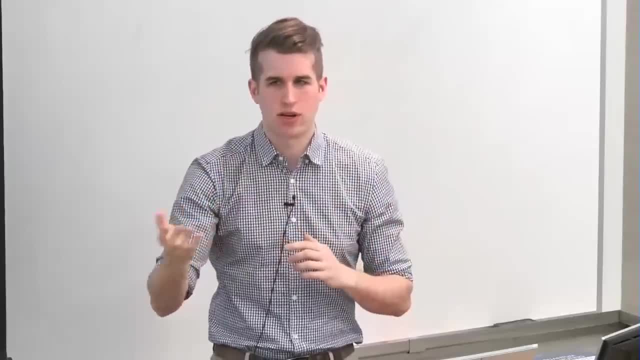 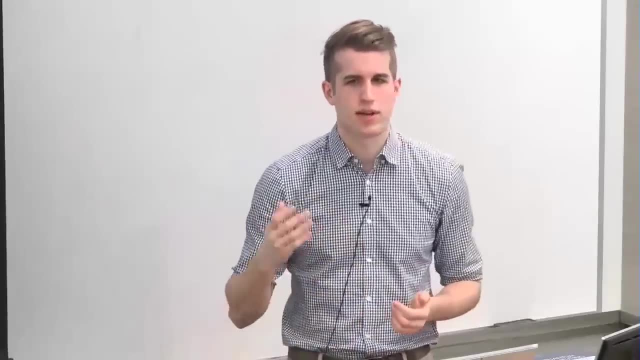 and like: see whether it goes through, then you can collapse it to zero or one. So that's our sort of intuition, pinning this to a physical concept, Of course modern. we found that photons actually make very poor qubits. they tend to collapse too easily. 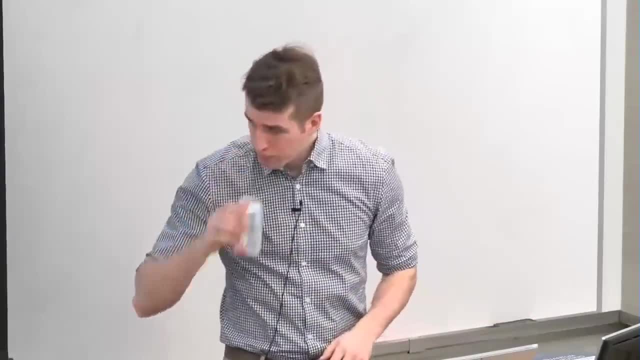 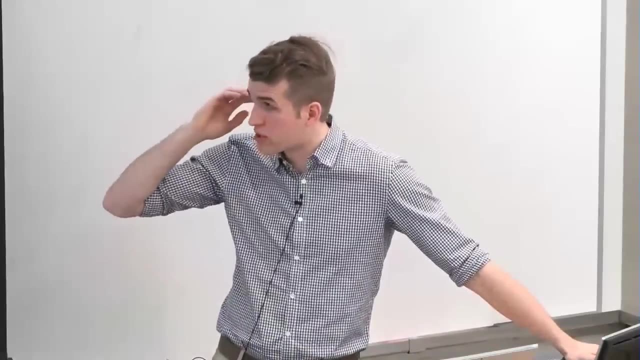 So we don't use those, but you can maybe think of that. Does anyone have any confusion here, really, About how this measurement process collapse probability works? Okay, great, We will learn about multiple qubits. The same is multiple C bits. 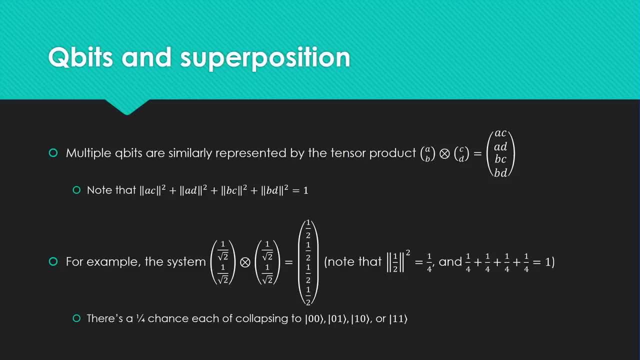 we represent them by the tensor product. It actually. why is it doing that? Okay, Hold on Laser pointer. Okay, there we go. Nope, that's not Okay. So if we have two qubits and we multiply them, 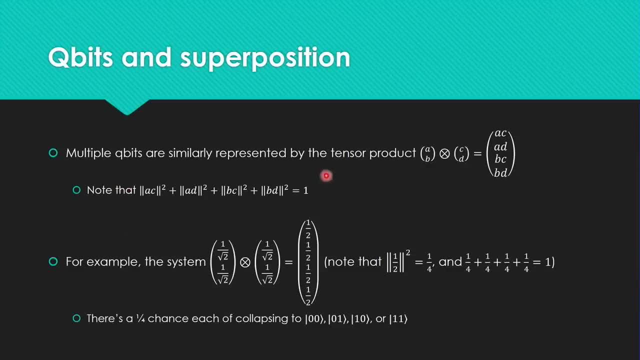 the sum of squares, identity actually is maintained. So if we consider our perfectly balanced 50 percent coin flip qubit and we tensor with another coin flip qubit, we get this four vector with one half in every single column and one half squared is of course one quarter. 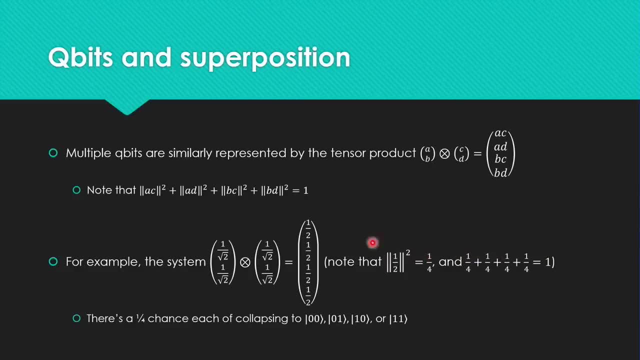 So one quarter plus one quarter plus one quarter plus one quarter is one. this maintains the property. The way to read this is: when you measure these two qubits, it has a one quarter chance of collapsing to zero, zero, zero, one. one, zero, one one. 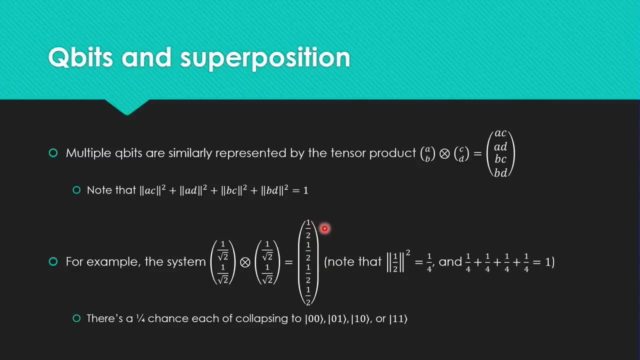 This is sort of the probability and when you measure it, finding a one there and zero everywhere else. So we could find that it's a one quarter probability finding a one in this position and all zeros everywhere else. Does that kind of make sense for multiple qubits? 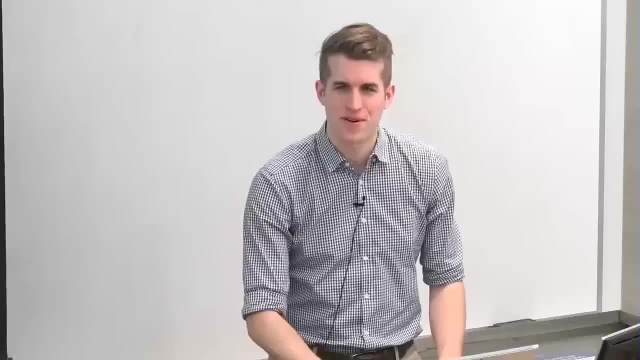 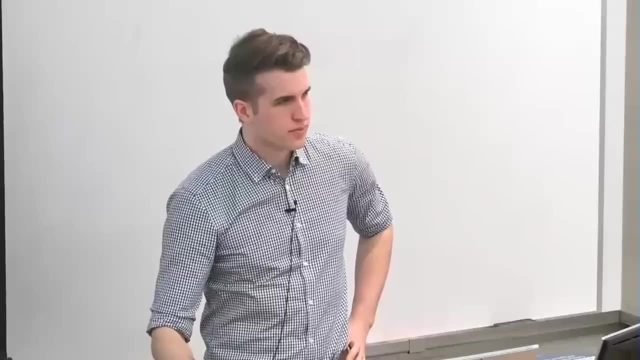 Okay, Great, You guys are just trucking along, no problem, It's to be super easy. Yes, I have a question, Absolutely So there's only going to be one, one left in the vector. Yes, There couldn't be two ones. 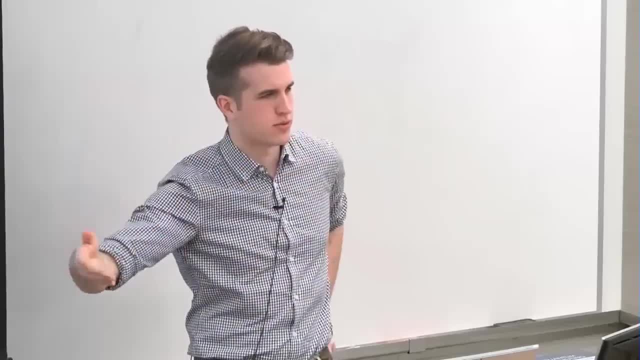 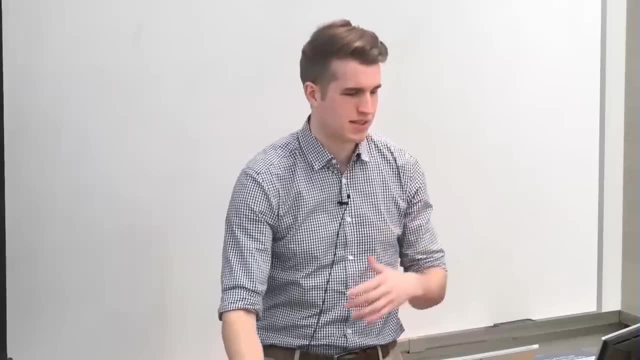 There could not be two ones, because that would actually violate our a squared plus b squared equals one constraint. Okay, But yeah, after measurement, there will only be one one here in this four vector, which we can then factor into two bits actually. 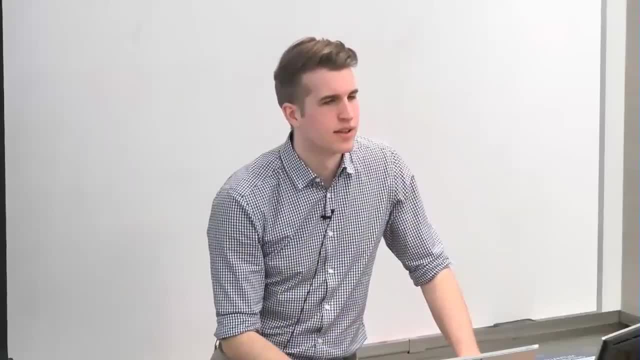 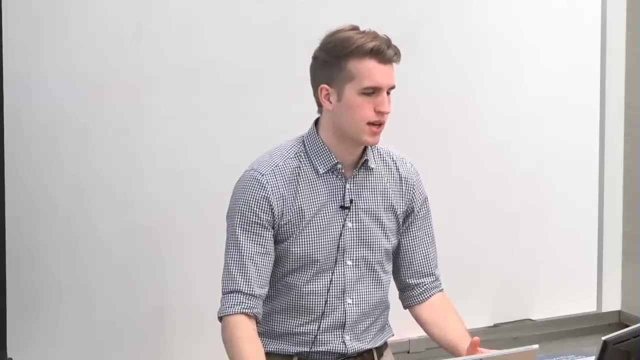 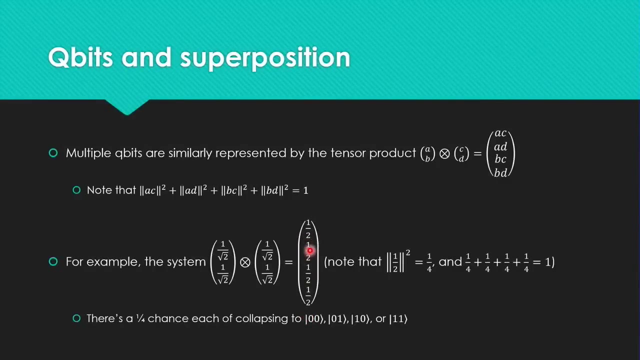 Okay, Yes, Could you also define collapsing for that longer vector? Yeah, So if you measure these two qubits at once, you can think of this product state vector as collapsing, And then that's just the probability of finding a one here and a zero everywhere else. 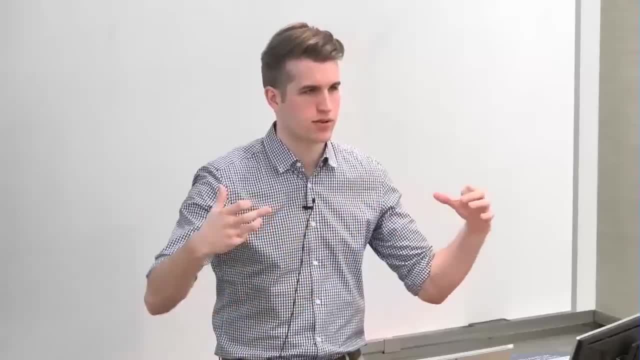 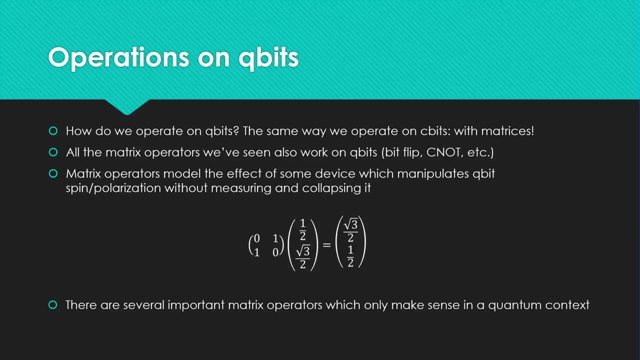 It'll become useful in the future when we can't actually factor out the product state. but that's anyway Okay. How about operations on qubits? We have these qubits. how do we actually manipulate them? The same way we do with the classical bits? 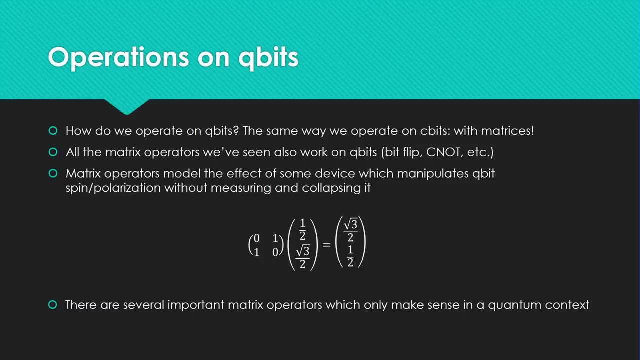 and all the matrix operators we've learned also work with qubits. So, for example, negation. If we have our qubit that has a 25 percent chance of collapsing to zero, 75 percent chance of collapsing to one if we run it through the bit flip. 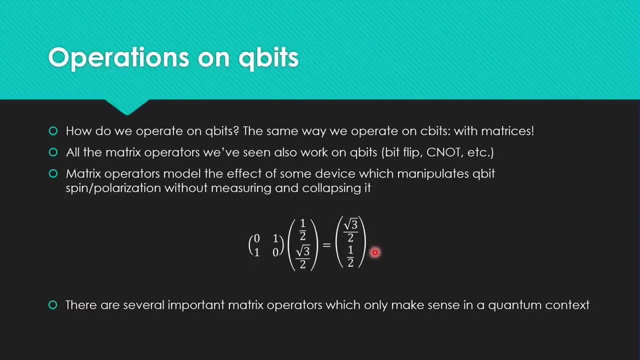 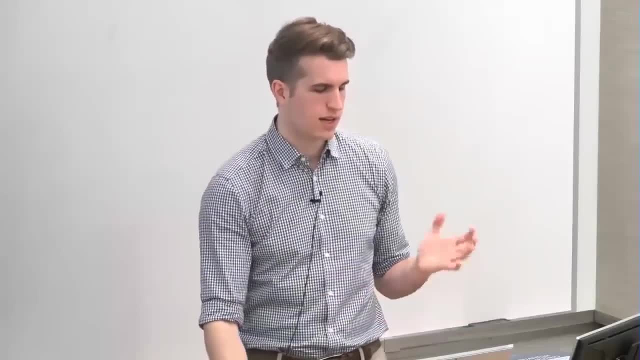 operator. now it has a 75 percent chance of collapsing to zero and a 25 percent chance of collapsing to one. So we can manipulate these probabilities- They're actually called amplitudes with gates, And you can think of a gates. 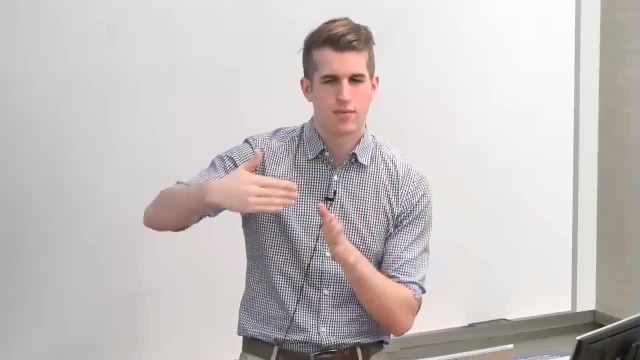 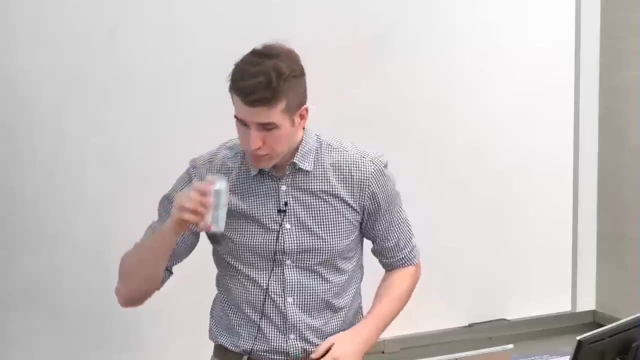 they correspond to some device scientists have created which manipulate the qubits with a gentle touch. Not enough to collapse them, but enough to change their state. So pretty neat. And there are also a couple important matrix operators which we haven't learned yet, because they only 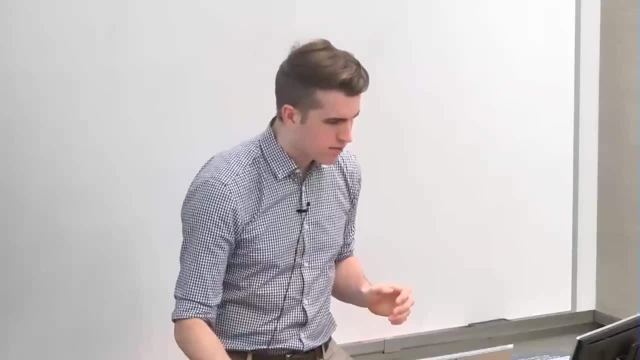 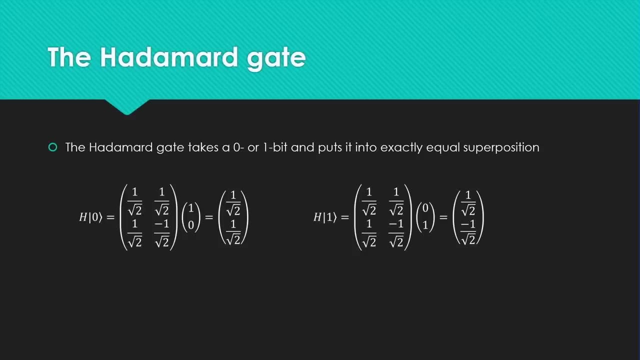 really make sense in a quantum context, The what is okay, sorry, Okay, All right, we're good. The most important one is the Hadamard gate, And what it does is it takes a zero or one qubit. 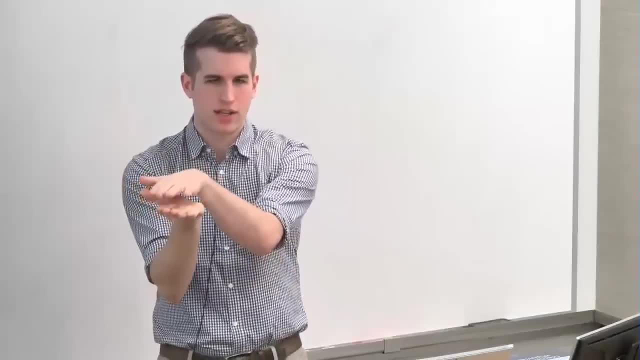 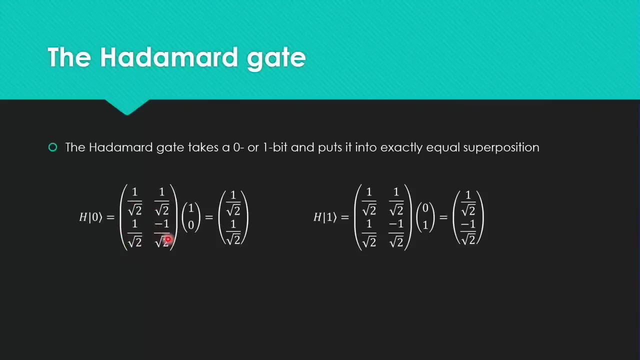 and it takes it to the coin flip state where it's in exactly equal superposition. The matrix looks like this: It has one over root, two in every single entry, except for a negative in the bottom right corner. So if you multiply that by this, 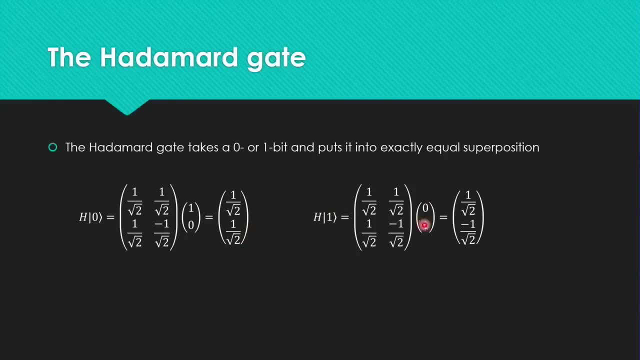 you get one over two, one over two. If we multiply this by one, we get one over two. negative one over two. So if we multiply this by one, we get one over two. negative one over two. Pretty neat. 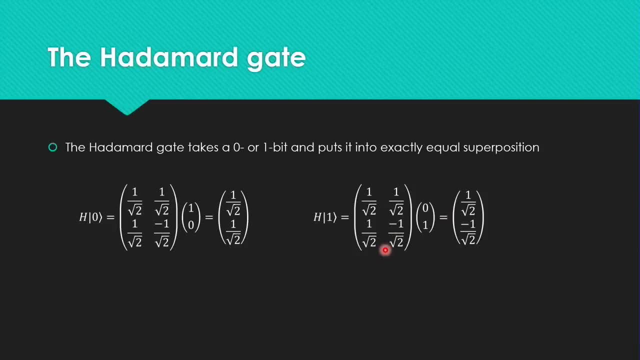 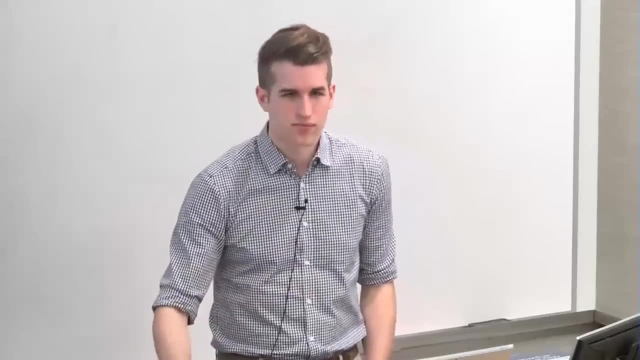 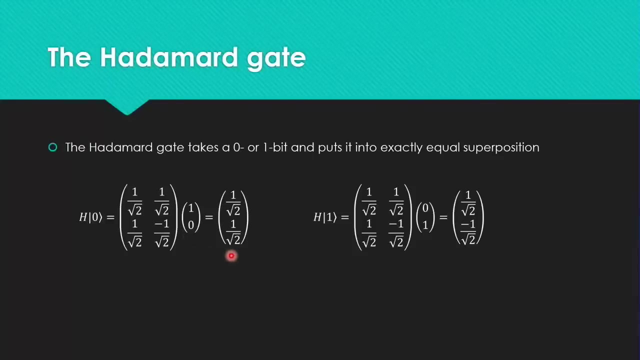 So this is how we actually get into superposition. We use the Hadamard device, which scientists have developed, and we can make much use of So kind of quiz time. Can anyone tell me why we need a negative one in the bottom right corner? 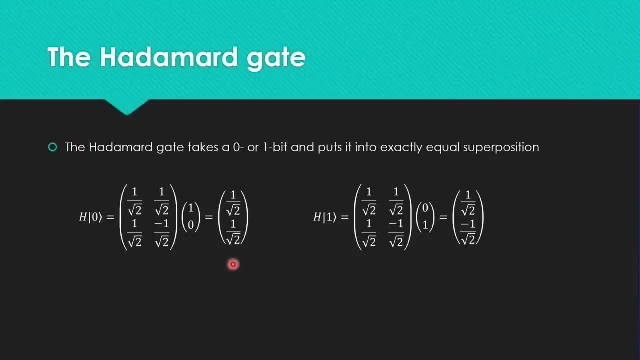 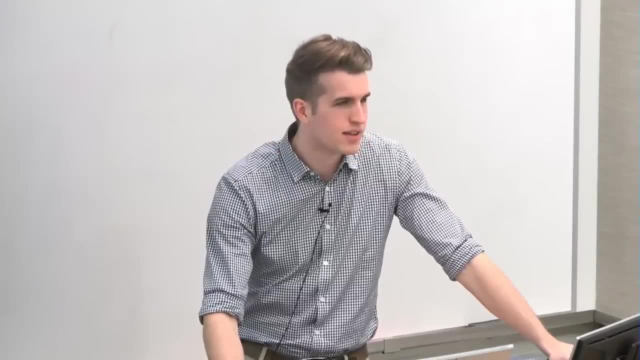 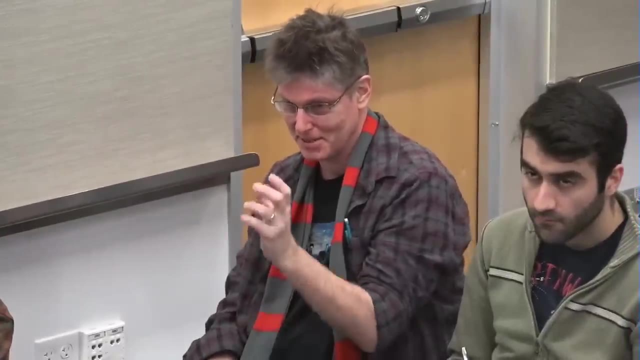 Why do we need a negative sign here? It's like a matrix, almost like a. I don't know exactly why, but it seems like it's Well. the answer, basically, is it has to be reversible. So if we didn't have this negative number here, 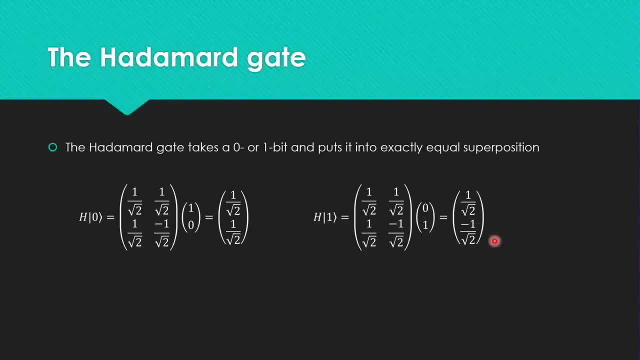 then both zero and one would map to the same value and it would not be reversible. So we need this negative sign. Yes, correct, Okay, Wait question. Yes, Review of superposition. what does that mean exactly in this? 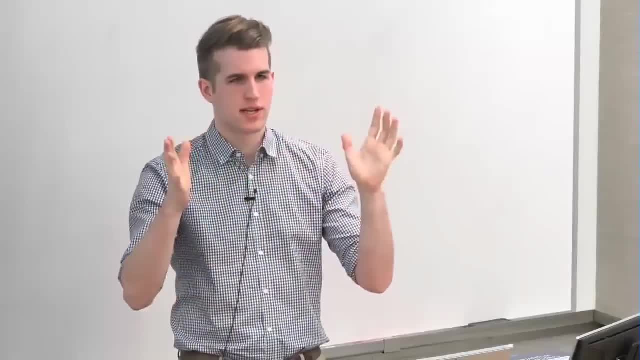 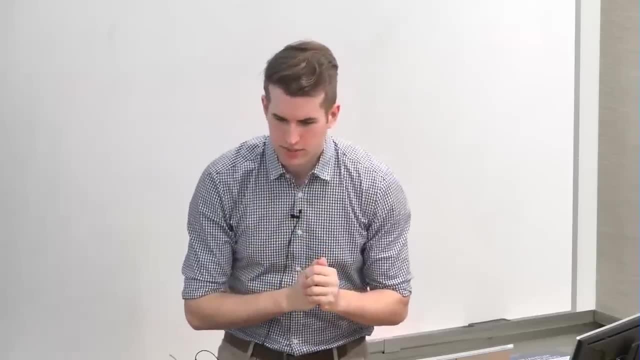 Superposition. yeah, So superposition means that, like qubit is kind of in both states zero and one at the same time. Okay, And I want to be, I guess, really clear about something here. This doesn't mean the qubit is secretly zero, or 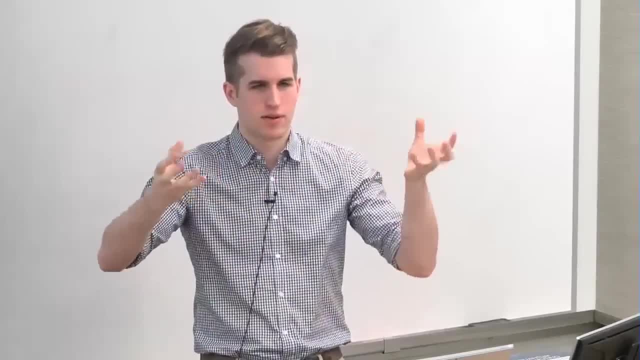 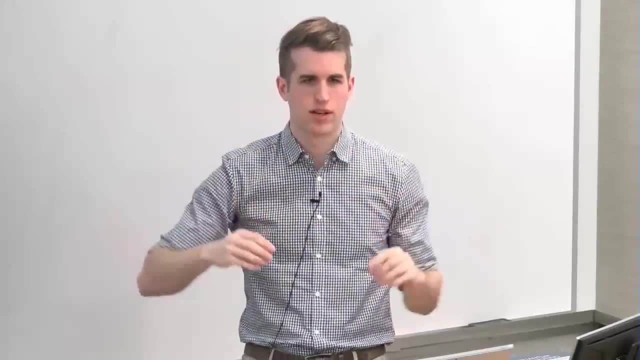 secretly one and we don't know. It means it's actually in both at the same time. This is like just quantum weirdness. This is just like what happens at the very, very small level of our world, which is that things don't have. 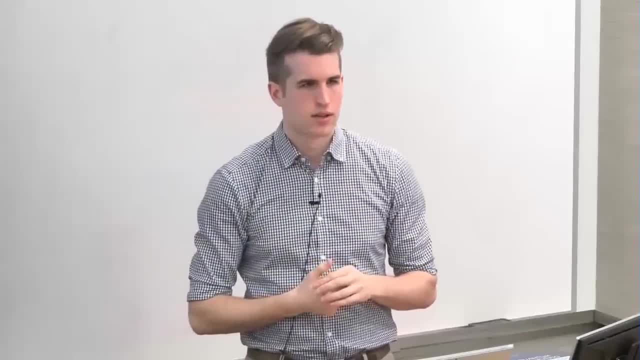 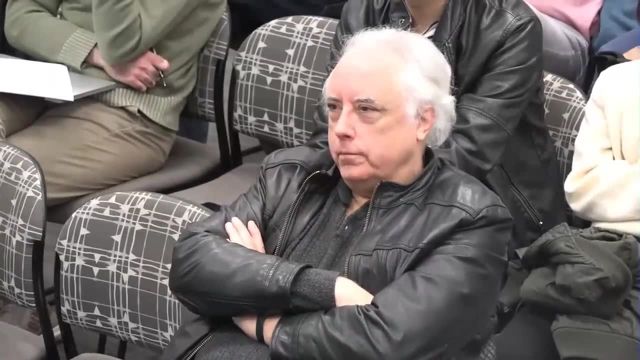 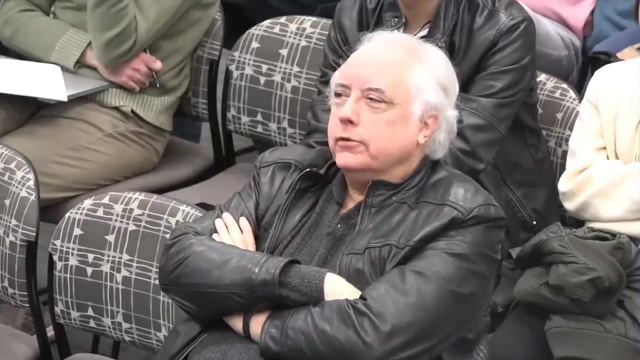 definite values until we measure them. But here you have zero when in superposition is one over root two, one over root two and one in superposition is one over root two minus one. So they seem to have different values, but they're representing conceptually the same thing. 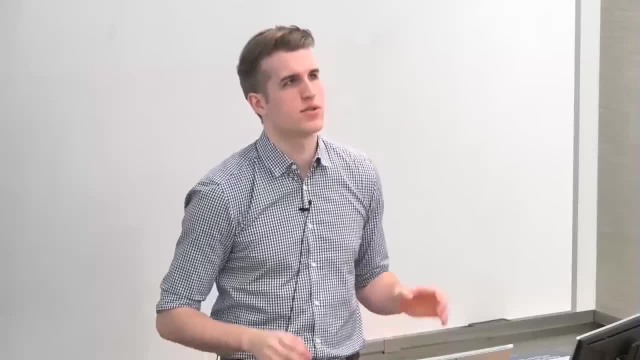 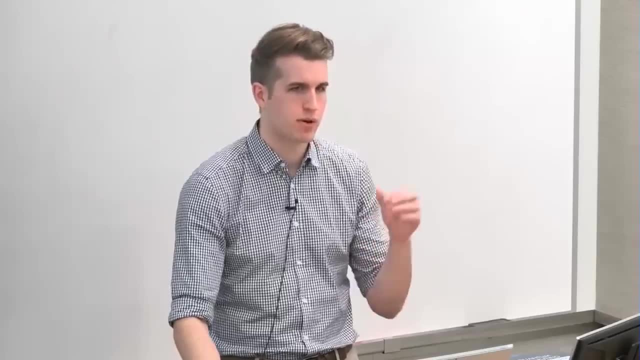 Right. So this kind of comes down to the distinction between the quantum and classical world, which is that from the classical perspective these two qubits are kind of the same. They both have 50 percent probability of collapsing to zero or one. 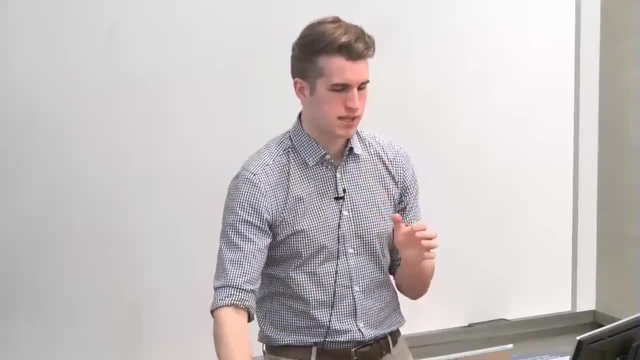 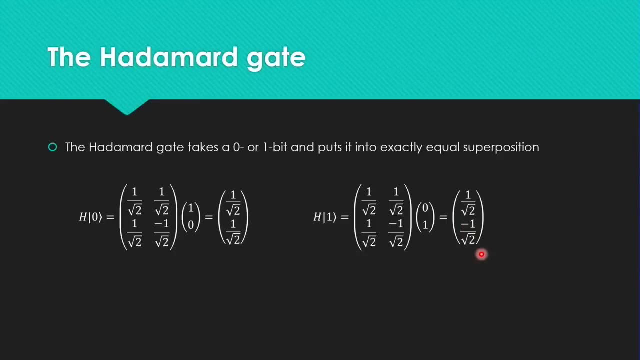 But if we stay within the quantum realm, this sign information. this information is preserved as long as we don't measure it and it can affect our computations. So it's kind of like it's got a 50-50 chance, but it has a sense that it used to be a one. 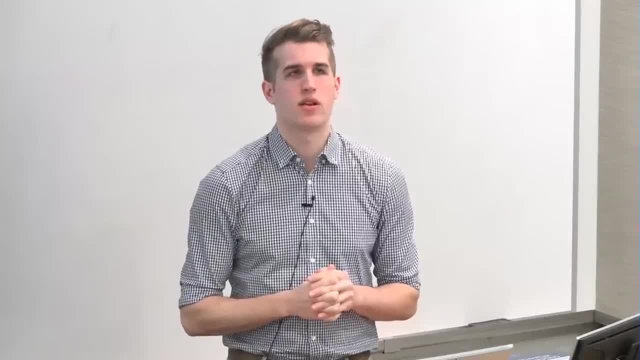 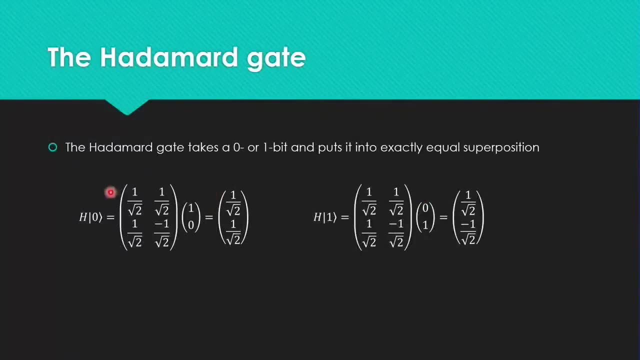 It has a sense that it used to be one. Not really, it's just it ends up in this state, which is different, within the quantum realm, than this state. These are two different states. Okay, Yes, Both with a 50-50 chance. 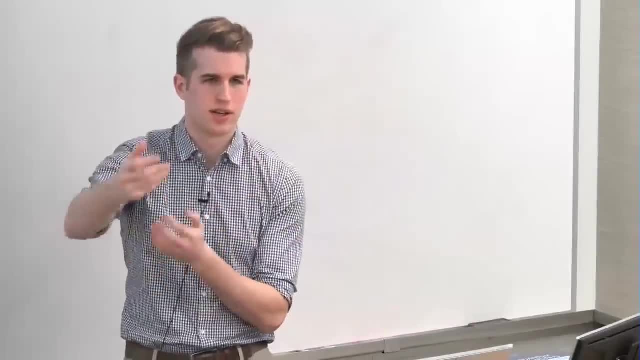 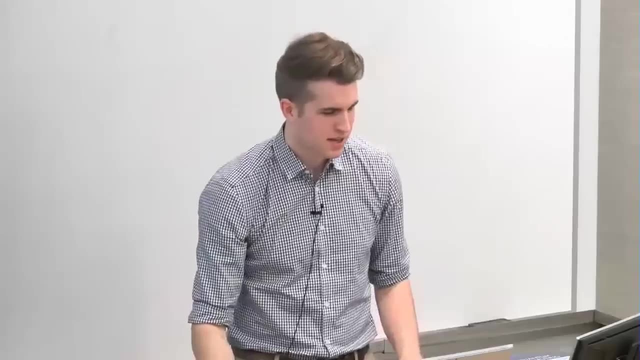 Yes, exactly Both. when you measure it and convert it into the classical world, come down with a 50 percent, 50-50 chance. Yes, but they are different and they have different computational properties. Okay, Now I'm going to show you something really. 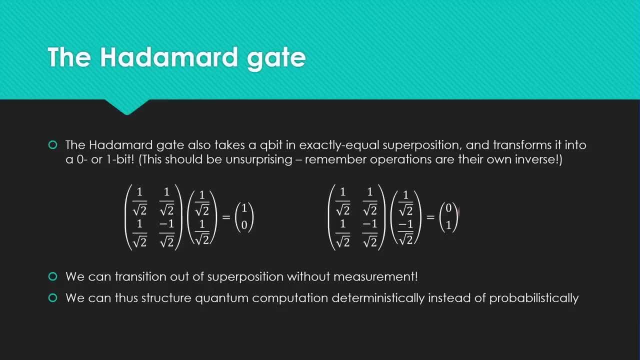 cool about the Hadamard gate which it actually takes us out of superposition into the classical bits. This should be unsurprising. Everything's its own inverse right If we just apply the Hadamard gate to our value here, our coin flip value. 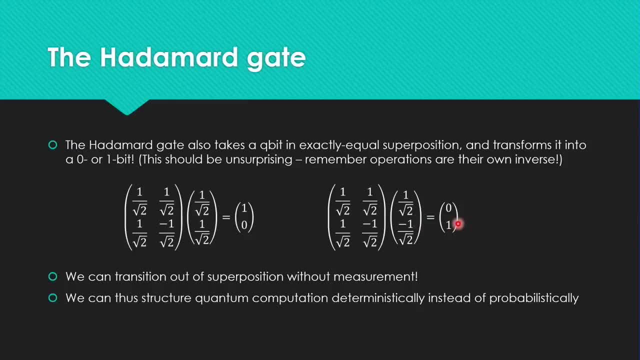 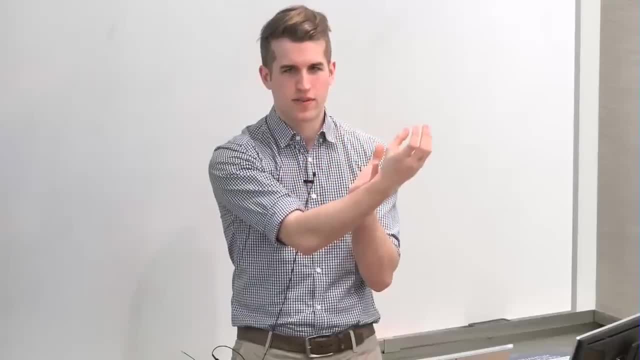 we get zero, and for this one we get one. So this suggests to us a sort of quantum computation structure. We can start with our classical bit values. we put them into superposition, do a bunch of quantum stuff to them. 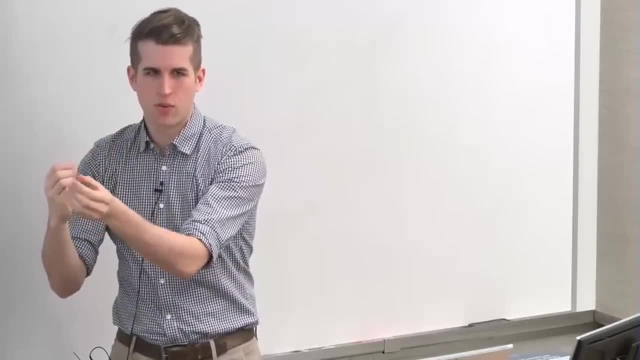 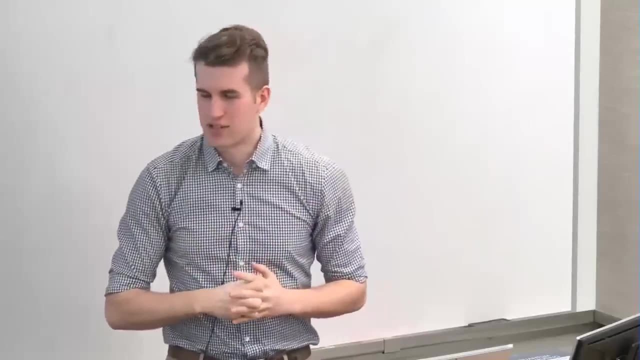 and at the end, if we're clever, we can transition them to zero or one, so that our whole computation was deterministic. Pretty neat, right? Okay, Now I should say that not all algorithms work this way. There are algorithms like Shor's algorithm. 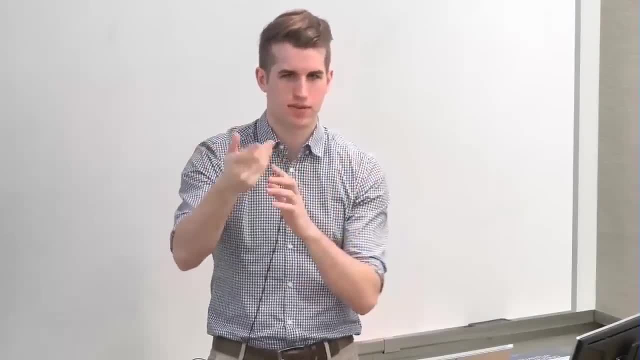 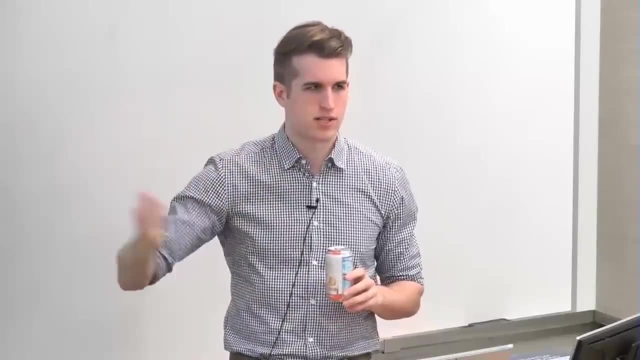 which only gives the right answer 50 percent of the time. You can't be clever and always get the right answer. It's just not doable. But the one the problem we'll look at- does give this sort of deterministic property. 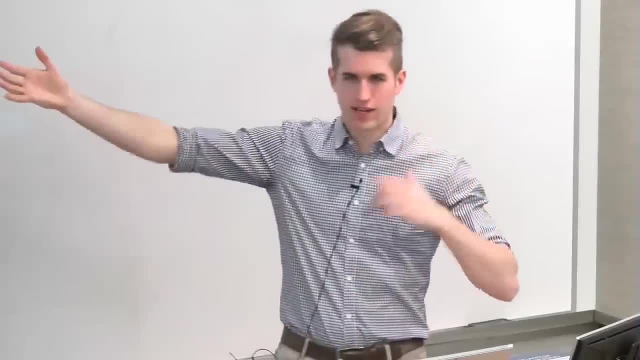 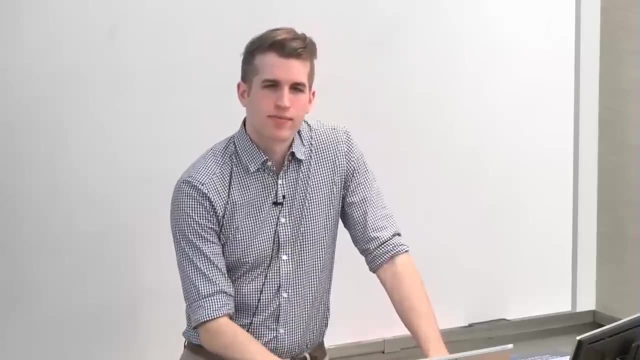 So does anyone have trouble with this concept? We can transition out of superposition without measurement. Pretty interesting. Can you go over this transition from a classical computation to quantum and then converting it back? Yes, That's correct. Like, let's say, two plus two. 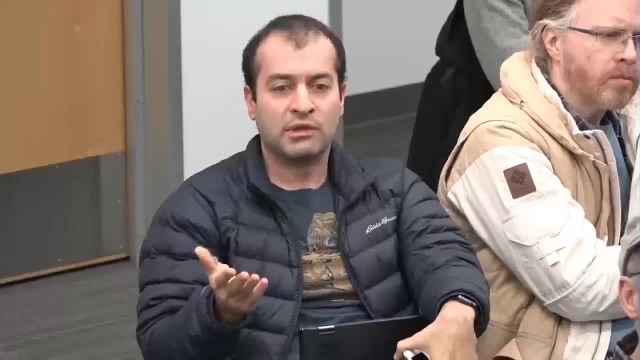 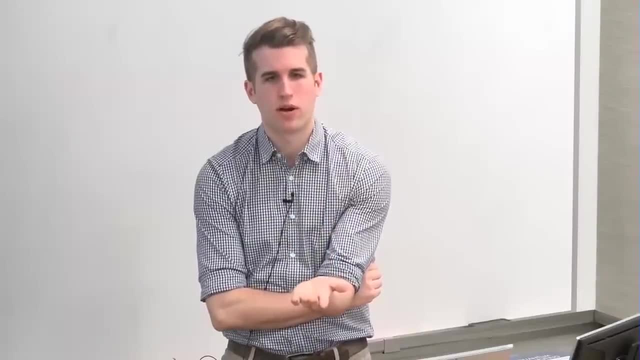 how would that look like? I mean, just the simplest type of math, The simplest type of math. Well, we're going to go over that. basically, We're going to go over a problem. There are certain problems where quantum computers are better than classical. like addition is not one of them. It works the exact same way in both. It should also be said that all classical computation can be done on a quantum computer. All you do is just restrict all the values to zero and one, and it works, But it's kind of a waste. 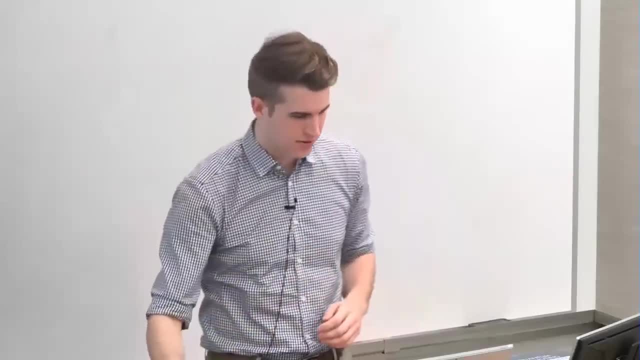 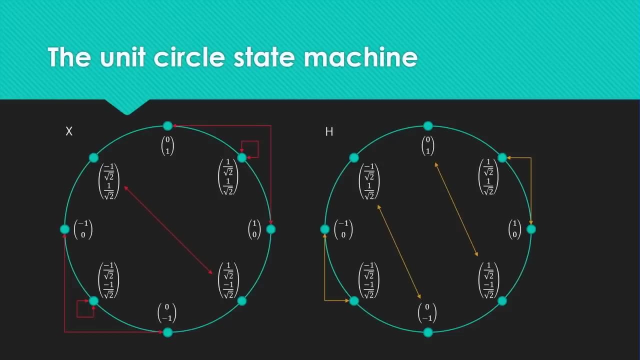 because you can also use all the extra values that we found Okay, And we've actually sort of defined a state machine here, which I'm sure many of you will appreciate if you're software engineers or computer scientists. Here is the action. Okay, So this is the unit circle. 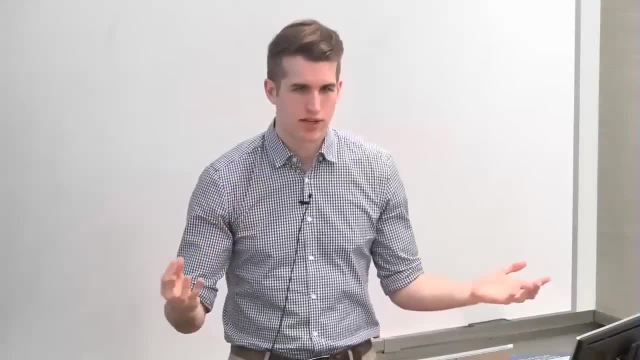 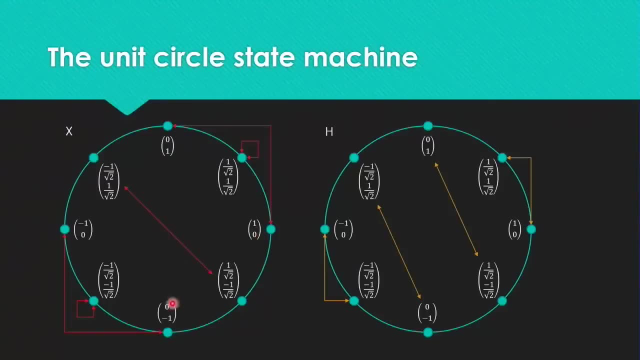 which many of you will remember from high school trigonometry. right, It's a circle of radius, one around the origin. Here's the x-axis, This is the y-axis You can think of. the top value is the value of the x-value, and 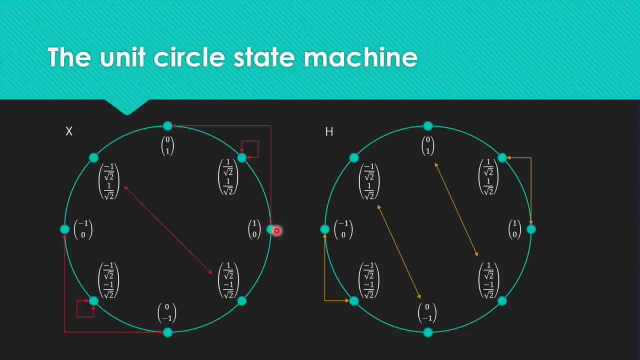 the bottom one is the y-value. So our zero value is at position one, zero which is along the x-axis. Our one value is at position zero, one which is along the y-axis, And this is the bit flip operator. 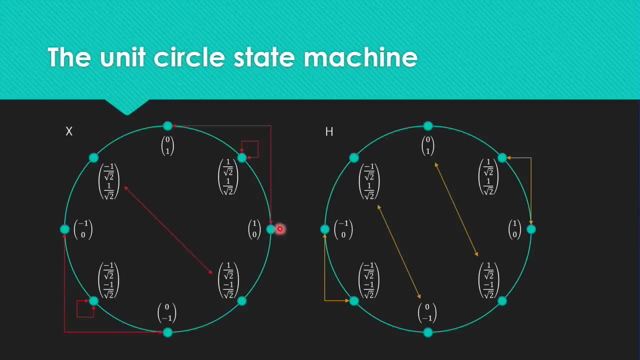 It defines transitions around this unit circle. So zero goes to one, one goes to zero, Zero. negative one goes to negative one zero which, when you collapse them, this is zero, this is one, and vice versa. Excuse me, 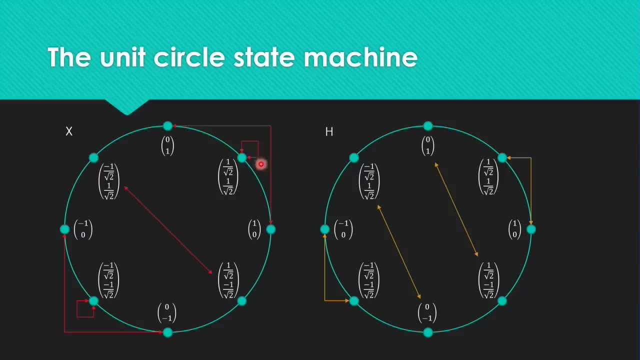 And if we look at the superposition values, here's something interesting: The bit flip operator really has no effect on them. For this one, if you flip it upside down, it stays itself. same with this over here. This one's interesting in that it transitions you. 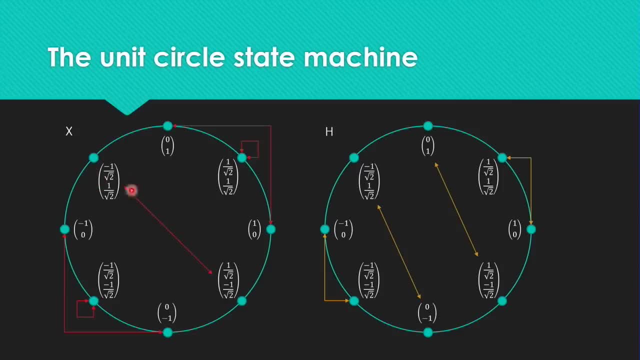 all the way across the unit circle and we'll make use of that. But yeah, okay, This is pretty much the full action of the bit flip operator on the unit circle. I should mention here that if we were using complex numbers, this would actually be a sphere. 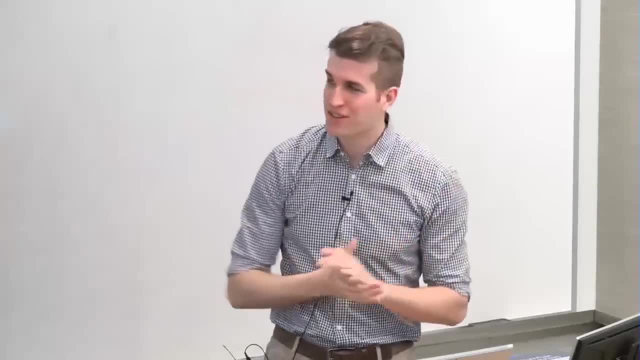 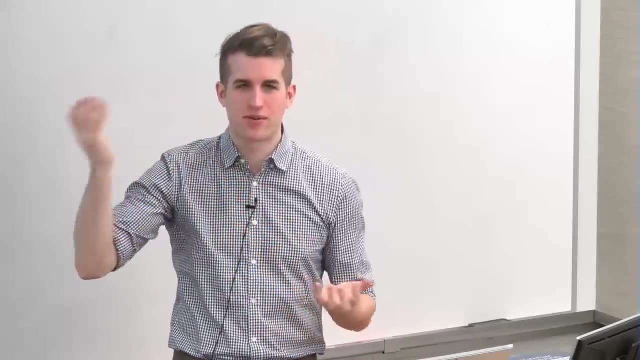 Much more difficult to intuitively represent or graphically represent. So we're sticking with real numbers. They suit us just fine, But it's nice to know that additional dimension is always available to us if we want to make our computation even more powerful. 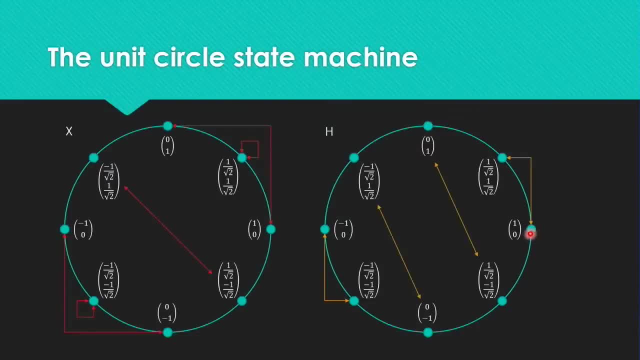 And then here's the action of the Hadamard gate which we saw the past couple slides. It takes us from zero to one over two, one over two, one to one over two, negative one over two, and kind of symmetrically. it also works in this way over here. 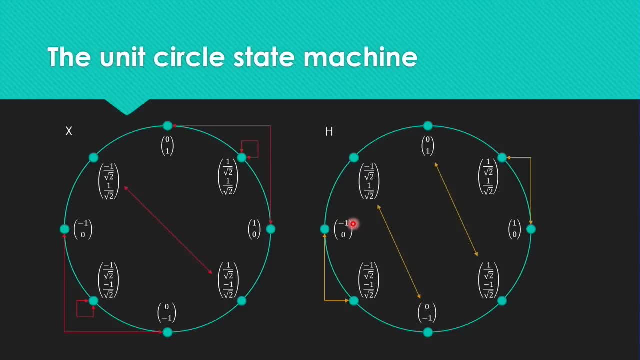 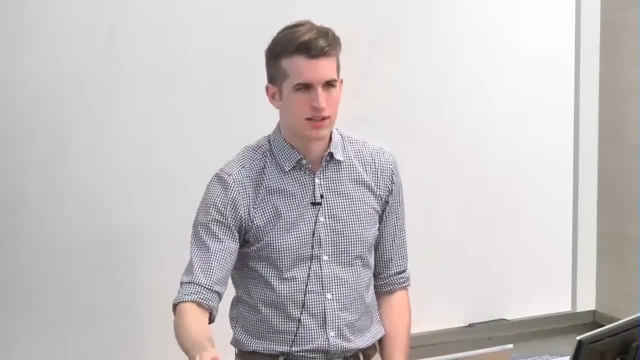 So we have a nice state machine that we've developed and now we can start running things on the state machine. Very nice, intuitive sort of representation. You don't need to do matrix multiplication all the time. Everyone kind of gets this. Okay, Great, So here's. 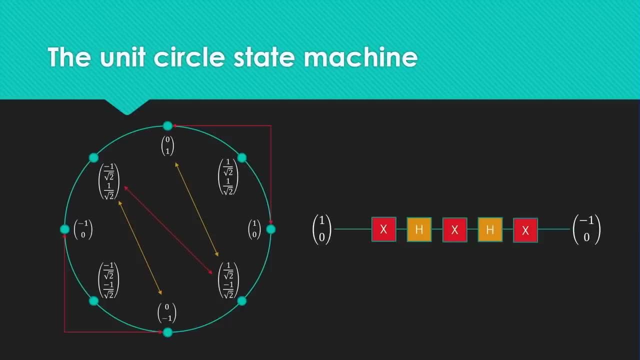 an example of something we could run through the state machine. Here I'm introducing something called quantum circuit notation. You can think of the qubit traveling along this line, has these operations applied to it as it goes through the boxes. So X is bit flip, H is Hadamard. 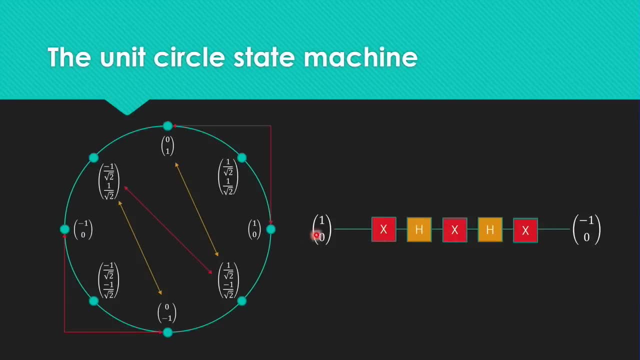 and then. so we go bit flip, Hadamard bit flip, Hadamard bit flip. If we start out here, we go bit flip, Hadamard, bit flip, Hadamard bit flip. So we start out at one zero and get to zero one. 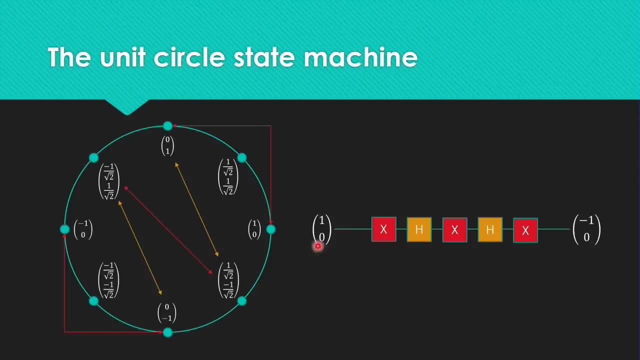 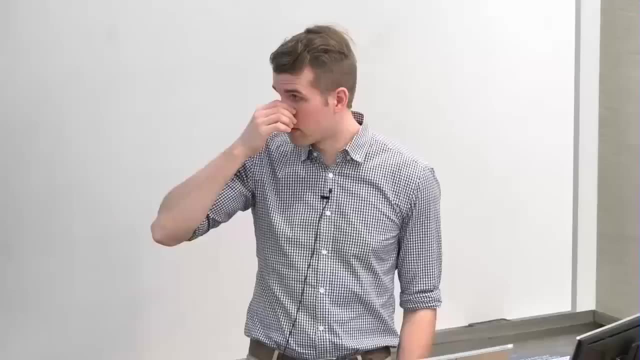 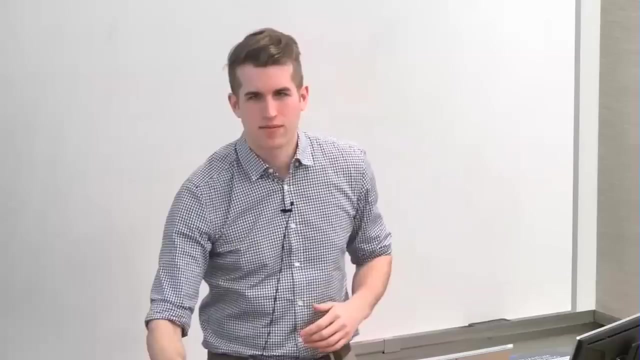 We get across the circle. Note: this is reversible, so we can also go this way and get back. So this is kind of how we'll be doing all of our computations like this, basically just hopping around the unit circle. Pretty simple, pretty intuitive, right. 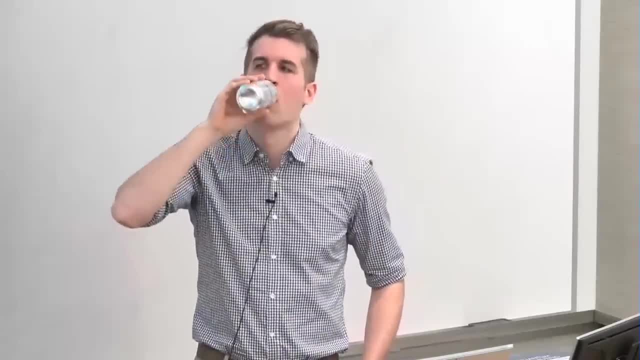 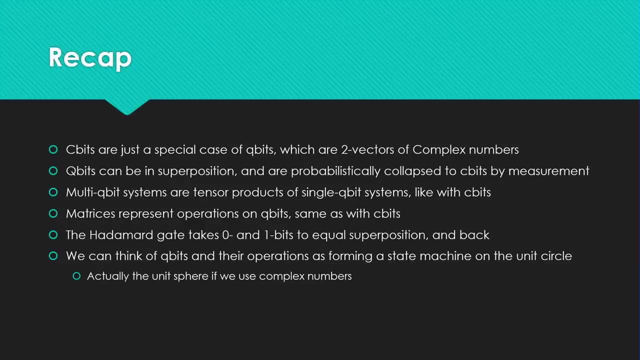 It's just a state machine. We've seen we use this in classical computing all the time. It just has a bit of weird rules with collapse and whatever, but don't worry. Okay, Now we have everything we need to learn the simplest problem. 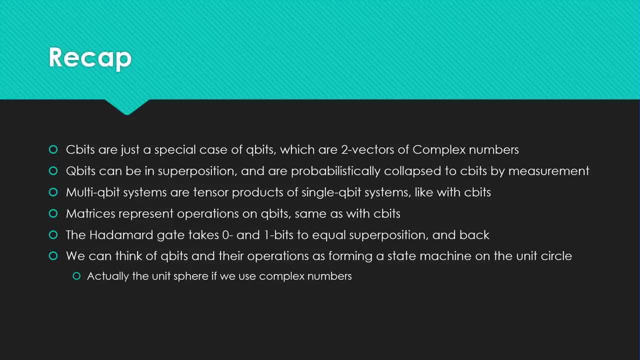 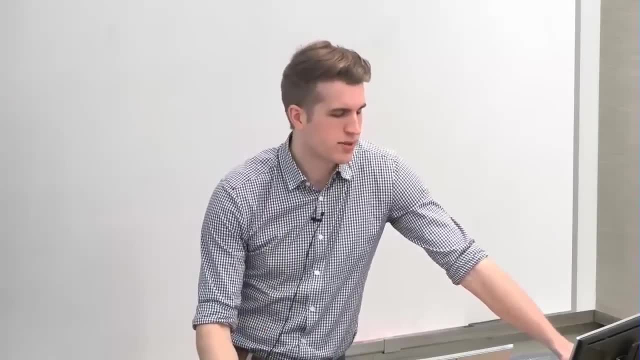 where a quantum computer over forms a classical computer. We learned that cbits are just a special case of qubits, and qubits are two vectors of complex numbers, such that a squared plus b squared equals one. We learned that qubits can be in superposition. 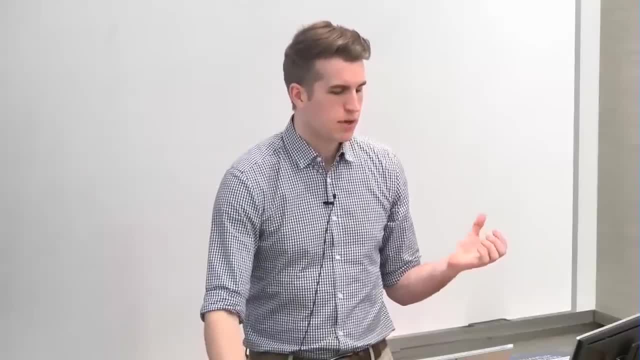 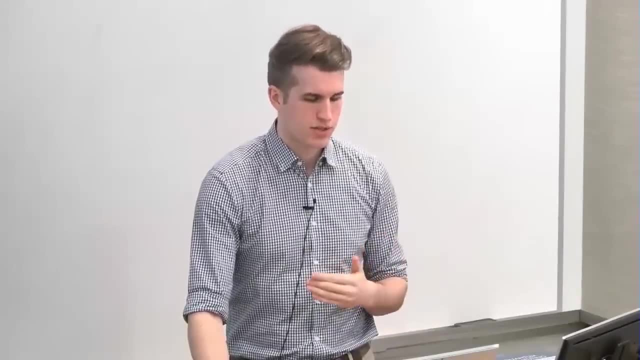 They are probabilistically collapsed to cbits by measurement. Multi-qubit systems, we learned, are tensor products of single qubit systems, same as with cbits. Matrices again represent all of these. They represent operations on qubits. We learned about the Hadamard gate, very important. 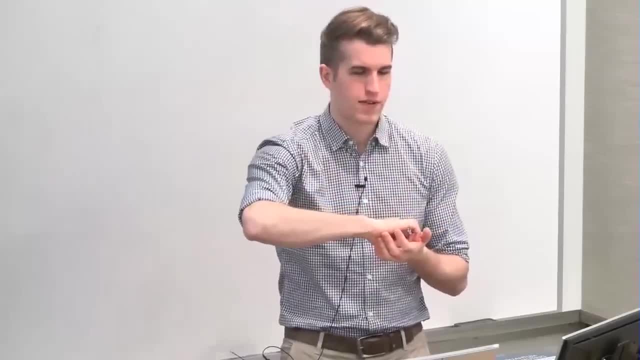 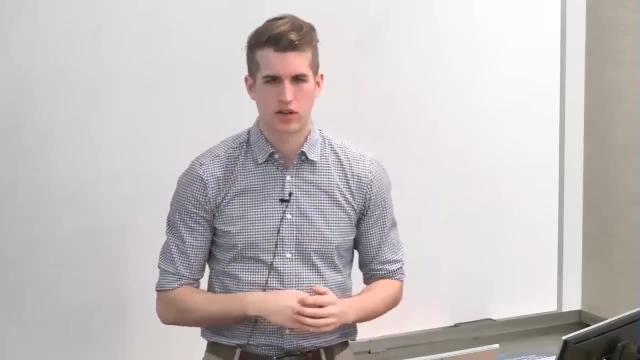 which takes our zero and one bits to superposition and back. Finally, we learned that we can think of qubits and their operations as forming a state machine on the unit circle or unit sphere. if we're using complex numbers, It's actually called the Bloch sphere. 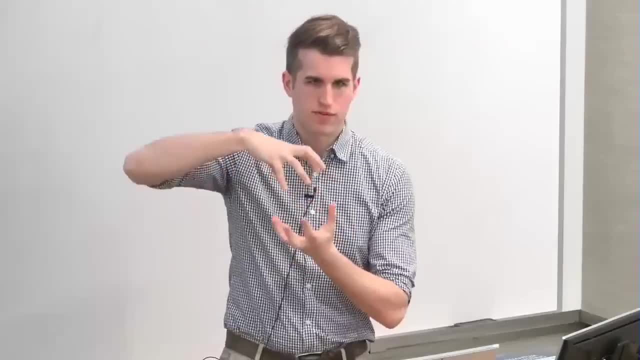 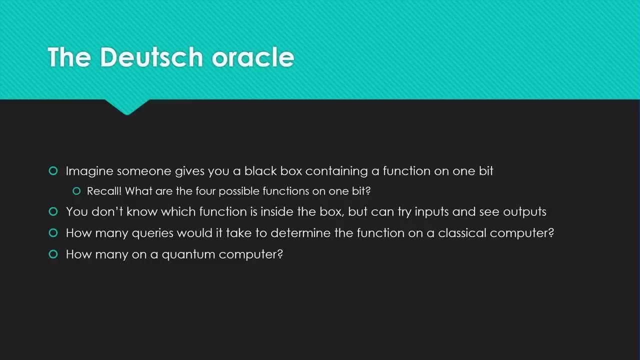 B-L-O-C-H sphere, if you want to look that up for the full complex numbers, but unit circle, just fine for us. Okay. So we're going to learn about something called the Deutsch Oracle, Originally proposed by David Deutsch in. 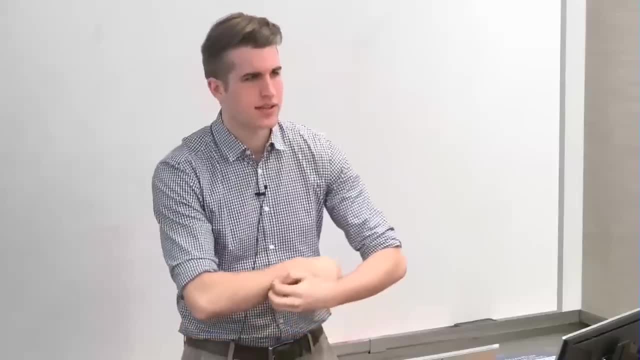 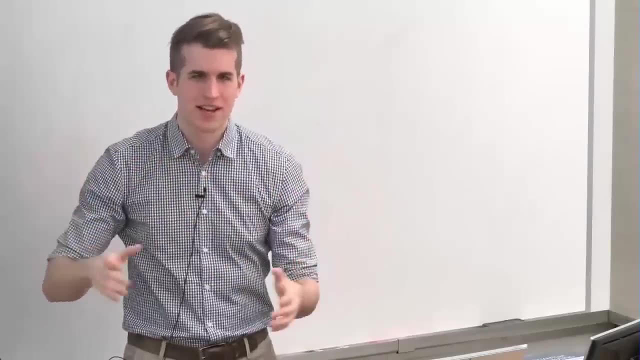 was it like 83 or something like that? The problem is this: imagine I show up at your doorstep and I give you a package. The package is just this black box. it's just a horrible present. It's a black box which has a function on one bit. 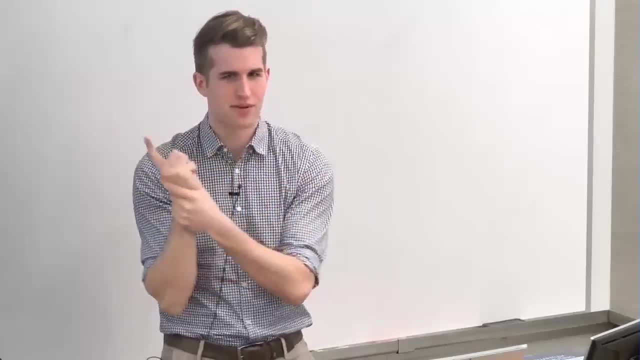 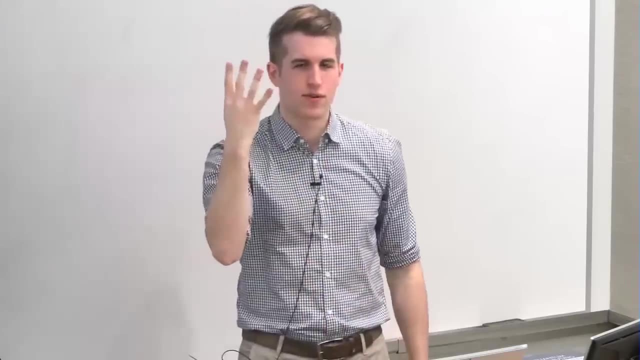 So it's one of those four functions on one bit. Do you remember what those are? I said I would ask you about them. Set zero set one. Set zero set one. identity negation, exactly. So one of those four functions. 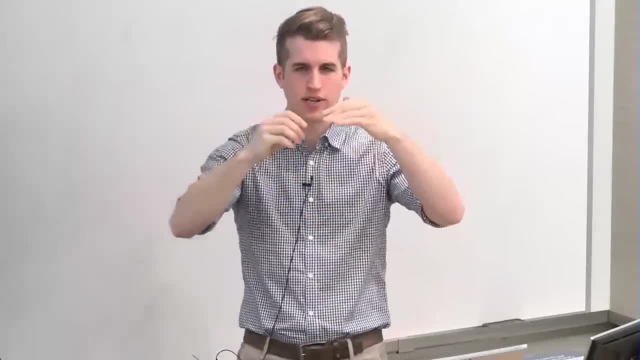 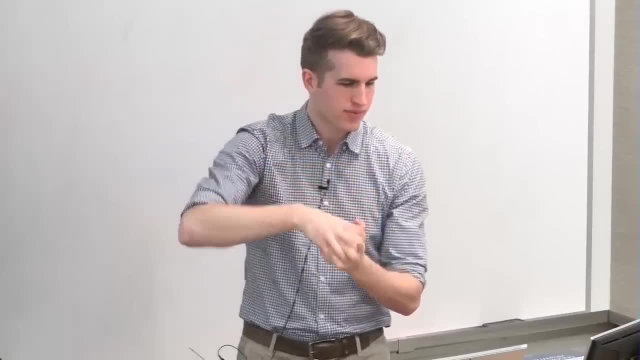 I don't tell you which one is inside this black box. It has a wire going in and a wire going out, So you can send in values, see what goes out, but you can't actually look inside the black box, okay. 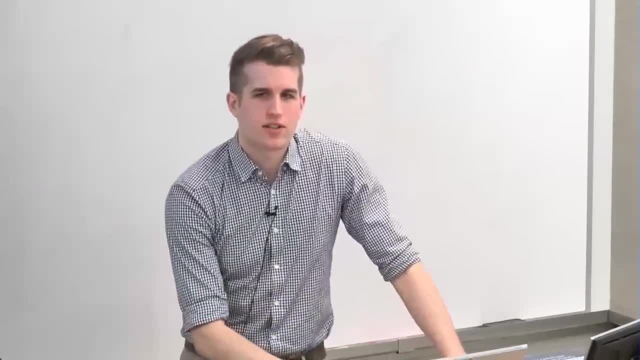 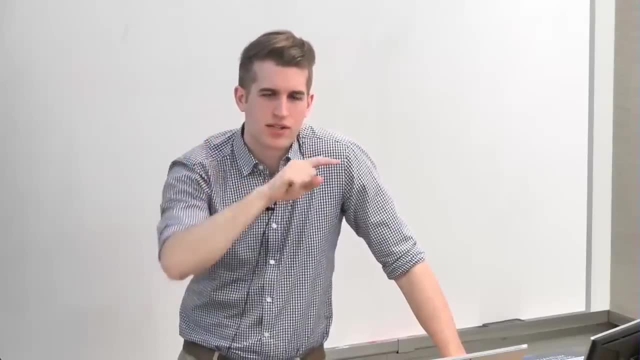 So how many queries on a classical computer would it take to figure out which function is inside the black box? Two, Two, exactly. You send in zero, see what comes out. You send in one, see what comes out. That will uniquely identify which function it is. 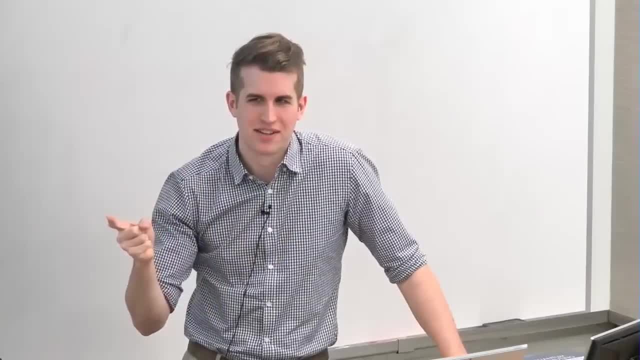 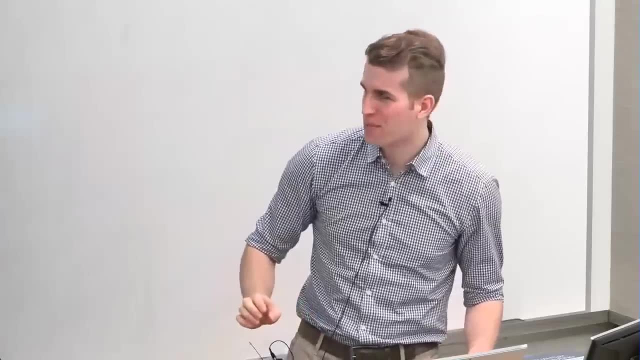 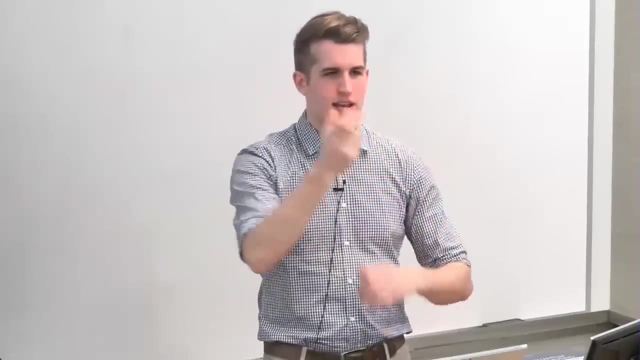 Now, how many queries do you think it takes on a quantum computer? One, You're wrong, It's two. I say this to illustrate an important point, which is quantum computers. they don't really compute with all values simultaneously. At the end of the day, 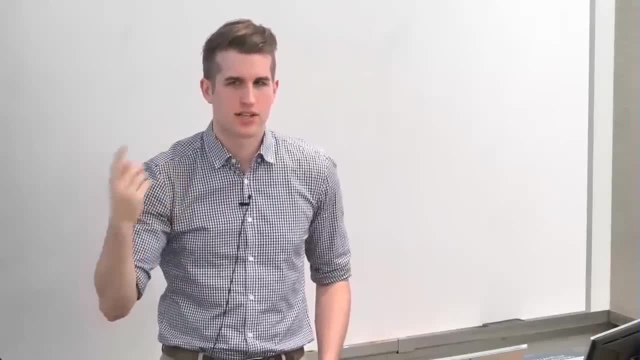 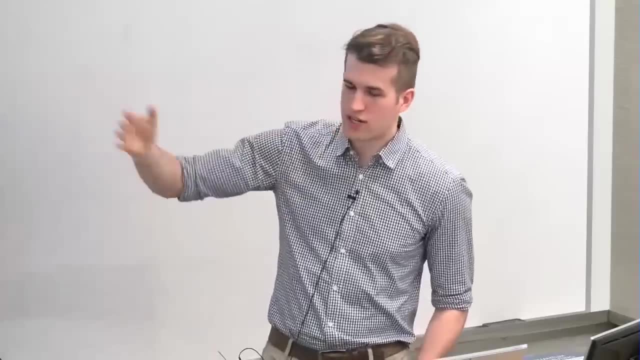 you collapse your qubit to a single bit of information, And a single bit of information is not enough to uniquely identify four functions. one of four functions? right, You need two bits at least. So this actually takes two queries on a quantum computer. 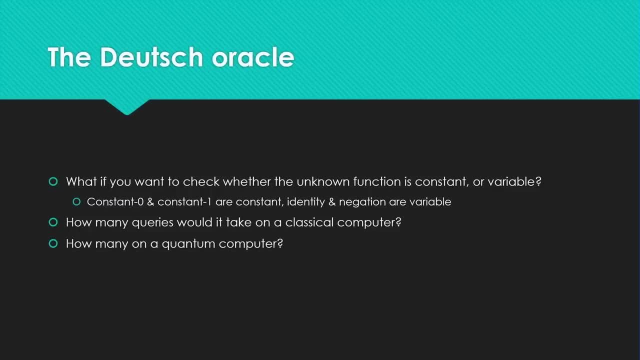 Well, not too exciting so far. Now, what if, instead of wanting to know which function it is, we just want to know whether the function is constant or variable? So the constant functions are the constant, zero, constant one. they always map to zero, always map to one. 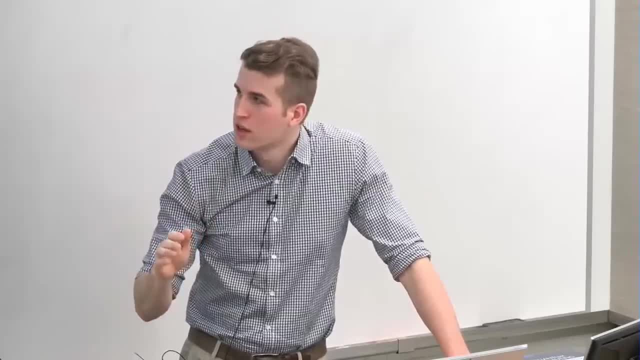 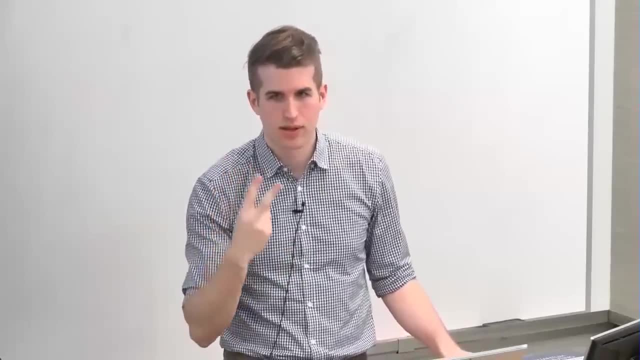 The variable functions are identity and negation. So how many queries would this take on a classical computer? Two, Two, You put in zero. If you get zero, you don't know whether it's identity or constant zero. If you get one, you don't know whether it's bit flip. 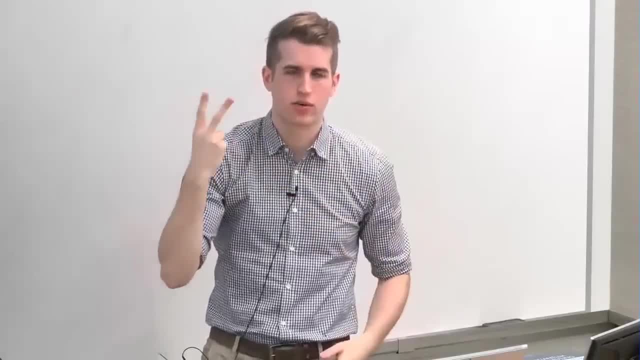 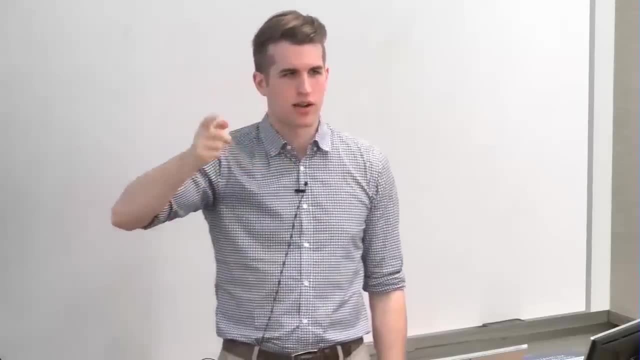 or constant one symmetrically with one. So it always takes two queries On a classical computer, even though there are two categories. So really we only need a single bit of information to tell us which category it's in. But how many queries do you think it takes on a quantum computer? 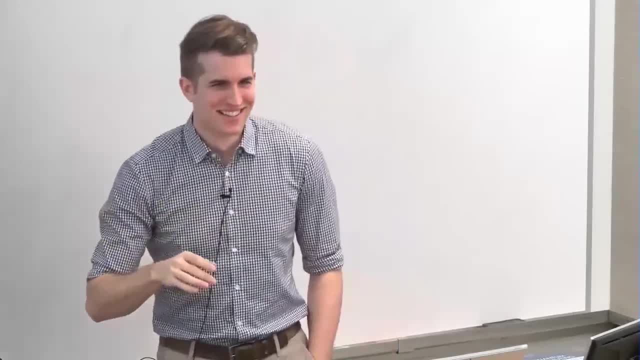 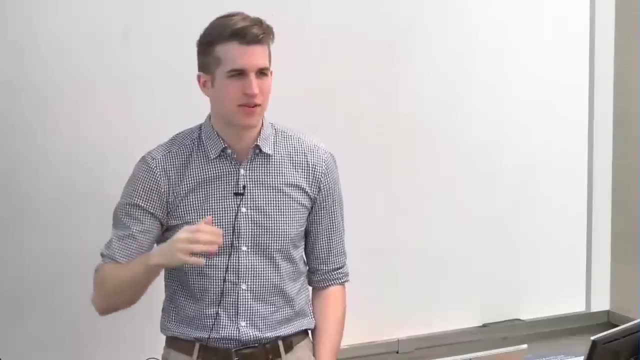 I've kind of burned you last time, so maybe you're a bit shy. I'm going for one One. You are correct, We can do this in a single query on a quantum computer. We can tell whether it's constants or variable. 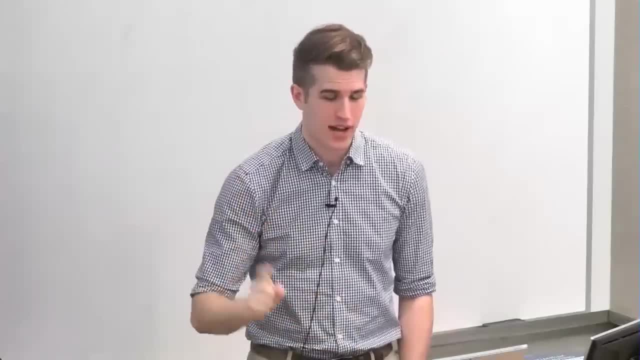 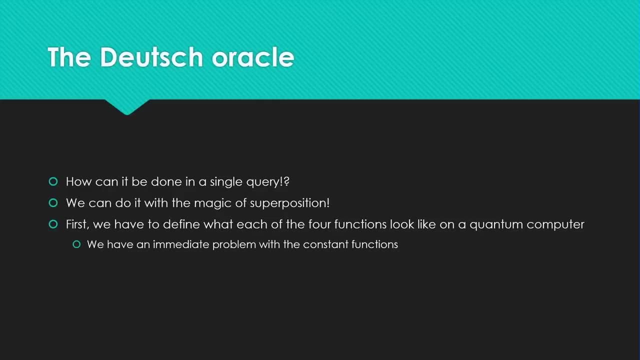 This like undeniably outperforms a classical computer and we're going to learn how. Okay, We deal with the magic of superposition, but first we have to define what each of those four functions look like on a quantum computer. We have an instant, obvious problem. 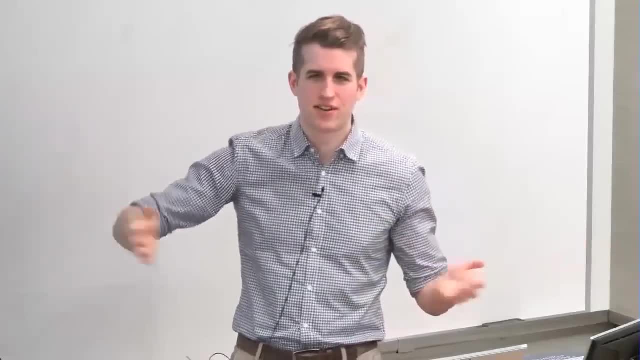 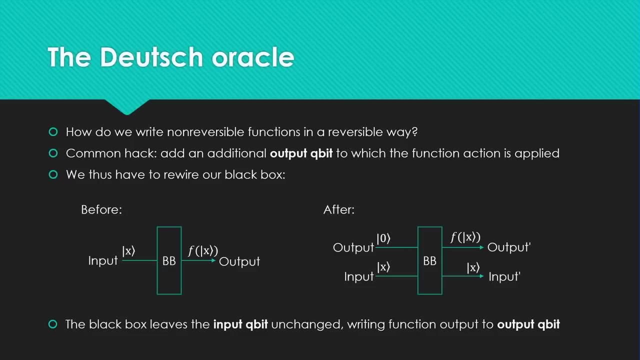 with the constant functions. Can anyone tell me what? it is Not reversible? They're not reversible. How are we going to write these non-reversible functions on a reversible computer? This is actually a really common problem in quantum computation. You really often have to deal with non-reversible functions. 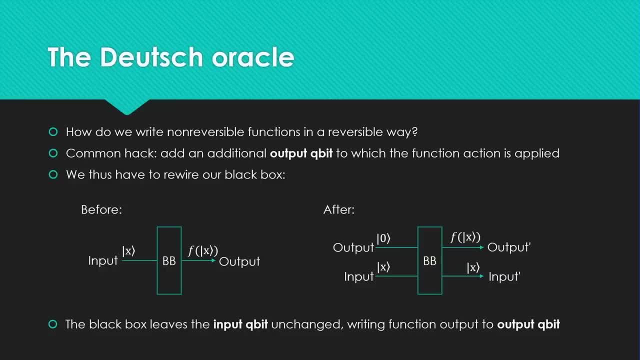 You have to write them in a reversible way, And the hack we do is this. So originally we had this. we had an input and an output, a single wire going through, And we just imagine that you put in the value and you get. 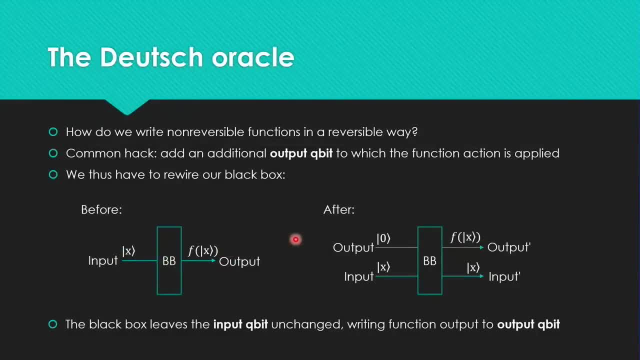 the function applied to that value, right. But the hack that you always do on quantum computers is you add an additional output qubit, So you actually have two qubits. We have to rewire our black box So you have your input qubit, which is unchanged. 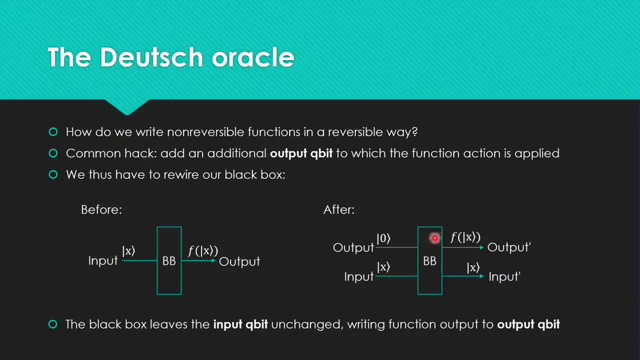 and then the value of the function on this input qubit is written to the output qubit. Does everyone kind of get this? This is, I think, the thing that people have the most trouble with This necessity. The reason we have to do this is so we can write. 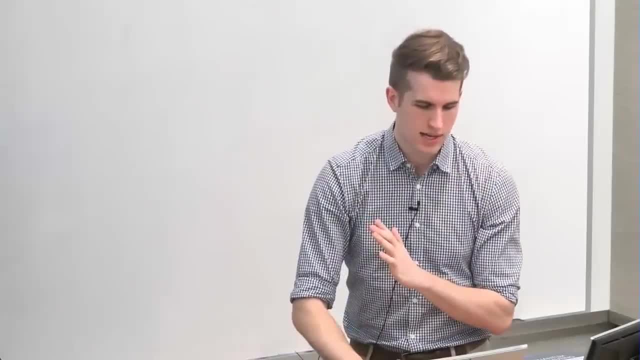 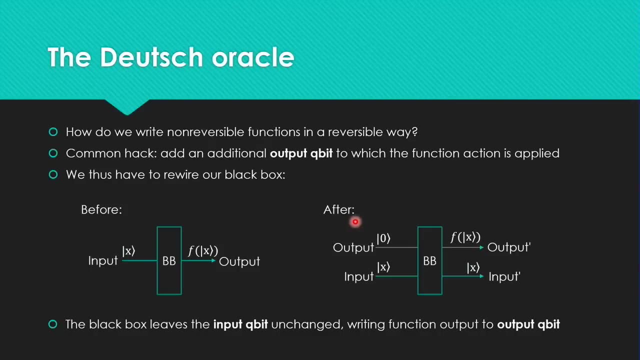 non-reversible functions in a reversible way, And the way to do that is to have a separate input and output qubit. So when you see larger quantum computations, instead of having all the bits go in and have transformations applied to them and then being measured, 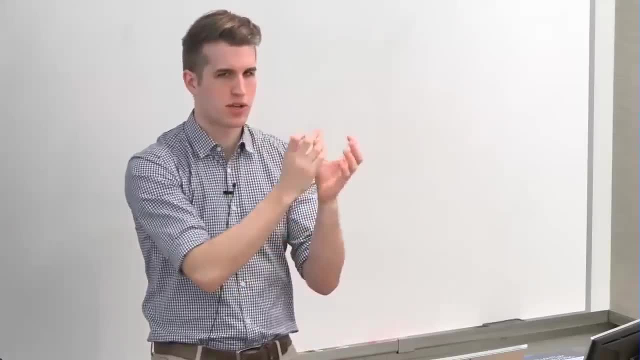 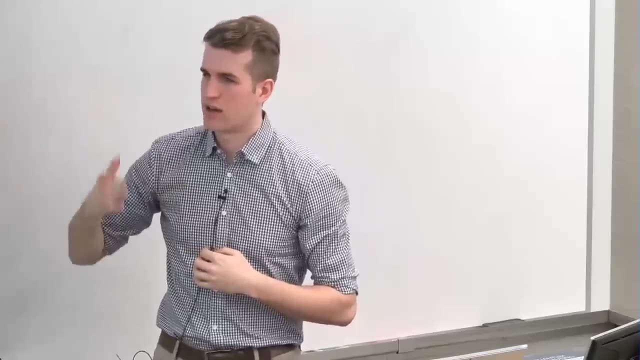 usually have a separate set of output bits. So the input bits go in, they have their value sort of written to the output bits and you measure the output bits. This is a very standard way of doing quantum computation, So does anyone have any trouble with this? 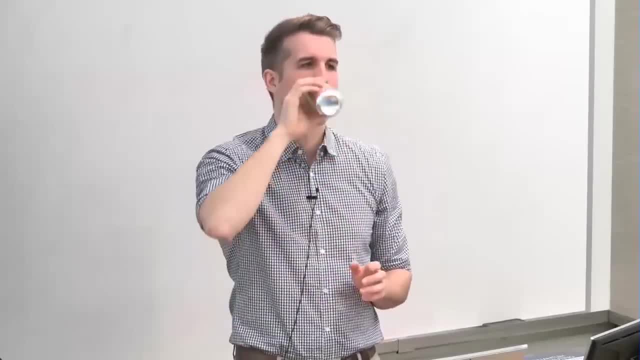 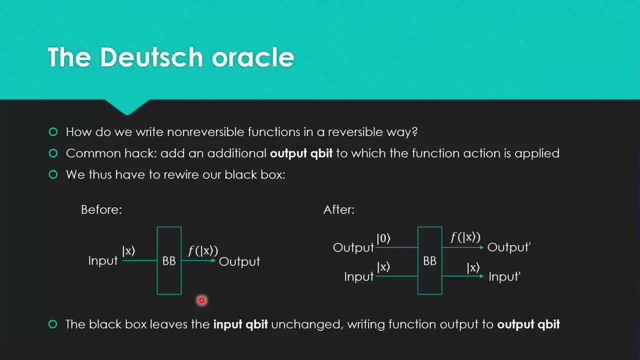 This is a very difficult concept. So, yes, I didn't get it. Yeah, Okay, Okay. So do you understand this model? basically, This is what we have now. Okay, We need to rewire it. So there are two wires going through the box now. 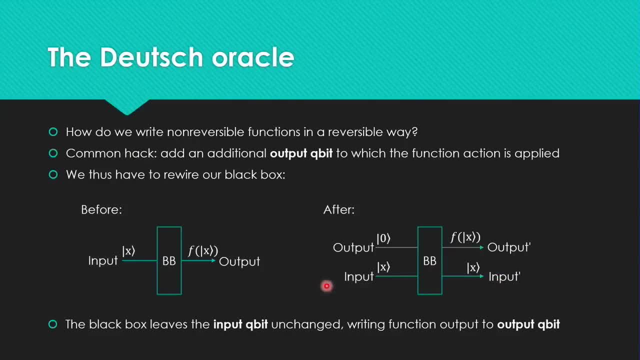 Okay, And one of those wires we call the input wire, one of those wires we call the output wire. We assume the output wire is just initialized to zero. Right, It's always zero. Now our input wire is what we actually give our input in. 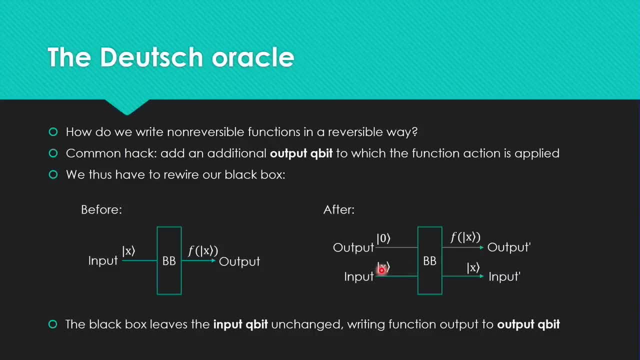 Like it'd be like zero or one or whatever value you want to give as input to the function. So it goes through the box. It's just unchanged. We don't touch the value of the input wire But we calculate the function in here on this input. 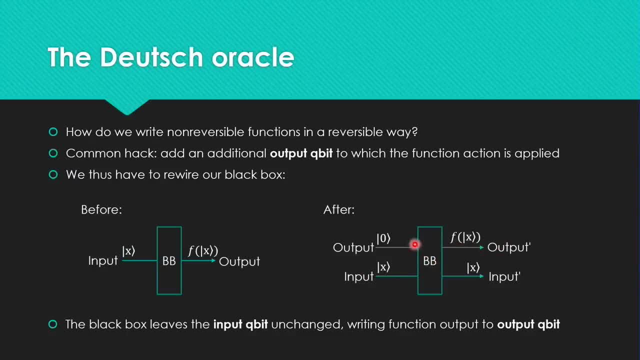 and then we write its value to the output wire. Okay, Can we rewire the black box? Yes, We are rewiring the black box. We have to rewire the black box in order for the black box to really work. So the black box I gave you has to be rewired. Yes, 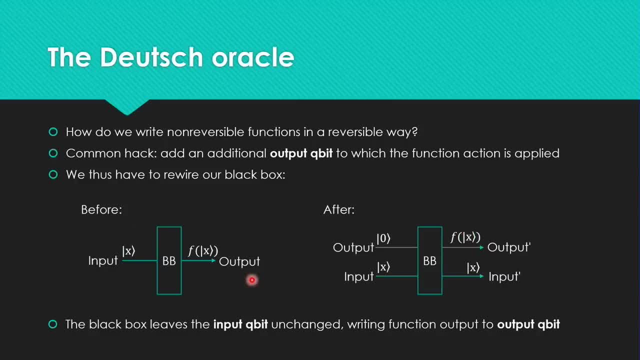 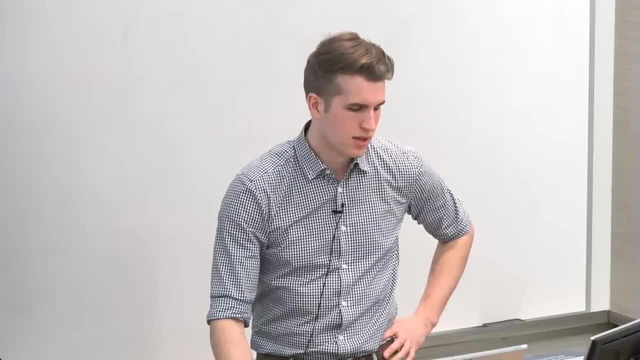 Did you use the first input, which is the output of zero? Did I use the first input? Yeah, Because one of them was kind of identity, right. You put the x out and then it was the f of x. One of them was x out and the other was-. 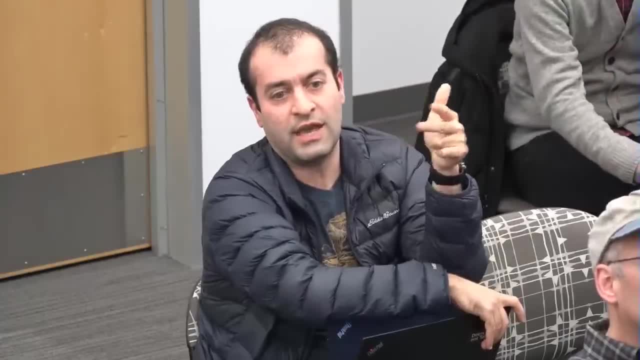 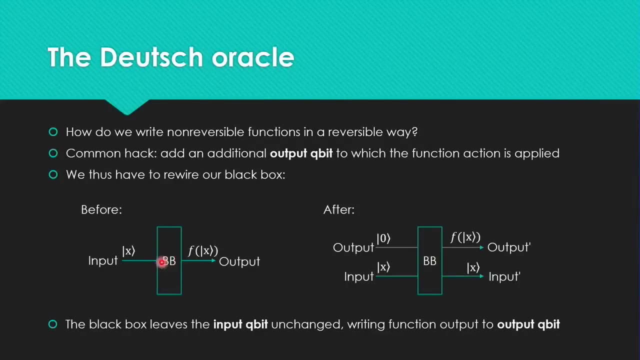 So why did we need the other input? So I guess you need the x out, Right? So say we only had this right. This is the old way of doing it. We can't have a non-reversible function in here, right? 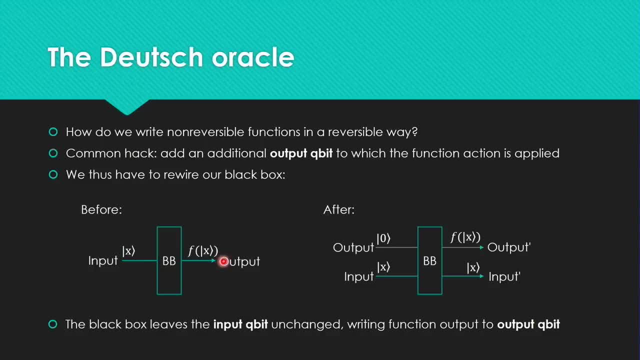 For it to be on a quantum computer. No, no, That I get, Okay. Okay, What I'm saying is that on the right side you have two going in, two going out. Yes, Two going in, two going out, Yes. 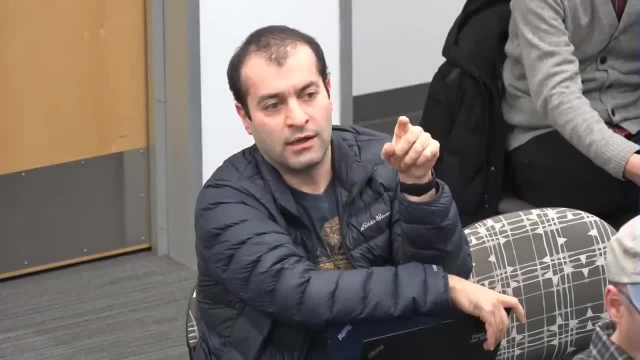 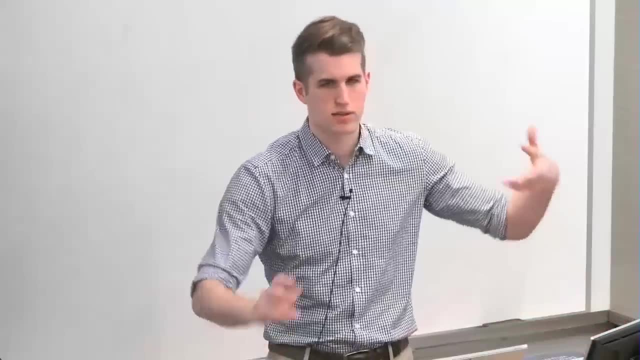 I get why two going out, Yes, But I don't get why the output of zero is also going in. It doesn't seem that you're actually using it to produce any of the outputs. Yeah, Yeah, You're correct, It's just, we need-. 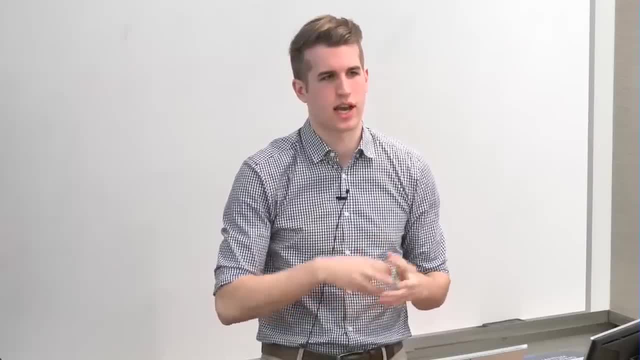 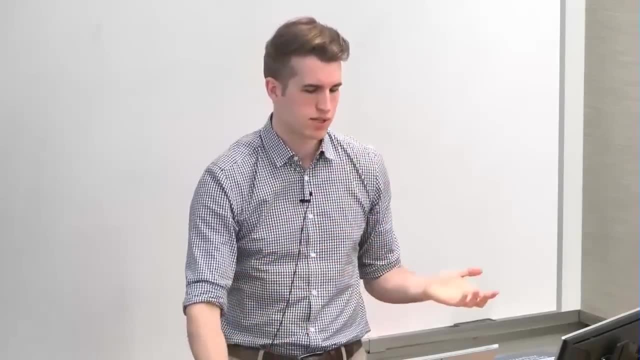 Symmetry, Not really symmetry. It's just like how we write the quantum, how we would write the quantum circuit, We would need two qubits In general, So and we just? you're correct that this output value isn't really used. 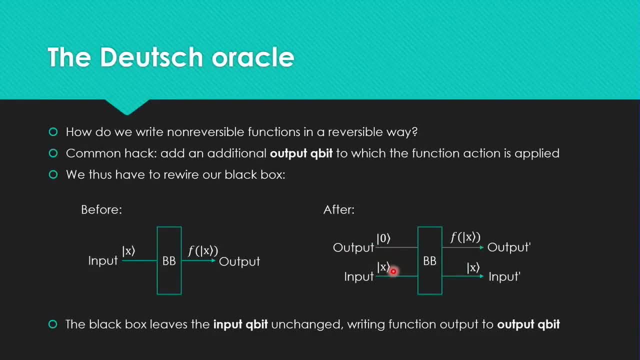 Is it like we don't care? kind of No, we do want it to be zero, Because this, the way that we write the circuit, assumes that this value coming in is always zero. Yes, Why is it called? why is that in going output wire called output? 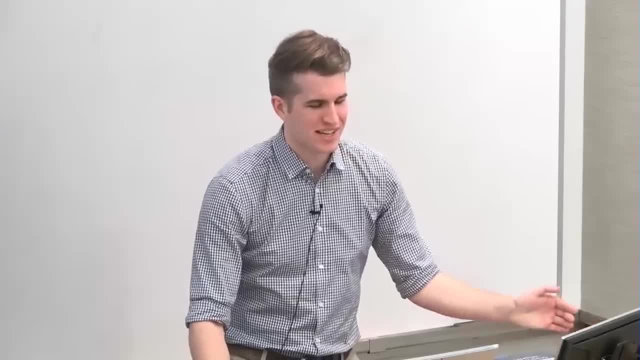 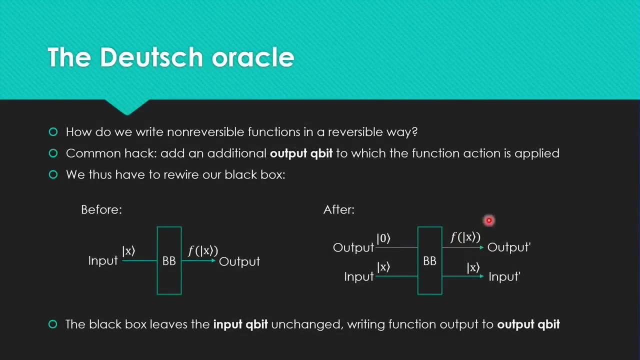 What? Yeah, yeah. So this is kind of weird that, like, the output of the input is called input, But we basically only really look at this value. here is the basic idea. This is like the real output. The input will always be unchanged. 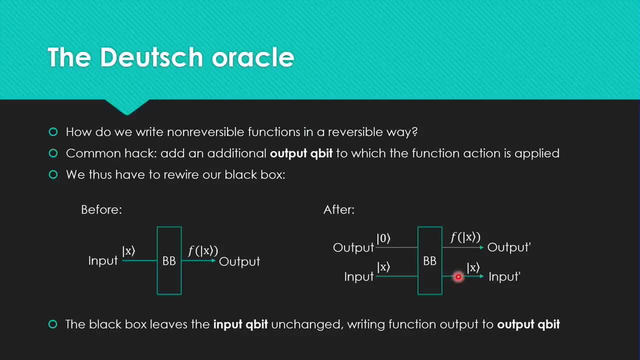 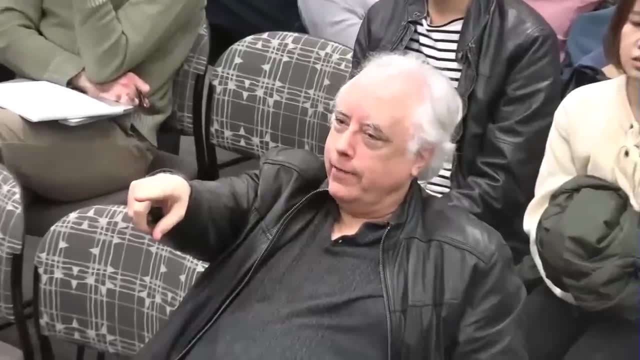 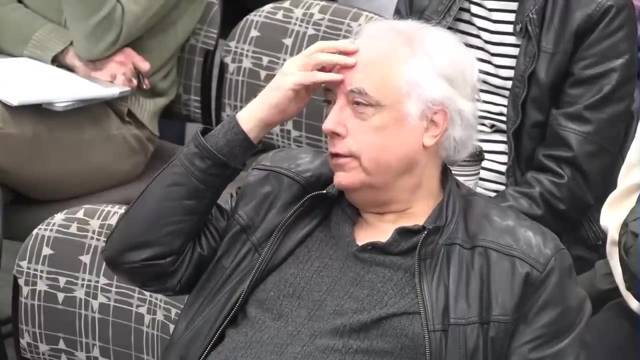 Question: Yes, So if I had multi, two black boxes in series, Yes, The upper input, which you have labeled as output, This one- Yeah, that's a bit weird. And the second stage would be the f of x output of the first stage. 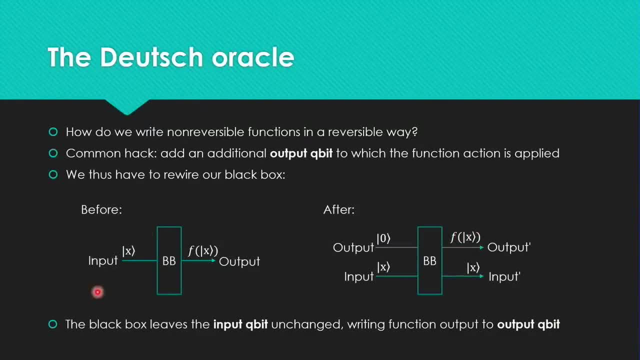 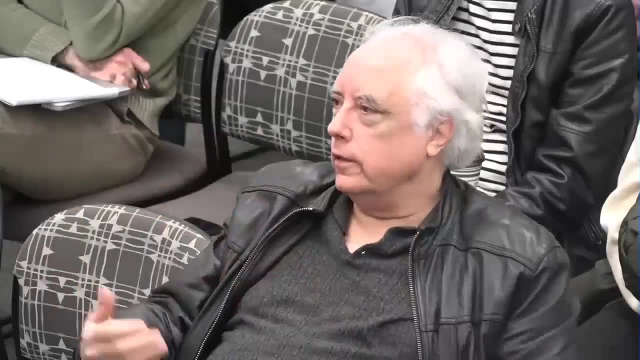 Yes, Well, okay. So you're saying, if you had two, these in series rather than sort of in parallel, what we're doing? Is that what you're saying? Yeah, I want to do two operations, one and then another one. 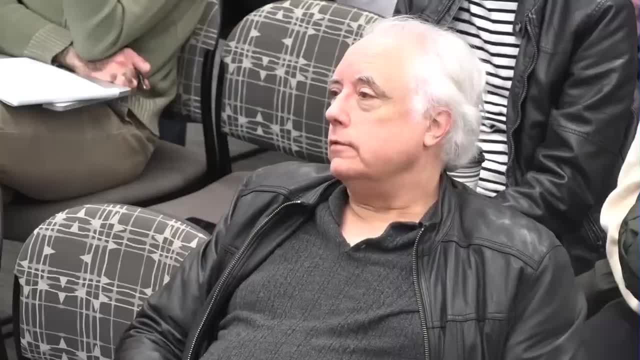 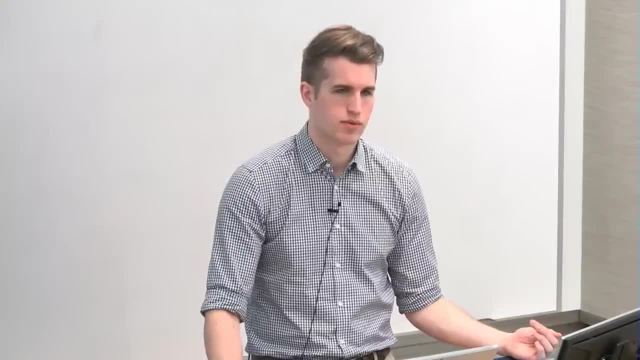 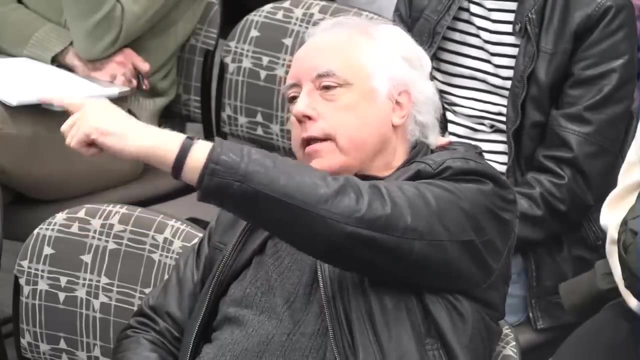 And the black box is doing some operation. The black box is doing some operation. You can have as many operations as you want in here inside this black box. basically True, but I'm trying to conceptually understand whether I would take the f of x output upper right and that would. 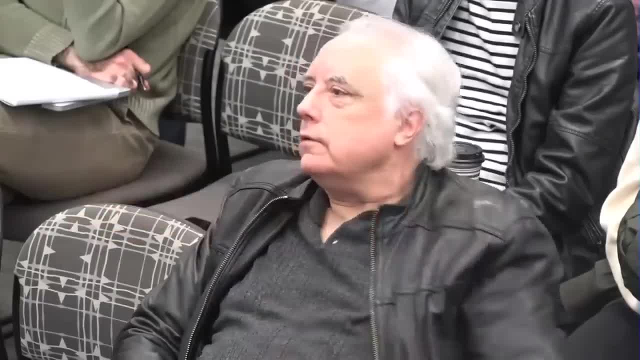 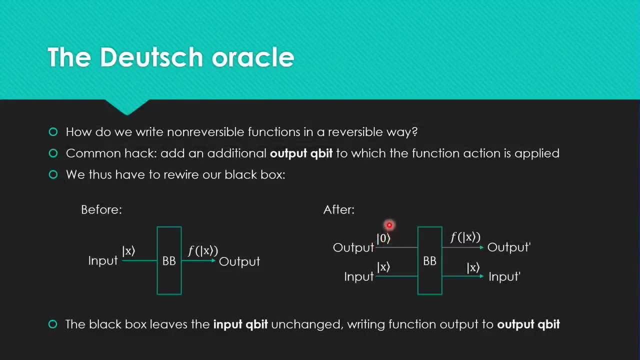 be the output input of the next one, Absolutely, And in fact I said that this black box assumes this value is zero. This is maybe throwing a bit much at you, But actually we can break that assumption and send it some other value which maybe will get us. 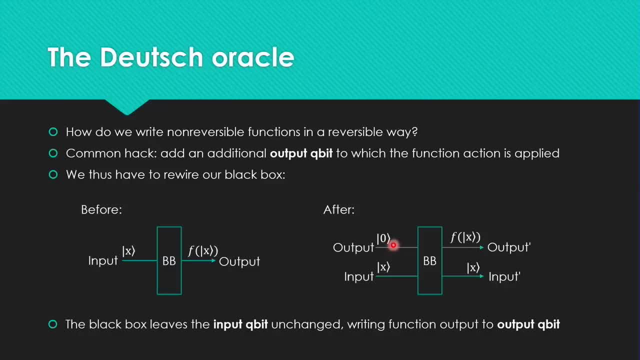 more information, which is in fact what we'll be doing. So the black box. the working of the black box assumes that the output, input, is zero, But we can break that assumption and be tricky. My way of thinking was: I didn't have any other value for. 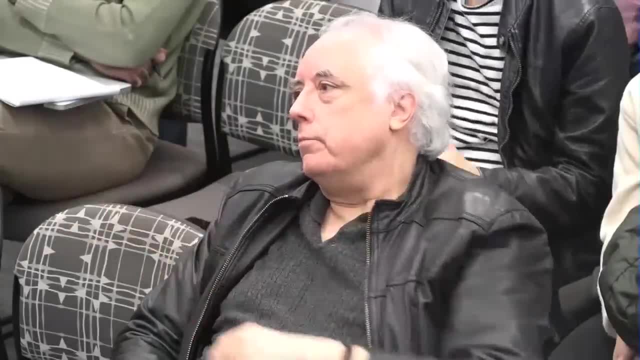 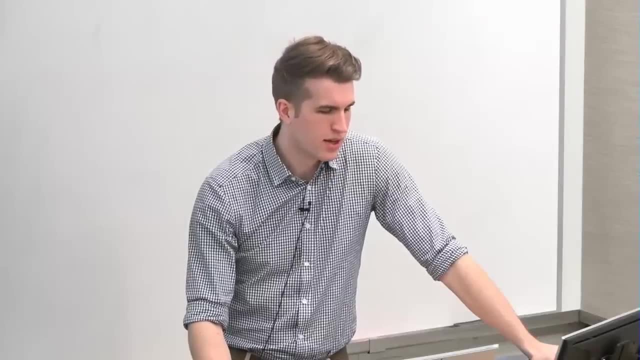 the first stage, but for subsequent Yes Inputs, I do have one, So I could use it if I wanted. Yeah, you could, Yeah, And you might get some interesting values, which you actually will. Okay, I swear, this is. 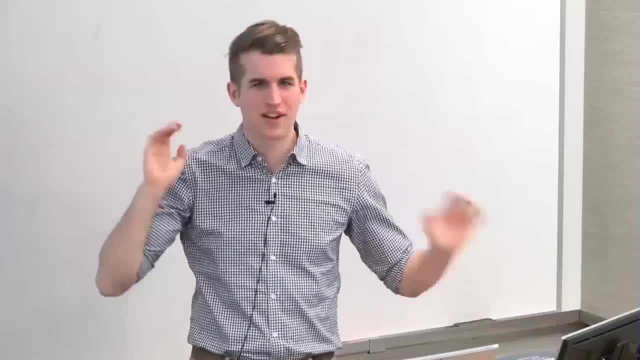 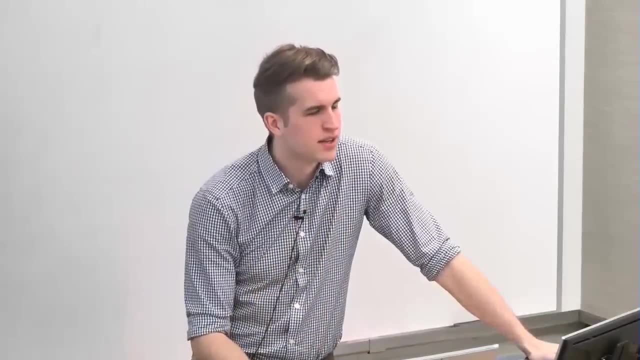 the most difficult part, conceptually, of this entire presentation, So if anyone has any trouble with it, please just let me know. Ask any questions. We can spend as long time on this as we want. Yes, Go ahead. Is there some additional clarifications to this? 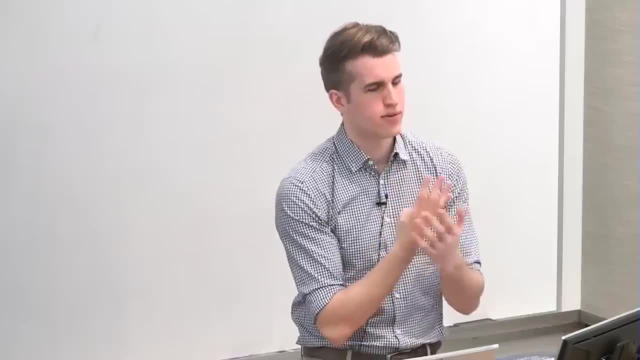 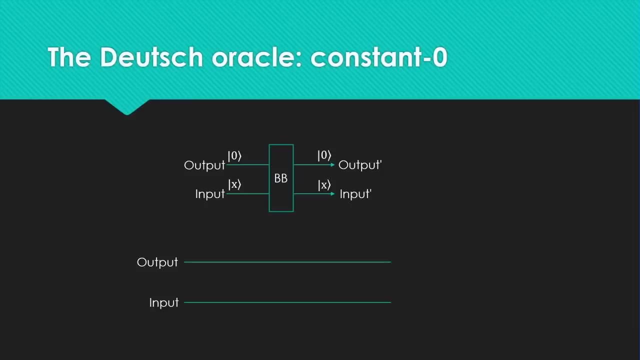 Because I didn't get it. Okay, Well, we'll go over how we'll write each of the four functions in this way, So maybe that will help. Okay, So, for example, constant zero. Here's how it would look. 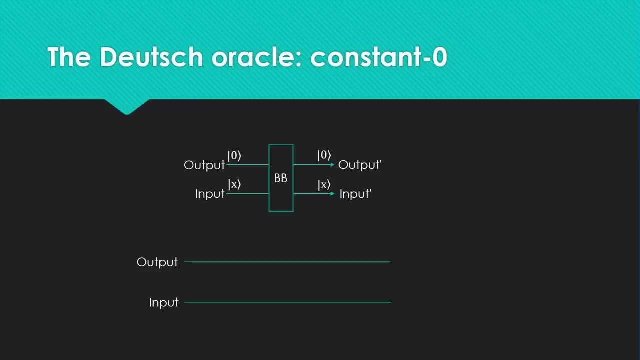 X goes in, X goes out, it's unchanged. Now the output is always going to be zero, right? That's just what the constant zero does, So we always want this value in the upper right to be zero, If we assume zero goes in. 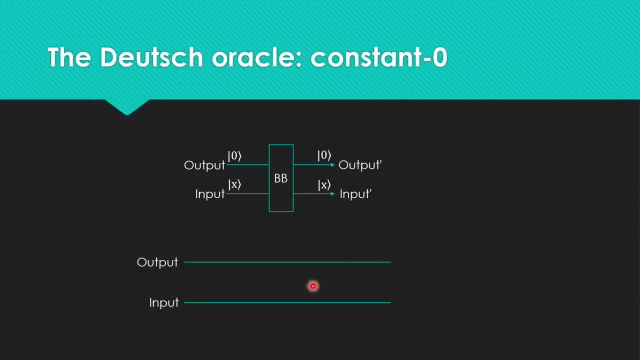 this is our circuit diagram. Neither of the two wires make any modifications, right, They're just, it's a straight wire. Does that sort of make sense? Okay, We'll see The next slide. What about for constant one? We want one to go out here, right? 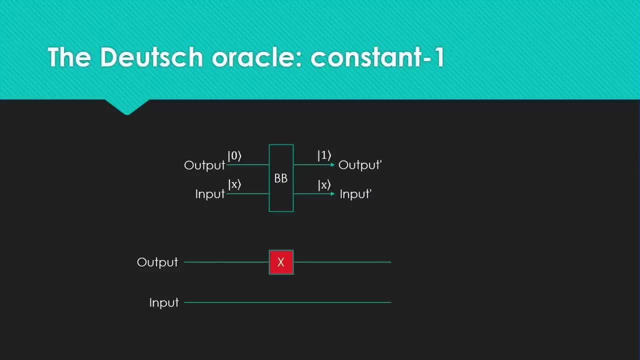 This is our function output value And we assume zero is the input here all we do is we do a bit flip right here And that gets us the semantics we want. Is anyone having any trouble with this so far? I swear this is the most difficult part. 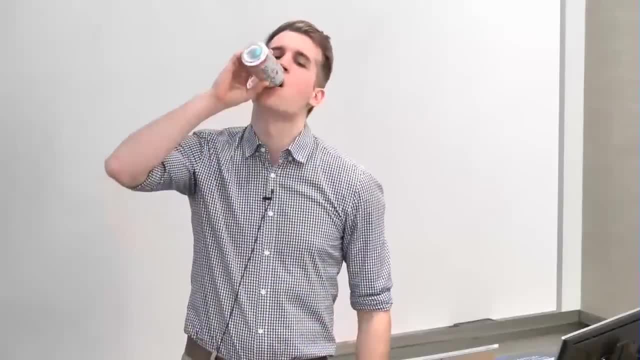 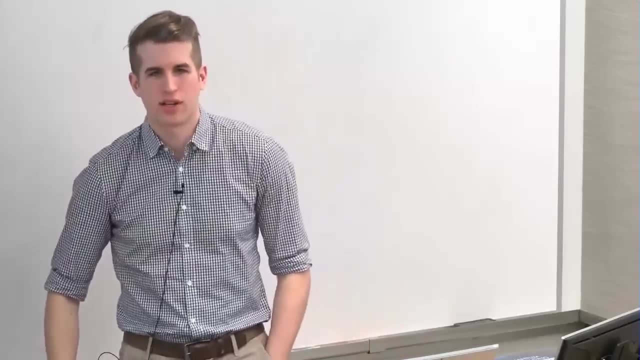 So if you get this, you're golden. Yes, So instead of these labels output and input, could you call them something like computation and spare? Sure, Yeah, you could. You can call like the compute and the spare bit. 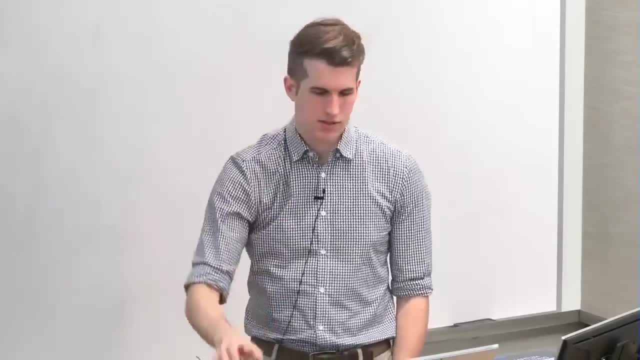 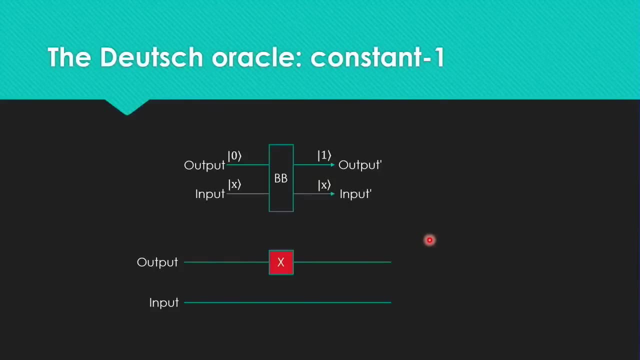 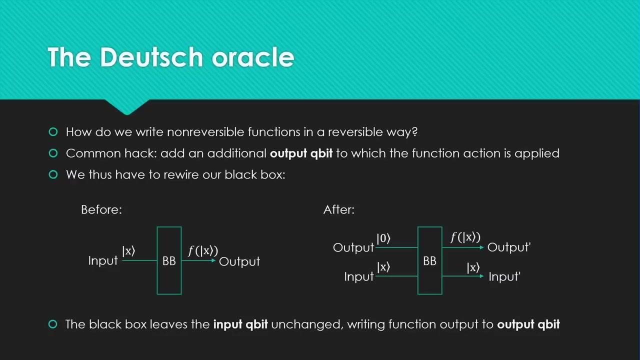 Yeah, that also works. It might reduce some confusion about there being an output-output and input-output. So again, why is it called output? Why is it called output? Because it's we call this the output qubit, because it's just the place that we write the output of the function. 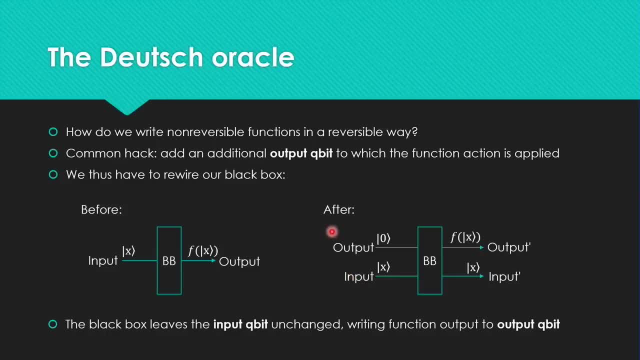 But we could call it like compute and spare or something like that, like he suggested. Like this would be the spare sort of bit that we write the function output to: Yes. So we did this to have a reversal computation right. 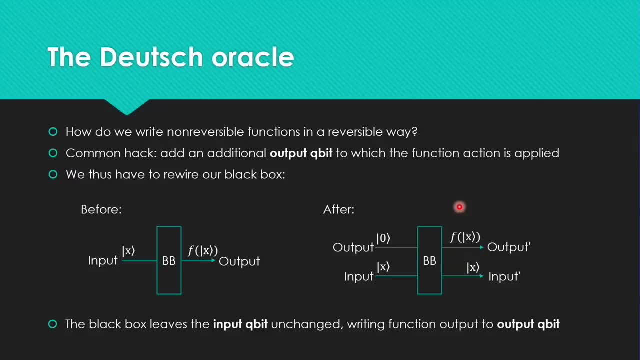 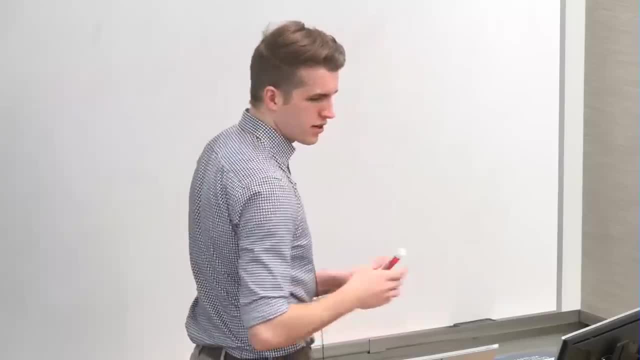 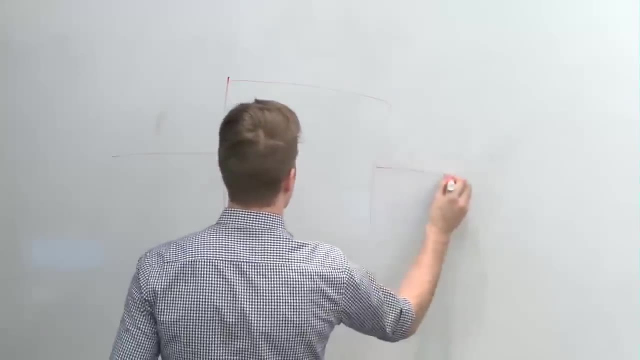 Why is this? Can you compare the reversibility of these two, Like, why is the right one reversible? Absolutely Okay. So let's consider this one right here. right, We have our black box with a single wire And say we want to do the bit flip operator. 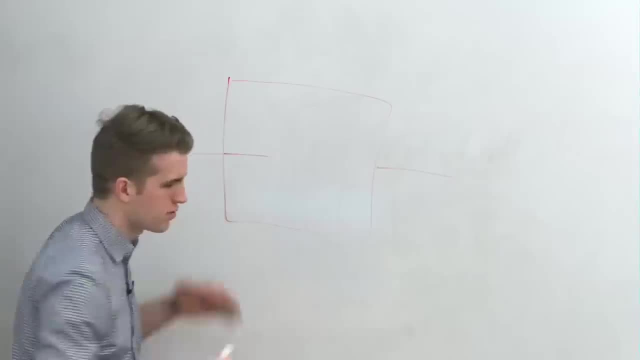 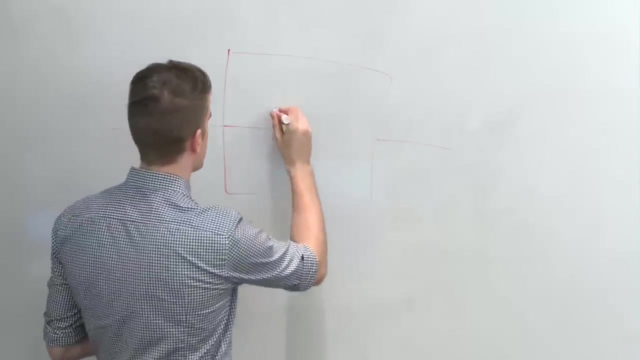 So that would just be sorry, not the bit flip operator. bit flip operator is reversible, So we want to do the constant zero operator. We always want to map this to zero, So you need some operation right here that would map this to zero. 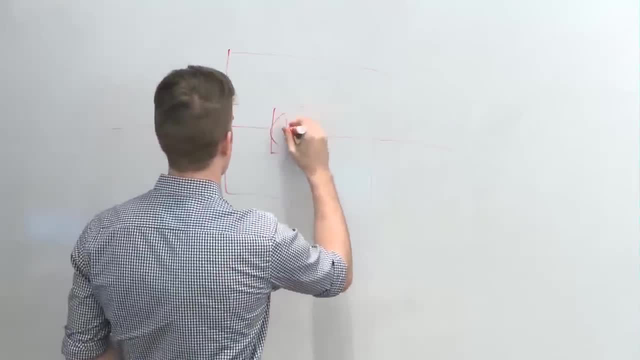 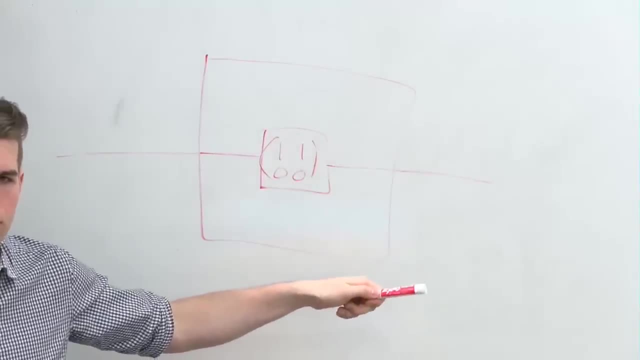 But it'll be the matrix 1100, but this is not a valid operator in a quantum computer because it's not reversible. So does that kind of make sense? It's just we can't construct a device which does this. It's just not permitted by physical reality. 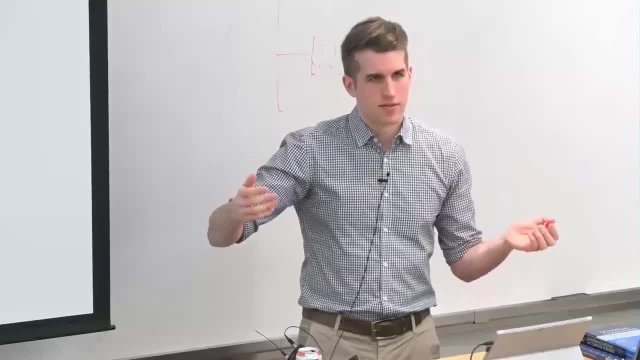 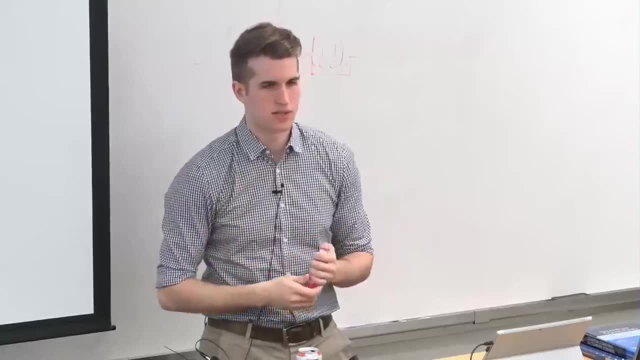 All this math and stuff I'm showing you. it's not like special, it's just we found that it corresponds to the semantics and workings of a quantum system, And so it's a nice way to reason about it. basically, Okay Versus yeah, of course. 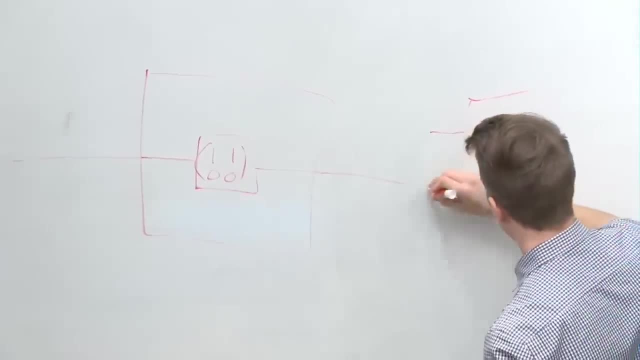 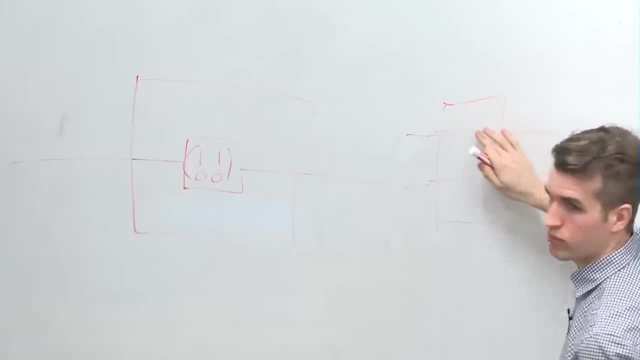 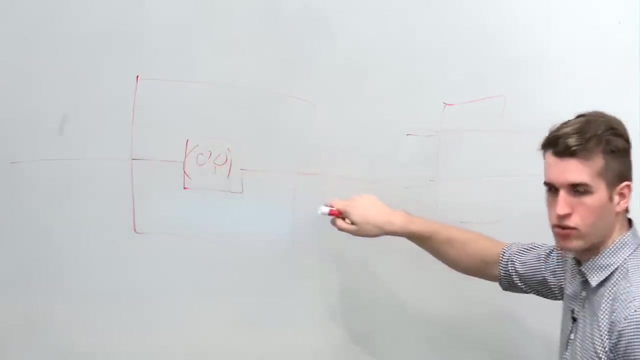 if we want to write constant zero here, with the two input or the two wire model, it would just be blank right. Or if we want to do this, is constant one always maps to one. We saw that this has an x gate here. 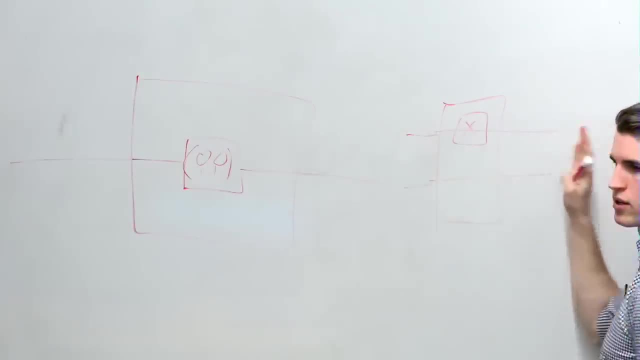 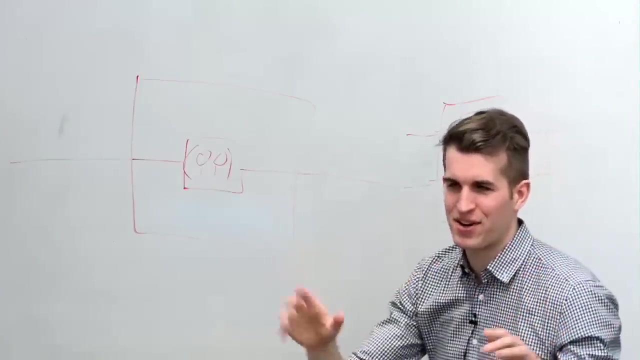 And this is reversible, right? Okay, So we managed to write a non-reversible function in a reversible way. If you got this, congratulations. This is the trickiest part. It took me a while to figure out why we needed to do this. 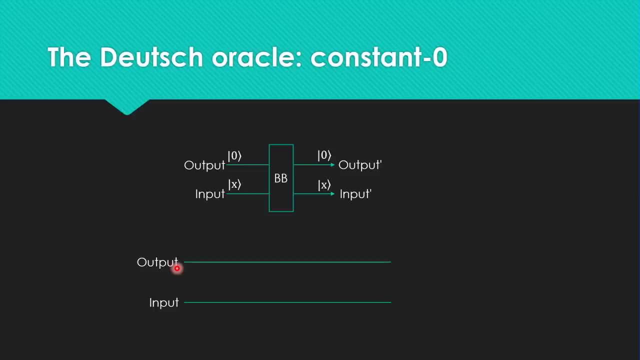 Staring at the textbook. Does anyone have any confusion here? No, Okay, So remember: constant zero is just blank. Constant one has a single x gate. Yes, Is the point that you always end up with a four by four reversible matrix. 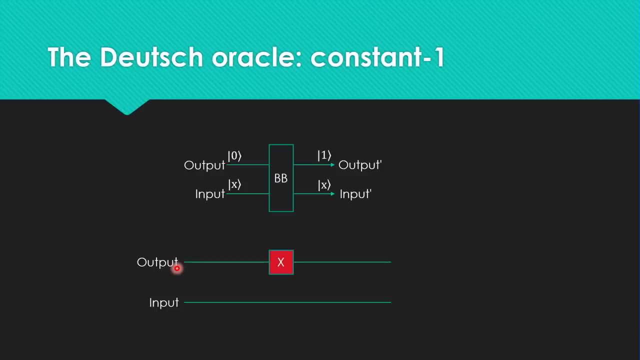 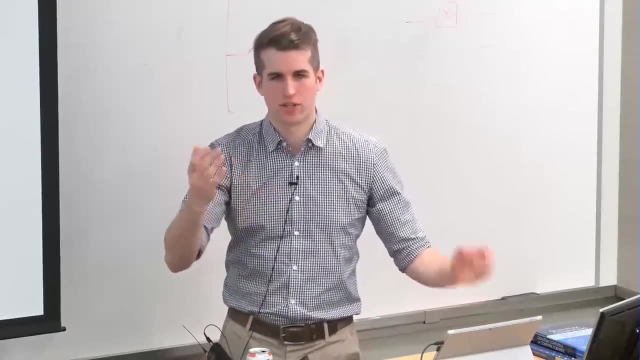 by doing this in black box. Yes, Okay, Yeah, black box is always a four by four reversible matrix applied to a product state. You're correct, Although we will be not going into the math in that way, we'll just be using the state machine to look at it. 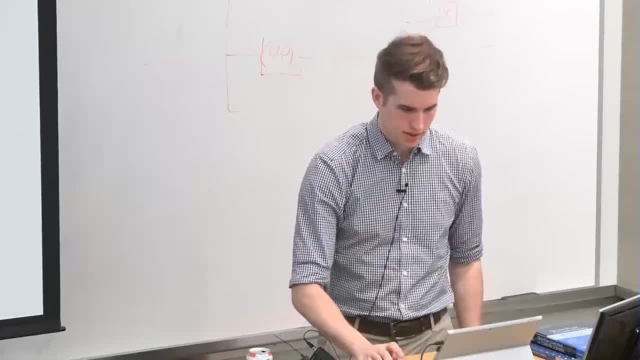 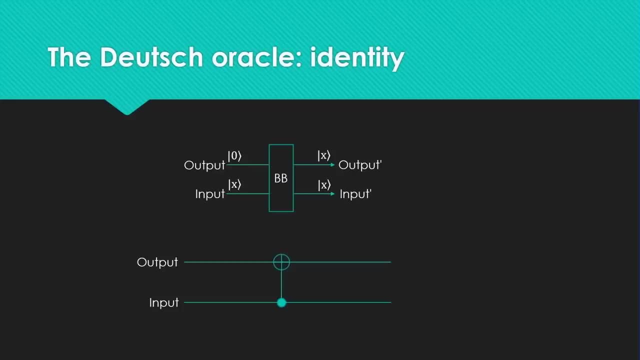 But the math is very easy for you to do it yourself, Okay. So let's let's look at identity. This is a bit more complicated. This is the c? naught gate, okay, Where this is the control and this is the target. 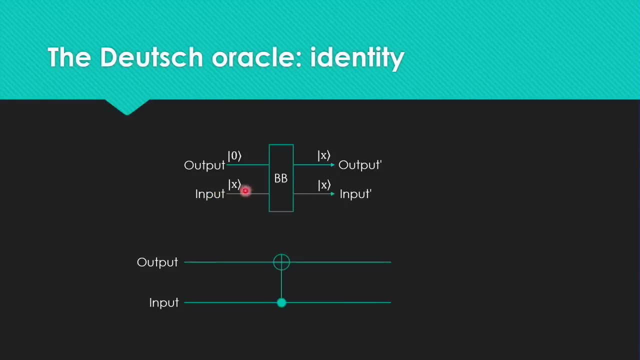 So we'll end up with. so input again is unchanged. We want output. we assume it's zero. We want to end up with the value x, right? So if zero is sent in here, then this is the control bit. 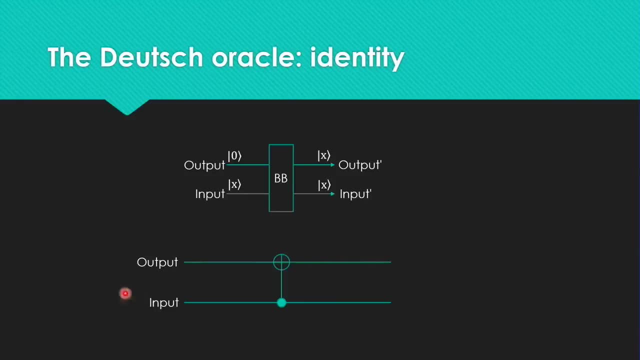 So the target bit is just left, unchanged right. So zero comes out. If one is here, one is sent in, then the control bit's one. So we flip this bit and we end up with one. Does this make sense? 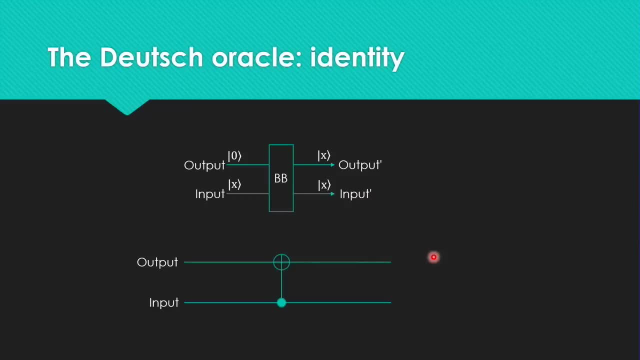 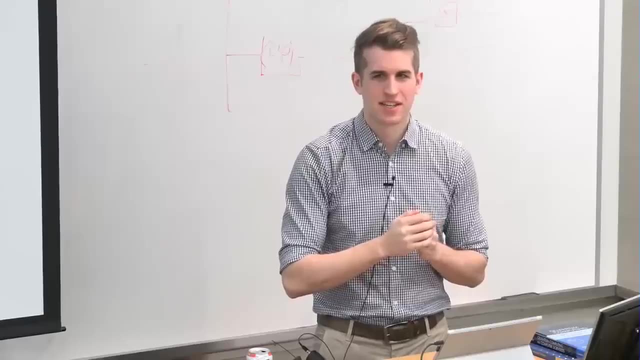 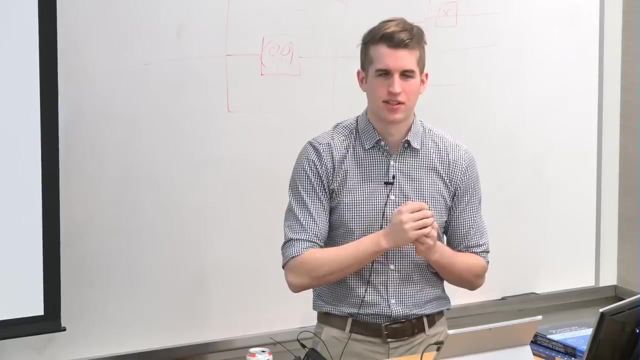 This is kind of tricky. This is a step up in complexity of our circuit, But everyone's fine with this. Wow, okay, Can anyone guess how we'll do negation? You can hard set the control bit to one. How can we hard set the control bit to one? 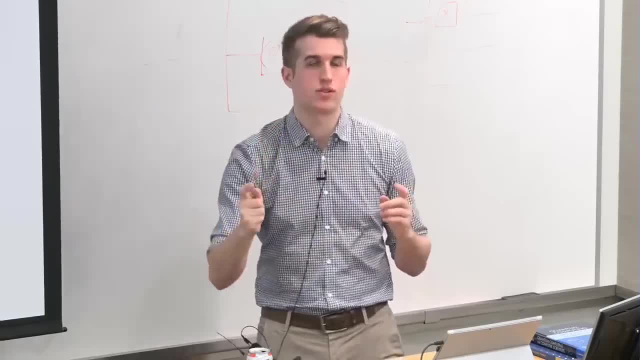 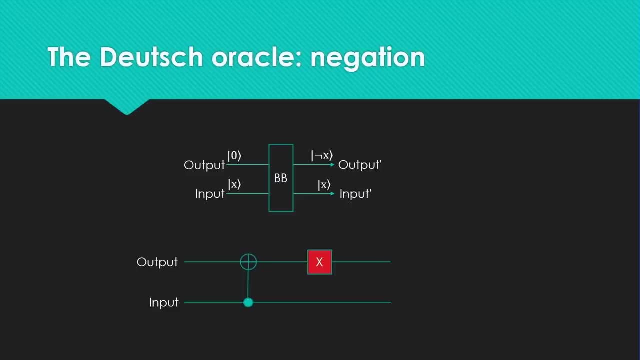 Two control bits, Not two control knots. We just have an x gate there, So up to here it's equivalent to identity right, And then we just flip the output bit and then we get knot x. So those are the four circuit values. 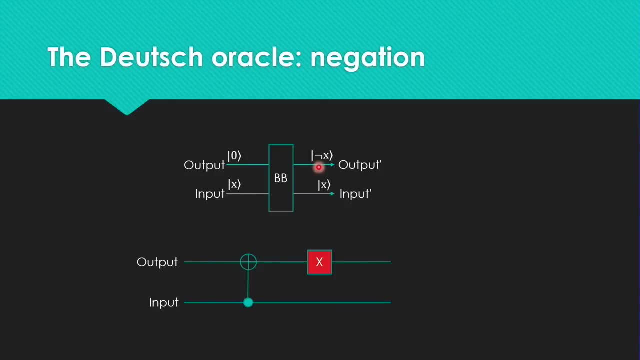 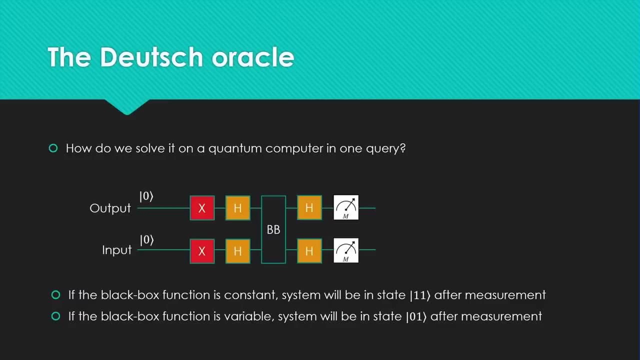 Okay, Everyone's good so far. Everyone knows how we write our four functions. Are you ready to see how we solve it on a quantum computer? We use this, So we're going to break the assumption that this value goes into the black box as zero. 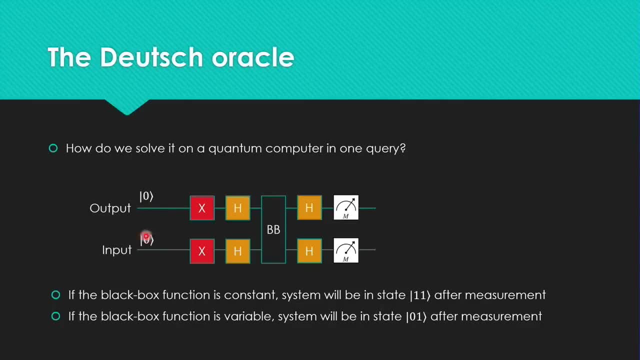 We initialize both input and output qubits to zero. We bit flip them, so now they're both one. We put them through the Hadamard gate to put them into equal superposition. Then we send them into the black box. One of those four circuits is applied. 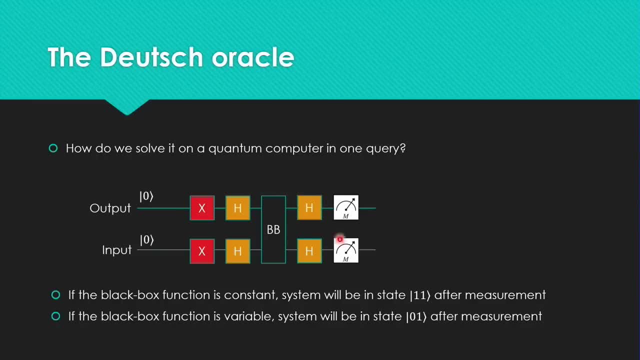 Then we do the post-processing, We send them through the Hadamard gate again and we measure them. This is measurement. I claim, and I will show it to you, that if the black box function is constant, the system will be in state one-one after measurement. 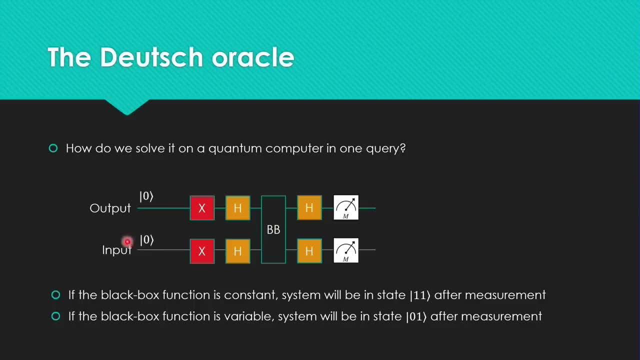 Like. this will have value one. this will have value one. We're using input as the most significant bit. by the way, If the black box function is variable, then the system will be in state zero-one after measurement. So this will be zero. this will be one. 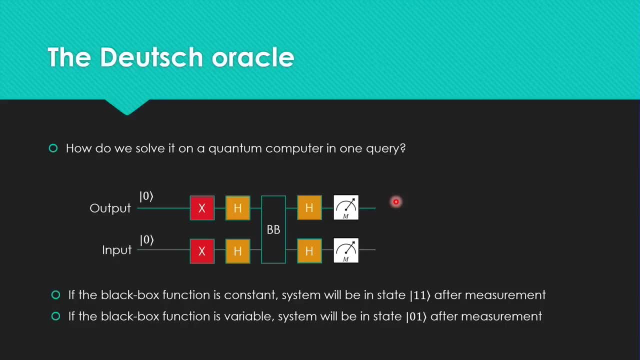 We will know whether the function is constant or variable in a single query. Pretty nifty right. I'm going to show you how it's done. First, the pre-processing. Remember we start with zero, then we bit flip both, then Hadamard gate, both. 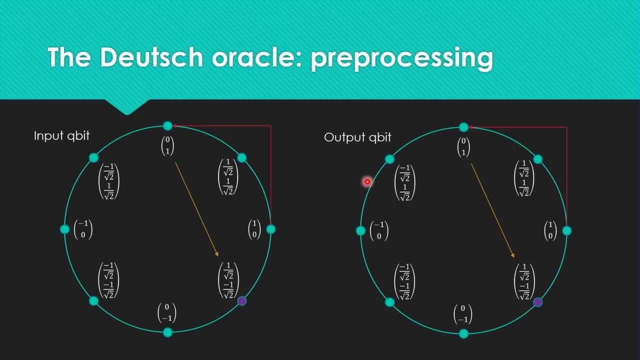 So we start here. bit flip takes us up to here, Hadamard gate down here. So this is the value that is sent into the black box. Just remember it's in the bottom right on the unit circle. This is the value right before we send it. 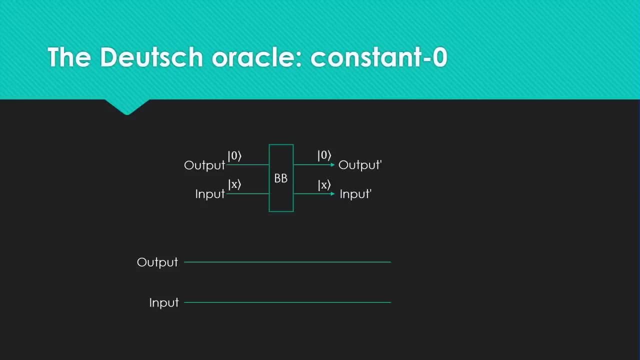 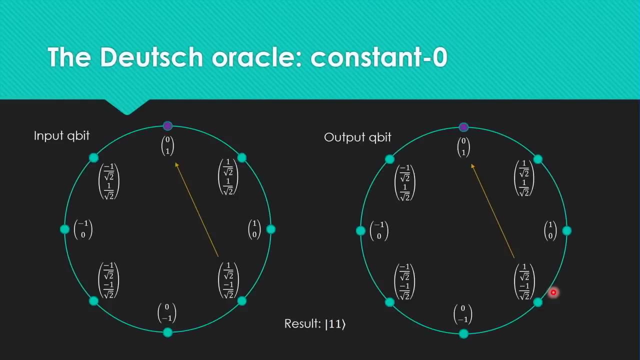 through one of those four circuits. Okay, Now let's look at how we do constant zero. So constant zero, remember, it's just blank on both. and the post-processing is a single Hadamard gate. So since no gates are applied, 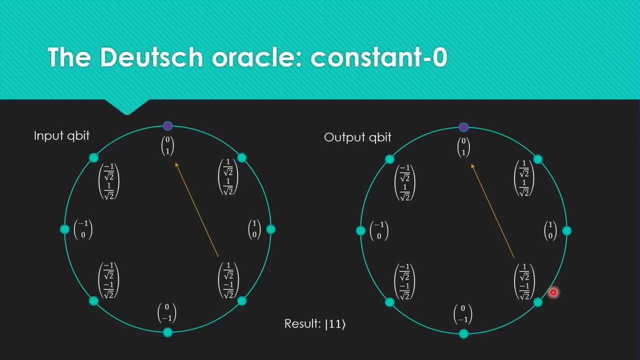 they stay in this bottom right value and since the Hadamard gate is applied as part of the post-processing, we flip back up here When we measure this. this is one-one. Remember I said the value would be one-one if it were a constant function. 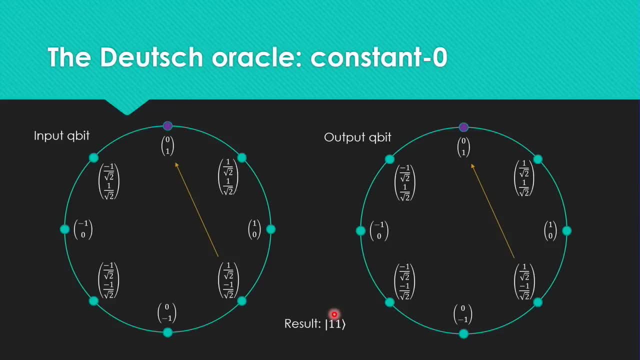 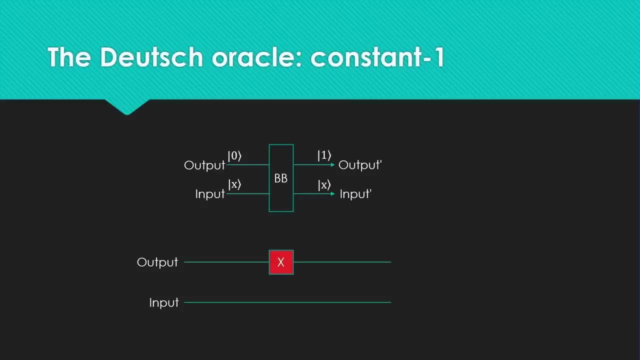 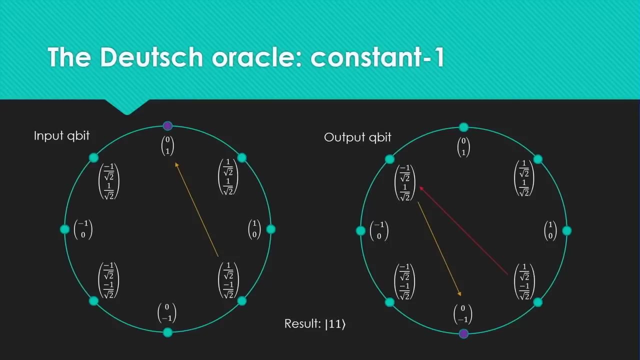 So we're one for one. Okay, Seem. okay. so far, All right. Let's add a bit flip, because we're going to go over constant one now. So this is the other constant function. Now, remember, if we do a bit flip in this state. 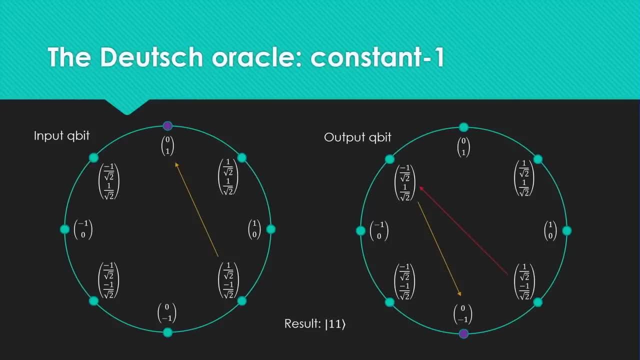 we flip across the unit circle over here and the Hadamard gate then takes us down to here. zero and negative one. When we measure it, we again get one-one. Okay, So we're two for two. Not bad right. 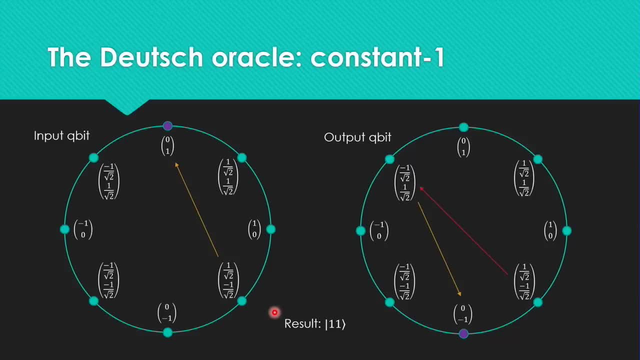 Okay, Things get a bit more complicated. Does anyone have any trouble with this? so far, Any of these? yes, I just didn't get like why it's results is one-one, Why it works out to one-one. Yes, Well, that's a good question, Okay. 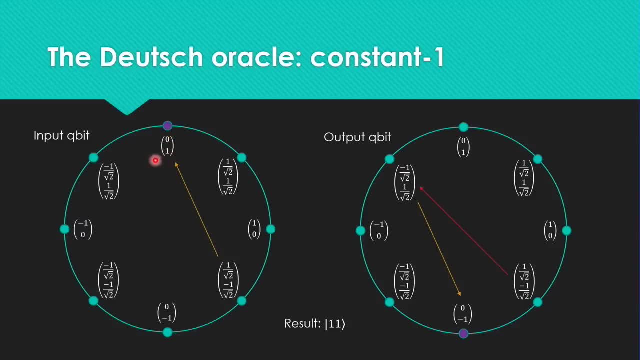 So we're up here, right? Yes, If we measure this, then what value do we get? This is just one. Remember: this is the value of the one bit. Yes, So if you measure one, we get one. 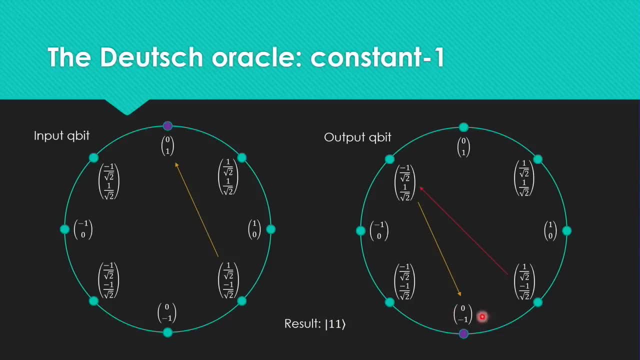 Yes, Now down here, if we measure this, we also get one, because negative one squared is one, So it's a 100% probability of collapsing to one, And so we can say this is one-one. This is like the most significant bit. 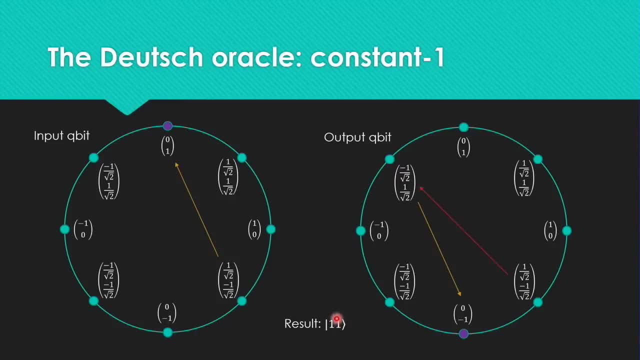 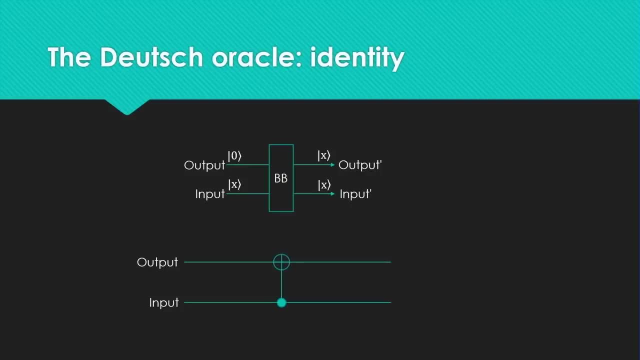 and this is the least significant bit. So we end up with one-one. Does that answer your question? Yes, Okay, Great, All right, Let's go on to something more complicated, which is C-naught. This is going to get a bit weird. 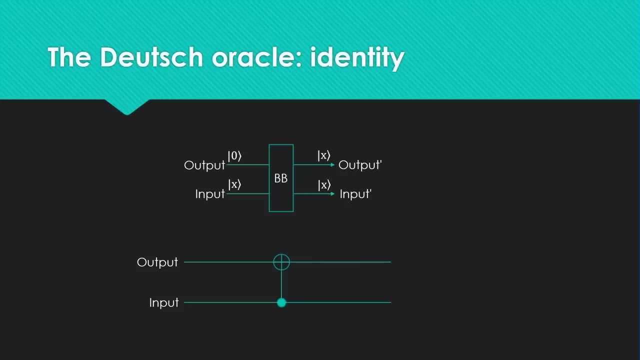 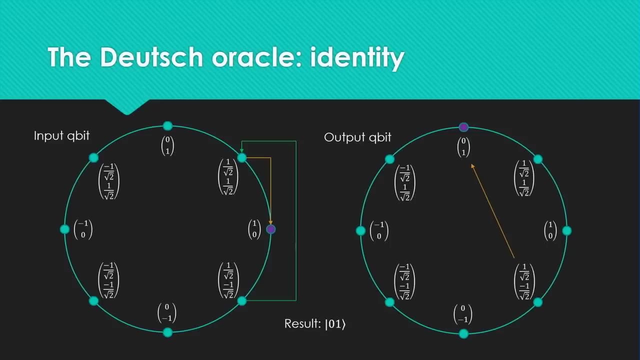 But this is how we do identity. remember: The input bit is the control bit, the output bit is the target bit. And don't panic, I'm going to show you why this is on the next slide. But the action of C-naught is to take. 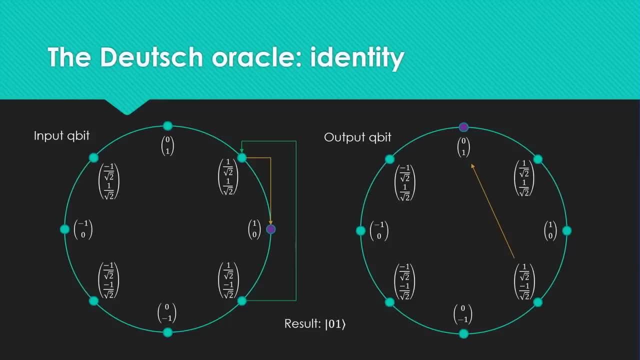 our input qubit up to here It's the green line. This is weird for two reasons. One is that the C-naught is supposed to leave the control bit unchanged, right, But here this is the only thing: the control bit. 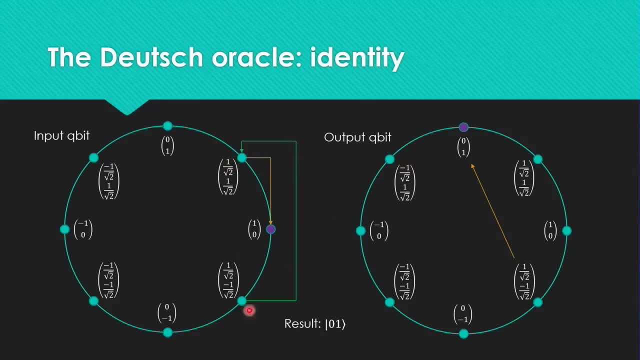 like, the control bit is the only thing that's changed, And this sort of action is a bit odd, But don't worry, I'm going to show you the math, the reason why this works, on the next slide, But just for now. so we flip from here up to here. 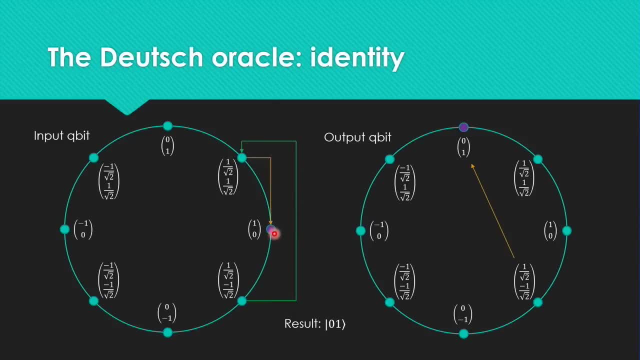 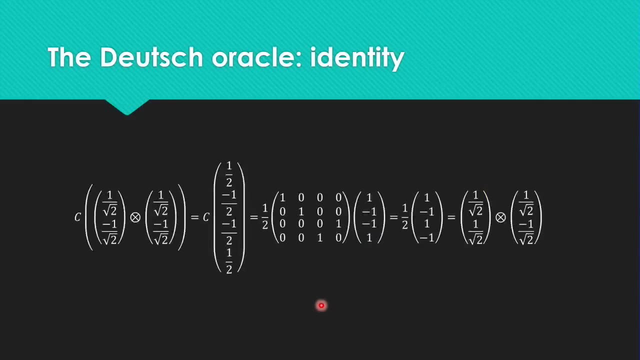 and then when we do the Hadamard gate to post-process, we end up in state zero, So zero one. Pretty neat. Okay, Here's how the math works. We are applying the C-naught gate to the state one over root two. 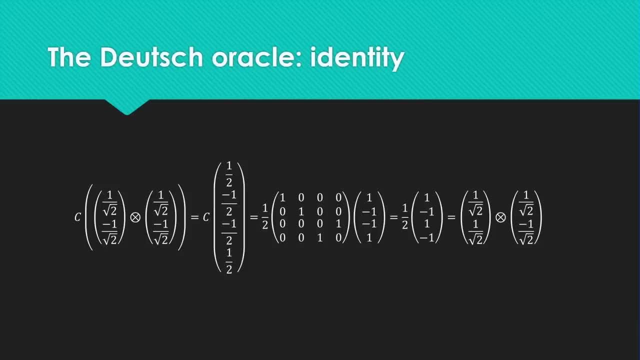 negative, one over root two and one over two, negative one over root two. right, When we tensor these together, we get this ridiculous matrix which I'm going to factor out one half, just to make it readable. So we get this ridiculous matrix, which I'm going to factor out one half, just to make it readable. 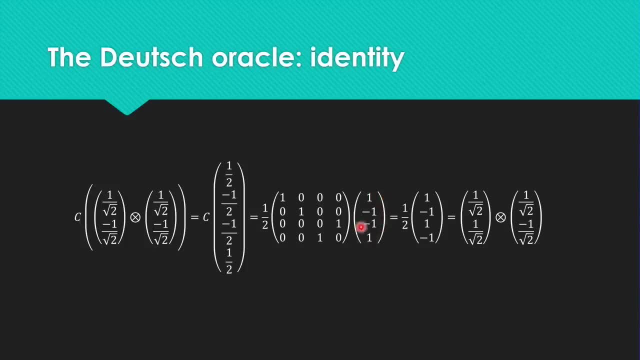 So we have the specter is one, negative one, negative one, one. right Now. we remember this familiar matrix from the C-naught slide. When we apply this matrix to this vector, we get this right: We flip the bottom two rows. 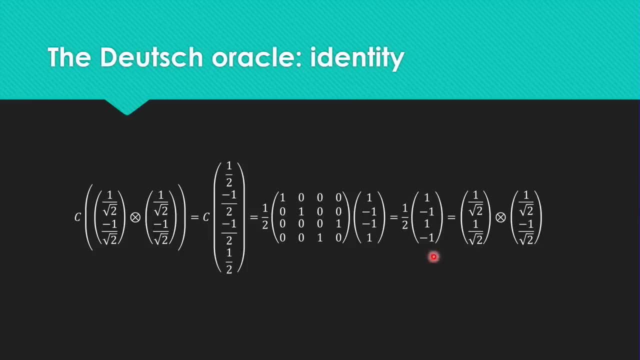 Now, when we factor this- remember this is the product state and we can factor it into the individual state- we get this tensor product. If you ignore everything in the middle and just compare our start values to our end values, this is the output, or least significant bit. 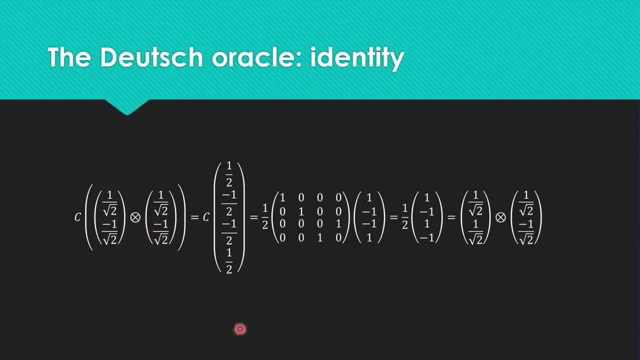 This is unchanged right. This is still one over two, negative one over two. The input bit, which we started out as one over two, negative one over two, ends up is one over two, one over root two. This is just the action of the gate. 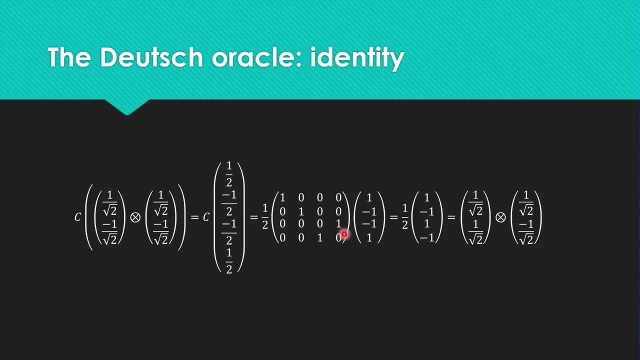 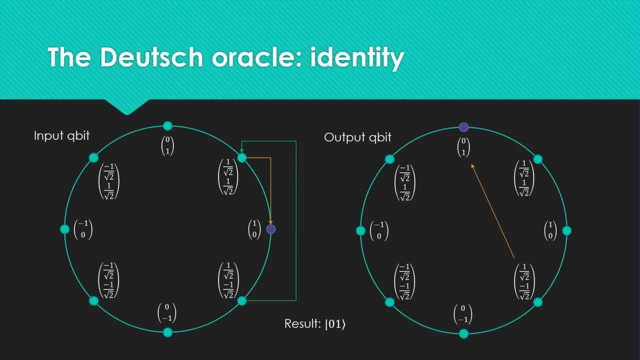 So this is kind of a limitation of our visualizer that we can't really show the state transition, But I hope I've convinced you that this arrow is in fact what happens. Does anyone have any questions about this? Okay, So we're three for three, right? 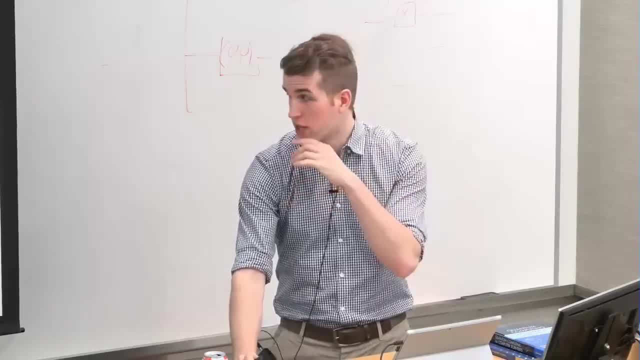 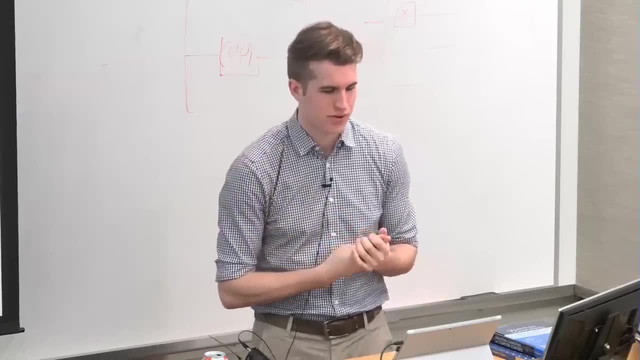 I said, the value, the output value would be, or the measure value would be zero one if it were a variable function. and indeed it is as I said. So for three, three, Three for three, Let's go over the very last one. 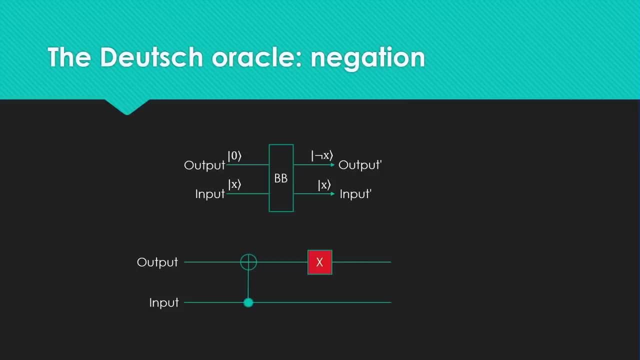 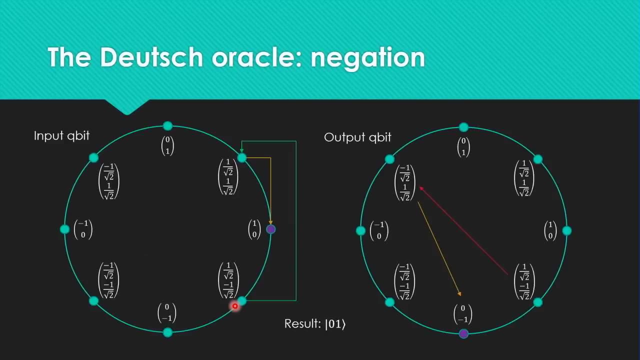 which is negation, It's a C naught, and then a bit flip. right, Let's see how that works. Again, we have this arrow taking us up to here and the bit flip takes us across the unit circle and we do the Hadamard. post-processing. 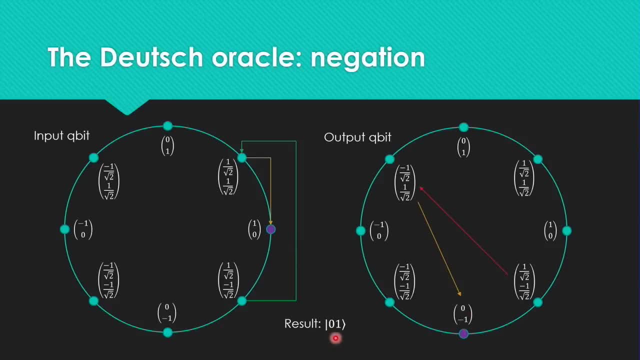 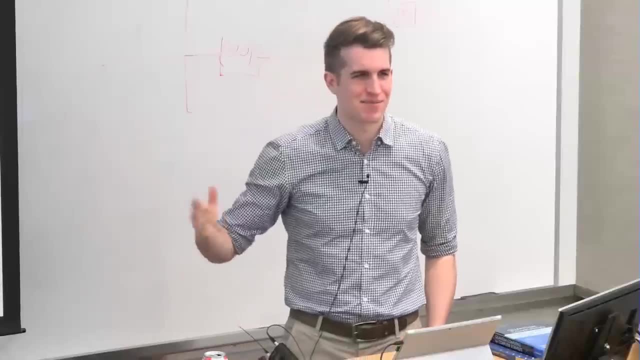 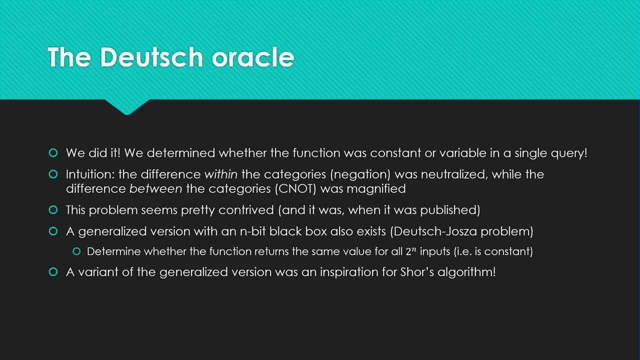 to get us down to here. When we measure these, we get zero, one. Four for four. Single query: outperformed classical computation. Pretty nuts, right, Pretty nuts, Okay. So we did it. We now we have outperformed classical computing. 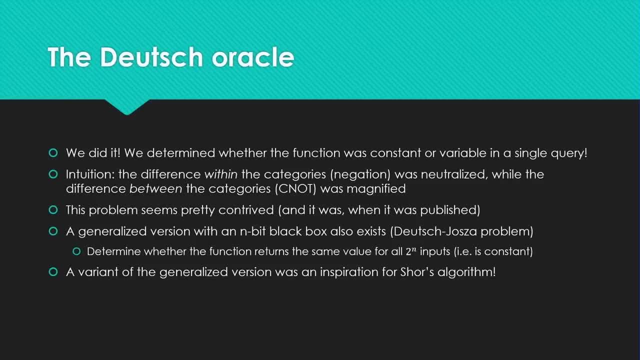 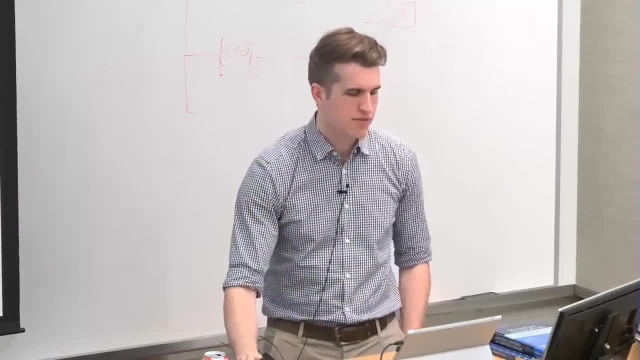 Classical computing is in the dust, It's done, It's dead. So you might think like, yeah, I see how the math works, but what's the intuition? I'm going to tell you the intuition. The intuition is the difference. 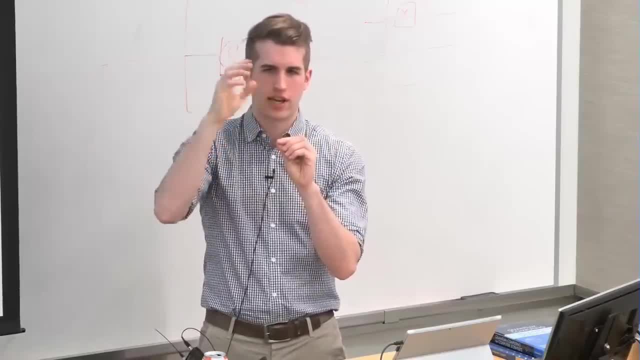 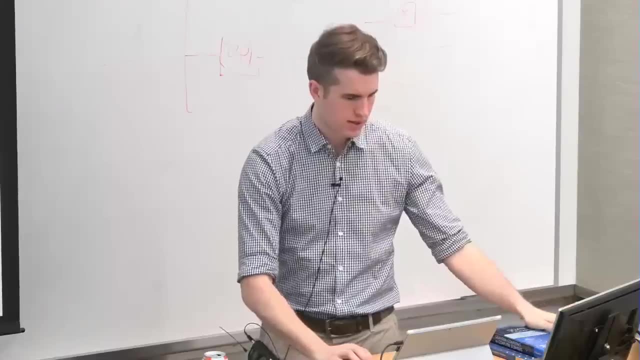 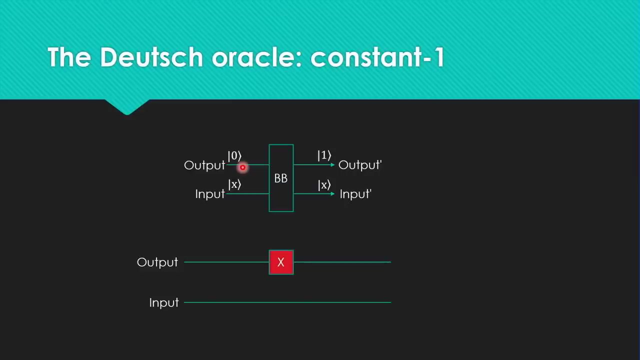 between the cab- within the categories was a single negation gate right. So if we go back to here, So we have constant zero and constant one. The only difference between them is a single negation gate. When you apply a negation gate in a superposed state. 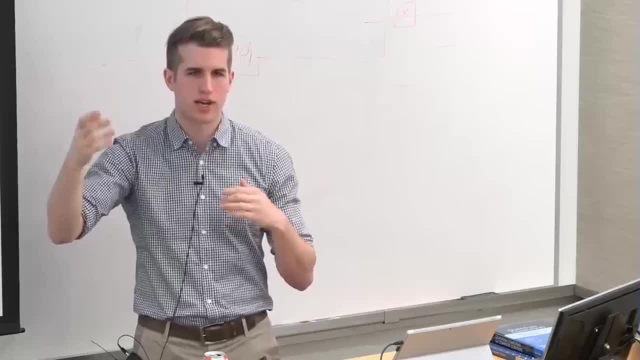 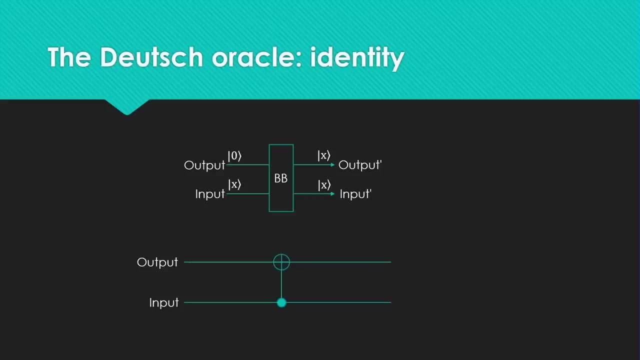 it's kind of it doesn't really have any effect, right? So we kind of neutralize the effect of the negation gate, So we neutralize the difference within the categories and then we magnify the difference between the categories. 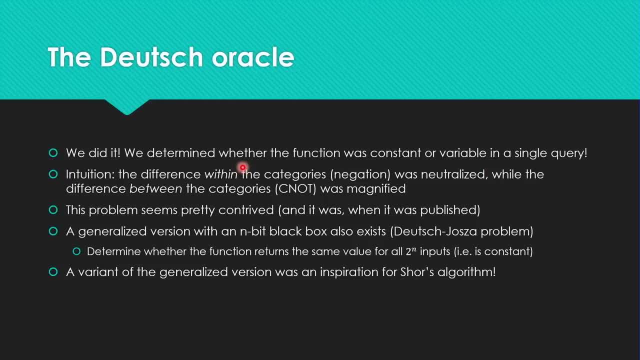 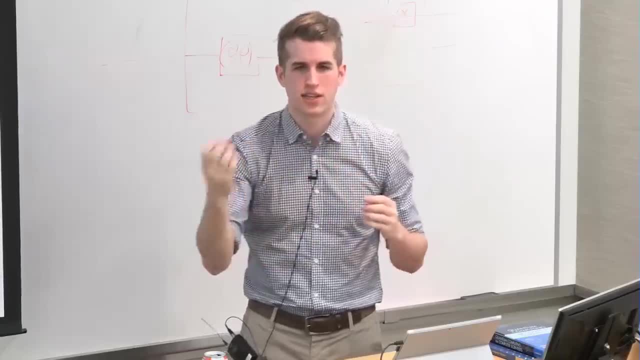 which is that the variable functions of a c naught and the constant functions do not. So we magnify the effect of the c naught and minimize the effect of the negation. And that's the neat thing about, that's a powerful thing about quantum computing. 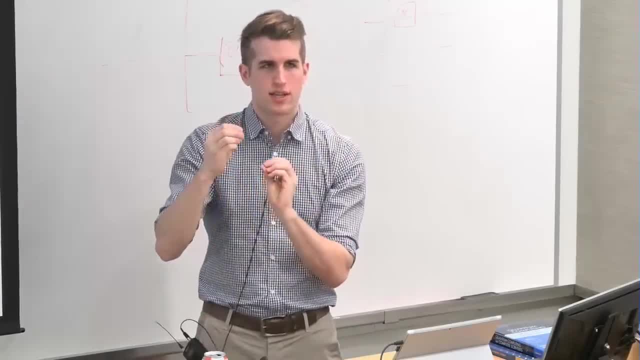 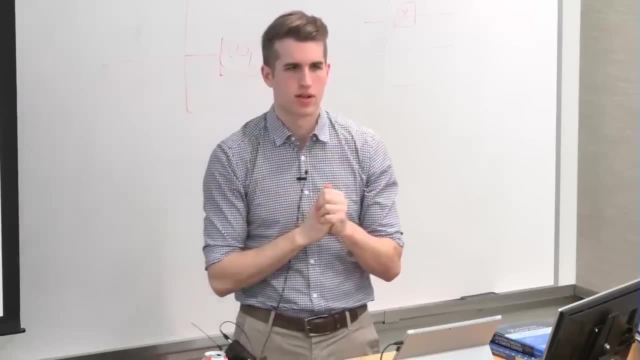 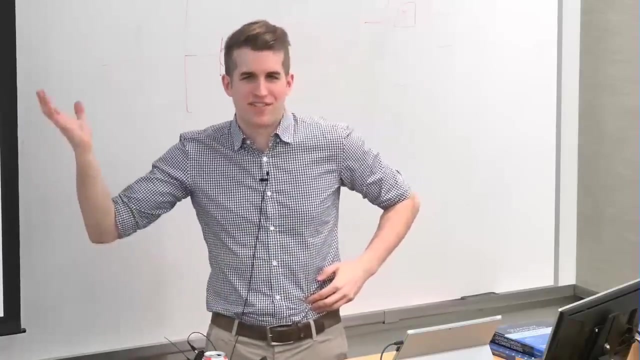 which is that you can change the action of various logic gates by putting yourself in superposition in different sort of states and stuff. So that's pretty neat. And this problem. you may say like okay, well, yeah, great, Whatever, It's really contrived. When do I ever do this in real life? That's a good question, And it was contrived back when it was announced, I think it was 1993.. But then a generalized version of this function was found, which it takes n bits as input, not a single bit. 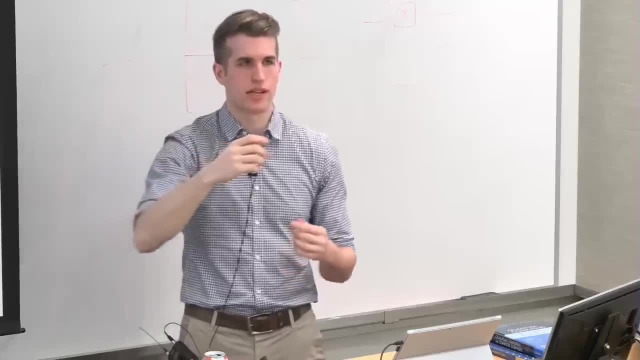 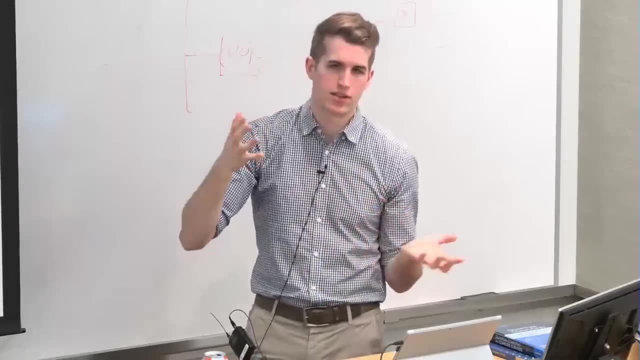 And the n bits either all map to the same value- sorry, like that's two to the n possible values. They all map to the same value, or they equally map to zero or one. They're constant or balanced. It's constant. 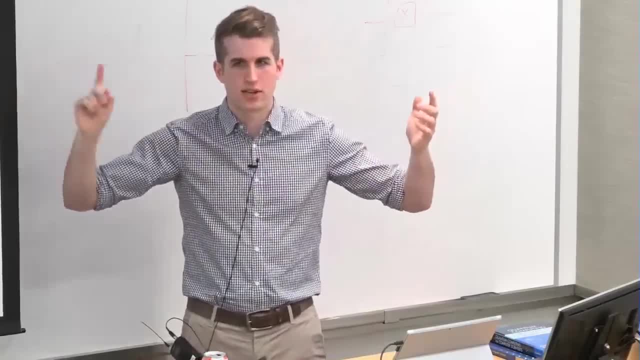 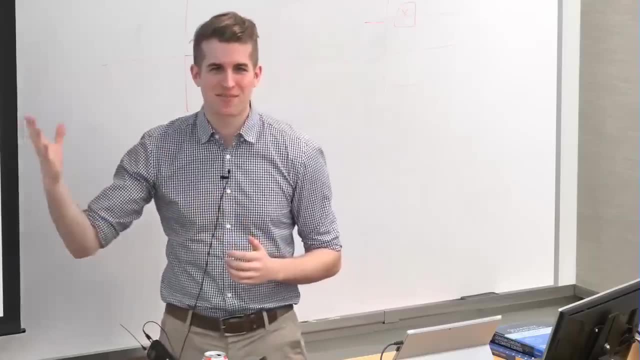 It's called. So it's a kind of just generalized version of this. It turns out we can still solve that on a single query- Exponential speed-up. Exponential speed-up- A single query versus on a classical computer. you have to try all two to the n values, right? 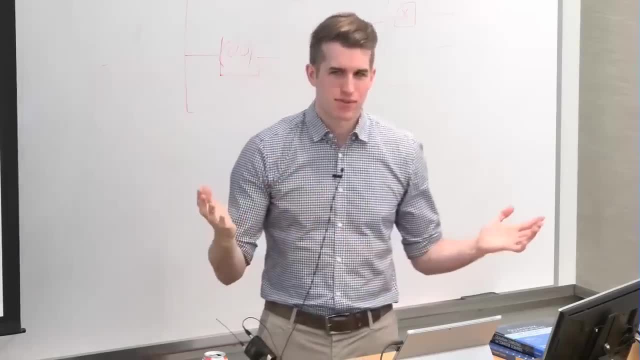 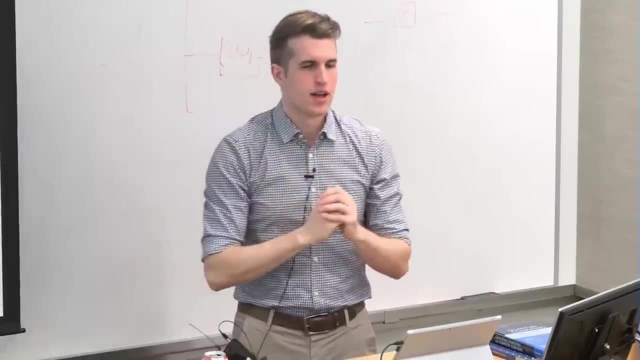 Before you know whether it's constant or variable. Pretty nuts, Okay. And then there's a variant of that problem building and everyone's kind of like building on top of each other. It's called Simon's periodicity problem. It's again, you have like a black box and you're 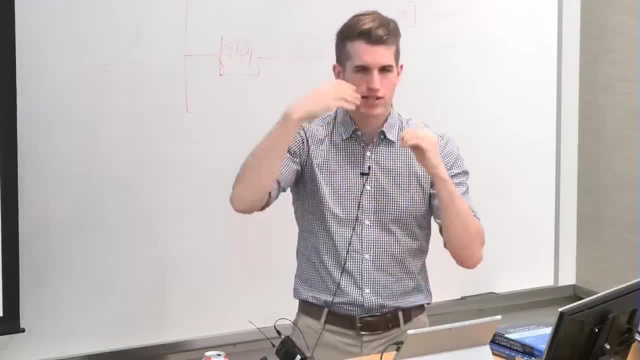 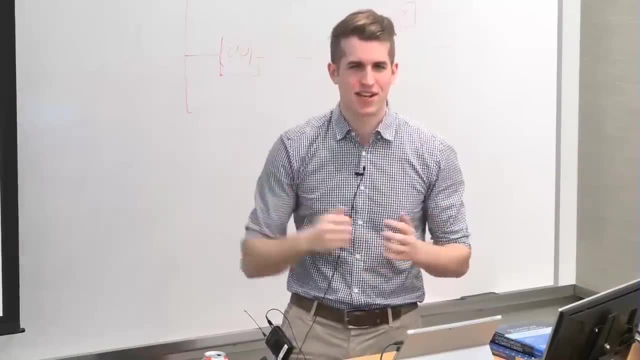 trying to figure out some properties of the function. And then, once that came around, Shor, he looked at this and he's like, oh, we can use this to factor large integers. And so he came up with Shor's algorithm. 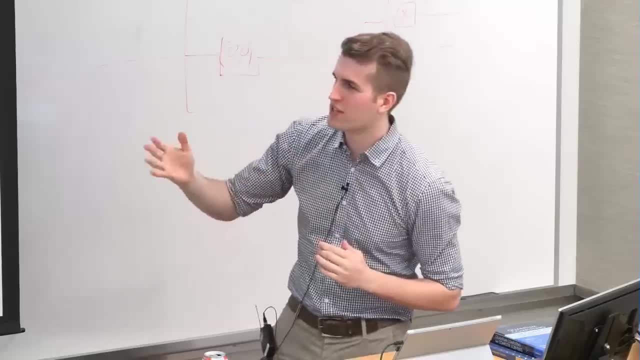 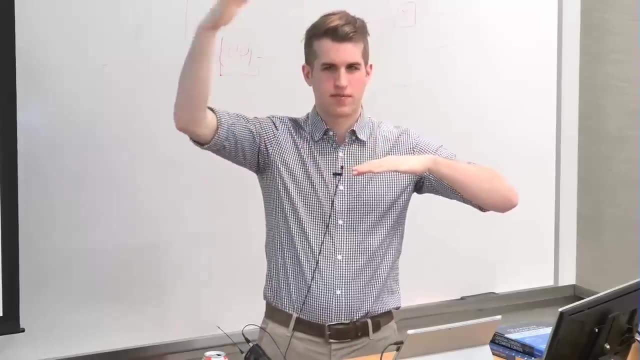 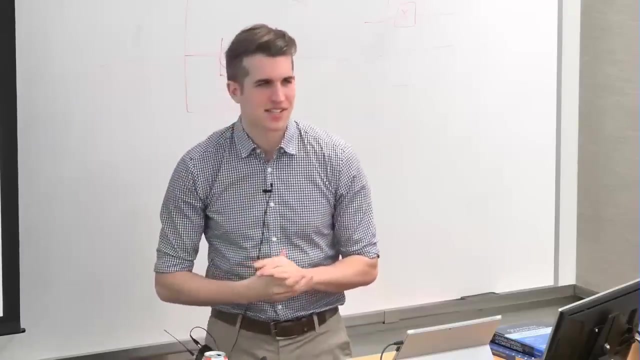 And that's when, like, the whole field really caught fire. So I hope I've convinced you that while this individual problem is kind of contrived and not that useful, it's the base, like the foundation, of some very interesting computational properties. Does that make sense? Anyone have any questions? 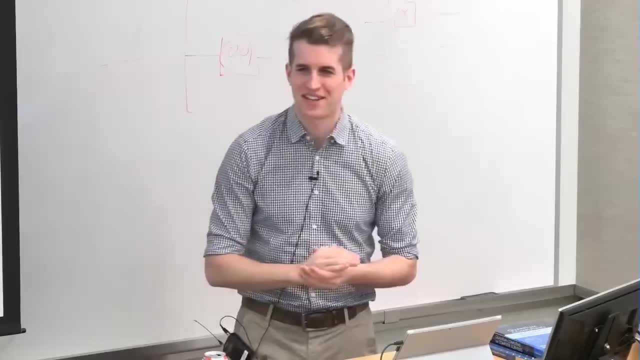 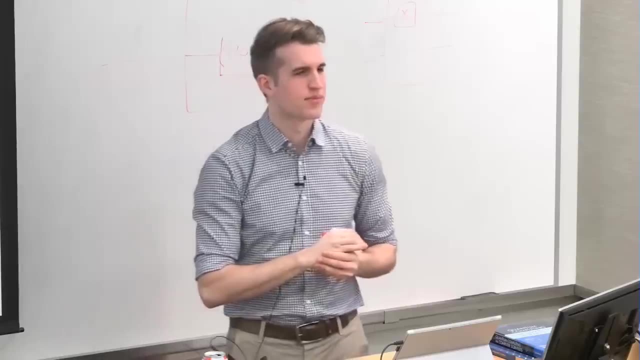 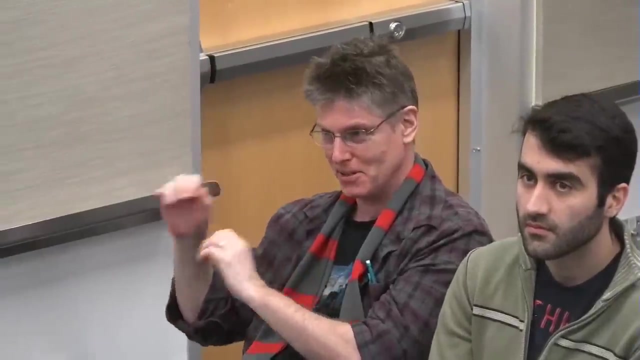 You're all like convinced that we just crushed a classical computer right here. Yes, On the Microsoft site there's an article where the guy was saying that with quantum computers you can take programs that take billions of years to run and run them in a week. 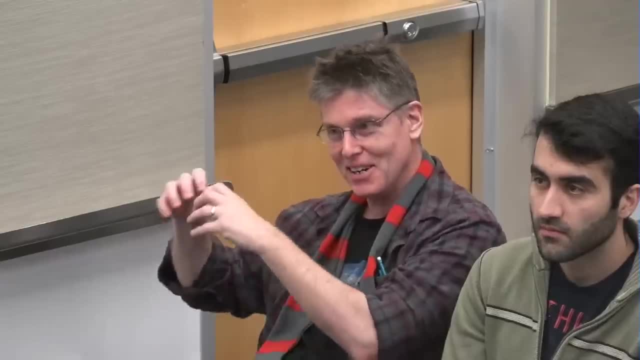 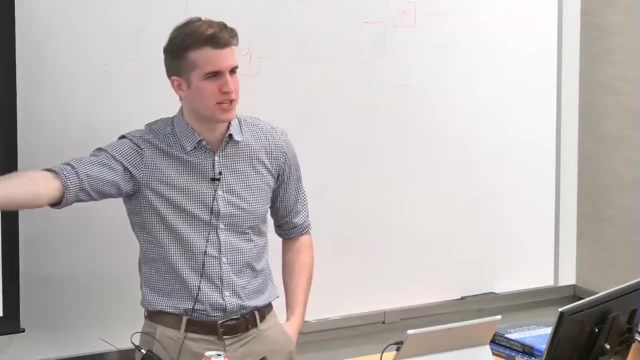 Is this- This could be that. I mean, yeah, You have an exponential speedup Hardware or- If you have, like I don't know what, would take something like a billion years to run, like if you have an 80-bit function. 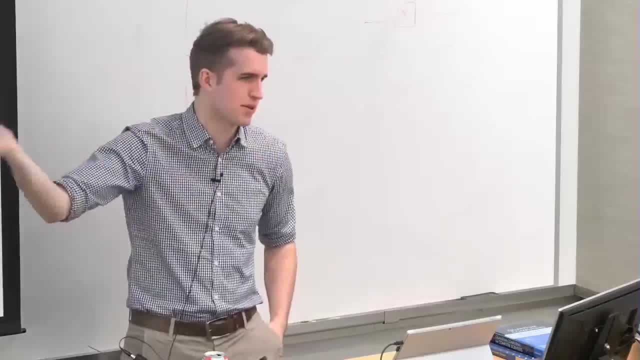 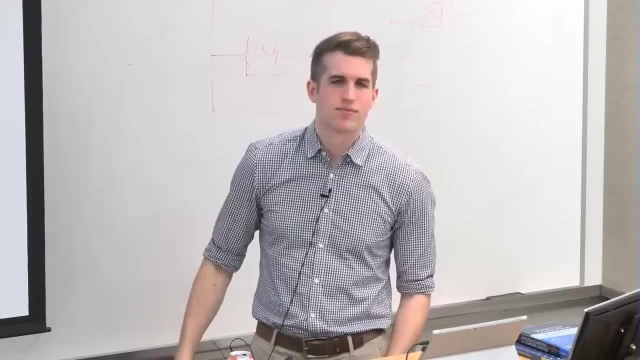 like two to the power of 80, versus like a single query. that's probably a billion years versus a week, something like that. So Okay question. So I understand the speedup, but this is a speedup in answering the question from. 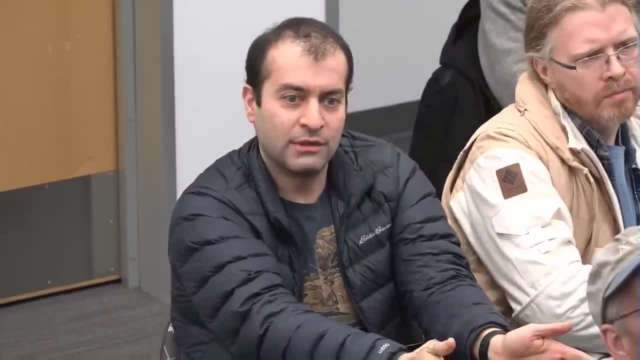 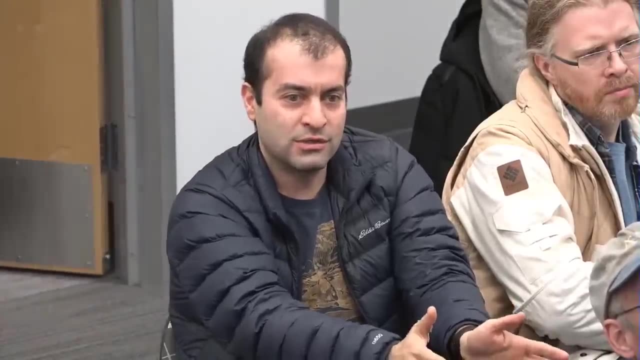 the output coming, to get the input right, Whether the function was a constant function or- Yes, Right, But in what context? is that question an important, Great question? Why do we care about this sort of thing? So, for example, in Shor's algorithm, 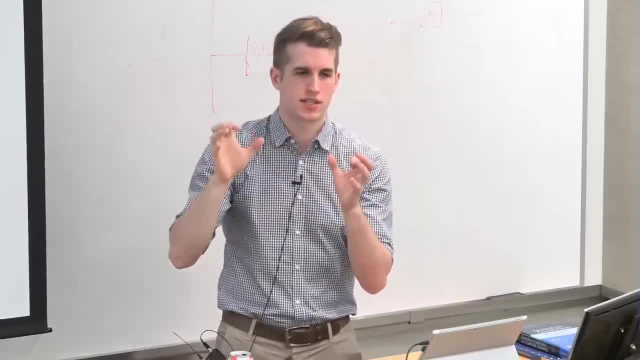 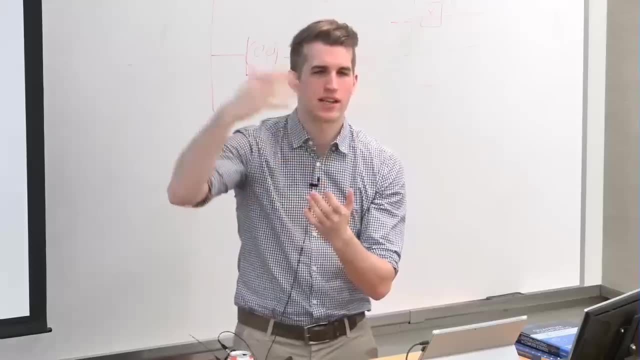 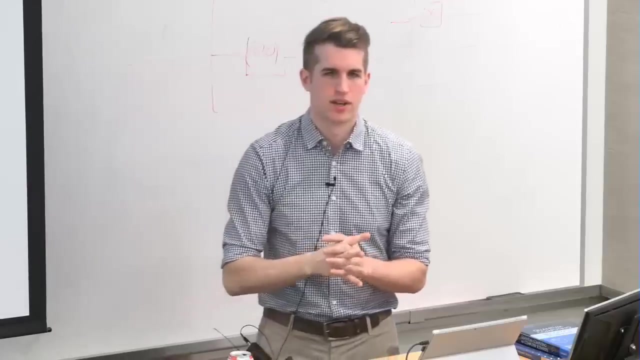 you can construct a question like: does this integer have a certain factoring structure, basically, And you can tell a property like whether it has that property or not, basically, which will allow you to, and if it does have that property, you can like factor it pretty much. 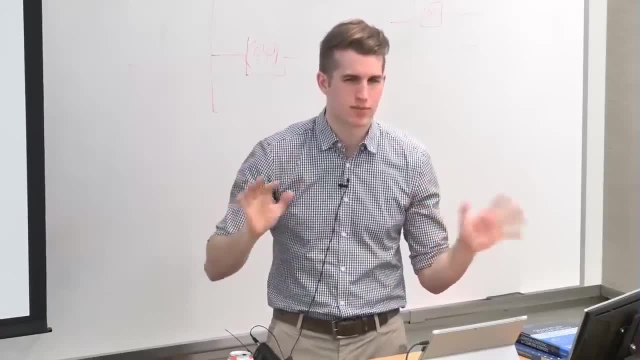 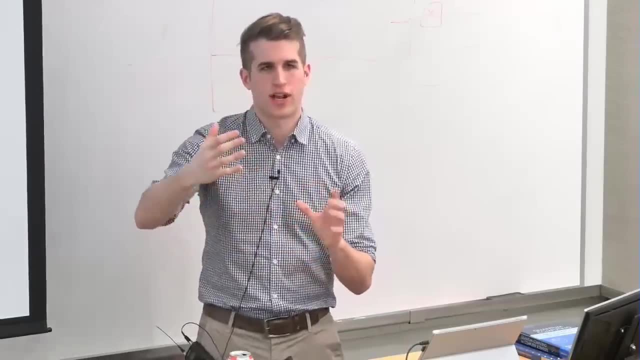 It's very, very hand-waverly explaining how Shor's algorithm works. So you can construct a lot of problems in terms of: does this function have a certain property or not which you can find efficiently on a quantum computer? I hope yes. 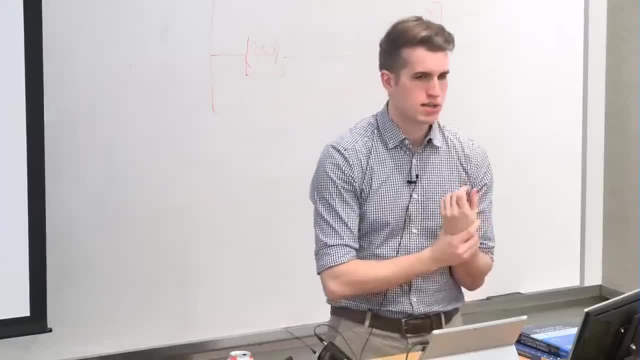 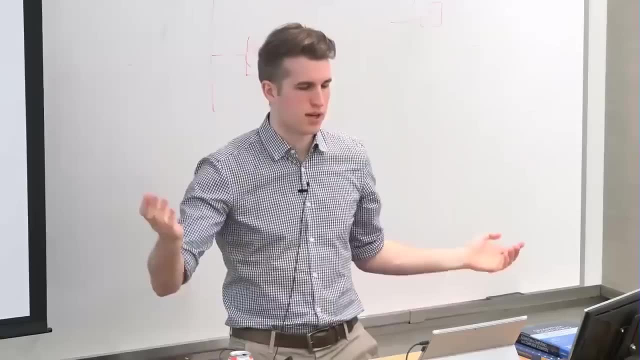 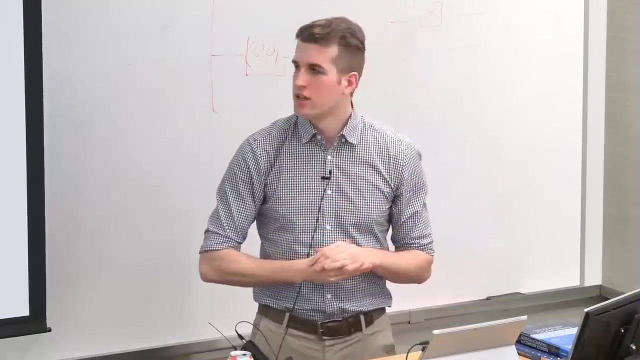 Do you mean decision problems? Mainly decision problems, Although, like as we know from theoretical computer science, decision problems can be usually be turned into like general find me the answer problems and vice versa. So yeah, Okay, Pretty good so far. 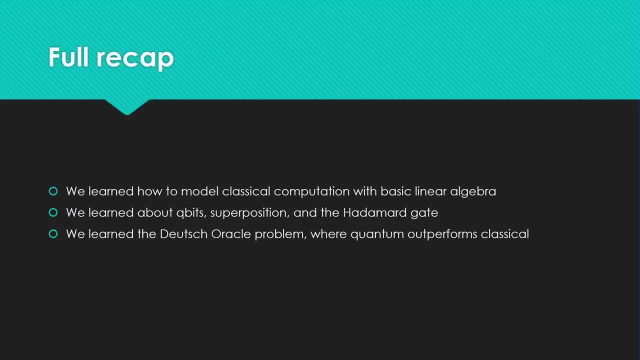 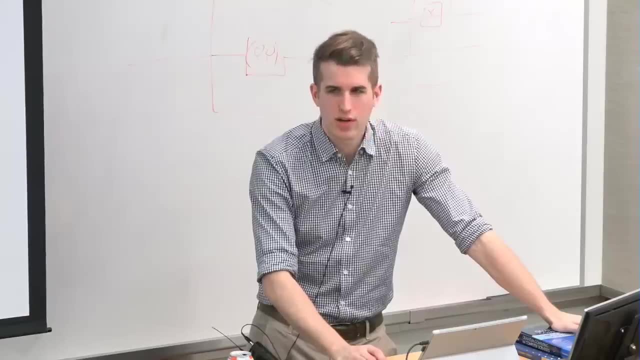 And yeah, to recap the whole presentation, we learned how to model classical computation with basic linear algebra. We learned about qubits, We learned about superposition and the Hadamard gate And finally, we learned about the Deutsch-Oracle problem, where quantum outperforms classical. 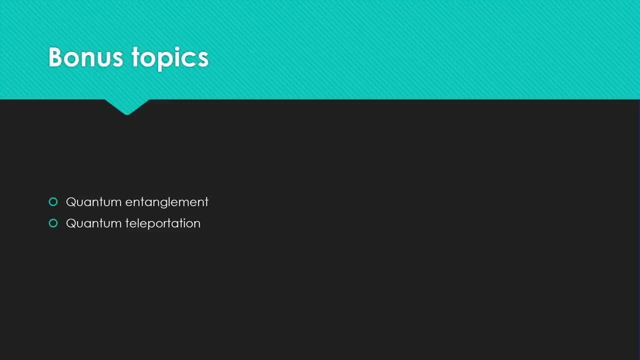 Pretty nifty, huh. Okay, Now the bonus topics. With all the tools we have, these will be a breeze for you. You'll never have to read some pop science article about quantum entanglement and like try and muddle through their horrible metaphors. 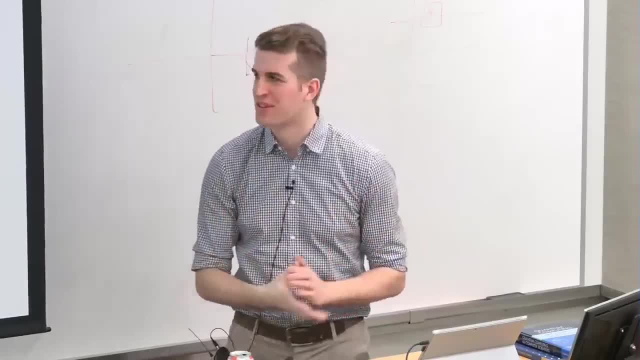 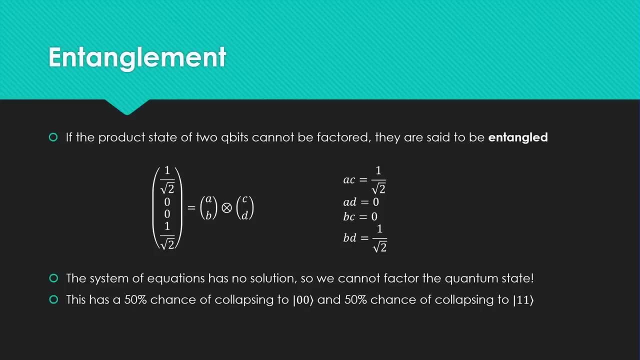 You'll actually know the math. all right, You'll know the math. That is incredible. And we'll go over quantum teleportation, which is super, super nifty- Like it is mind-blowing. Okay, Quantum entanglement. 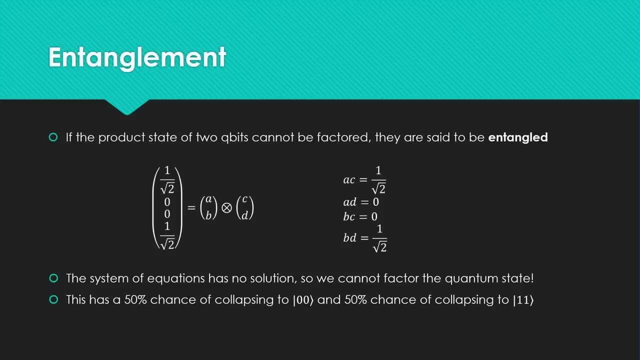 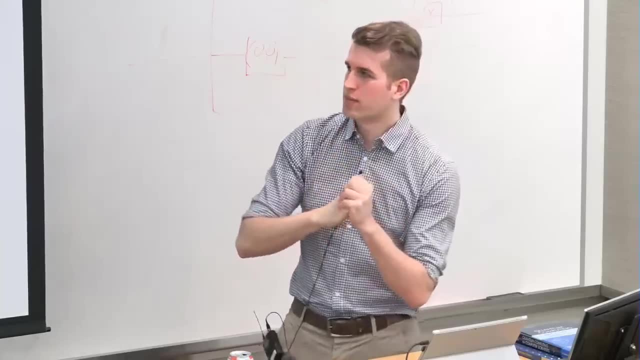 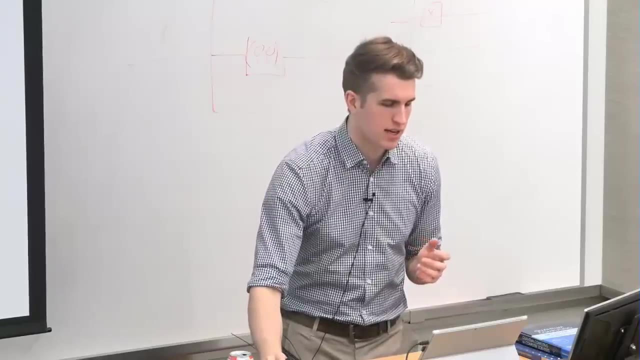 You asked a great question, a very pressing question, earlier, which is: can we always factor the product state into the qubit state? When we cannot do that, that means that the qubits are entangled, For example, this state If we have qubits in this state. 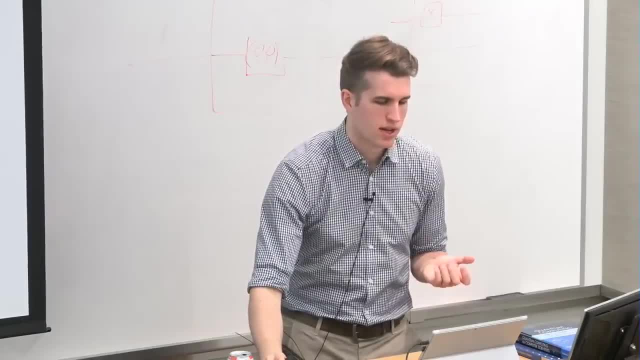 which is one over root two, zero, zero. one over root two. If we try and factor this, we can't. So let's try and factor this We should. if we can factor it, we should be able to write it as: 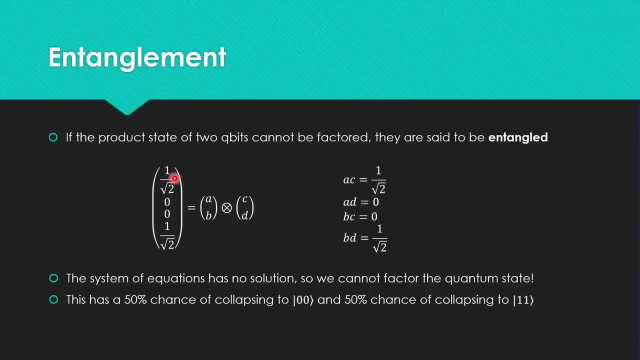 the tensor product of two matrices Right, Where A times C is one over root two, A times D is zero, B times C is zero and B times D is one over root two. So we have this set of equations right. 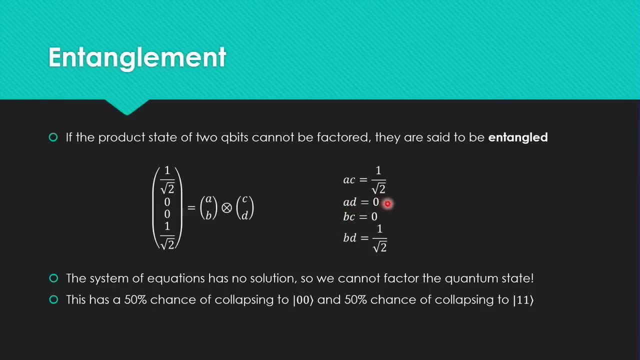 Now A times D equals zero. That means A or D has to equal zero. If A equals zero, then AC would equal zero and it doesn't, so A cannot equal zero. If D equals zero, then BD would equal zero. 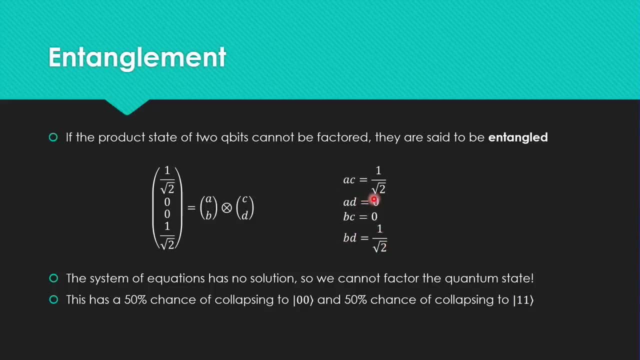 but it doesn't. so D cannot equal zero. So the only solution is: there is no solution. We cannot factor this. This is an unfactorable state, And what this means is we cannot separate these qubits. They have no individual value. 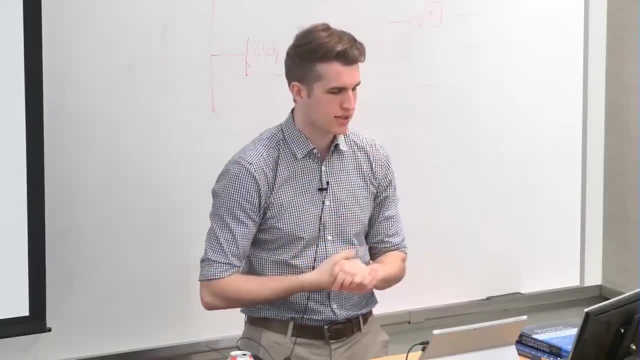 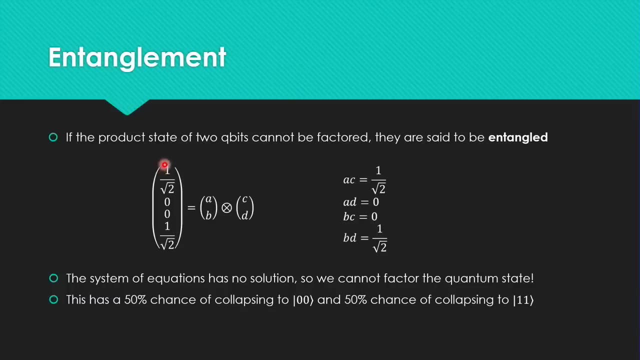 Their value only makes sense together. They're called entangled, And the way we might think of this is that this: if we measure this state, it has a 50 percent chance of collapsing to zero- zero and a 50 percent chance of collapsing to one one. 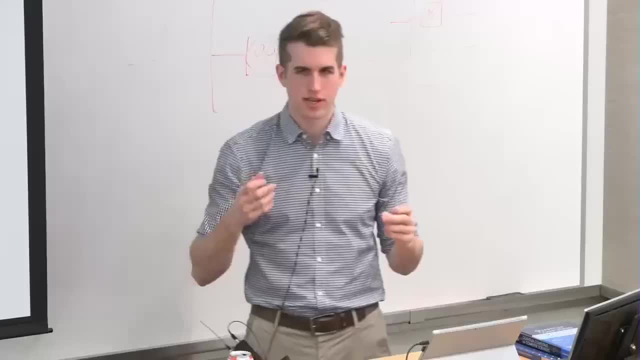 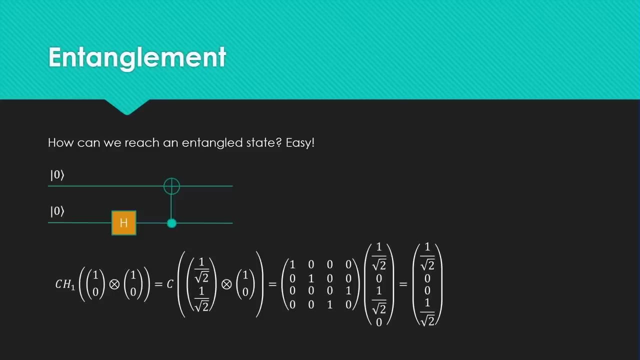 So the qubits are coordinating right. Does anyone have any confusion with this sort of mathematical representation? Okay, let's talk about what it means. Well, let's not talk about what it means yet We might be like. well, Andrew. 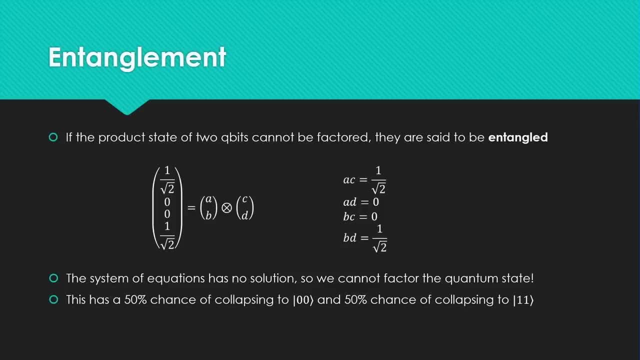 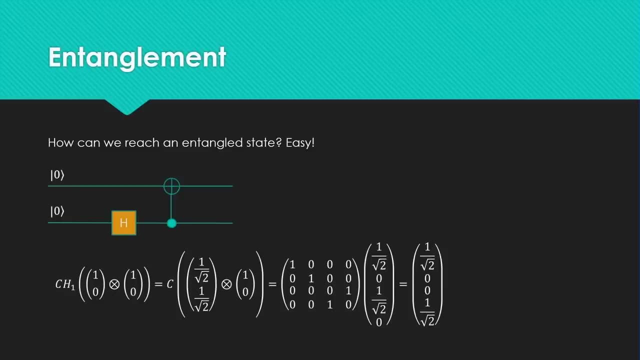 I can sling any old value into the vector. How do you actually entangle qubits? It's really simple: If we have two qubits, we just put one qubit through the Hadamard gate to put it in superposition and then that qubit is the control bit in a CNOT. 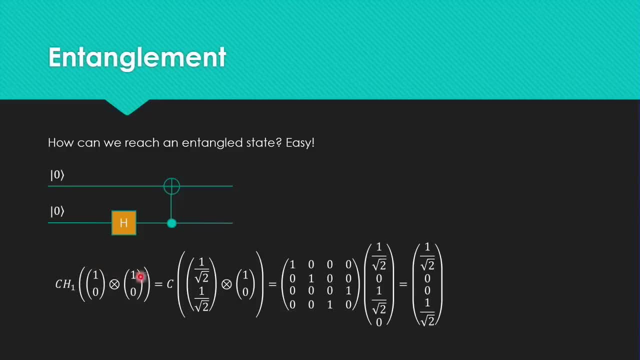 Two gates. that's all we need. Here's how it works mathematically. We started with zero zero, We put the most significant bit in superposition right, And then here's our familiar matrix- CNOT matrix. If we apply it to the product state, we get this: 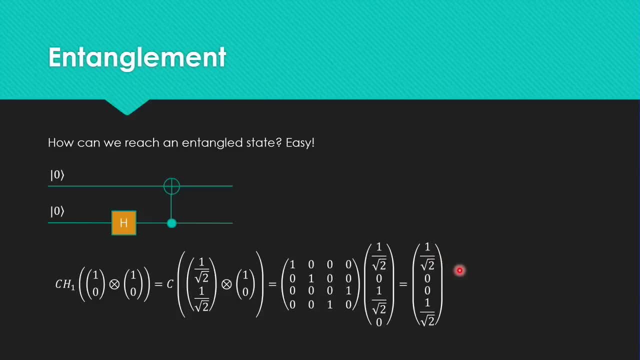 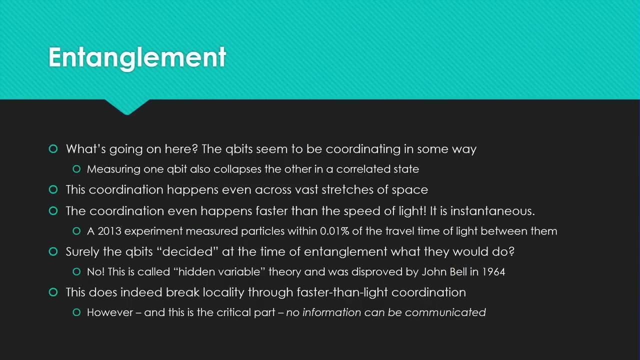 This is the state from the previous slide, right? So really simple to entangle qubits. okay, What does this mean? I mean they seem to be coordinating or like communicating or something in some way. right, These two qubits. 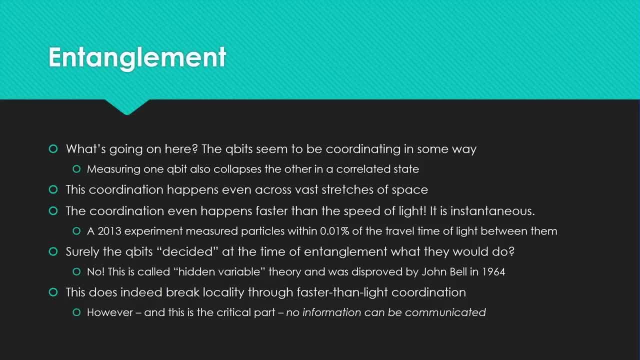 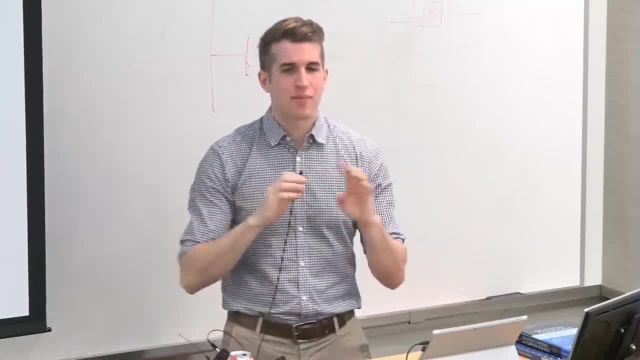 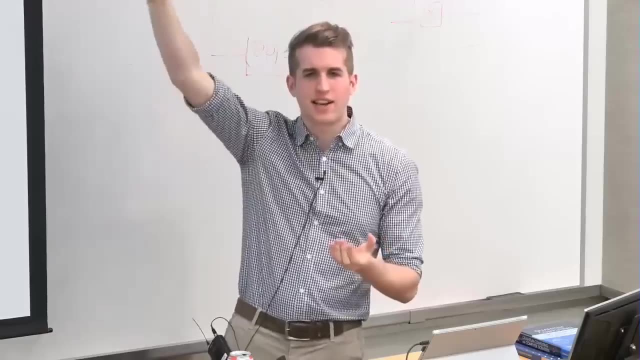 And if you measure one qubit, it collapses the other in a coordinated state. Now the weird thing here's how we're getting into really weird stuff here. okay, This happens across huge distances. China just this year managed to do this between Earth and a satellite in space. 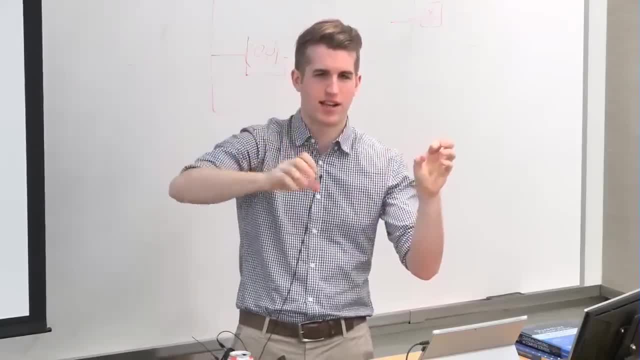 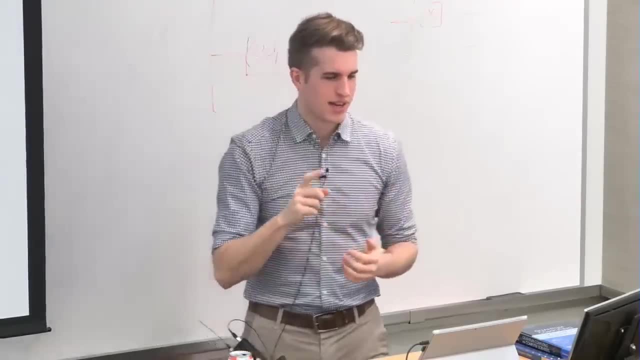 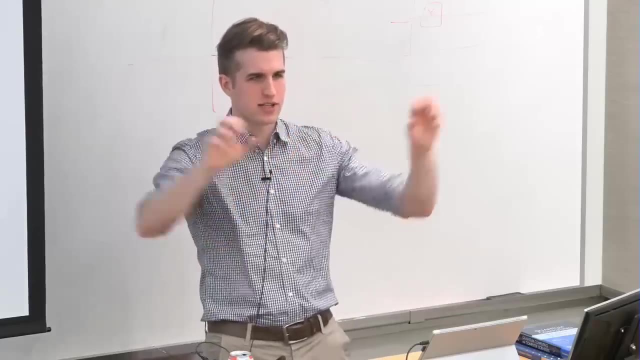 They entangled qubits, put one half on the satellite. It was launched into space. When they measure them, they're the same value. It happens across huge distances. It happens faster than light. It is instantaneous. A 2013 experiment entangled qubits. 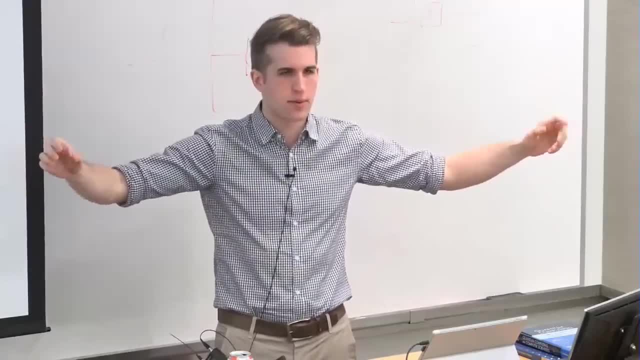 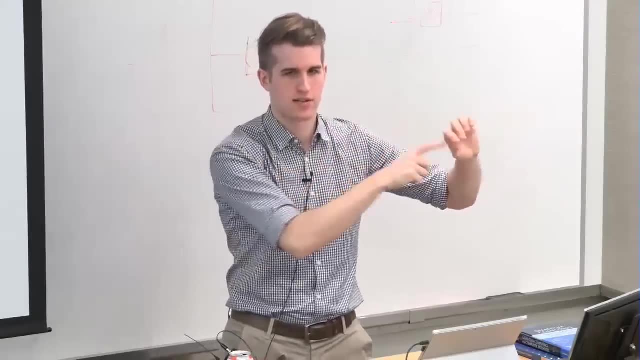 moved them very far apart, Synchronizing with an atomic clock. they measured them very close together, So close together in time that it would have taken light 10,000 times longer to travel between them. So they aren't communicating with any sort of radiation. 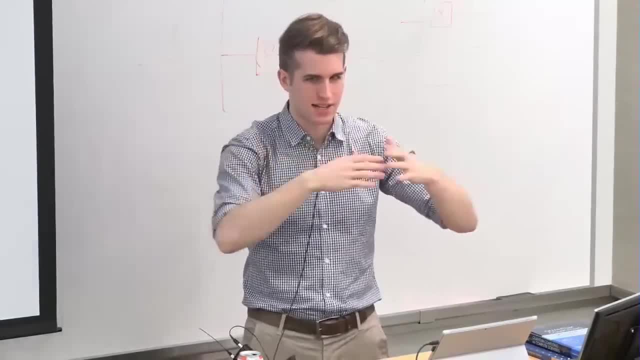 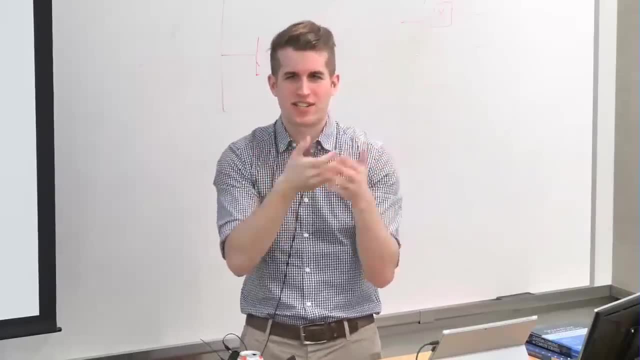 anything like that. okay, They are, it's instantaneous, It's faster than light. And you might be like: well, it's pretty obvious what's going on here. When the qubits were entangled, they just decided ahead of time what they're going to do, right? 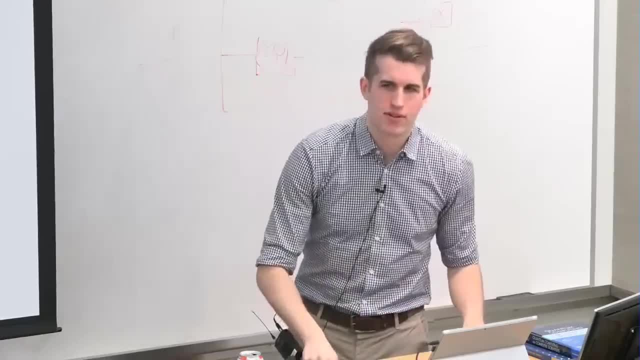 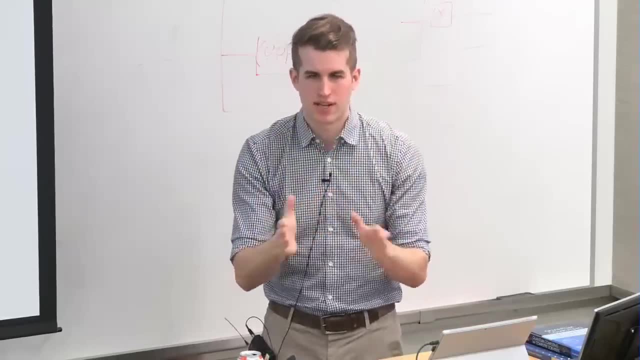 Like that explains everything, But that's called hidden variable theory. This is hidden variable theory. It's the same reason that when a qubit's in superposition, it isn't secretly zero or secretly one, it's both. It's the same thing. 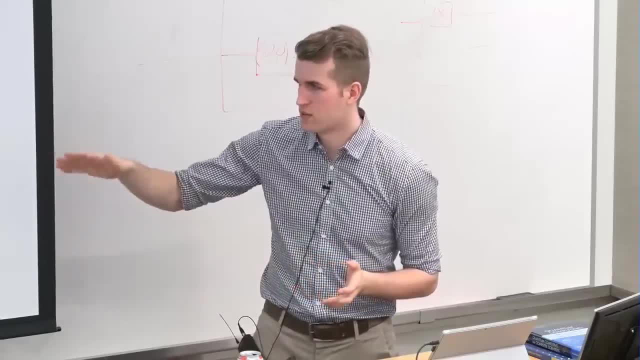 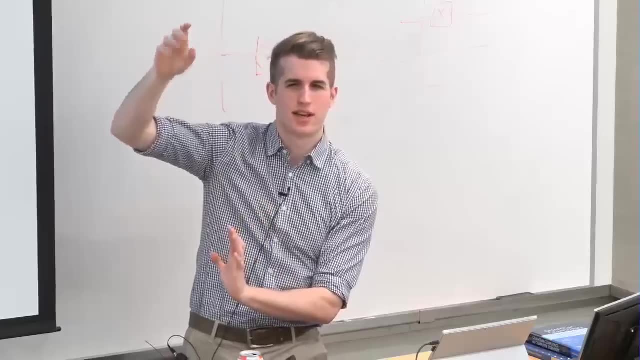 And hidden variable theory. we're not going to go over the proof why it doesn't work, But basically there's this guy named John Bell and he showed that if hidden variable theory were true, it had some really weird implications And therefore it's untenable. 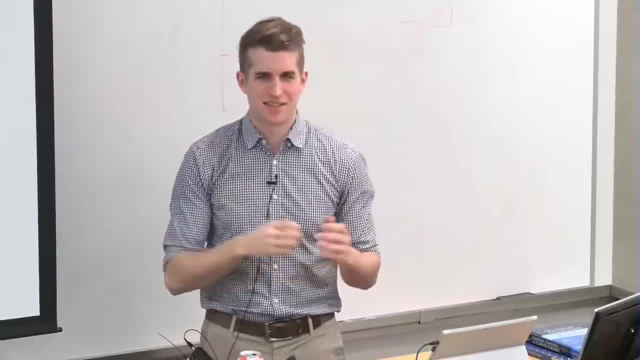 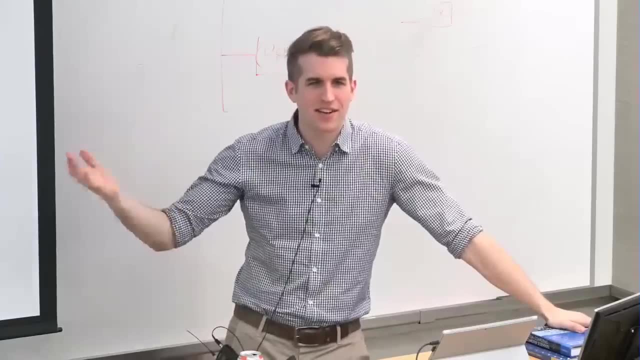 It's just the state, it's just how the universe works. They coordinate faster than light. They just do That's nuts And you might be like. well, I've been taught my entire life there's a universal speed limit- the speed of light, right. 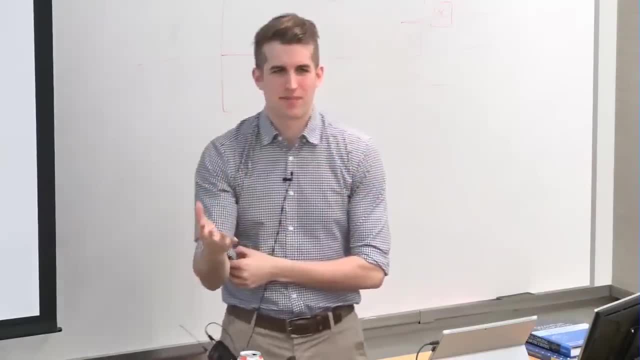 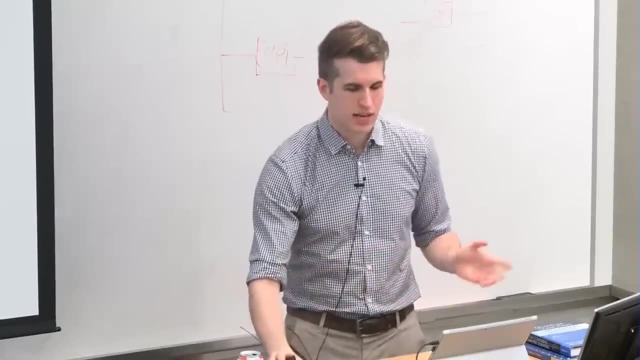 Like: what's up with that? We can't just chuck it all out. And this was, in fact, a big source of consternation to Einstein: the idea that locality wasn't true. And then it was discovered that there's a really important qualifier. 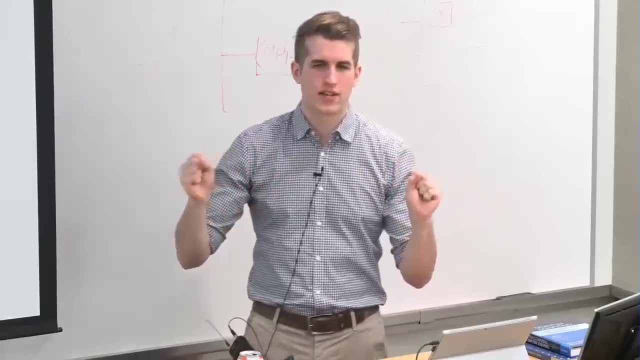 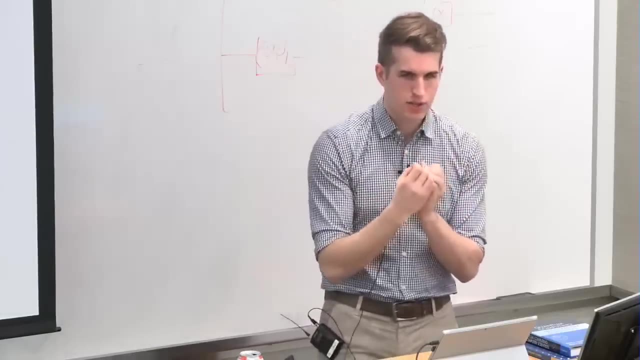 It's. you can have faster than light coordination, but you cannot have faster than light communication. So information cannot be communicated. So think about it. If I entangle two qubits, I give you one. we go to opposite ends of the universe. 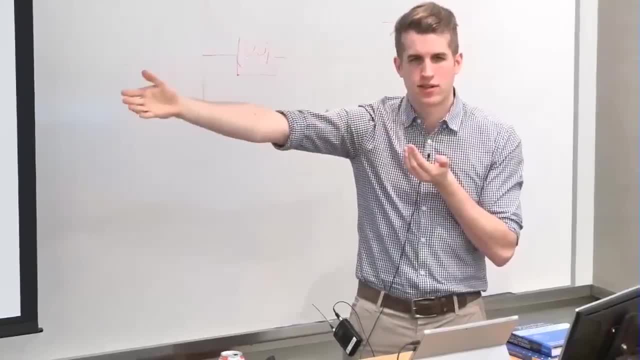 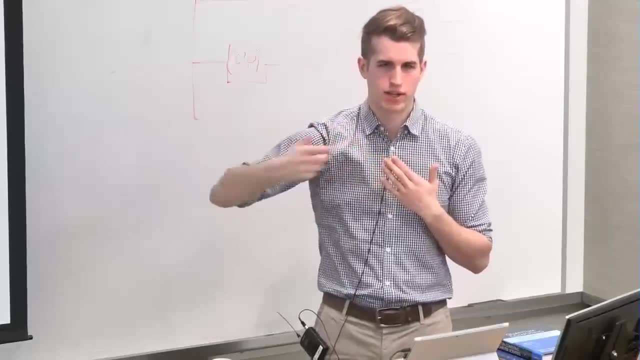 If I collapse mine, all I know is that you collapse yours. when you collapse yours, you will see the same thing. There's no, no information that can be communicated there really. So faster than light coordination is okay. Faster than light communication- not okay. 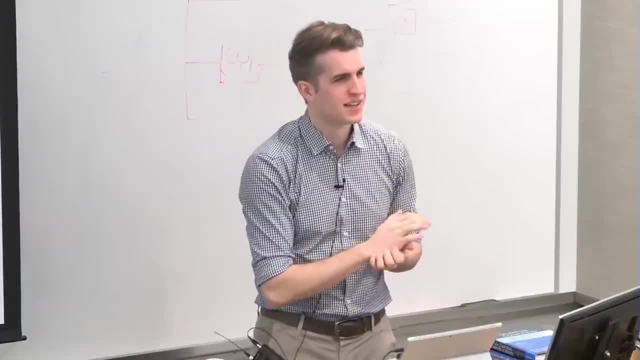 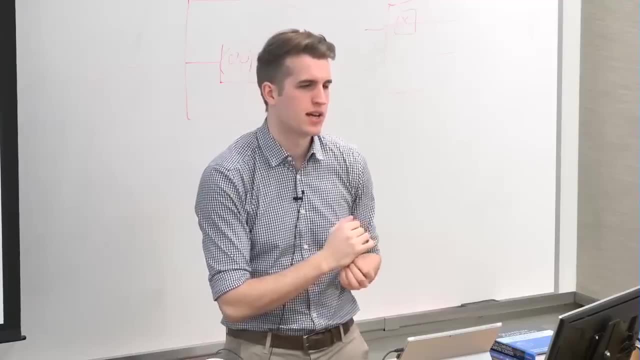 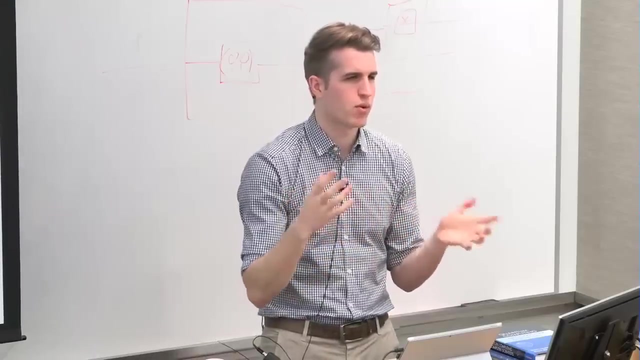 Okay, Yes, So coordination does not involve communication. It does in a way, but communication here is a technical term which means, like you, can I have a bit of information that I can transfer to you pretty much. So I use the term coordination to try and give a name to. 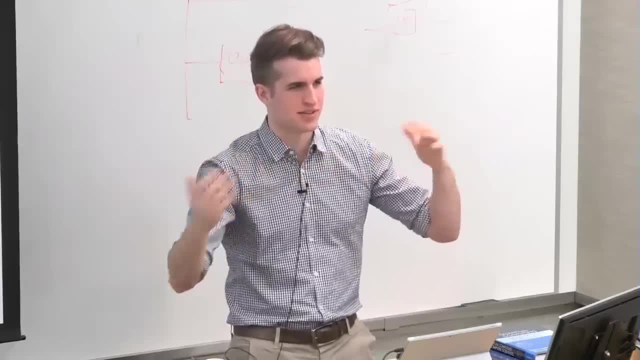 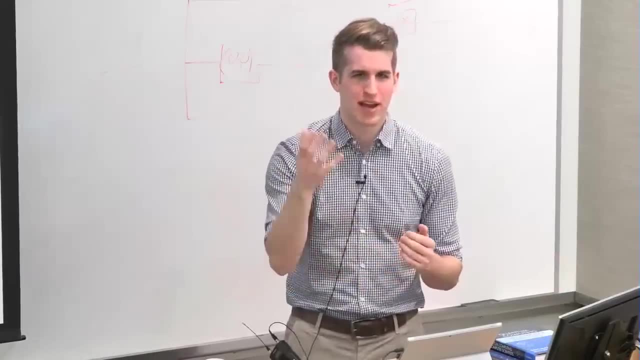 something which is not that but still involves, like some kind of coordination. I guess, Like I said, this is a limitation of our language. All we can do is look at the math and see what it does, and our language is not. 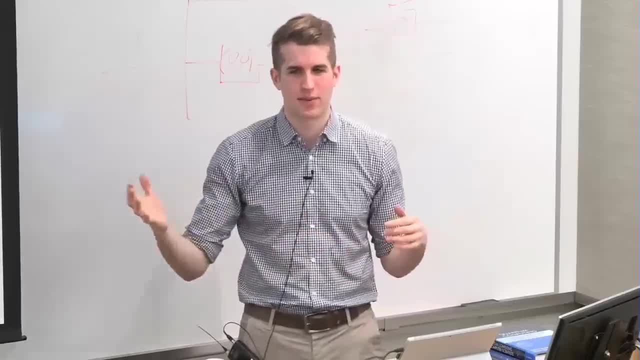 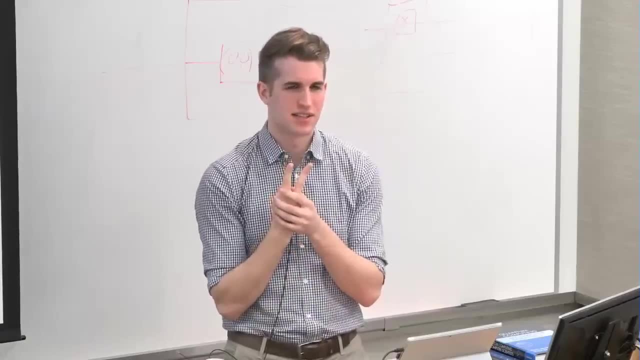 it was not developed for this. Anything I try and tell you is fundamentally a lie, except for the math. I have a question? Yes, So let's say I have two entangled qubits here and I measure one and I know its value. 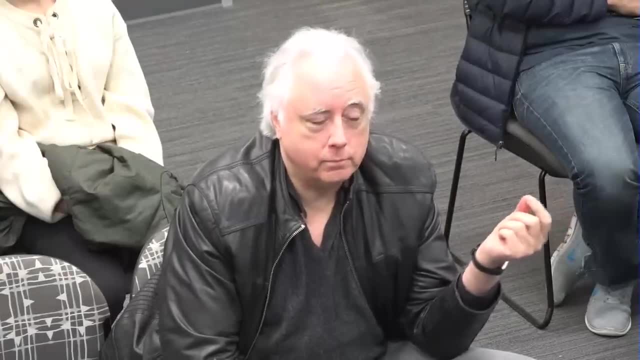 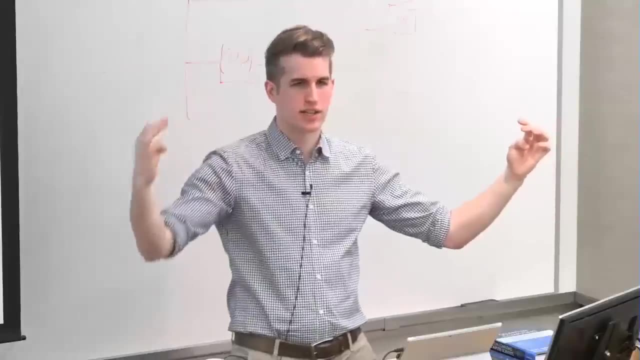 Does that mean that the other one is still, potentially still not be measured, But when it is measured it will have the same value, Right? When you measure one, it instantly collapses the other actually. Okay, That was my question. 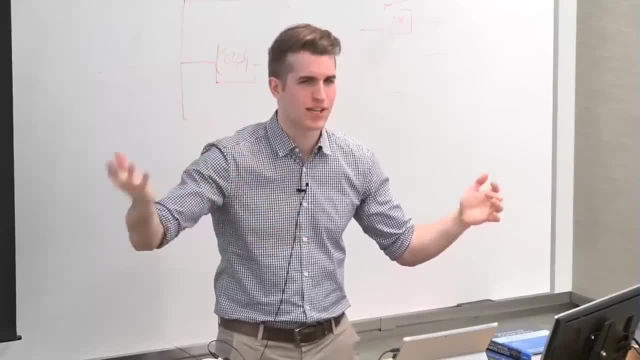 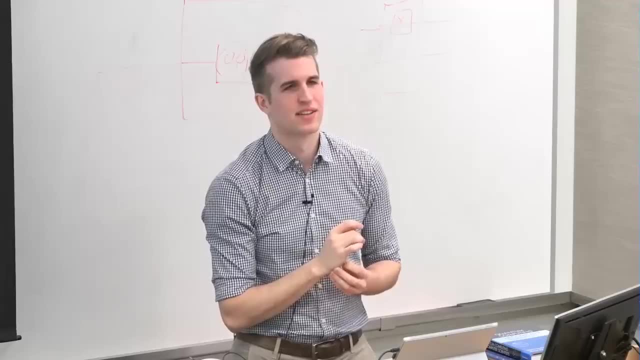 Yeah, Good, I mean, that's a simplification again of language, but you can think of it that way. Yes, Sorry, you had a question. So there's no way to tell if something has been collapsed or not. then 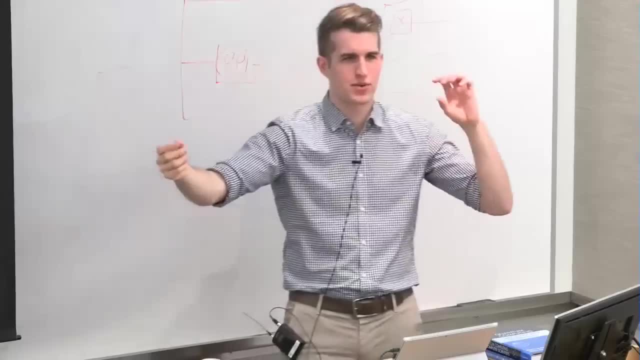 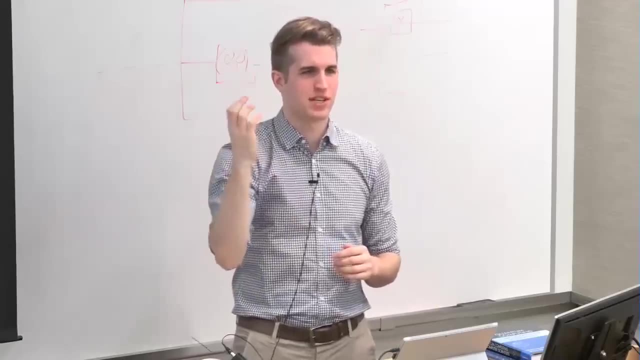 Excellent question. If you could tell whether something's been collapsed or not, you can measure one and use that as synchronization faster than light synchronization. right, Right, Yeah, you can't. Yeah, The process of telling whether something's in superposition or not would just collapse it. 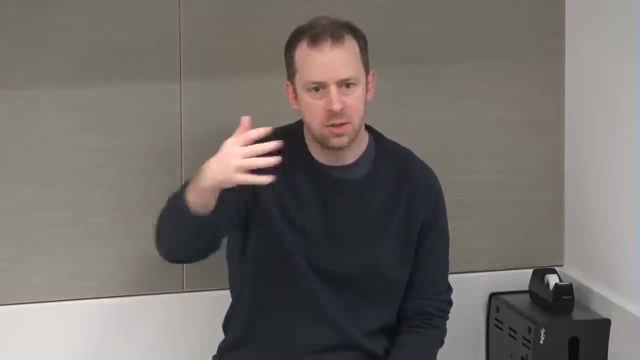 It seems like you would be able to tell through some of the quantum computation, like you do some computation on it. Yes, And if it was collapsed, it would only be this state, and if it wasn't, it would sometimes be this, sometimes be that. 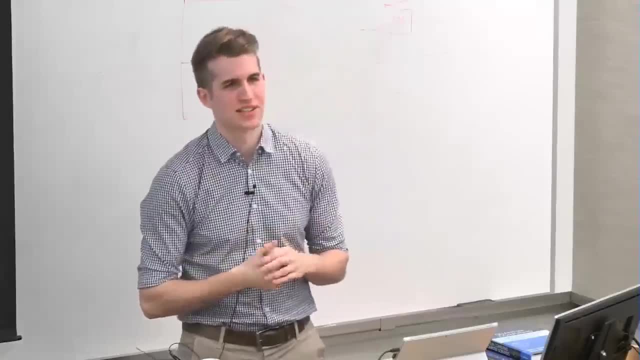 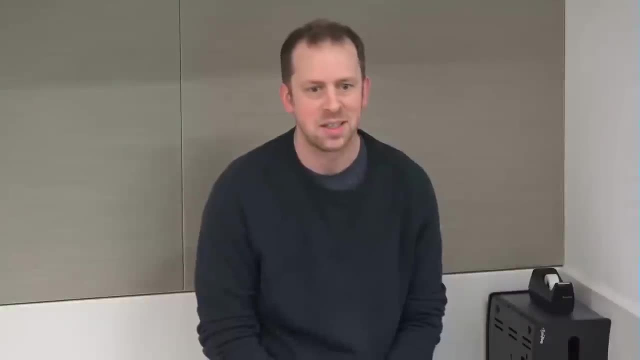 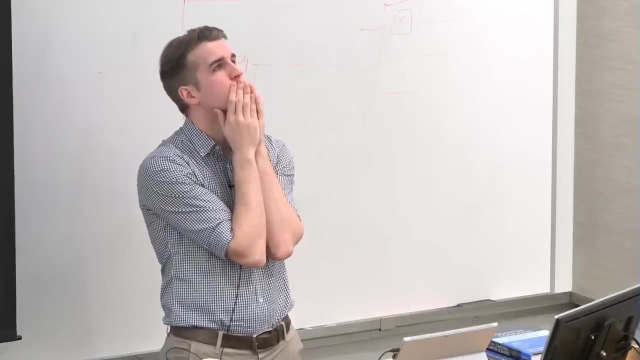 You would think so, but in fact it is not the case. I believe you. I was just ranting Yes. Is there an intuition why it's not the case? Is there an obvious? Can I say the truth? Shut up and do the math. 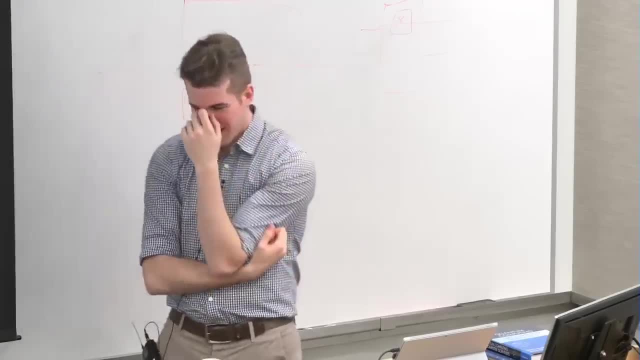 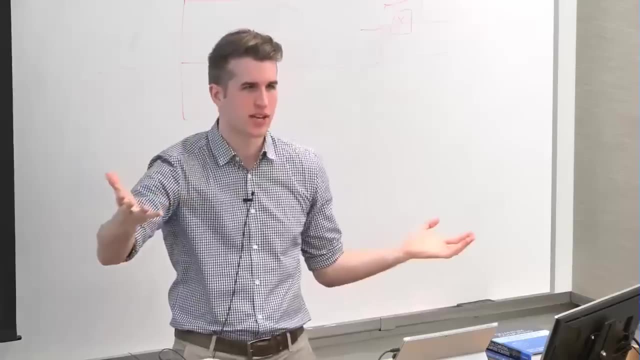 Shut up and calculate. That's a good way out. I'm not sure I can say it intuitively. I can say that if you do put a pencil and paper, it try it yourself. try and come up with some sequence of operations you could do on the other qubit which would 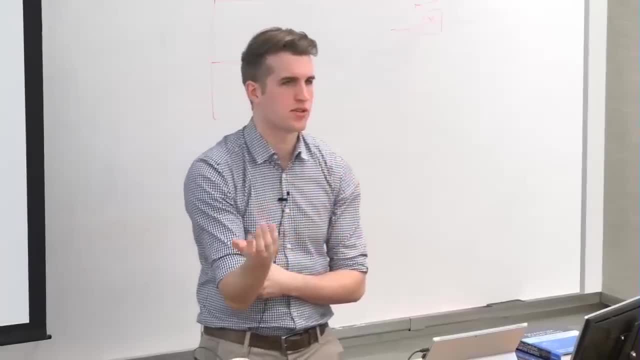 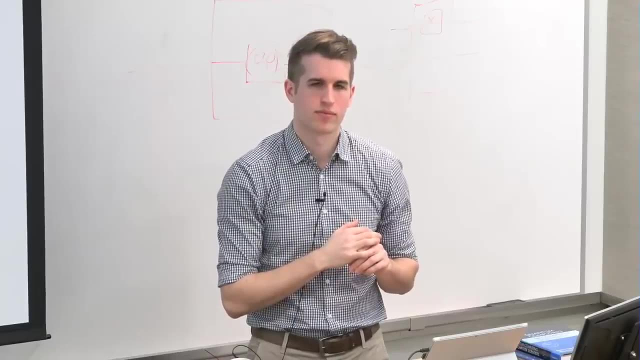 reveal it as having being collapsed or not, then maybe. but yes, Doesn't this coordination, communication, conversation that you're having violate causality, or does it? Yes, This is the critical thing. It does not violate causality. If we could communicate, then it would violate causality. 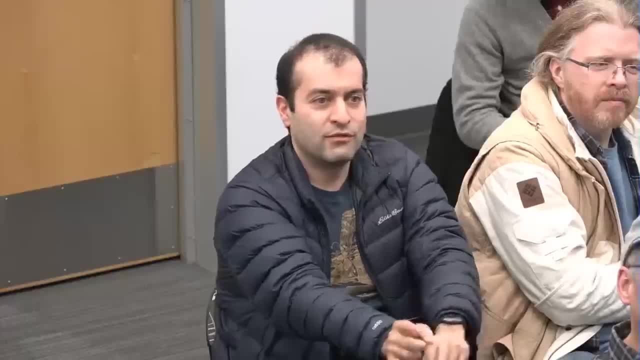 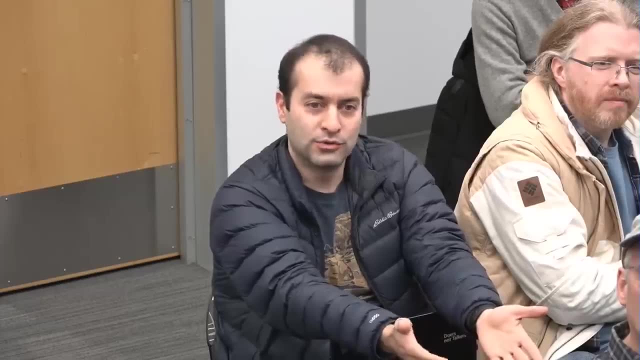 But since we coordinate, it does not violate causality. But the statement you said was: if you measure, the other one is going to be as well. Yes, The act of measurement is in your control, right? Yes, So how can that happen on the other side? or? 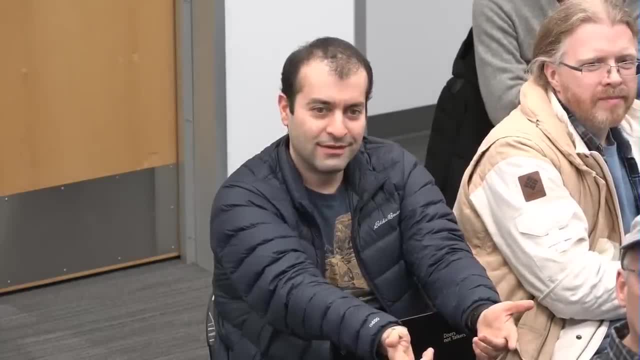 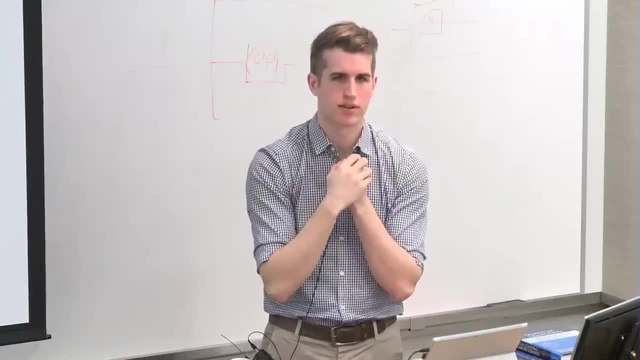 the other qubit, if you don't have communication, Because that's-? Well, let's define what communication is. Communication is I have a bit, either zero or one, and I'm able to send it to you in some way, Somehow, yeah. 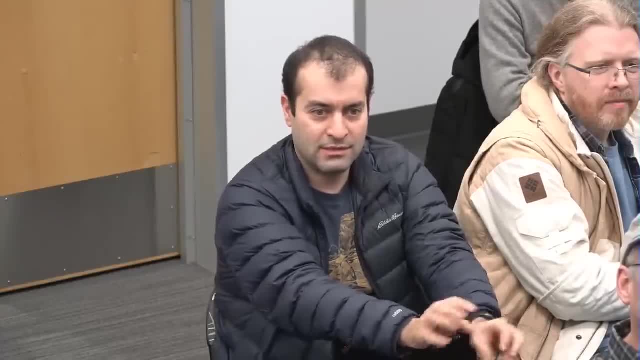 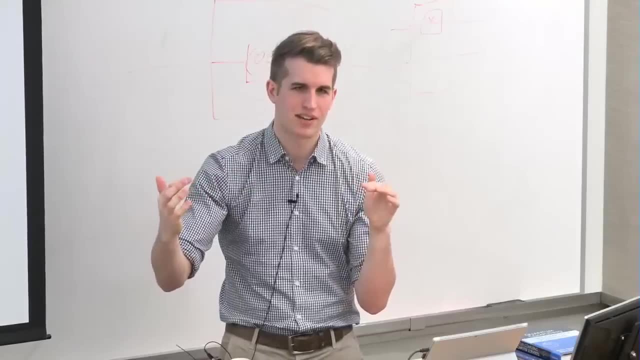 Yes State that is not collapsed be communicated to the other side. that is my, Yeah. I mean, this is a language problem. The qubits are like communicating, but we can't get information through them. basically, You might be able to say that: 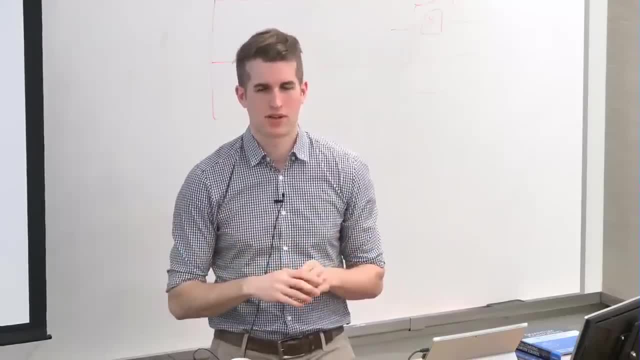 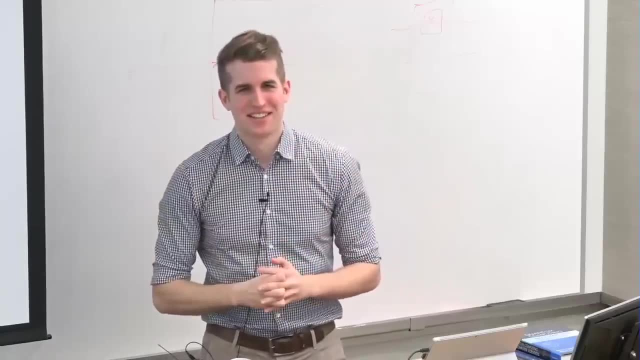 or I use the term coordinating to try and avoid this problem. Other times in literature you'll just see the word correlated, which tries to like avoid that whole problem. But the coordination, the state that the word here when you're using it. 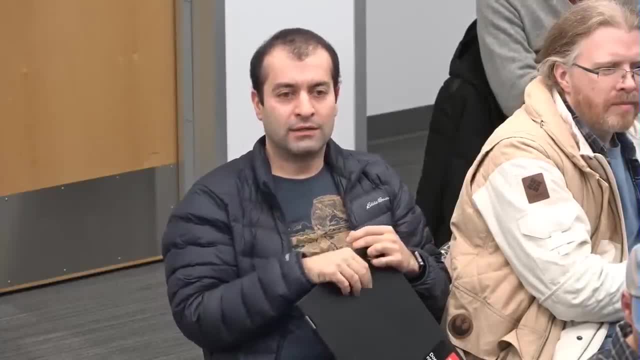 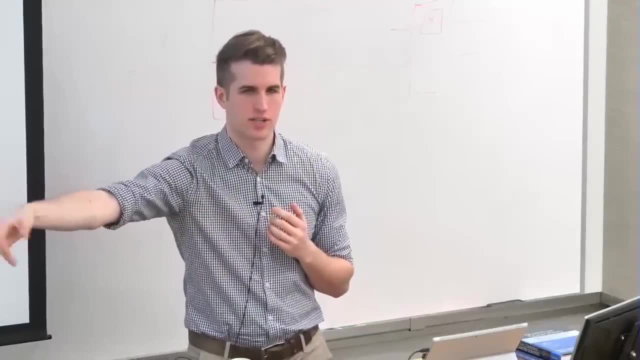 it has an action that you have performed. Yes, So you control. when you measure a qubit, it collapses the other. But there's no way you can change causality in that other qubits frame. Basically, there's no way you can get. 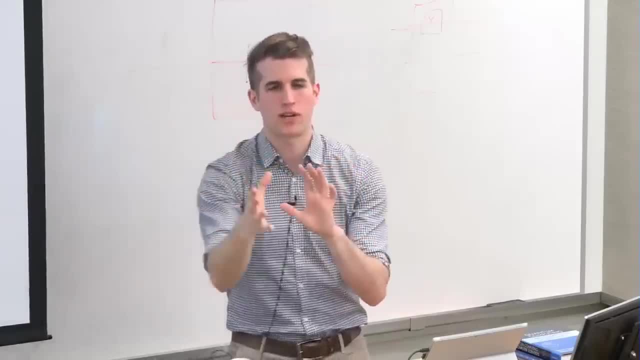 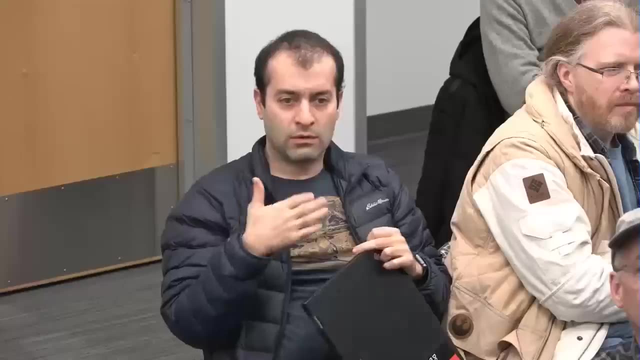 information from your frame into that frame, which would affect their causality. All we can know is we have generated the same random numbers basically. Yeah, It's kind of like pre-coordination, So these are- I want to avoid that Pre-coordination is the qubits decided ahead of time. 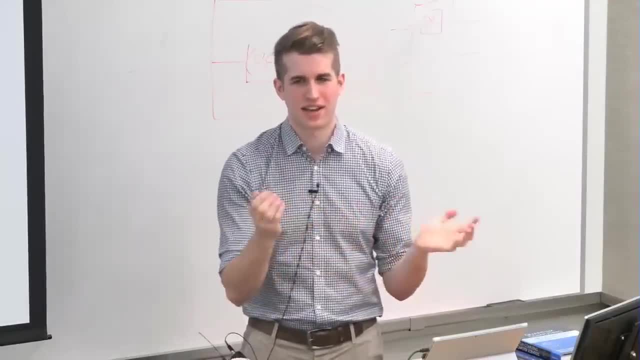 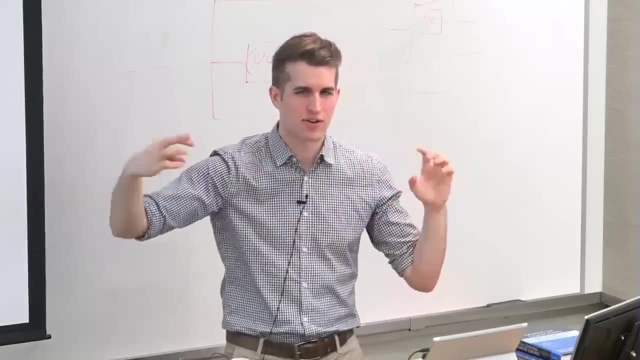 Yeah, Which is not the case, Until you measure, Until, yeah, Or until these, At the time they measure they like, decide whether they're going to zero or one and they somehow communicate that coordinate, correlate, whatever, to the other qubit. 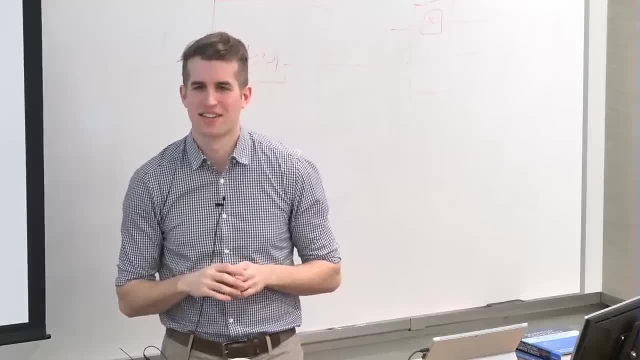 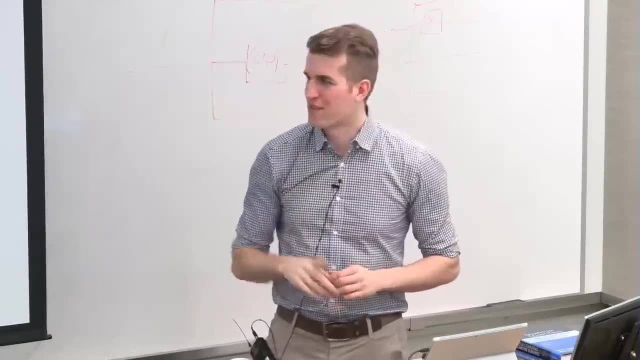 and it goes in the same. Yes, So if you cannot communicate, what's the practical application of it? Great question. We're going to get into quantum teleportation on the very next slide. First, I want to tell a funny story about this. 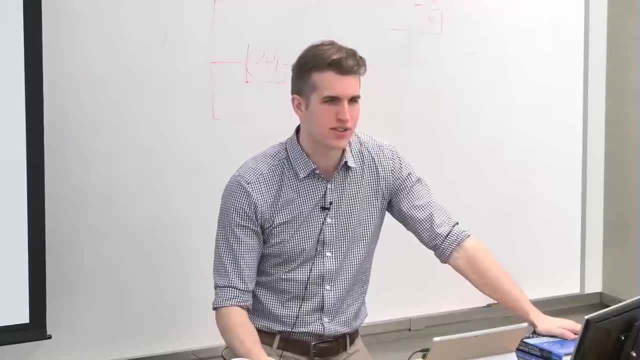 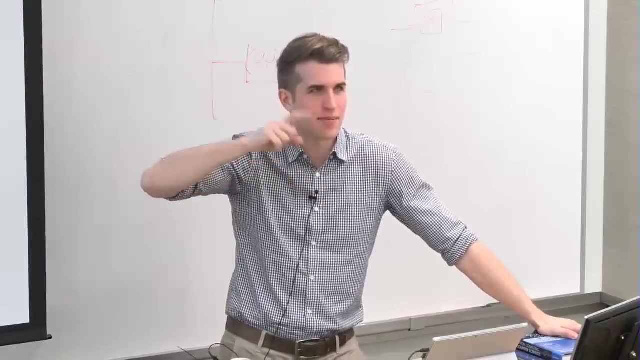 So you may have heard the phrase spooky action at a distance. This is Einstein coined that he was referring to this. So Einstein, Podolsky and Rosen are three physicists who actually came up with the idea of quantum entanglement. They call it the EPR paradox. They're like: the workings of quantum mechanics result in this. This is obviously observed. therefore, quantum mechanics is garbage was the basic argument, But then the experiments came out and they're like: no, this is how it works. 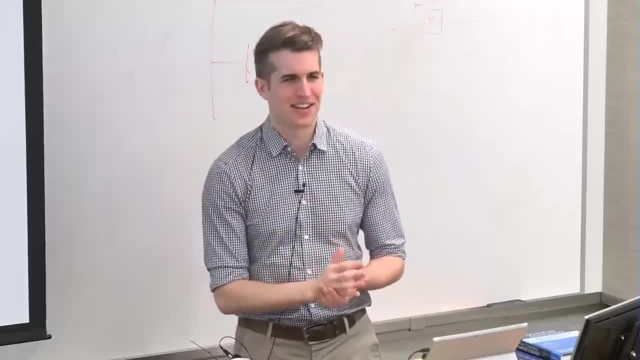 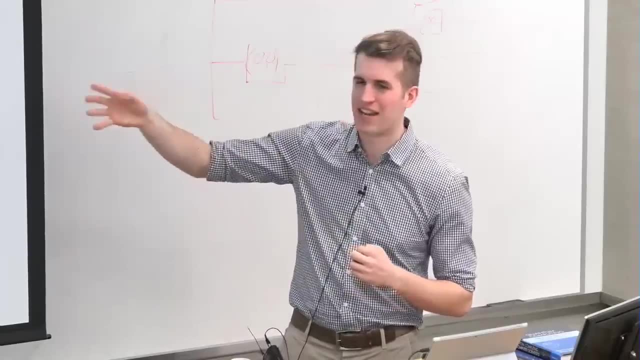 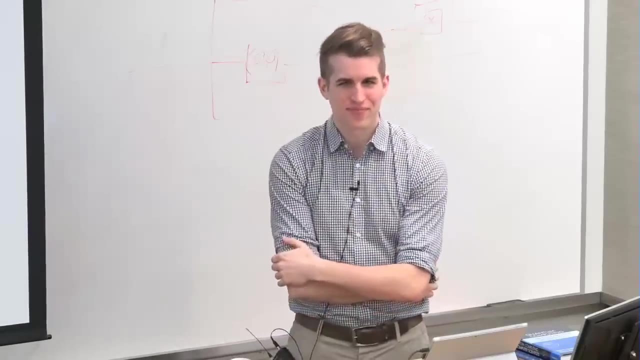 This is the universe is, in fact, absurd. locality is broken, So it's kind of funny that the EPR- paradoxes are originally designed to discredit- quantum mechanics turned out to be the actual way the universe works. I think it's a great little story. 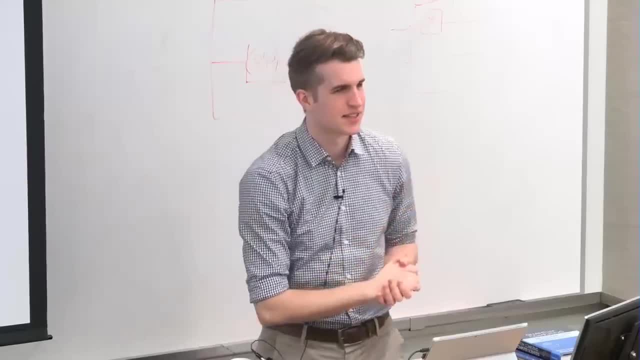 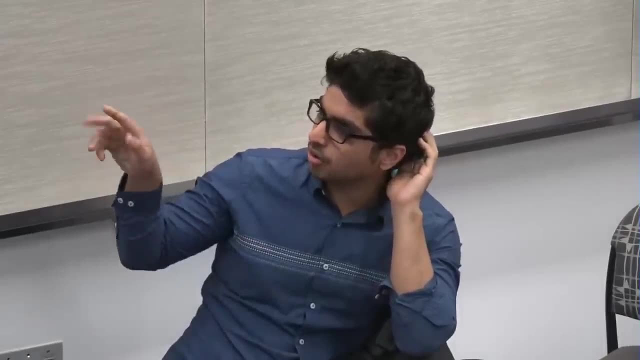 Okay, Any other questions? about entanglement: Yes, Let's say the same problem- the qubits and factors: Yes, If we say that this has a certain probability of collapsing to zero, collapsing to one, and then we observe that it collapses to one, 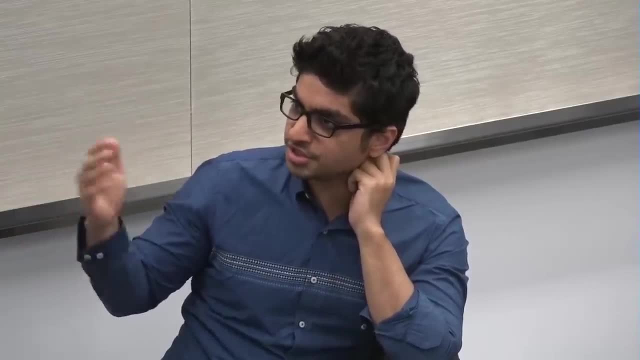 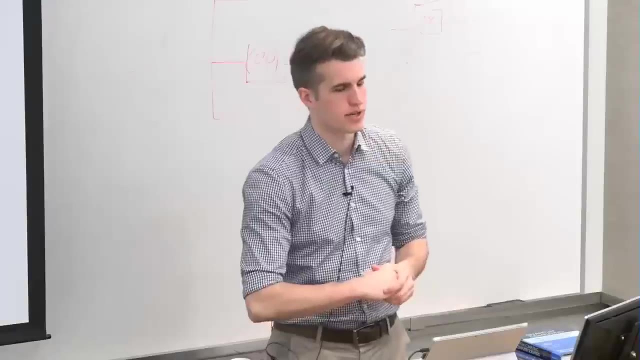 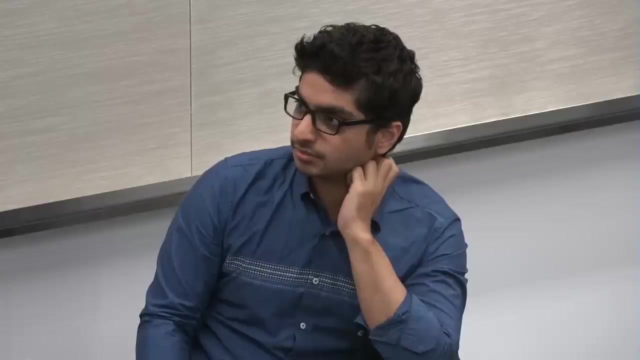 Yes. How can we justify that? our presumption that it had a probability of collapsing to zero was valid? Excellent question. The answer is: you just do it a whole bunch of times and you see that you get a 50% distribution of values. Exactly, They won't be occurring at the same time. 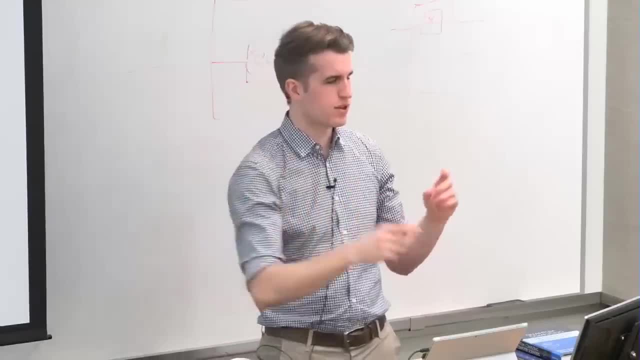 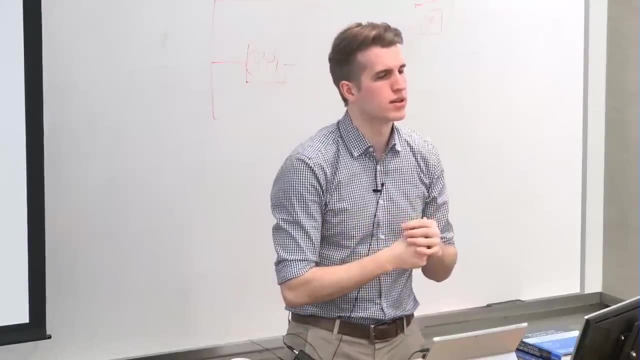 Experimentally, we know that they occur at the same time with the 2013 experiment. It entangled qubits, took them far apart. it used-. No, I mean the same qubits. Yes, It happened at time X. 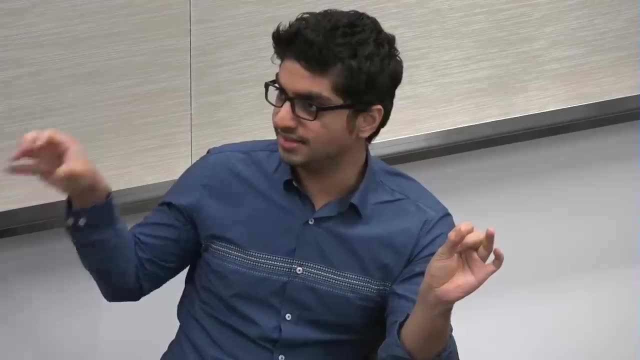 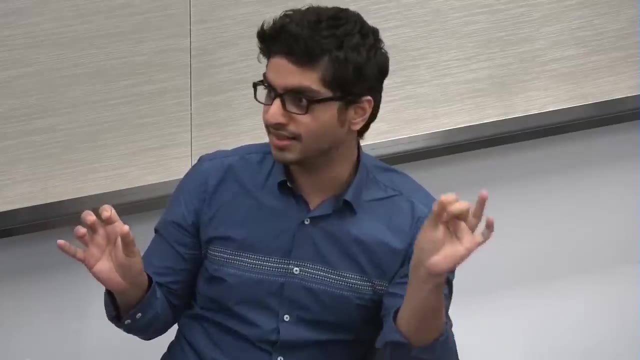 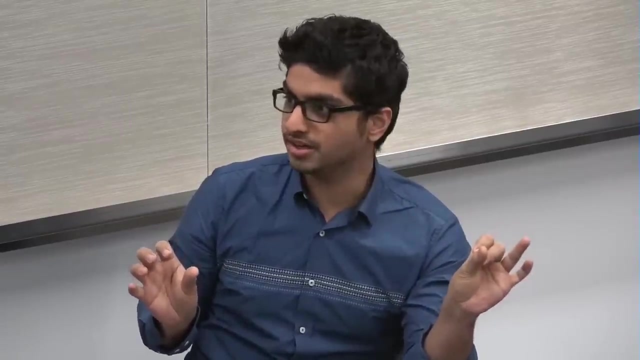 Yes, And now you take another pair of qubits, and this is another pair of qubits, but not necessarily the same ones. Yes, So until it happened at that time that space or whatever, you can't really tell that this was happening, probability: 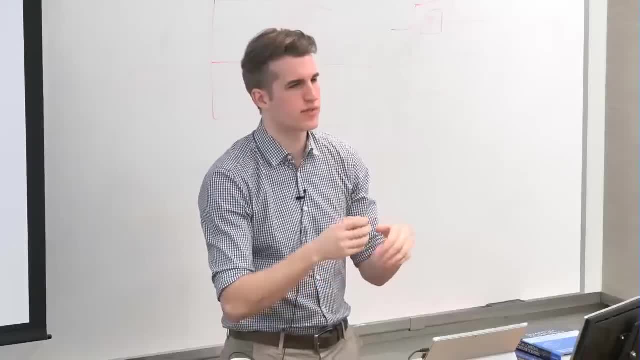 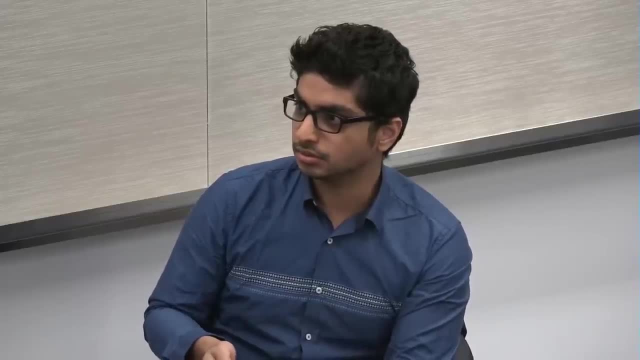 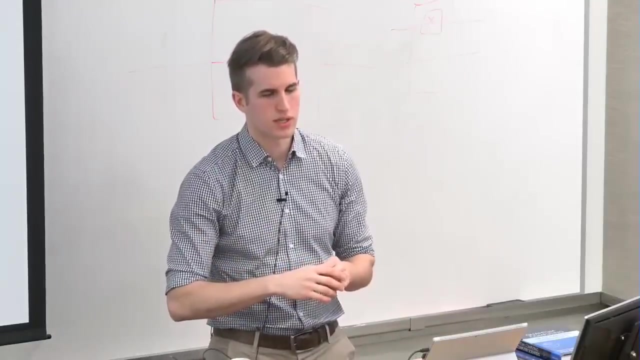 One half. Yes, You're questioning Okay, So they could have decided ahead of time, for example, maybe or- Or probably. the language of probability itself is not applicable. It works, Probability works. I mean, it's just the amplitude squared gives you. 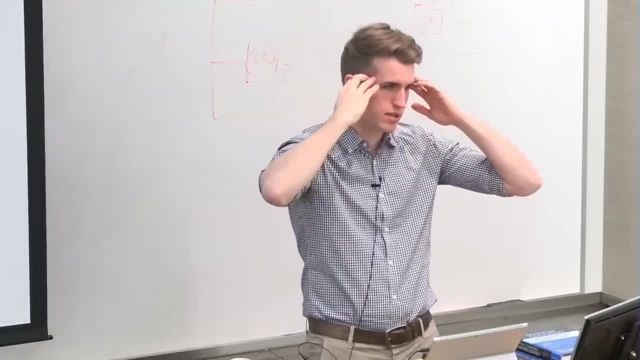 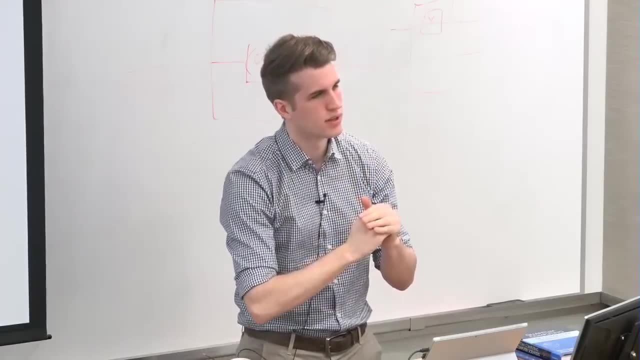 the classical probability of it collapsing to zero or one, I guess I'm not 100 percent sure what you're driving at. So So I mean: once observed, then we rationalize. Once observed, then we rationalize, yes. 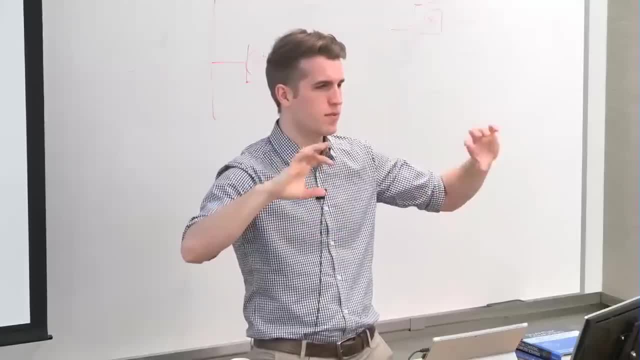 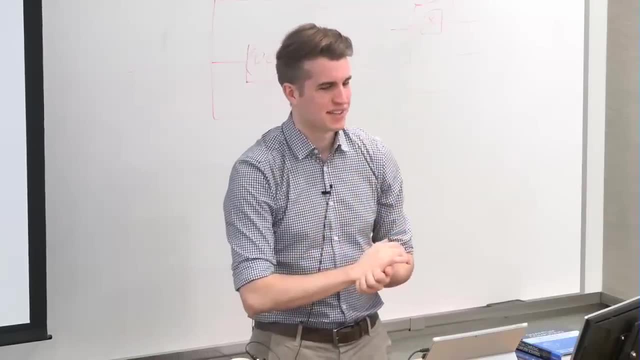 And then if we do the experiment a whole bunch of times, we see that it's about a 50 percent chance of them both being zero or both being one- Which in fact I will show that to you live on a quantum computer that we do that. 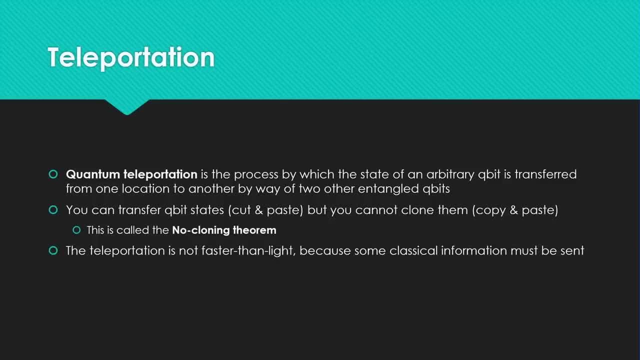 Okay, All right, Let's move on Teleportation. This is the actual use which you asked about, And you've probably read about quantum teleportation again in PopScience articles. Needless to say, it's not a problem. 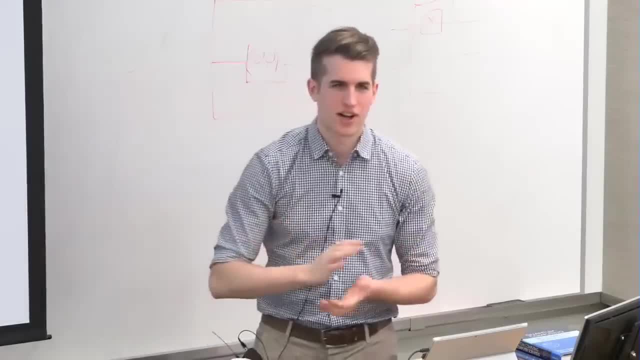 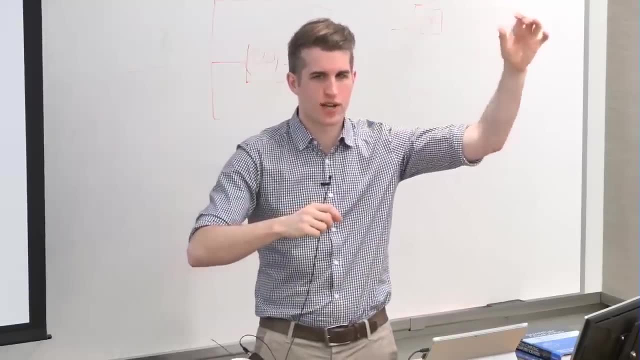 Needless to say, their explanation was complete trash, made no sense at all. But now it will make sense to you. Okay, It's the process by which we take an arbitrary qubit state and transfer it across space and time somewhere else. 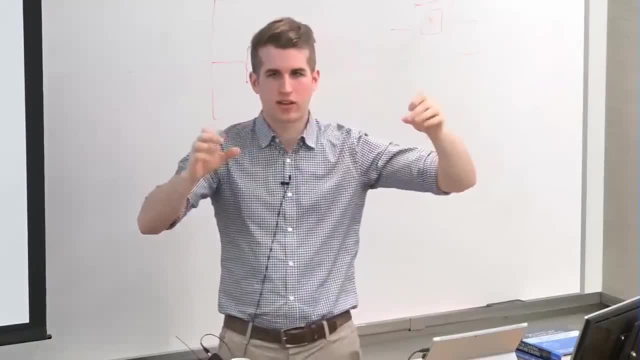 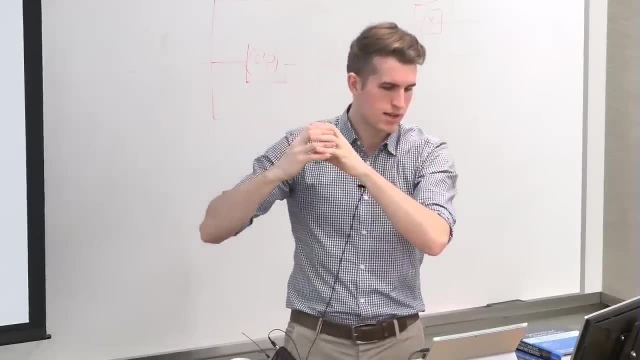 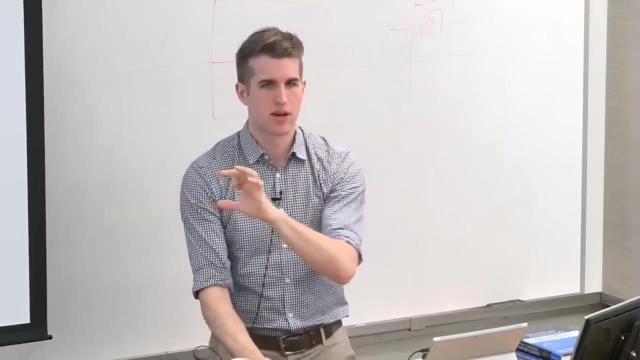 So you use entangled qubits as a sort of bridge to send a qubit from one place to another. And here's a very important thing, It's called the no cloning theorem. You can transfer qubit states, so you can cut and paste them. 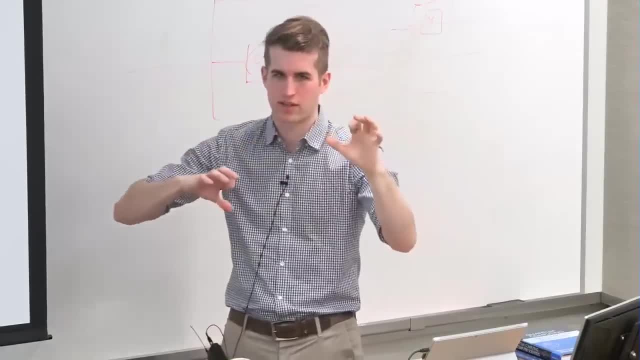 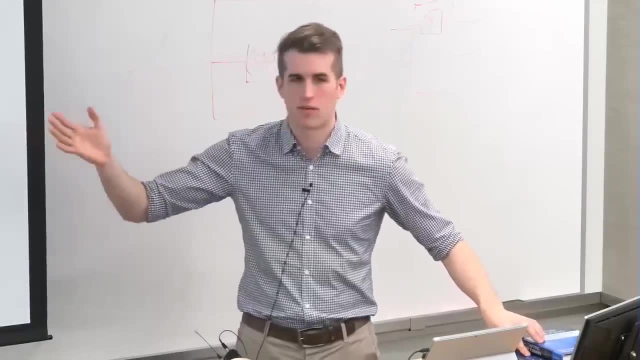 But you cannot copy them. You cannot copy and paste a qubit state. You cannot clone it. This is called the no cloning theorem. It's actually pretty simple to prove. You just show that any off such operation would not be reversible, or its own inverse. 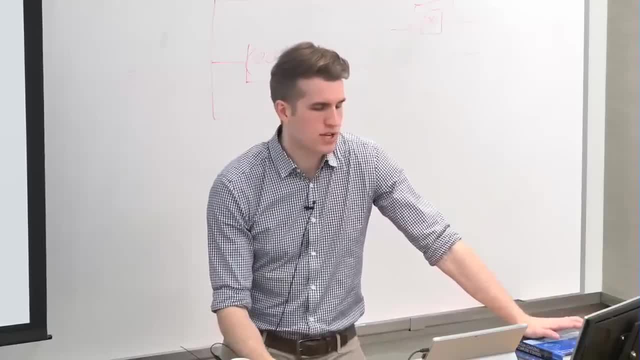 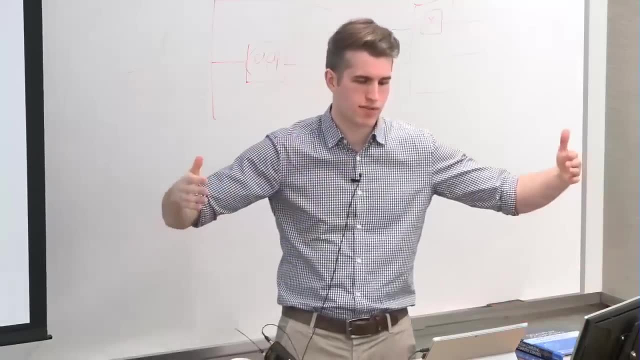 But we're not gonna go do that. And here's an important thing: The teleportation, despite using a faster than light phenomenon of entanglement, is not itself, the whole protocol is not itself faster than light for communication, because you actually must exchange two, three. 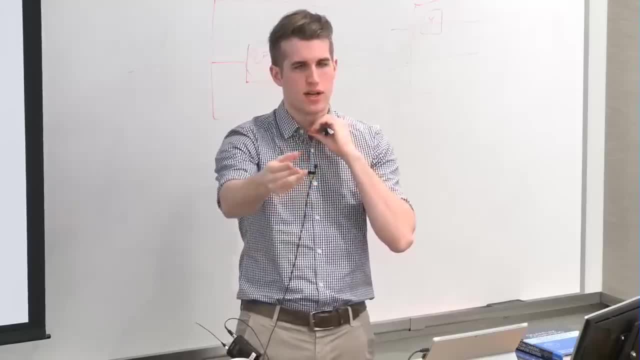 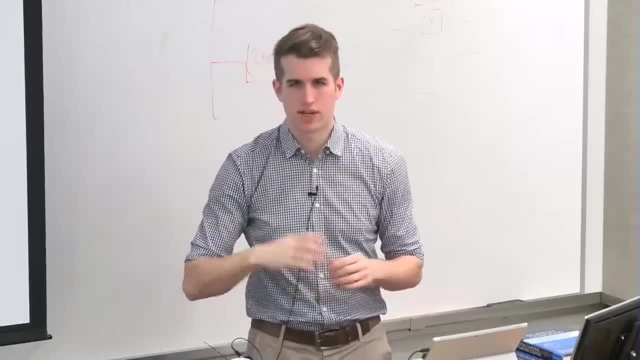 two classical bits. So if I'm teleporting my qubit to you, in addition to us having an entangled qubit pair, I also have to send you two bits of information and we'll show why that is in the next slide. So everyone kind of conceptually grasp the, I guess. 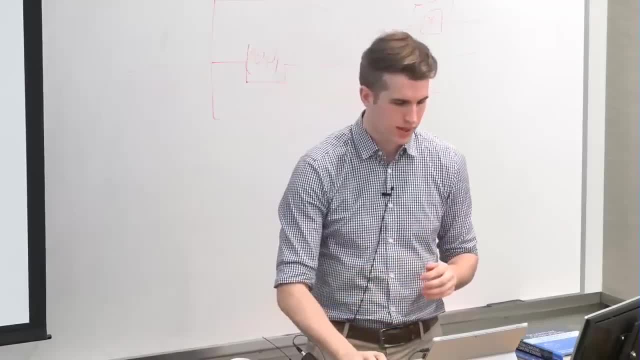 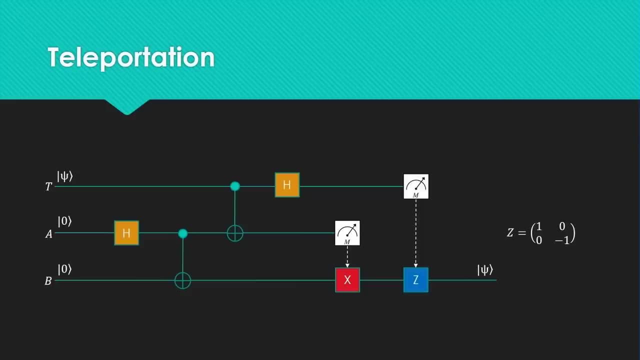 the purpose of quantum teleportation. Okay, so here's what the circuit looks like. We're not gonna go over the math. There are appendices to this slide deck which I will you can see after the class to go over the math. but it gets a bit complicated, so we're not gonna do it. So we have the qubit that we want to be want to see, but we're not gonna do it. So we have the qubit that we want to be want to see, but we're not gonna do it. 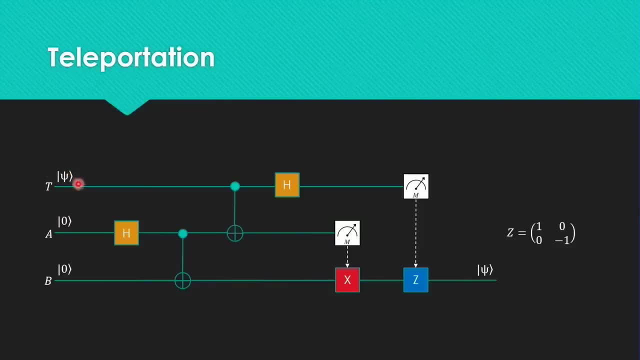 So we have the qubit that we want to be, want to teleport here. We call it t and its value is phi. It's just. this is a generic qubit value. It can be any value. And then we have these two qubits, a and b. 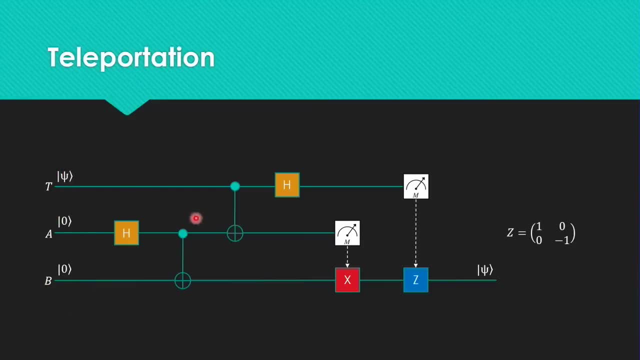 which are both initialized to zero. Now you'll recall, this is the entanglement circuit, So these two qubits are entangled. all right. Now after they're entangled, we'll say we have Alice and Bob. Alice wants to send her entangled qubit to Bob. 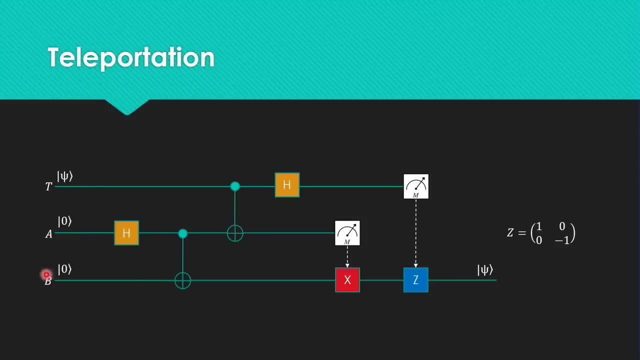 So Alice has these two qubits, Bob has this qubit And these two qubits are entangled. So the qubits are like: these two qubits are separated right after being entangled. basically, Now Alice then entangles her qubit. she wants to teleport with the other two qubits. 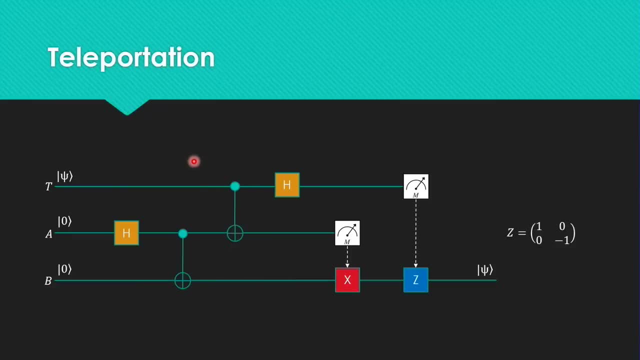 So it's a three qubit entangled system. If you were to write out the product state, you wouldn't be able to factor it into three qubits. Then she puts this qubit through the Hadamard gate. Finally, Alice measures. 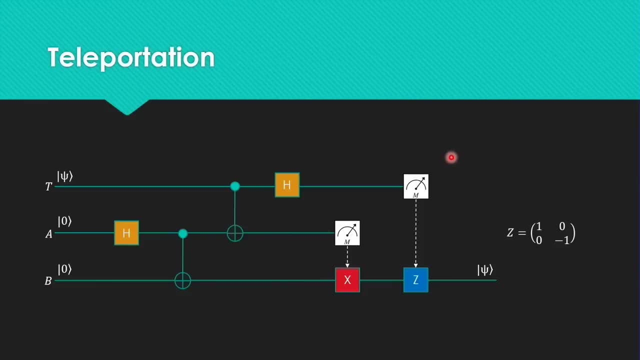 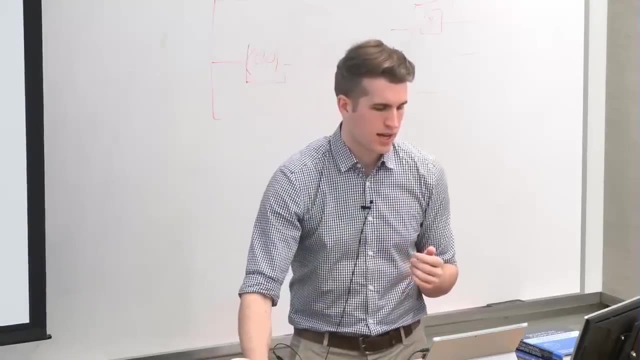 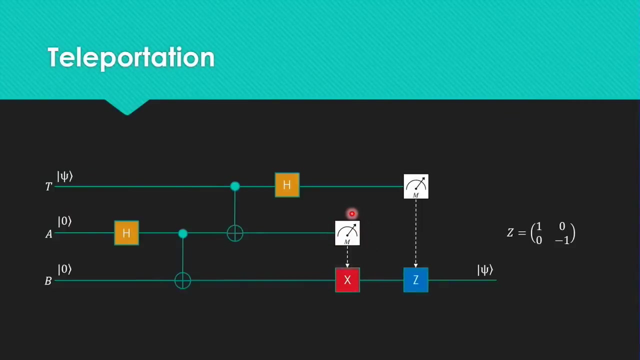 both qubits in her possession- and those are the two, and this results in two classical bits. These are the two bits that Alice has to send to Bob And the measurement result of this bit determines whether Bob has to run his qubit through a bit flip gate. 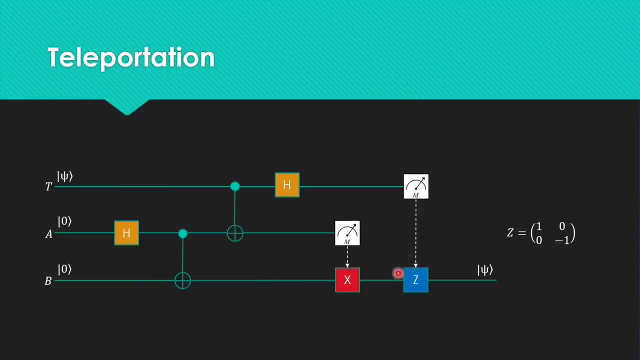 And the measurement result of this qubit controls whether Bob has to run his qubit through a new type of gate which we haven't seen before. It's called the phase flip gate or Z, And this is what they may try to do. 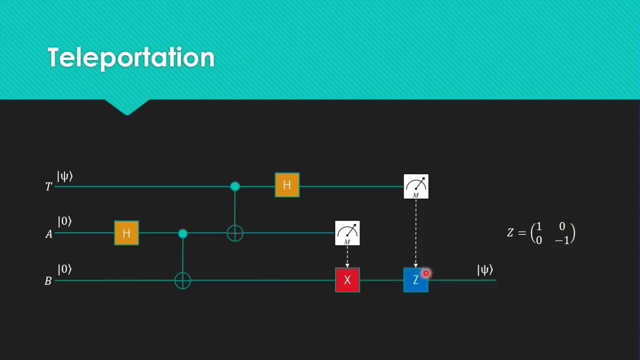 This is what the matrix looks like And basically, once Bob has applied those two gates or neither gate, if both of these end up being zero, Bob doesn't have to apply anything. He'll end up, somewhat magically, with Alice's qubit value. she. 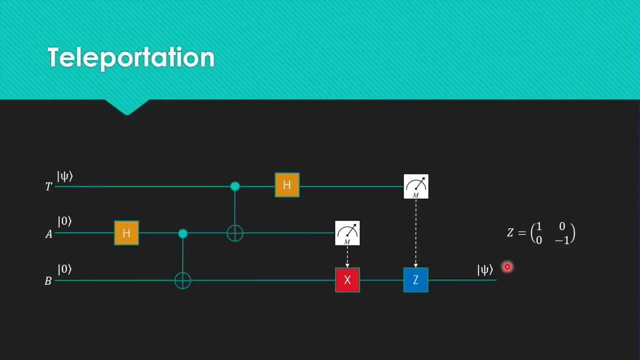 wants to teleport Pretty nifty, huh, Pretty nifty. And you might be like: well, we're already exchanging a qubit here, Why do we even care? Like we're obviously just giving a qubit to Bob. Like couldn't we just Alice, just give her a qubit. 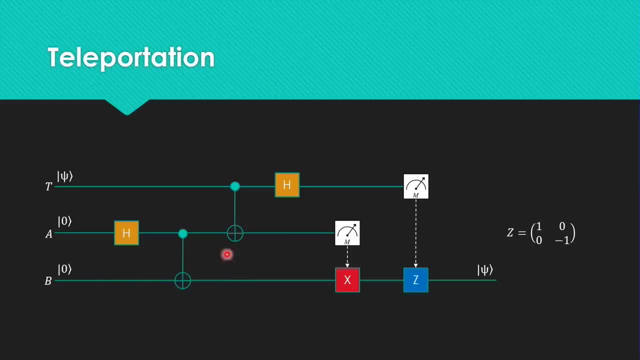 like right there, Yeah. So what you can do is you can pre-entangle like a whole bunch of qubits, like a few billion qubits or something, And then you ship them by mail. They're called EPR halves. 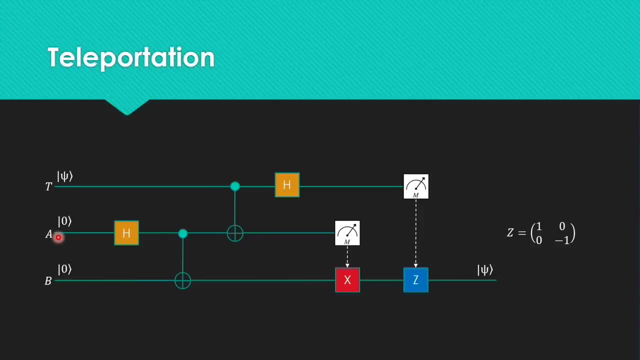 You ship them by mail or something. So Alice and Bob have a big repository of these entangled qubits And then any time Alice wants to send a qubit to Bob she can just use up one of the EPR pairs, EPR halves. 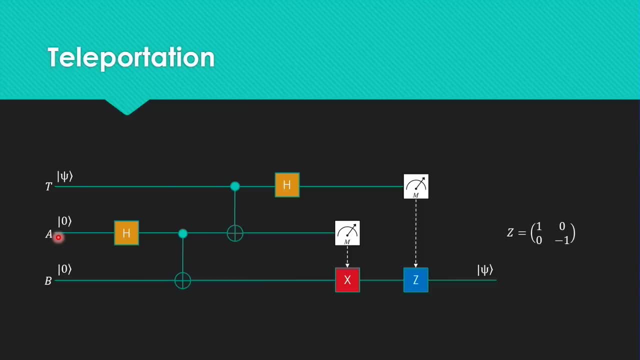 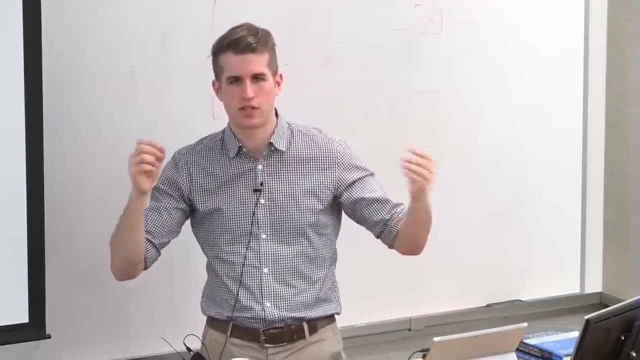 Yeah, EPR pairs- And at that point that EPR pair has been collapsed- can no longer be used, So it's a non-renewable resource. But Alice can just send as many qubits as she wants over to Bob. 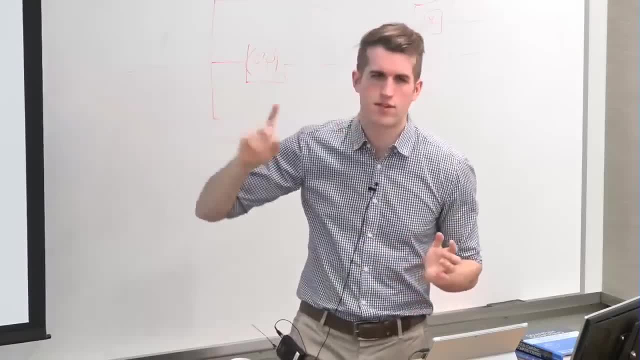 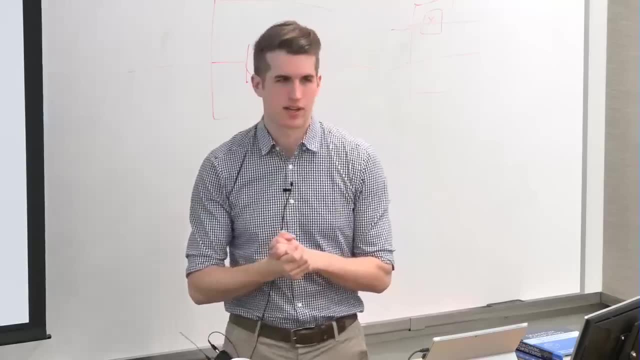 Okay. Now you might be saying, well, I don't really get this. The math is in the appendix. if you really wanna go see it, It gets pretty complicated, but I think I did an okay job of explaining it. so. 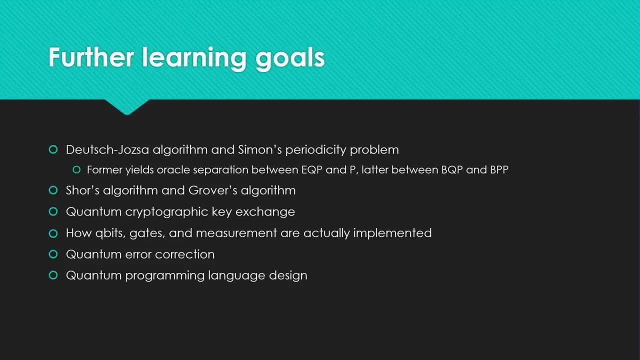 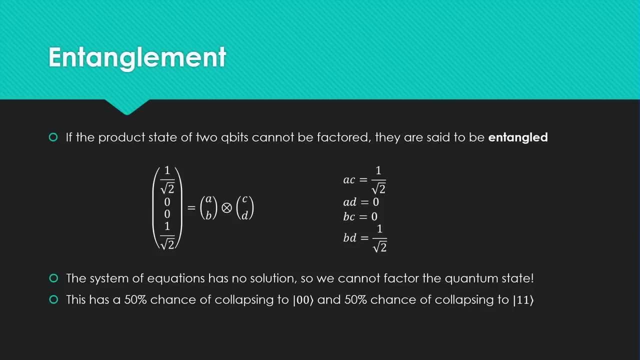 Okay, you might be like: okay, by the way, I forgot to say Really cute, really really important thing: You may have heard that we can simulate quantum computers on a classical computer, but it takes exponential slowdown or exponential memory. 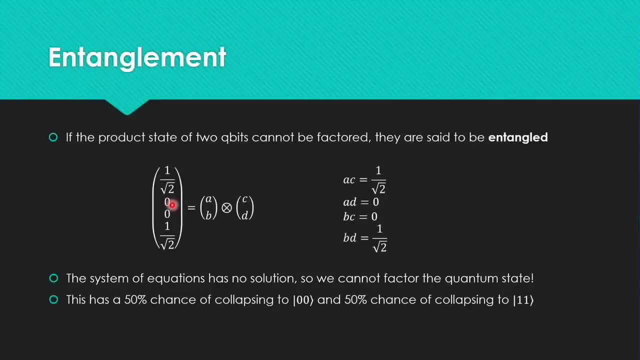 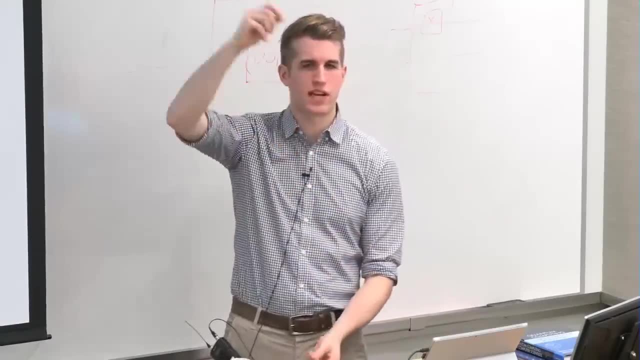 This is the reason: If two qubits become entangled, you have to keep their full product state around. So if n qubits become entangled, you have a vector of size two to the n you have to keep in memory And that is why it takes exponential memory to simulate. 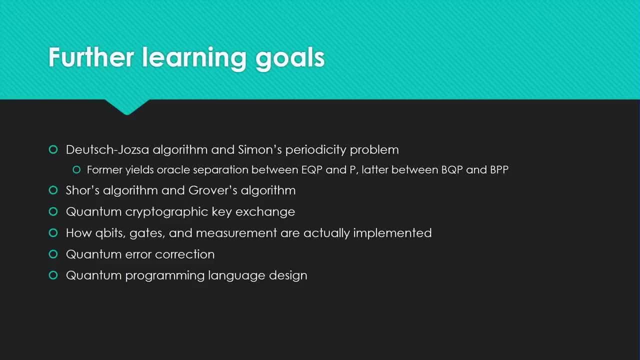 a quantum computer on a classical computer. Pretty nifty, okay. So you may be like: okay, this is all pretty interesting. Further learning goals: You can learn the Deutsch-Joseph algorithm. That's the one with n bits that I talked about. 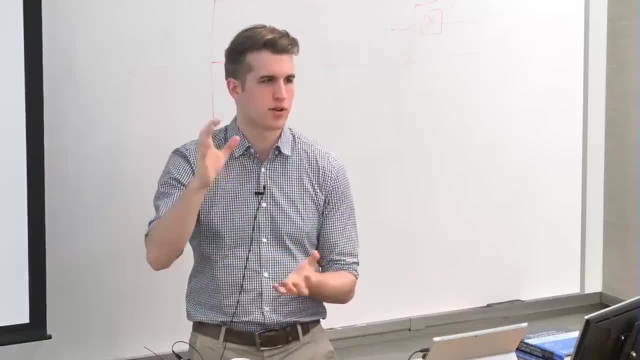 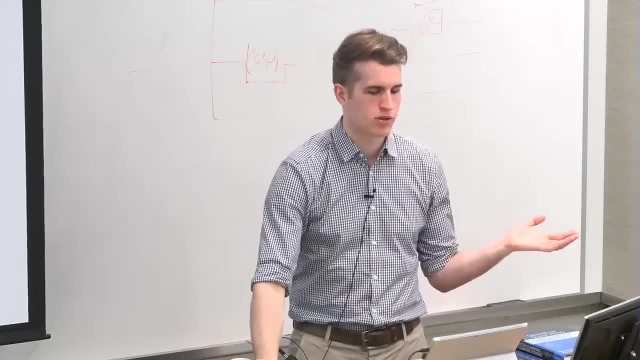 And also Simon's periodicity problem, which is another. figure out some property about this function. I'm not gonna talk about the complexity stuff, But anyway you can also learn Shor's algorithm, Grover's algorithm, quantum cryptographic key exchange. That one's actually pretty simple. I recommend looking at that. You can learn how they're actually implemented in physical terms, if you care about that. An important thing: quantum error correction. Since these systems are so small, like a spare cosmic ray could just come out of nowhere and just wreck your entire system. You need very, very stringent error correction schemes. So I think theoretically it takes five physical qubits for a single logical qubit, like we've been operating at. In practice it's looking more like we'll need one or 200 to get a qubit of 100% probability, like we've been using pretty much. 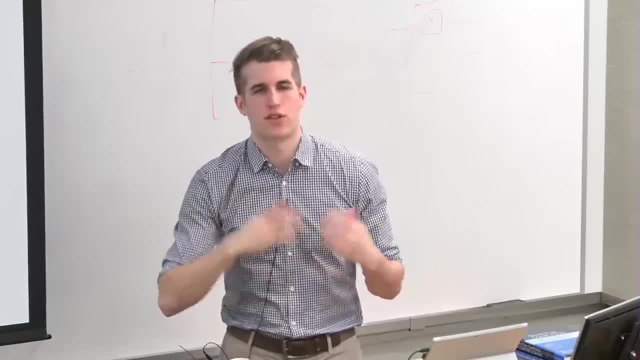 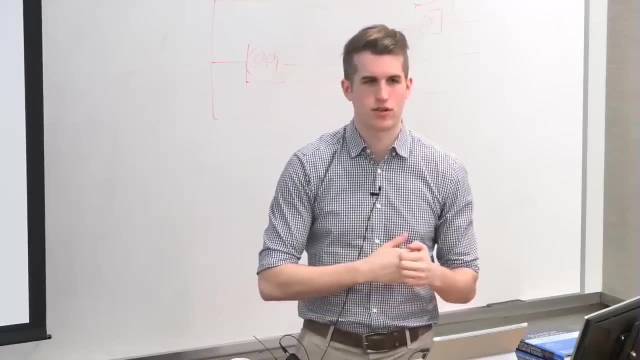 So that's something to keep in mind When we see Google's coming out with a 30 qubit computer. that maybe doesn't mean as much as we'd hope. Maybe it'll only get us two or three really high-quality qubits. 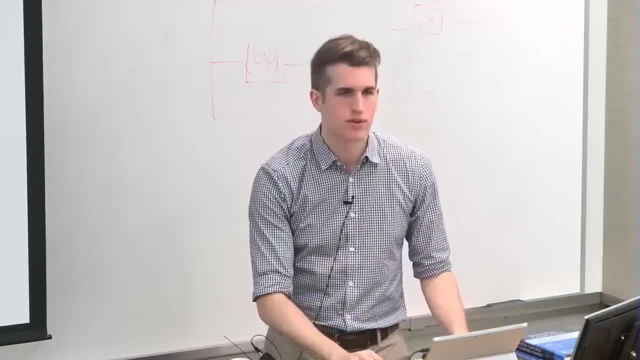 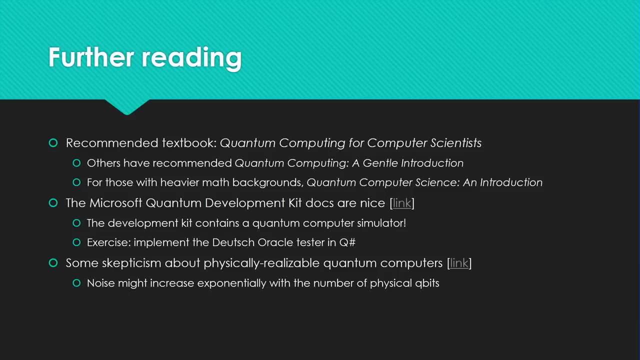 And also quantum programming language design, which I will go over because I'll show you a Qsharp example. But anyway, recommended textbooks. This one is my absolute favorite. has the same title as the name of the talk: Quantum Computing for Computer Scientists. 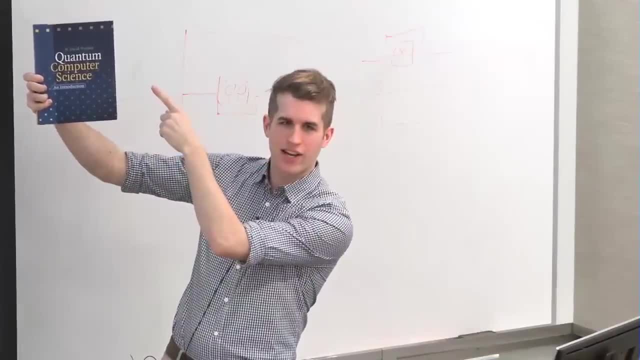 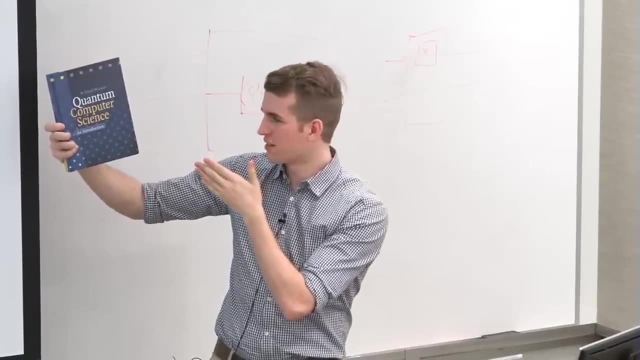 This algorithm is by our friend David Merman, the Shut Up and Calculate guy. It is a meat grinder of a textbook, But I started out with this one. it was horrifying. It was just like: but it skips a lot of steps, basically. 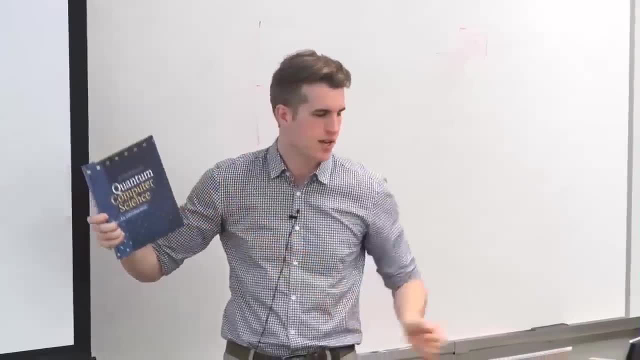 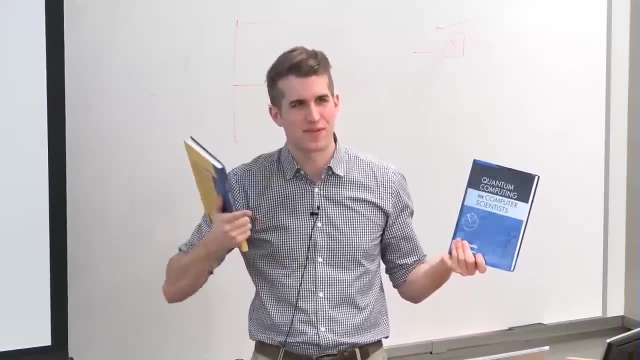 It's more symbolic manipulation. You won't see as many vectors and matrices. I like to write out the vectors and matrices to see what's going on, which gets really unwieldy when you're writing out like a 64 by 64 vector or a matrix. 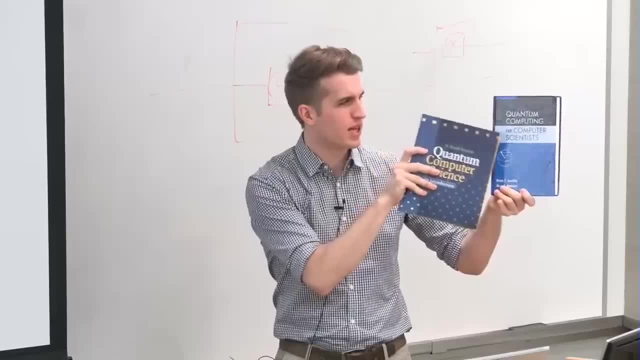 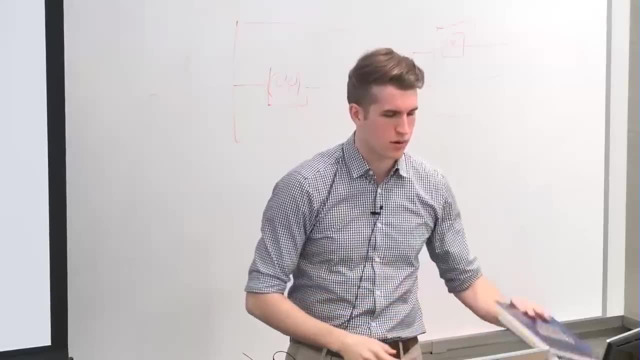 But I like to have both of these, So I'll use this to fill in the gaps with this. This has more interesting sides- stuff like that. This is also in the MS library. There's another one called Quantum Computing and Gentle Interaction. 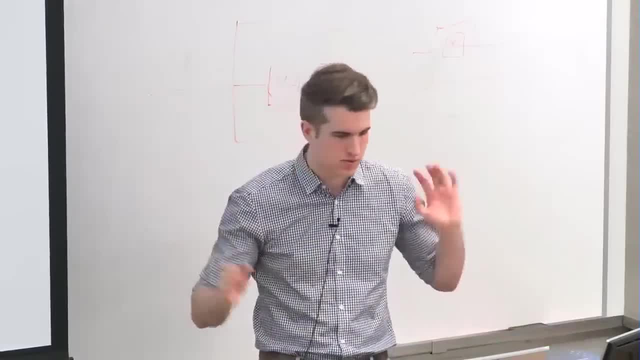 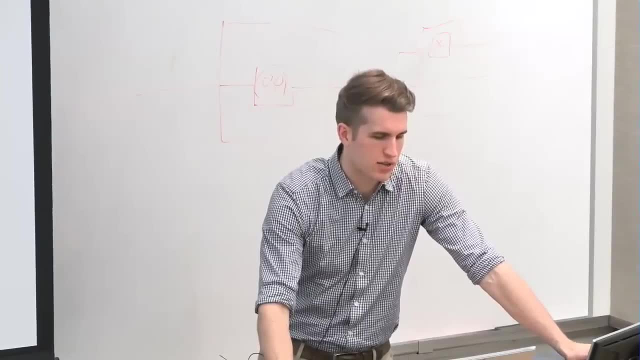 also in the MS library. I've heard mixed reviews or semi-decent reviews of it. I haven't looked at it myself. There's also Microsoft Quantum Development Kit. They have the docs. They're actually pretty nice. They include a quantum computer simulator. 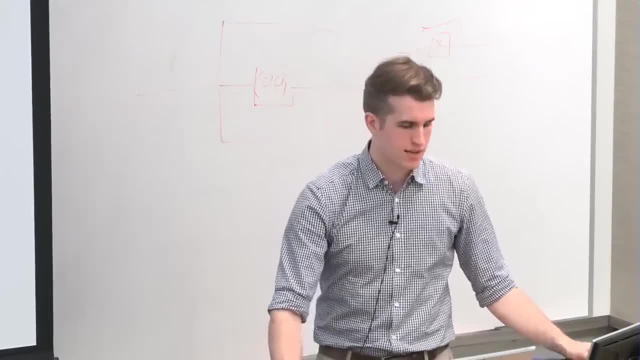 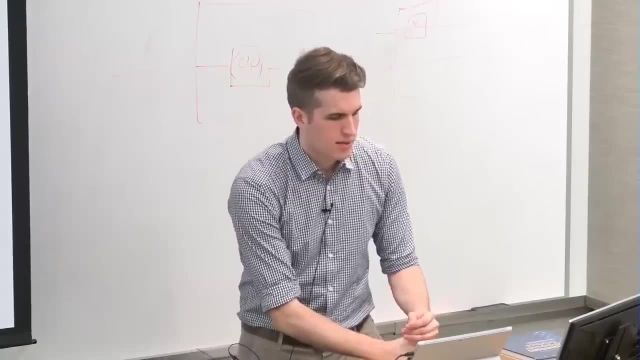 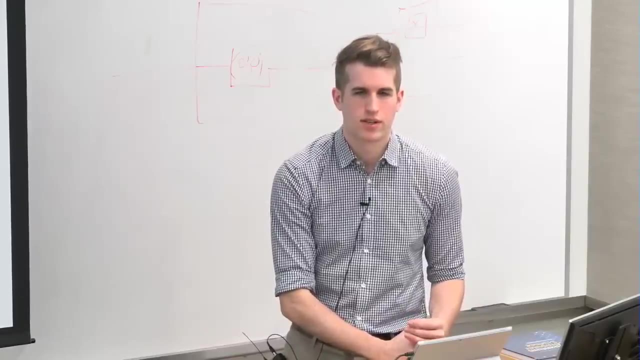 and Q-sharp, as we'll see Now. I said I would end the talk on some skepticism which there's. an article came out- I think it was Quantum Magazine, pretty prominent recently, Interview with a mathematician who believes that physically realizable quantum computers cannot exist. 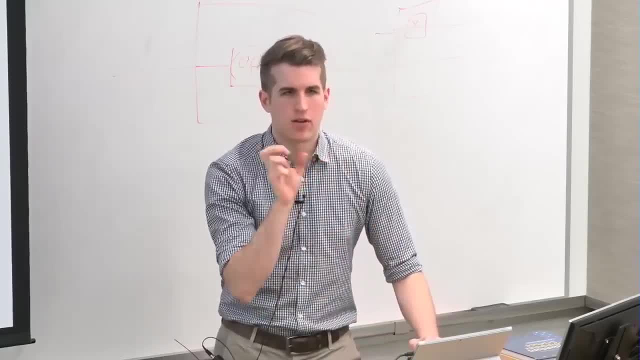 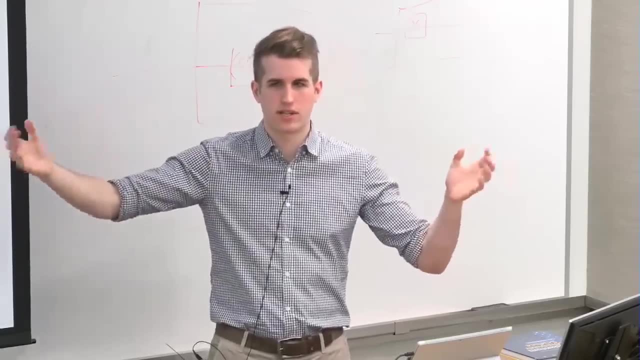 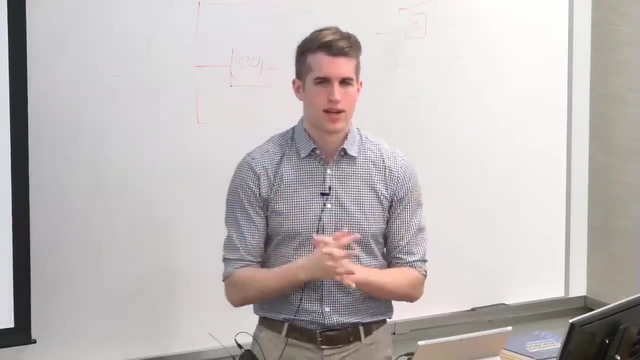 His basic argument- simplifying- is that the amount of noise in the system grows exponentially with the number of qubits. So we cannot get a really large qubit system because our computation will just keep collapsing in the middle of it and it's just like an exponential term. 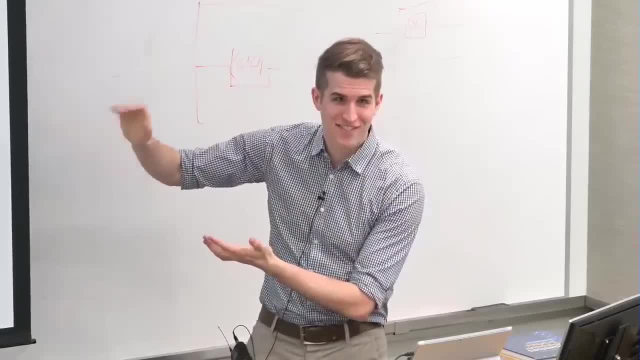 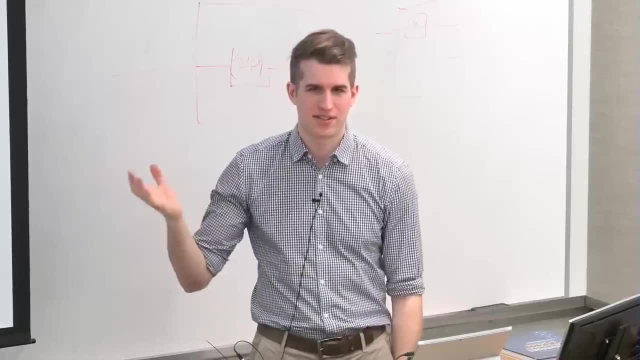 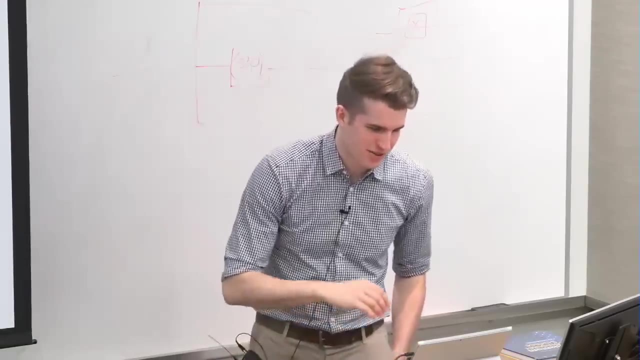 And so I would be very sad if this happened. I'd feel like the universe is against me. It'd be very sad if we could not realize the benefits of quantum computing- Some like cosmically sad. But anyway, you can't argue with the universe. 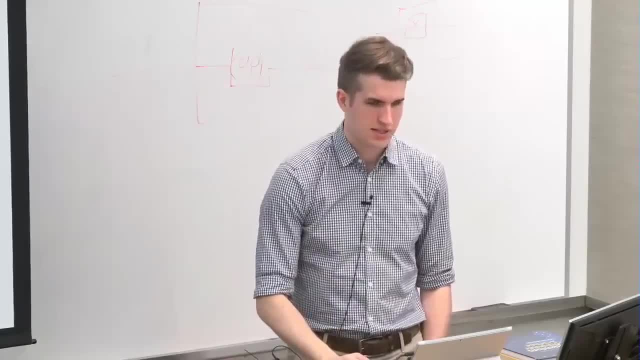 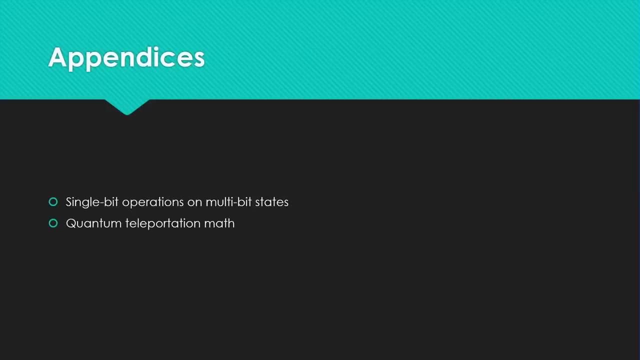 And, yeah, you can read that article for some skepticism. I think his name is Gil Kalai is the mathematician. There's some appendices, but I'm going to do some demos now. Okay, The first demo is just the Deutsch article. problem in Q-sharp. 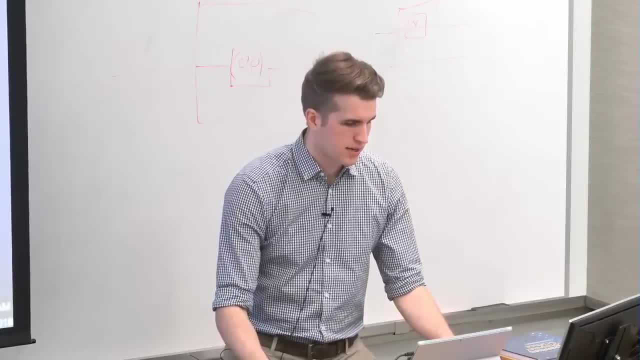 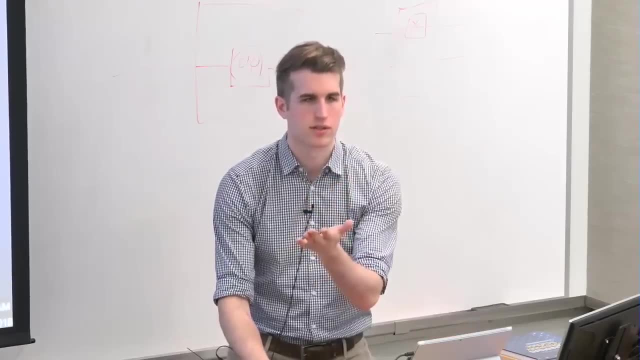 So Q-sharp is based on F-sharp and we have this function I've written is black box constant. You take in a black box and I tell you whether it's. oh gosh, sorry here, of course. 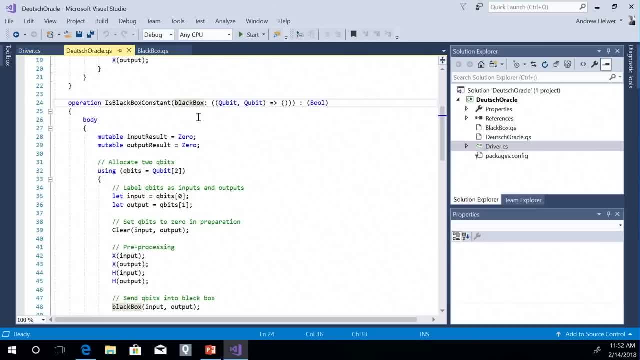 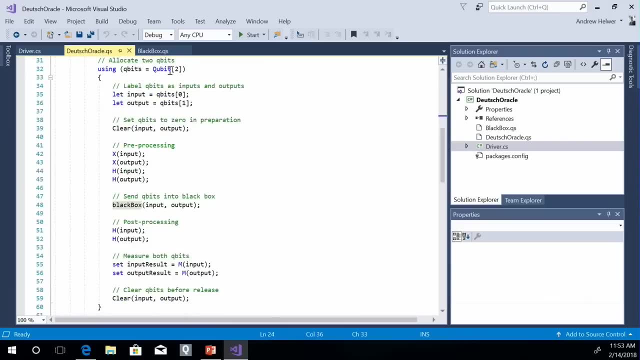 Okay, We have our function: is black box constant, where it takes in a black box and it just returns a bool- Is it constant or not? And it just uses the same protocol we went over. It allocates two qubits. 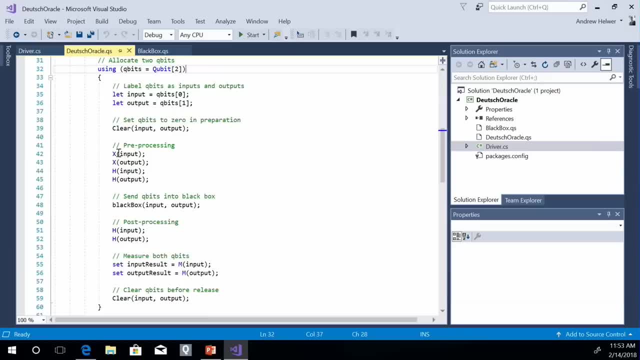 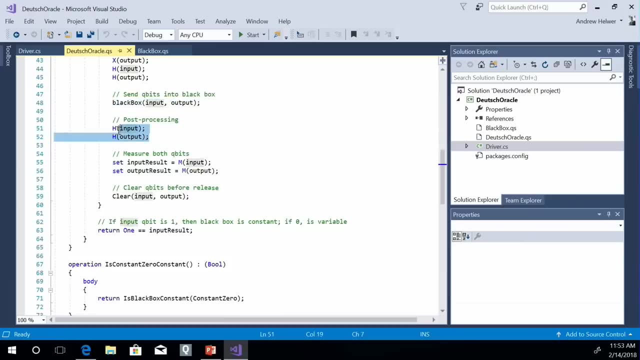 calls one input, one output, clears them, sets them both to zero, does the pre-processing, flips them, puts them through the Hadamard gate. Then it sends them into the black box. Afterward it again puts them through the Hadamard gate. 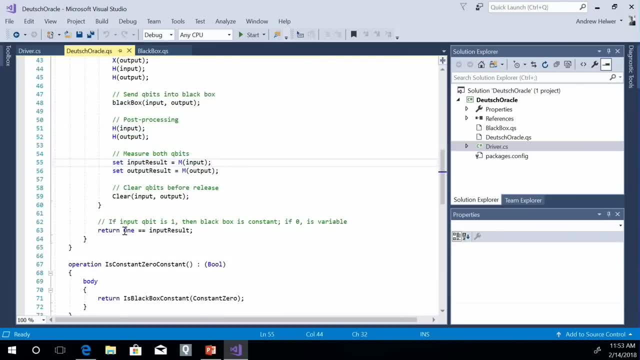 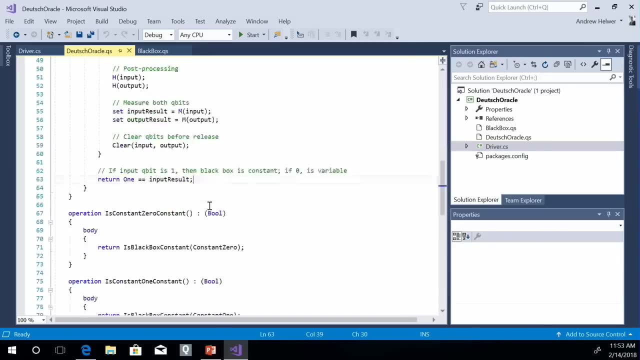 and then it measures both of them. And again, if the input result is one, then it's constant, otherwise it's variable. Okay, We have our black boxes defined here. So constant zero. again, remember it's nothing. For constant one, we flip the output bit. 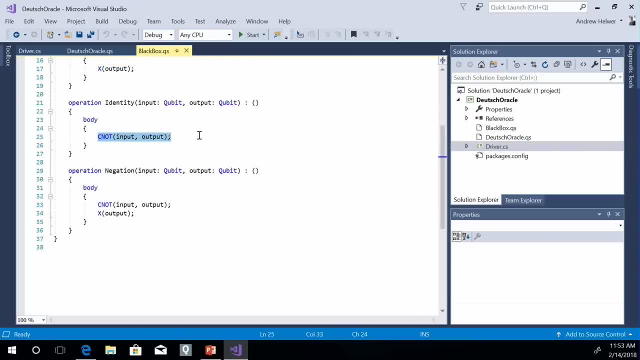 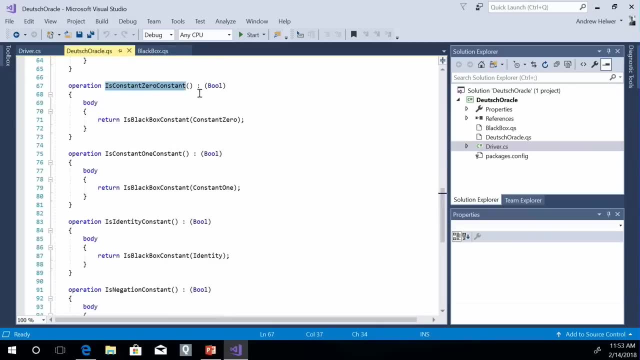 For identity. we run a CNOT gate with input as control, output as target and negation we use CNOT next. Okay, And we just have these like: is zero, constant zero, I call is black box constant with constant zero. 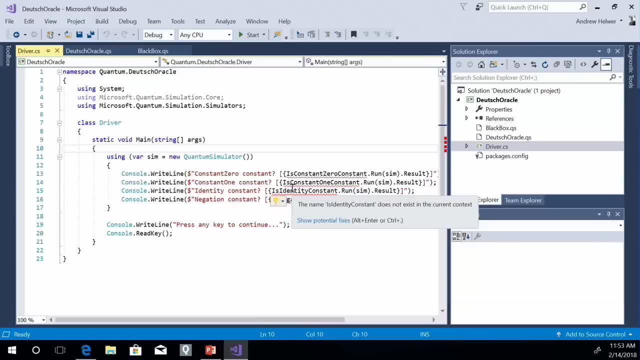 And then we have our classical driver. Any quantum computation will have a sort of classical computer to tell it what to do, And so I ask for each of those four: Well, what's going on? And we can run it, and it runs on a simulator. 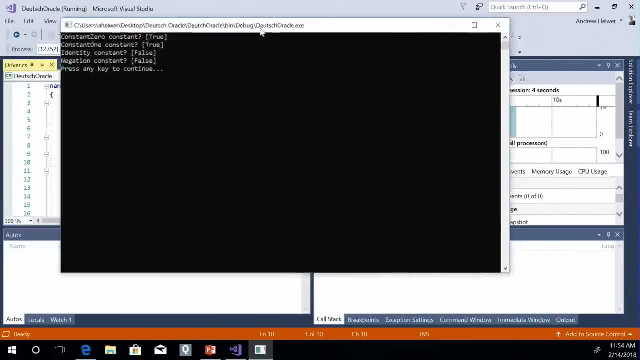 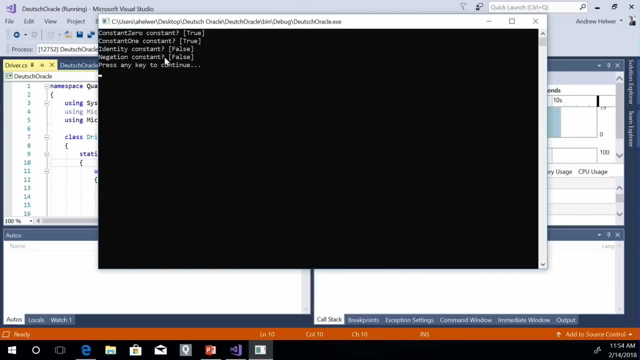 and we see the output Is constant, zero, constant True, Constant one, constant True Identity, constant False, Negation, constant False. So there you go. Yeah, we wrote the do-it-your-call, ran it on a real quantum simulator. 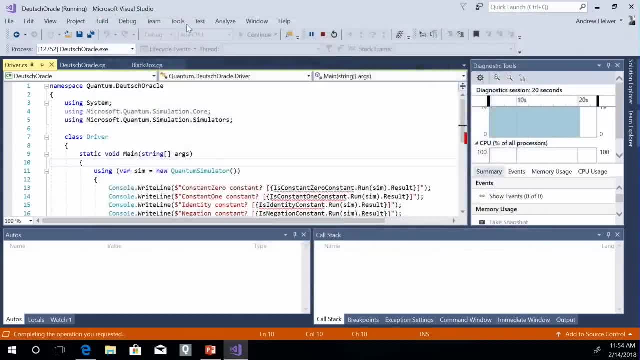 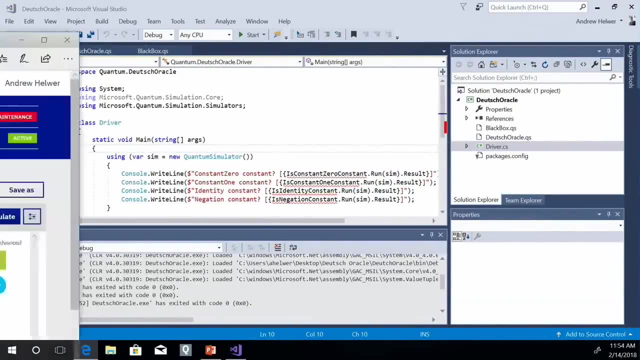 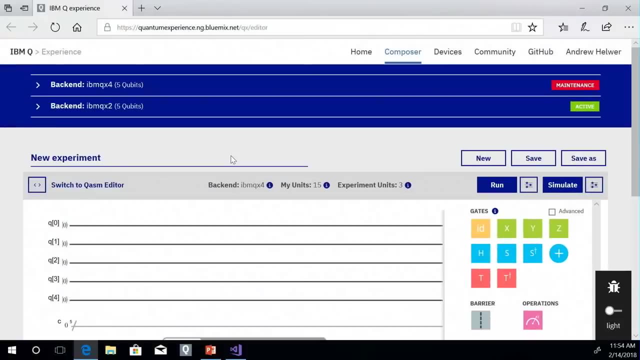 We saw that it worked out. Okay, The final demo of the day- and then I'll let you get out of here is here we go. This is called the IBM Quantum Experience. There is a real like world quantum computer that IBM has built. 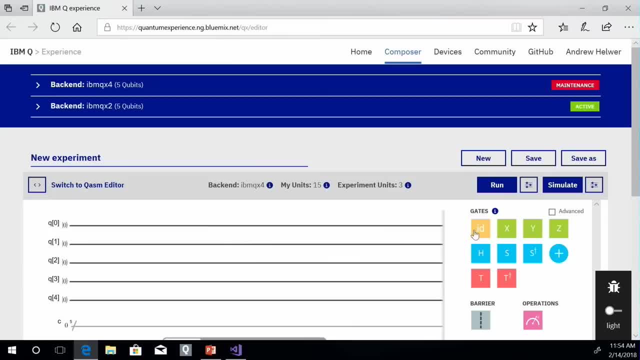 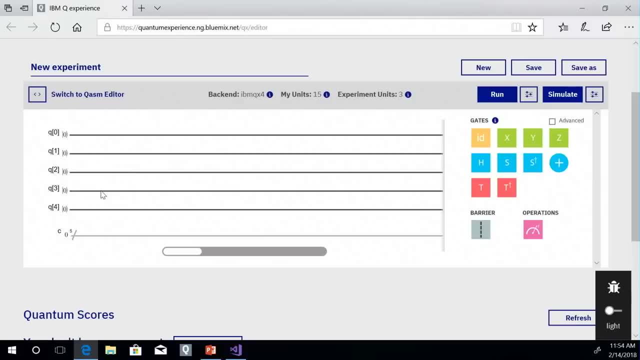 It only has five qubits But they just let you online just drag gates onto this quantum circuit diagram and run it on a real quantum computer. So I thought it'd be pretty nifty if we demonstrated entanglement right. 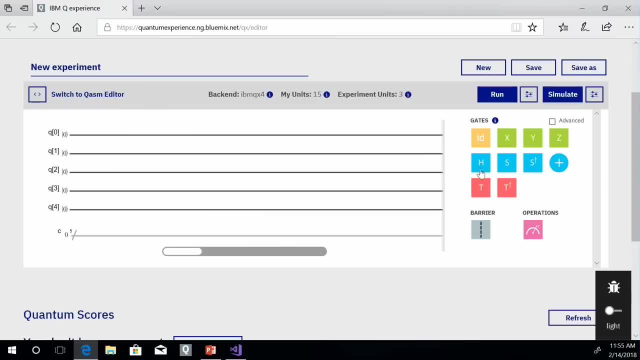 Live for you on stage. Let's see. So, if you remember, the first thing we do is you drag a Hadamard gate onto one bit and then we use the control knot. Oh no, Okay. So the way. 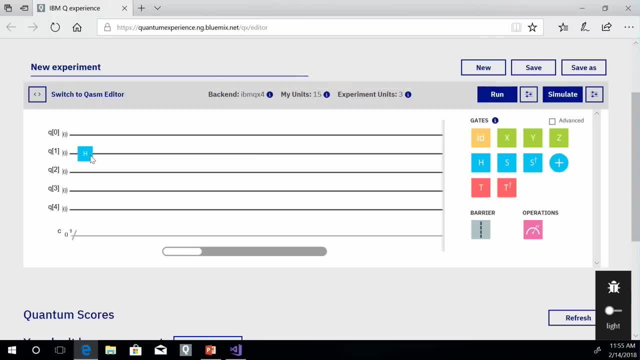 the quantum computers are constructed, you can only usually put C knots between certain bits. basically, It's just kind of otherwise, it's just mechanically impossible. Let's see, Can we do that? Nope, Okay, How about success? 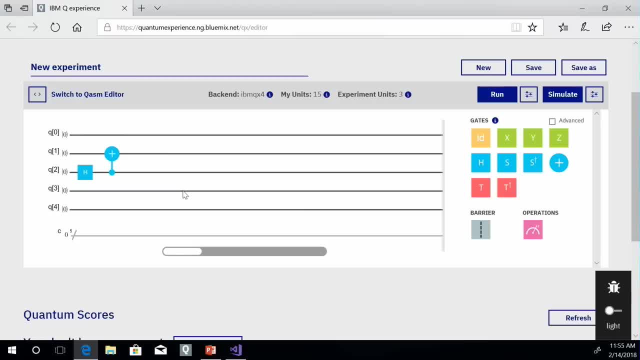 Okay, We did it. Here is our. this is the C knot gate. You can see varying representations of it. It's like the O plus And I say we'll run it on a quantum computer. All right, Measurement gates. I forgot. 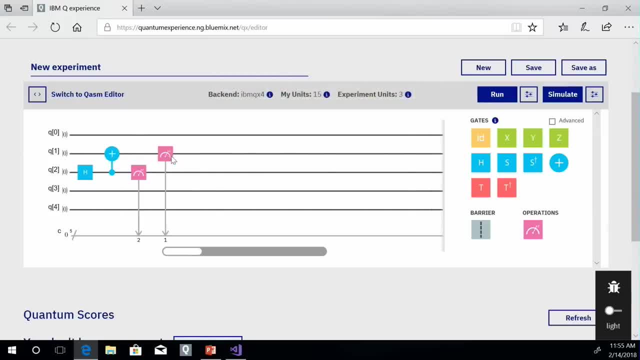 We need to add the two measurement gates, obviously. So we're measuring both of these qubits after entangling them, And what we expect is to see them predominantly being 0, 0, and 1, 1, right. 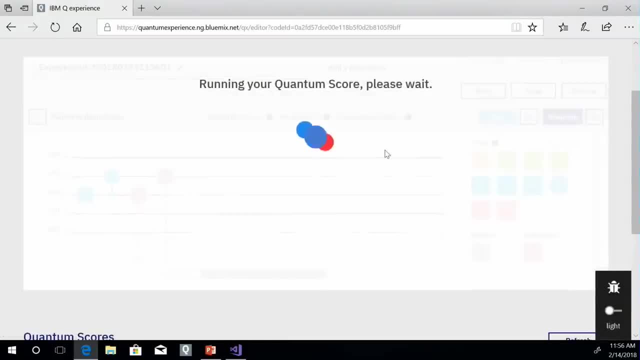 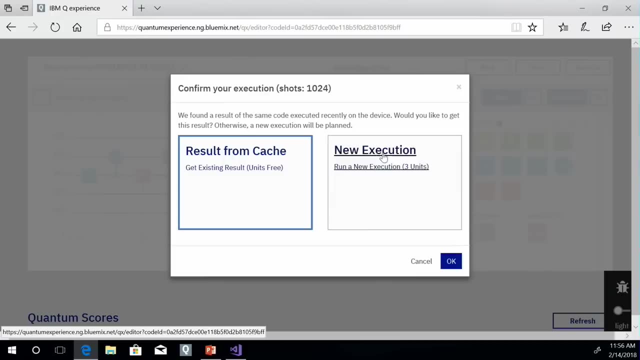 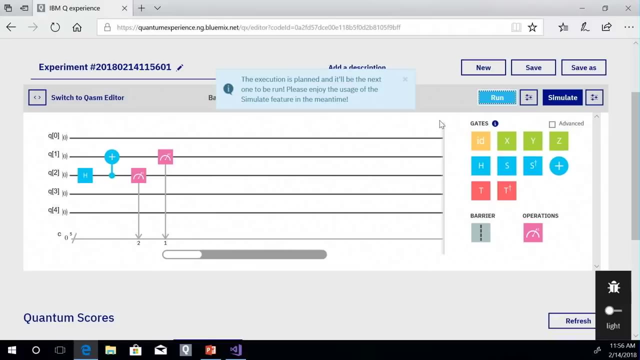 Well, let's test it, We'll call it that And we can say the result from cache. but I want to do it live for you guys. So I'm going to run a new execution And you can imagine right now, deep in an IBM research lab. 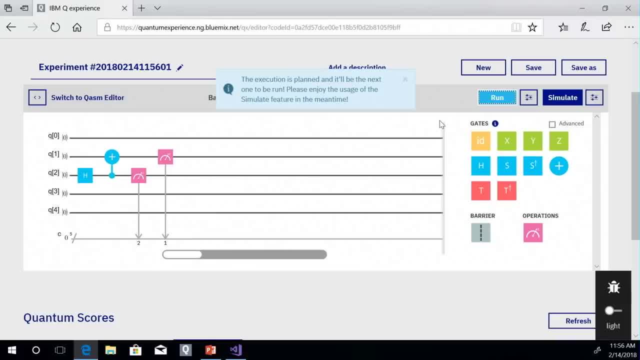 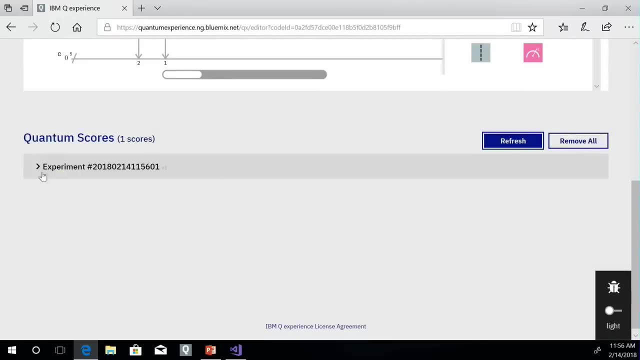 nestled within a dilution refrigerator operating at slightly above absolute zero, we have real qubits being entangled and measured thousands of times for our entertainment. That's pretty cool. That's pretty cool. Okay, Let's see if it's. oh, here we go. We got the results and executions. 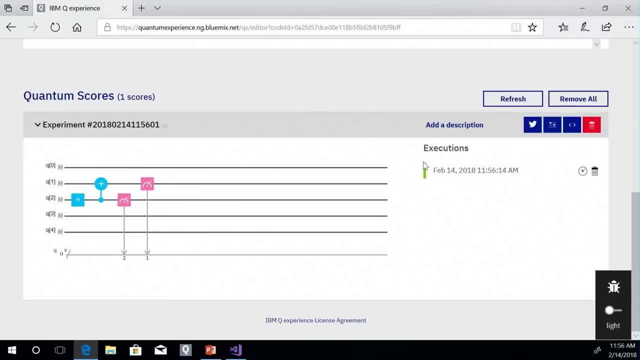 Is it? it's pending, Okay, So it might take a couple minutes. We can just hang out. Does anyone have any questions while we're waiting for this? Yes, I have another question. You said this experiment where they sent an entangled qubit up to space in a satellite. 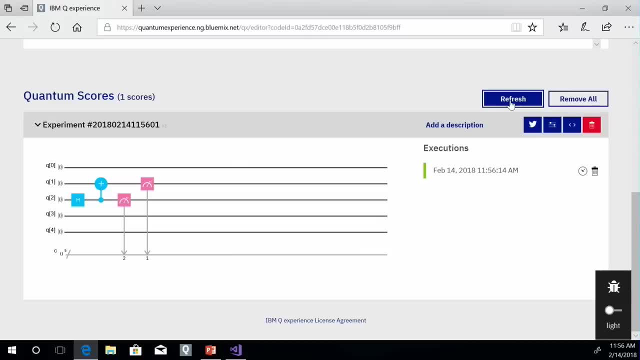 Yes, Are we good at storing like qubits for a long time? I'm really surprised they were able to do that. I thought they kind of-. Yeah yeah, So that was actually a lie. They managed to send the entangled qubit up by a laser. 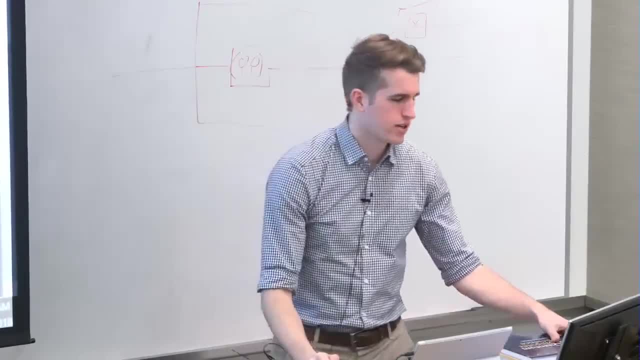 But yes, Oh okay, I don't think we're that good at storing qubits for a while. I think they're fairly short-lived. That's what I thought. Yeah, I thought maybe there was something, But yes, They actually. 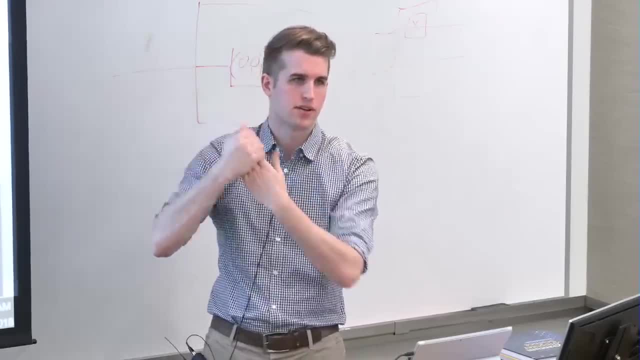 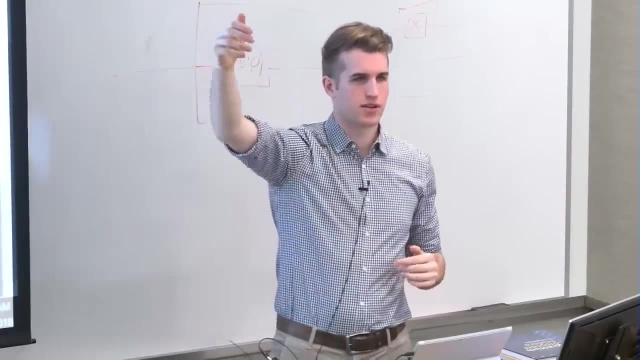 the Chinese satellite experiment. they teleported a qubit up there. Oh, okay, So they sent one EPR half up by a laser and then they use that EPR half to teleport the qubit up there. Pretty cool, That's awesome. 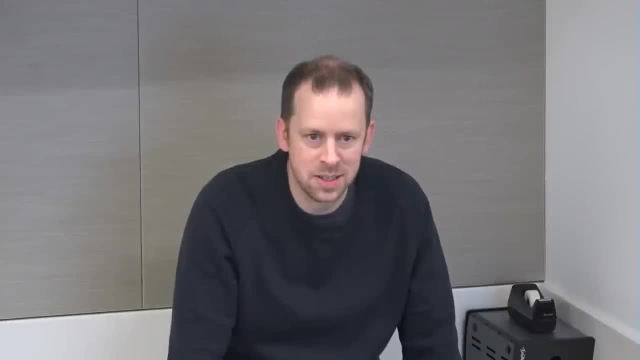 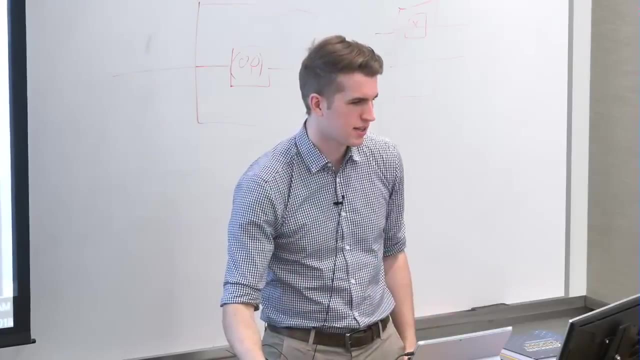 Yeah, So we can send entangled qubits by laser. You can send entangled qubits by laser. Yes, Okay, That's even cooler. Yeah, Let's see It's still not. Okay, That's fine Anyway, yes, 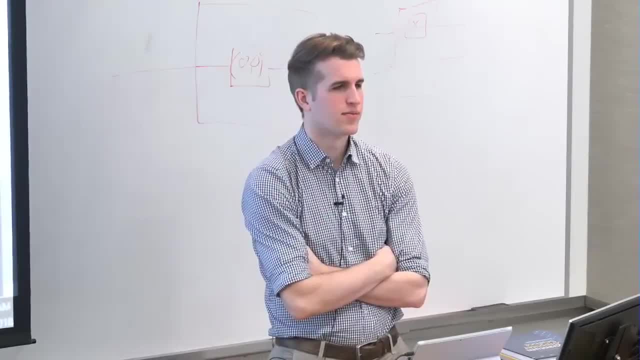 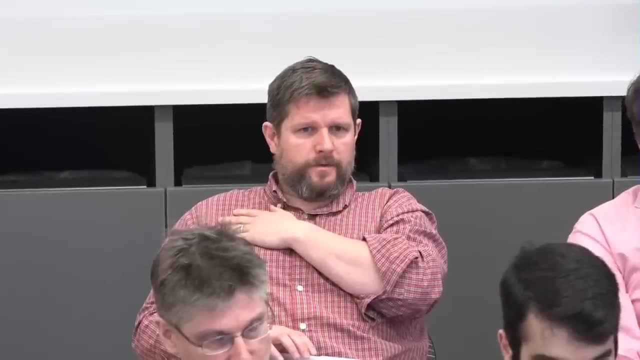 You mentioned that there was this new article by the mathematician that said: the noise is going to grow faster. Yes, But the whole purpose of the topological quantum computer was to resist that. Of course, Any quantum computer will have issues with noise. 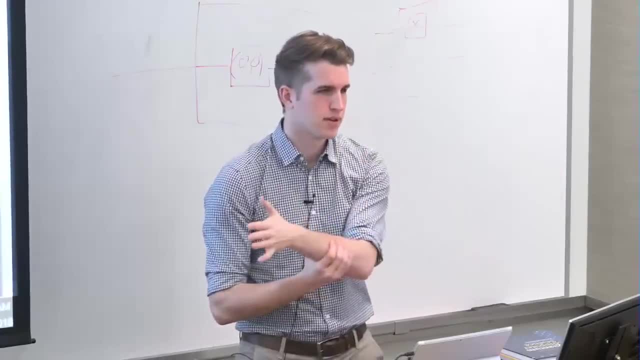 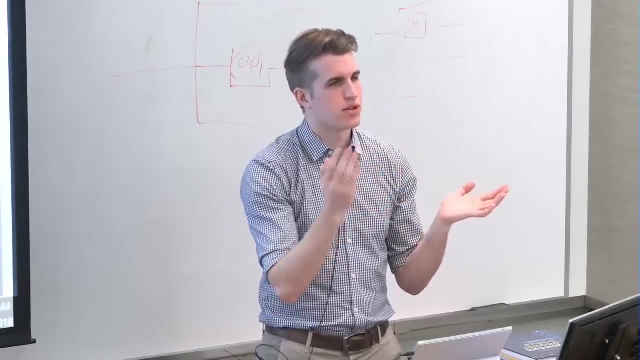 The topological quantum computer is supposed to be better than its IBM counterparts in terms of noise, But it'll still grow exponentially Like. it can still be better, but it still runs with the exponential barrier, And so this, the next couple of years, are really sort of. 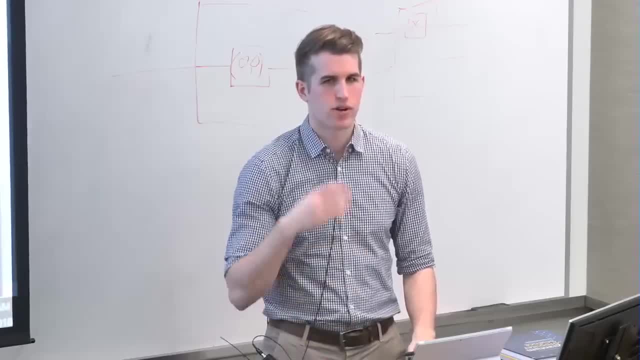 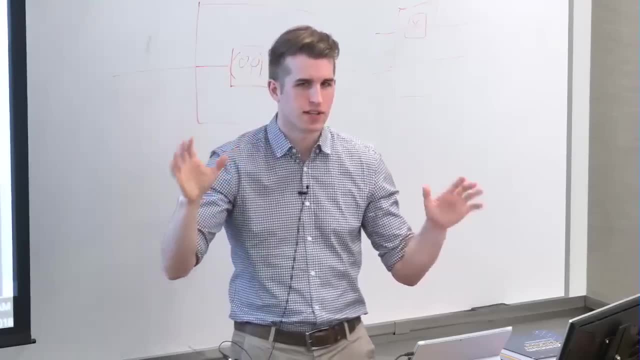 a make or break for quantum computing, Because we now have the ability to create computers which run into this exponential term, if it exists, if it exists, And so we will see within the next couple of years whether quantum computing is really possible or not. 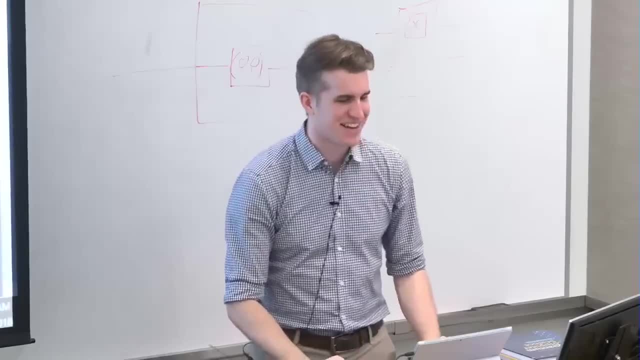 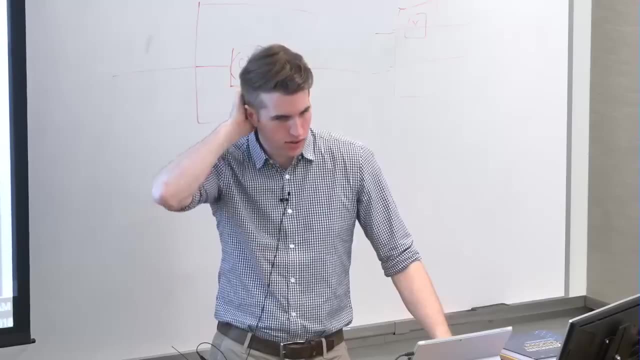 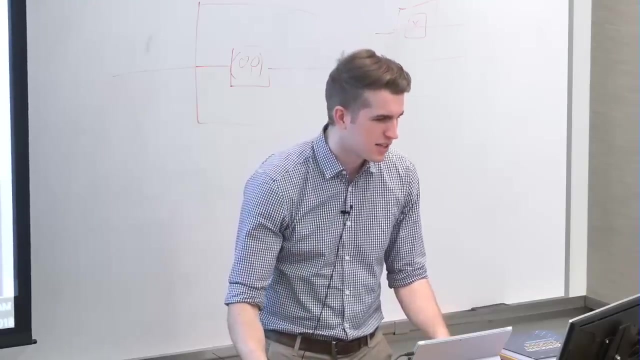 It's nervous, It makes me nervous, But yeah, because we'll run into this limit, probably like this year, If Google does not manage to demonstrate quantum supremacy. it'll be a bit scary, I guess. But yeah, Let's see, We don't have. 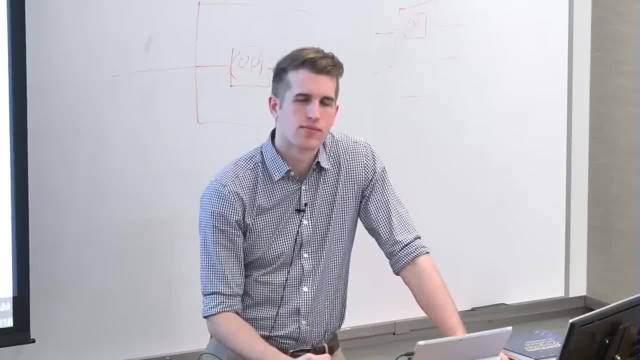 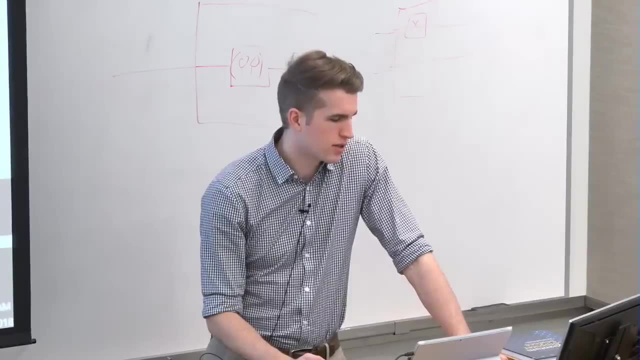 I think I'll just refresh the entire Question. Yes, Do we know what Google uses quantum computing for? Like what? What they use it for? Yeah, yeah, yeah, I don't believe we do, I think they just have. 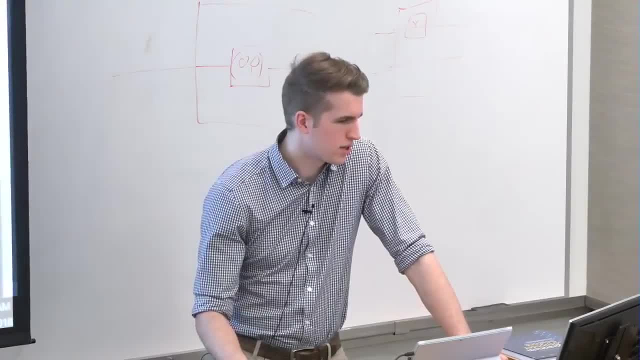 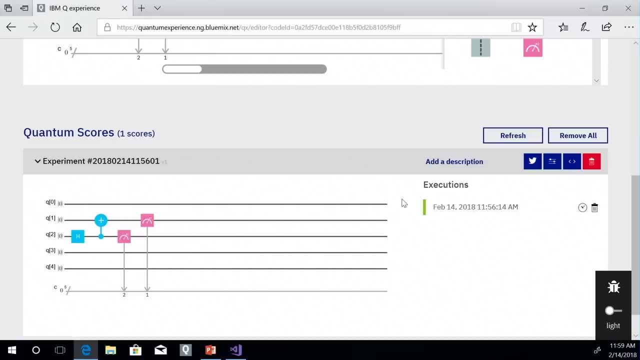 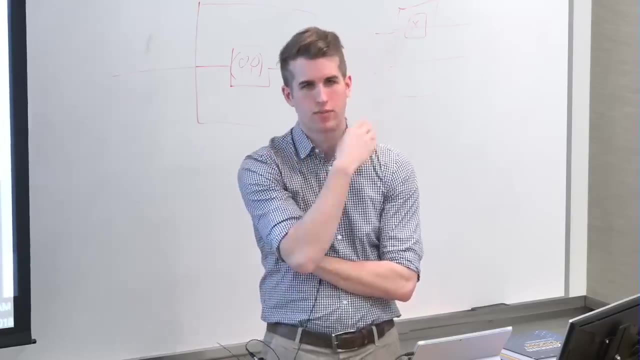 Is it experimental? It is Actually no, They haven't announced what they use it for. My manager is actually playing around with the D-Wave simulator. to D-Wave is a Canadian company. Yeah, Everyone's like. everyone thought they're. 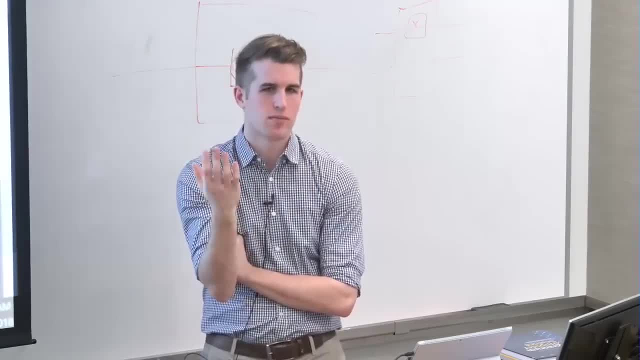 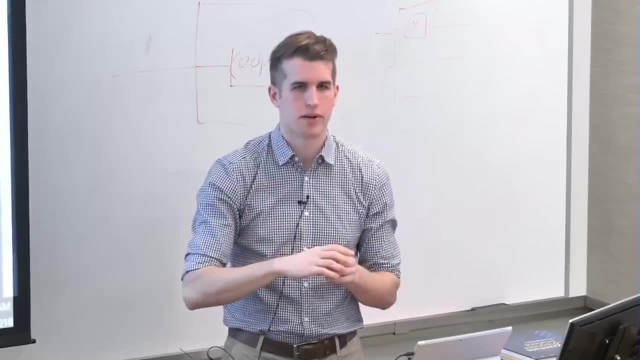 like really scammy and not really quantum. Now, everyone kind of believes that they're quantum but it's a different paradigm. It's like optimization basically, but it uses quantum computing. They have a simulator you can use. My manager has been using it to kind of play. 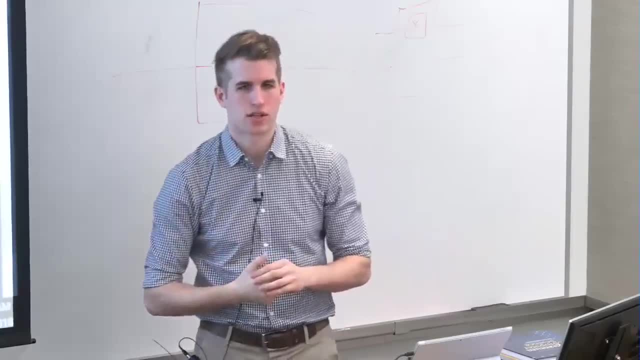 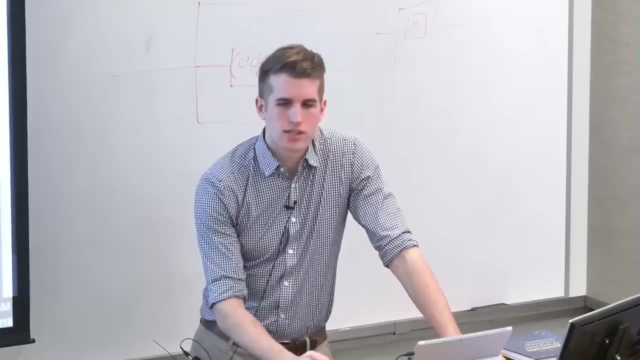 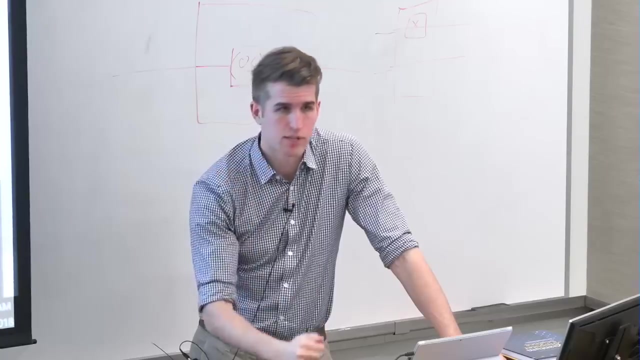 around with finding routes in the network. It has like general applications like that. Well, this is taking a while. Is publicly available somewhere? Yeah, It's in the invitation And I think it'll be probably be posted on the ResNet website or I'll post it online. 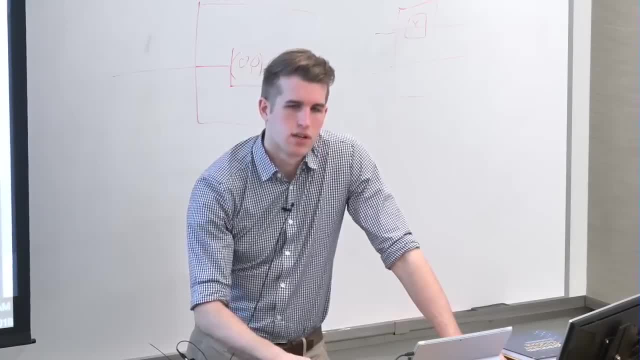 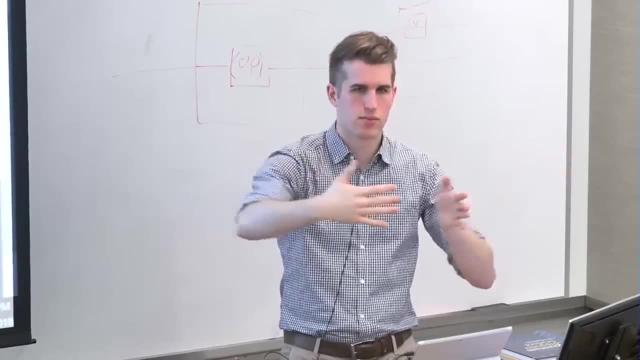 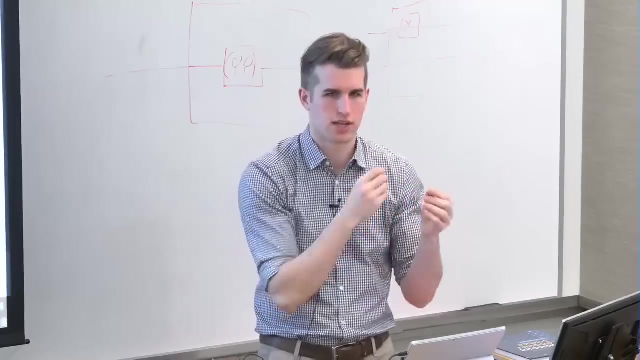 So that application is like a graph search type of application. Yeah, Yeah, It's optimized. You're able to express the network graph in terms that, like, an optimization result would be the least energy path, in terms of, like, the least cost path through the graph, sort of. 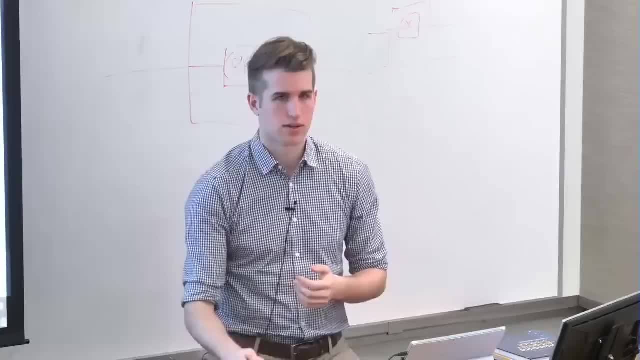 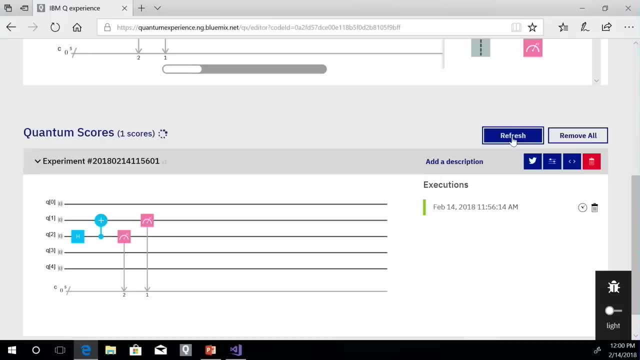 So that's different than the way that, than the paradigm. Open, shortest path it's- Come on, why isn't it going pending? I'll be really sad if this doesn't finish in time. Oh well, So on D-Wave, I saw a presentation. 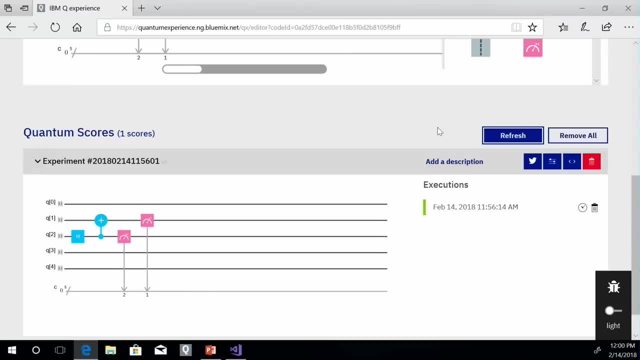 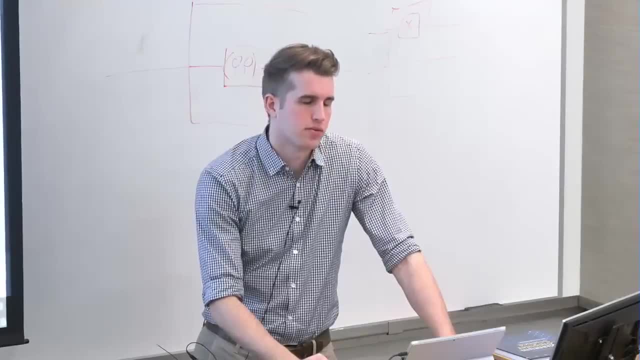 Someone was saying that you could do classically faster than what they were able to do on D-Wave. So they've improved it now, or what's changed? I don't know. Actually I haven't looked into that, It's probably. they're probably about comparable. 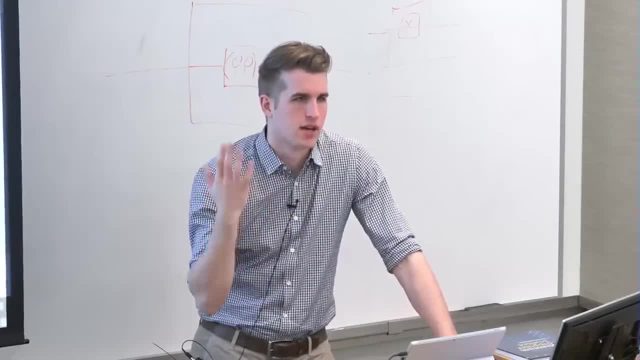 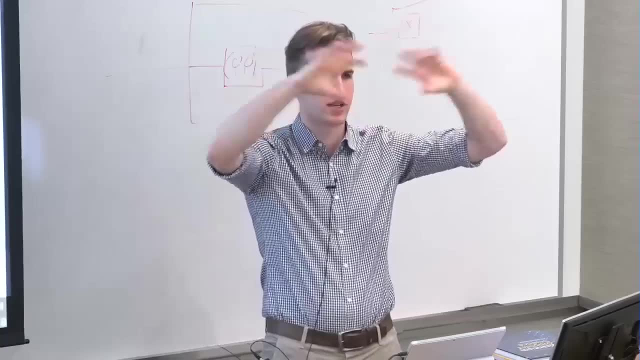 I would say because, given that it's just like optimization and especially with the explosion of machine learning, there's been a lot of development in making optimization better. Optimization is like you have a surface and you're trying to find, like the highest point or the lowest point. 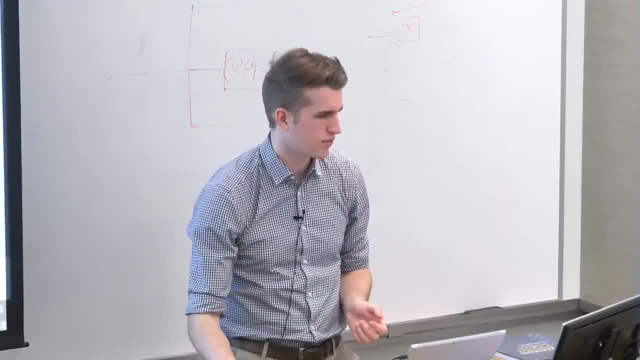 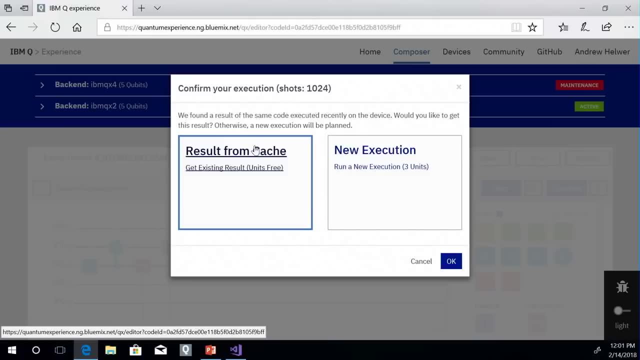 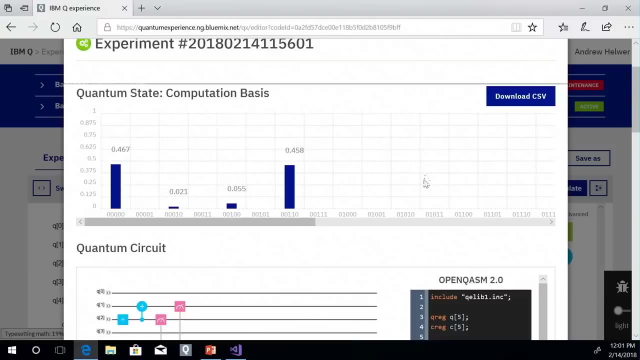 So there's been a lot of research that goes into that. Well, that's how about we here? we'll just run it from cache And okay, Here we go. Okay, So here's the results from cache. 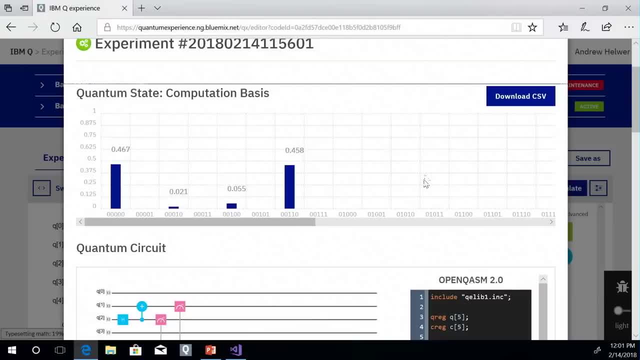 Unfortunately, our real execution didn't finish yet, But so we see that indeed they entangled some different qubits than ours, But we end up with zero, zero and one one, almost exclusively. But then there's some in the middle. 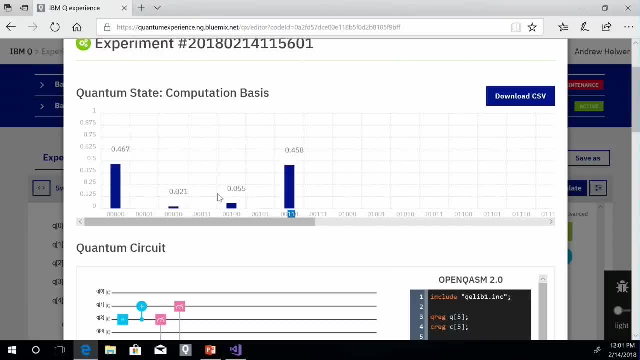 because of the error rate, right? So this is on a real quantum computer. We have some error rate where it doesn't exactly work according to our model all the time. But pretty cool, These are entangled and they're measured and we have that. 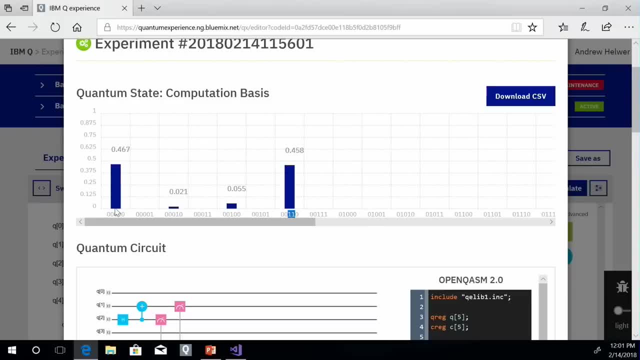 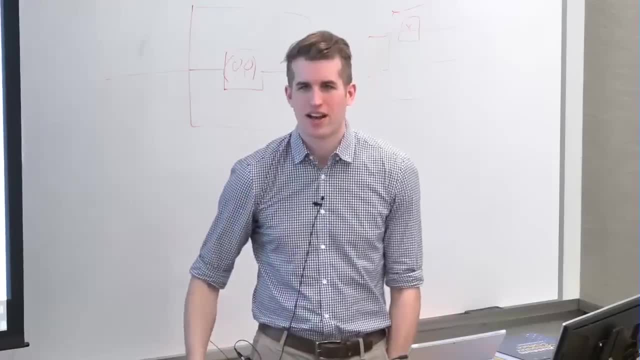 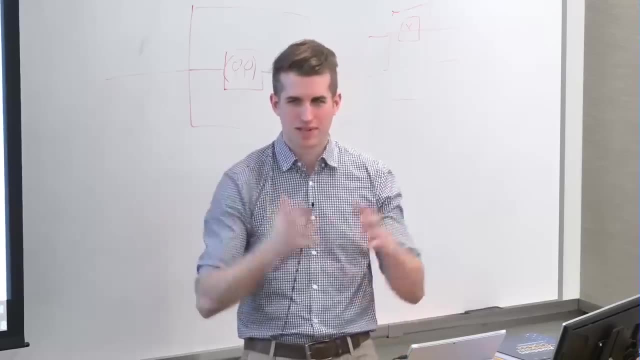 That's the experimental data. right there, That entanglement is a real thing, Yeah, Okay. That concludes the presentation. Thank you very much. I hope you all feel as though you followed the whole thing- no real confusion- and feel that you could keep on learning. 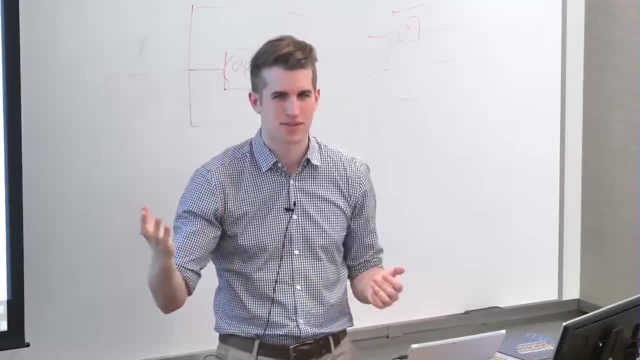 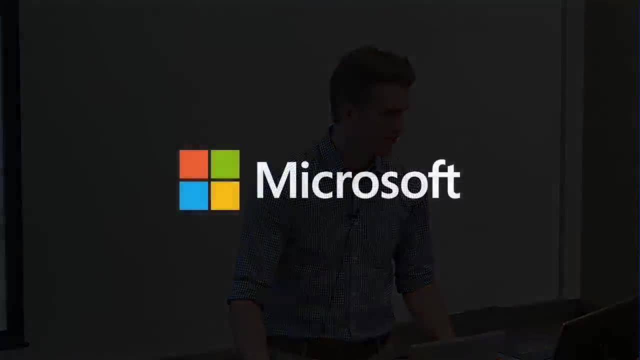 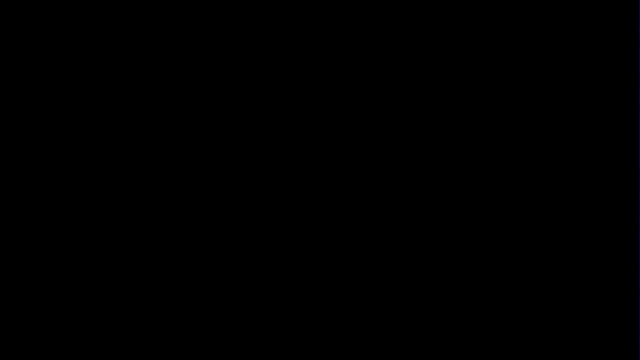 This isn't like mad genius science. This is very accessible science. So yeah, Thank you very much. Thank you very much.